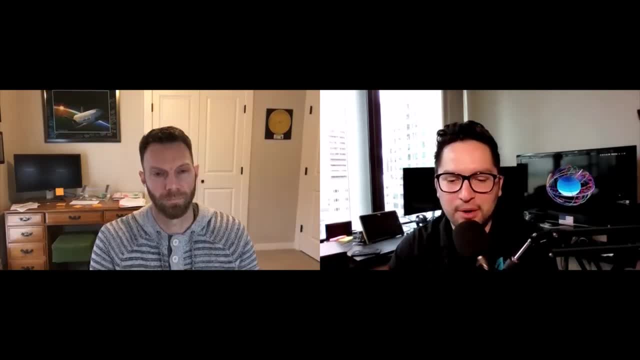 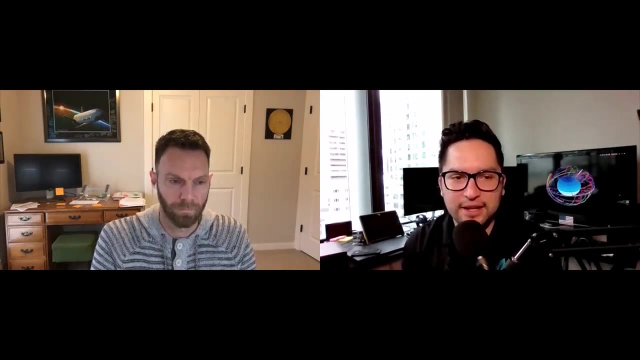 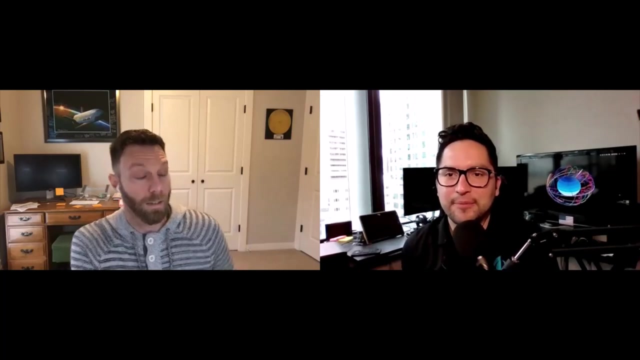 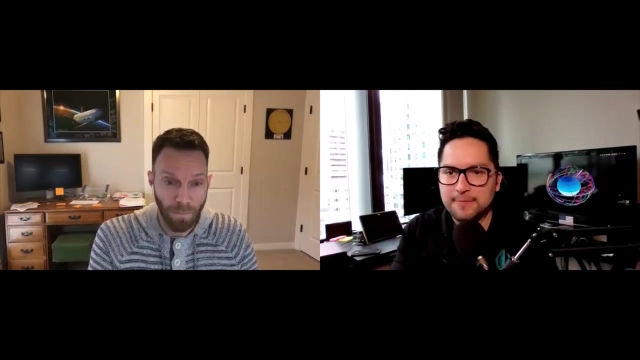 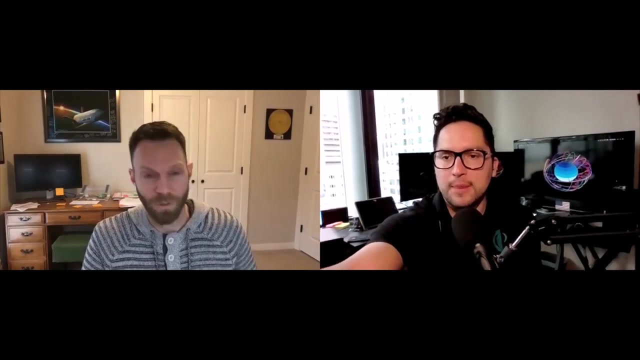 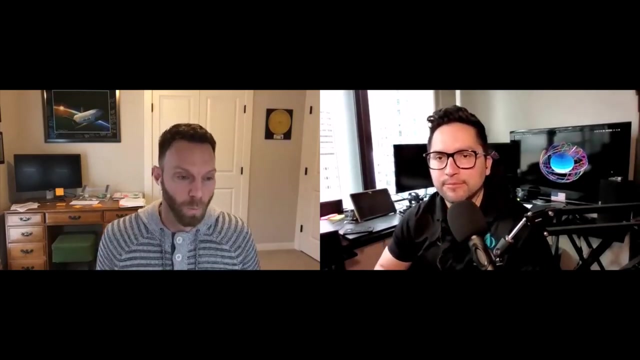 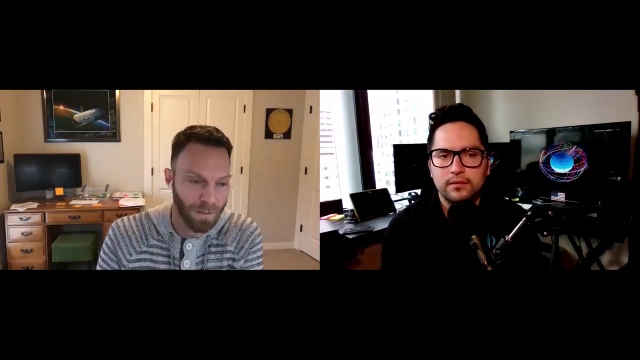 So the first question is, so you had a pretty stable job at Boeing. I know you mentioned that your wife also worked at Boeing. So it wasn't the biggest risk in the world. But you decided to leave your job at Boeing to go ahead and go to planetary resources. So can you talk a bit about that decision process and kind of what made you kind of what attracted you to planetary resources and how you went about that decision? Yeah, sure. So at Boeing, I spent the first 10 years or so working space projects, moved from California up to Seattle and started working commercial aircraft. Which was still an interesting engineering problem, but it didn't hold my attention like space problems do, mostly on the exploration side of things. I liked building machines that were going to go to places that were difficult for humans to go to. So I spent a year and a half or so working 737, 747 primary flight controls and was looking to get back into space. And it just happened to be good timing. So I spent my first year doing those. Right? 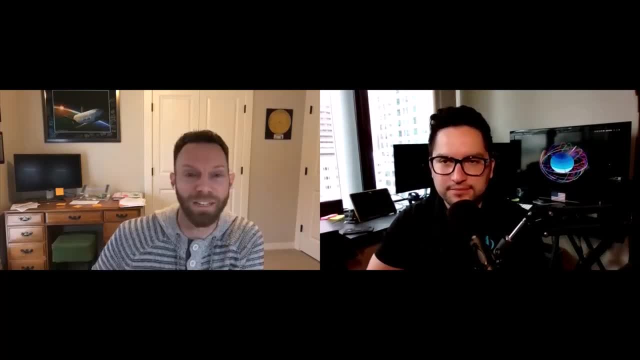 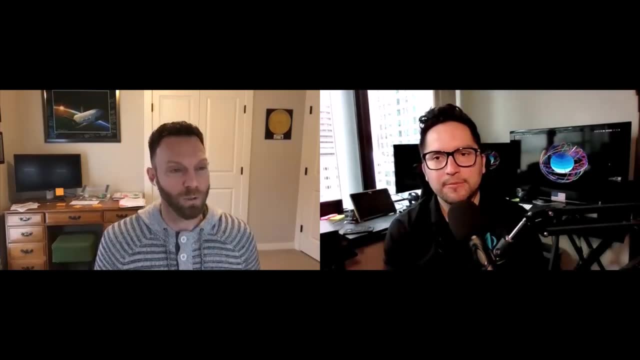 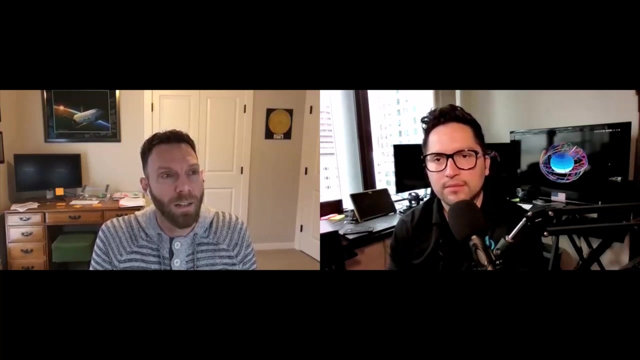 And I also had a role with Planetary Resources, having their Kickstarter and being in the news everywhere and just being essentially down the street from me that I applied. One of the things that you mentioned, not a huge risk. Everything felt like a huge risk at the time, or not really, a huge risk, but you just don't know. Right? You're going into some new scenario and you don't know how it's gonna play out. In hindsight, it wasn't really that big of a risk. I had been sort of coddled. I guess. I guess. I guess. 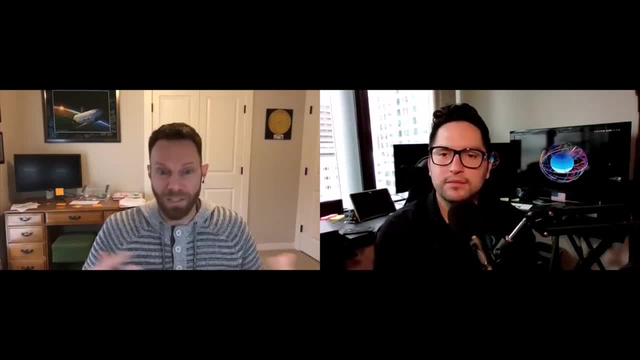 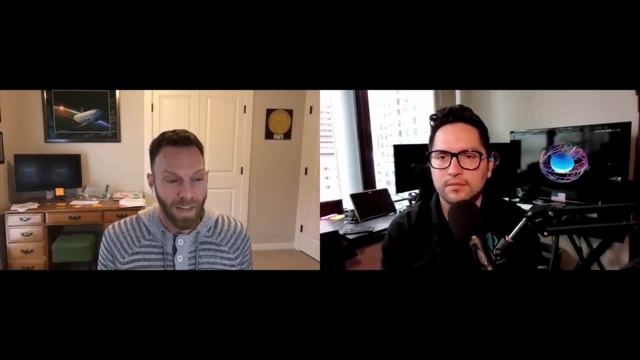 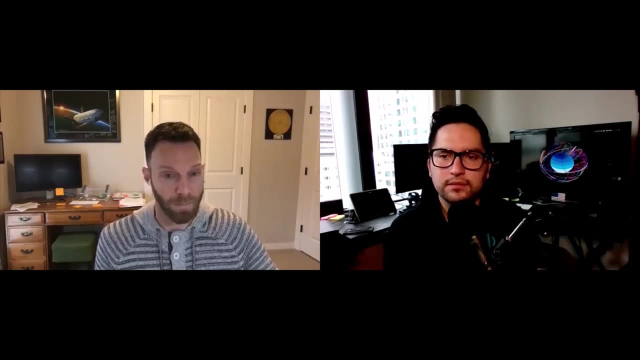 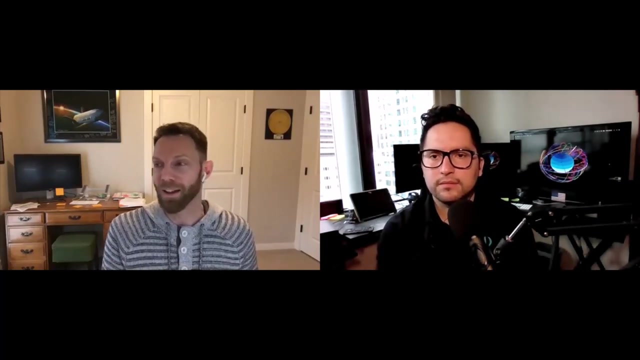 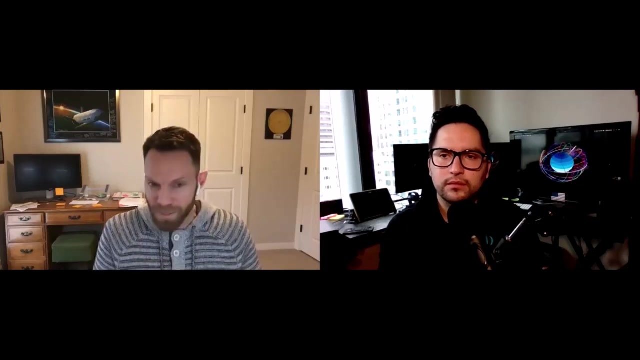 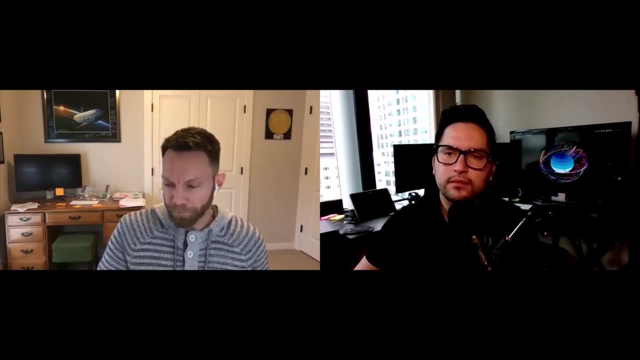 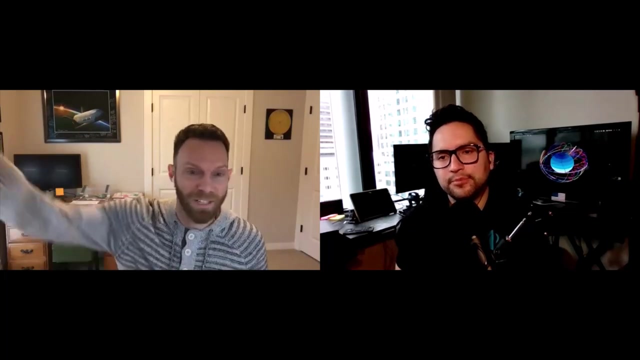 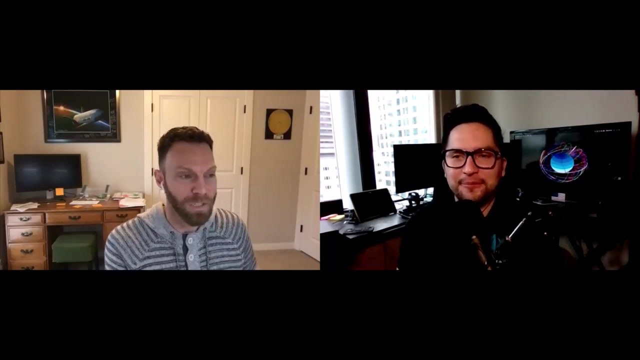 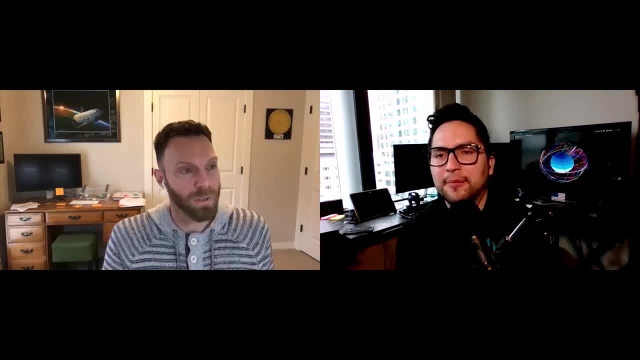 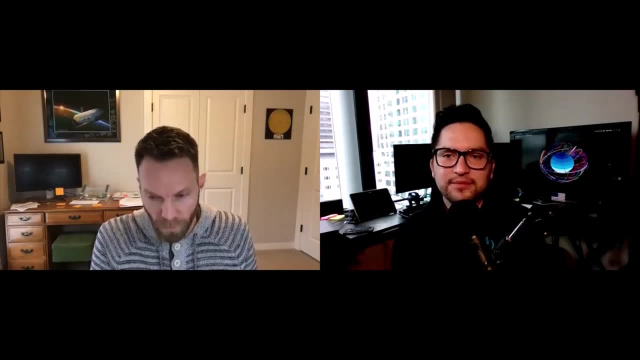 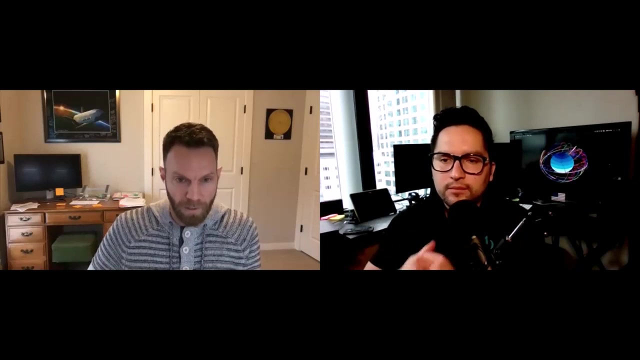 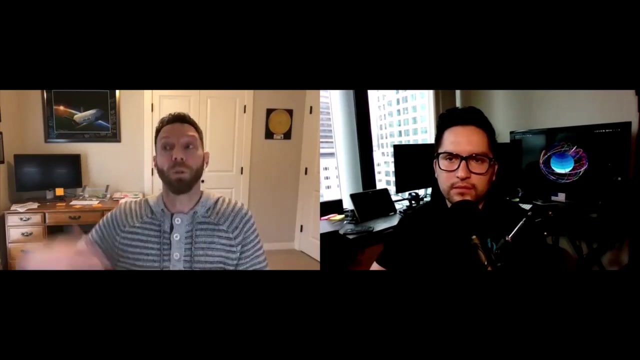 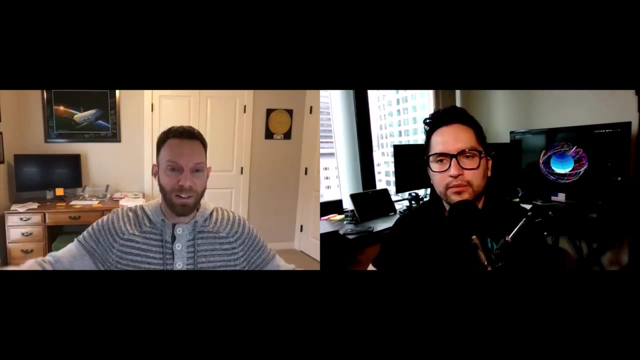 um but so Planetary Resources was a space mining company um but so Planetary Resources was a space mining company I mean that's that was the goal and originally we were building spacecraft uh low earth orbiting spacecraft to sort of test out our hardware test out our methodologies that we wanted to pursue and how we wanted to build spacecraft as a team which was a lot of fun but the the ultimate goal was to then do prospecting which is to to investigate potential mining spots um in deep space at these asteroids and then ultimately build mining equipment you know that's that's the far out goal um so that that whole string of long-term plans was just exciting to me and so it was easy sort of to leave Boeing then at that point and go and do just something kind of wildly crazy. So then when you when you first joined you 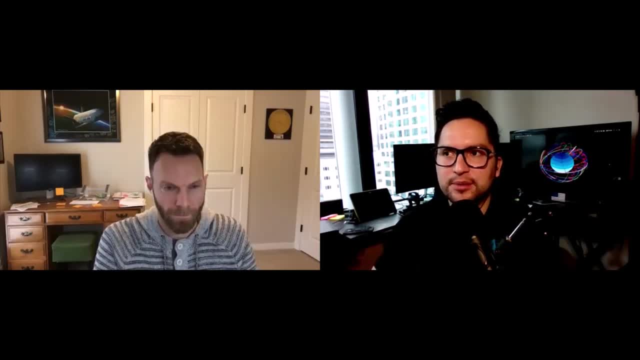 were in the ARCID 3 days so that was the first CubeSat and was that after the was that after the um the high altitude balloon days? Yes I was not I'm I'm post high altitude balloon wait so what what was the what were the mission objectives for the high altitude balloons I don't really remember I don't know I mean I have like some theories and hunches but that was before my time and nobody really seemed to talk about it 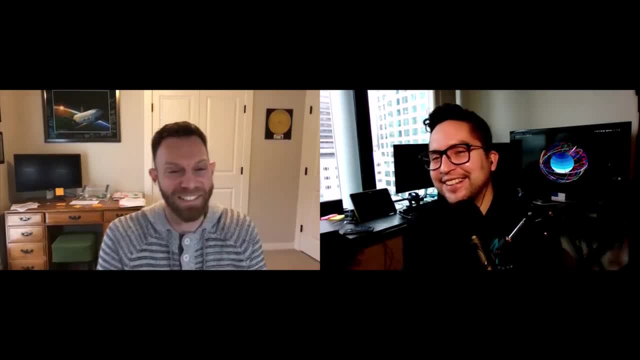 much afterwards so I don't have a good I don't have a good answer for you okay so then so then 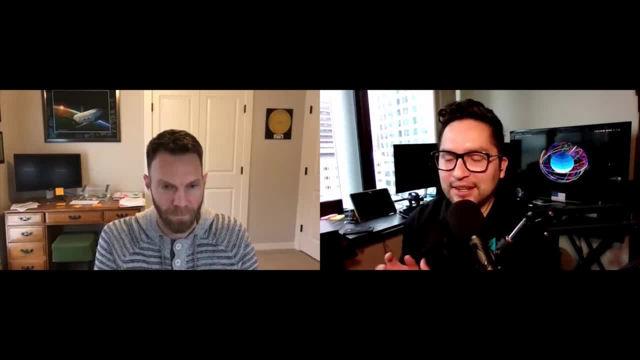 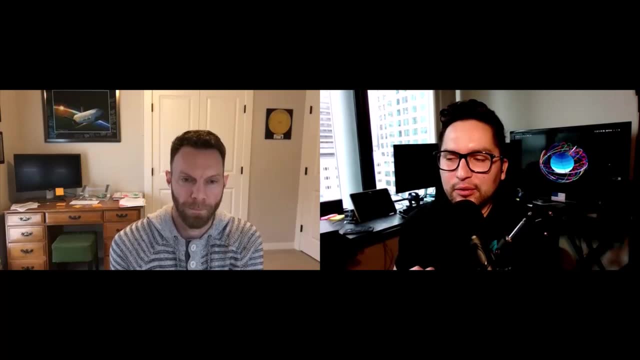 we did come in so ARCID 3 was the first 3U CubeSat um and then you mentioned in the last talk that when you came in it was decided that for the high level objectives and requirements that the spacecraft wasn't going to have any active control um so can you kind of talk about that decision of you know just that whole requirement of not having active control and kind of why that was acceptable for that mission? 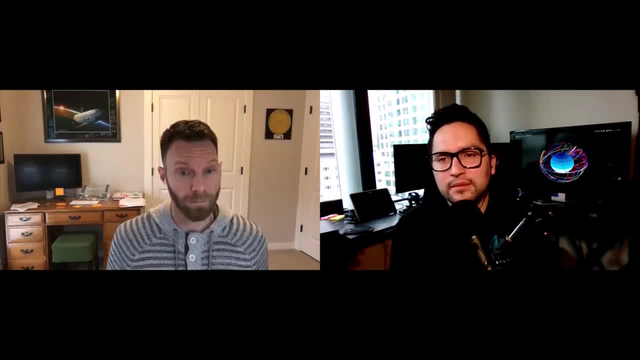 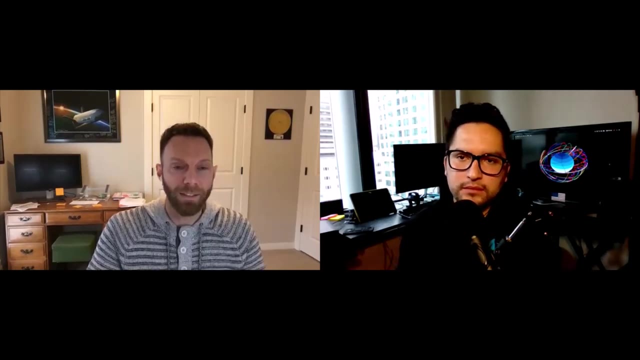 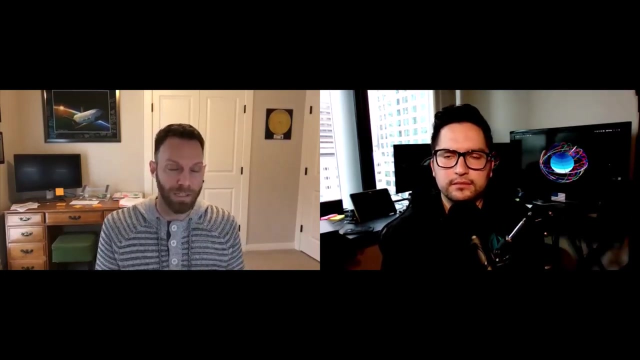 Sure yeah well we didn't start that way okay I mean we started with having active control as part of the A3 or ARCID 3 spacecraft um the the high level goals of that spacecraft was to rally around something that we could build a team you know around we could build um we could we could hire people we could work on an engineering problem we could build up our our clean room our engineering manufacturing processes we could design our own hardware architecture from scratch we could design our own software architecture from scratch with the ultimate goal of of saying that these are the first iterations of these things that we want to take to deep space right we weren't trying to build a CubeSat we were trying to build a platform that would allow us to uh to design and test out some of our deep space architectures that we were trying 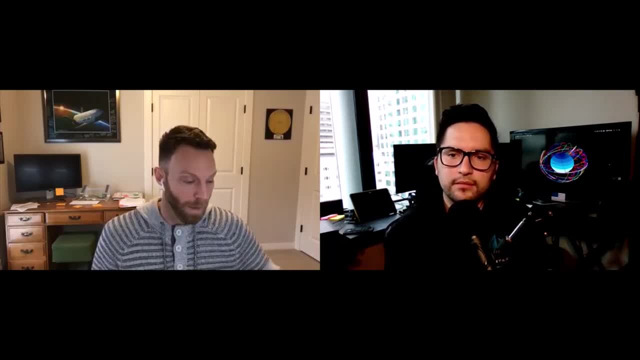 to come up with and so that was the ultimate goal um and and part of that was just figuring out what tools and processes and people we needed to accomplish that and what does our team look like and how do we interact with each other um what is the structure of responsibility look like because we you know we're building up this team from scratch we didn't have a lot of that or at least we wanted to trade a few different options and practice and things by building real hardware so that we would be in a better position to then take the next step so that was the main goal of A3 um and and part of the way 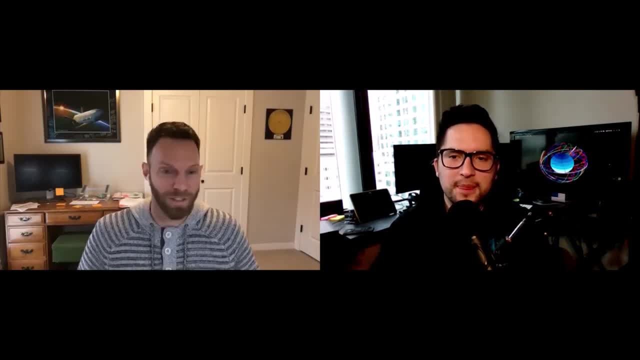 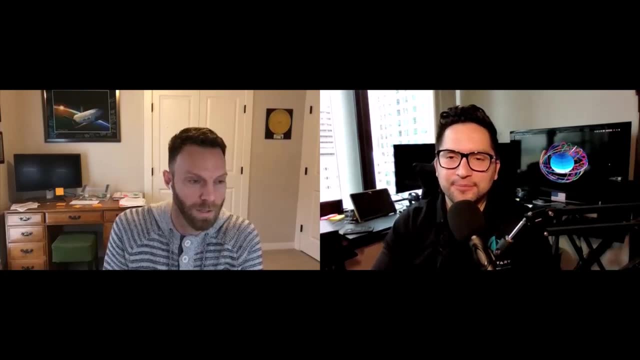 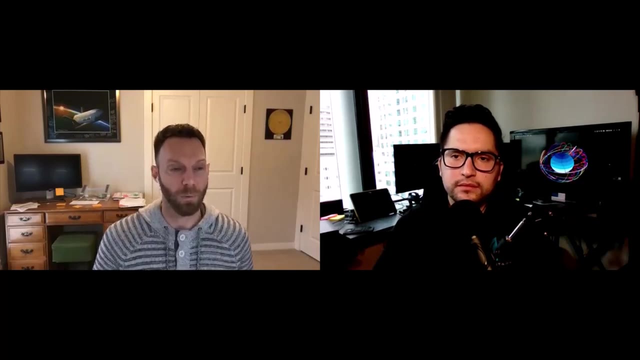 through that process you know we're a ride share and the launch is going to happen with or without you you don't really have a whole lot of say in that and it got to the point where the launch was coming up and we weren't as far along uh with this full you know full up design from scratch that that we wanted and we there were some concessions that had to be made and so the ADCS the attitude determination and control system uh that's responsible for determining attitude and pointing the spacecraft ended up getting 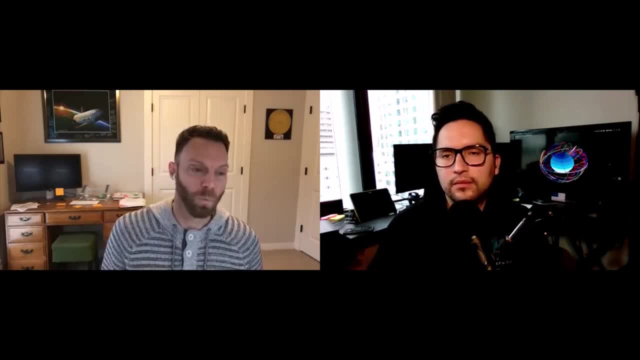 scoped from from the project um which was kind of a bit of a running joke then from that point on 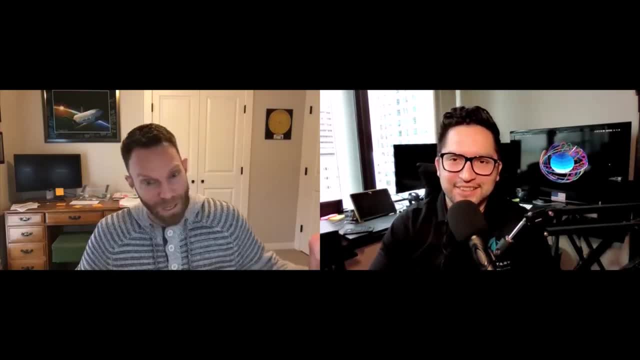 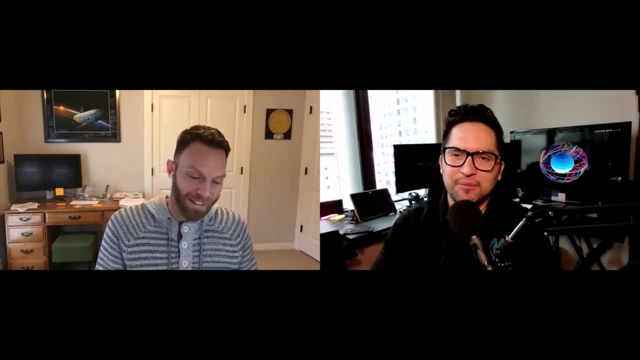 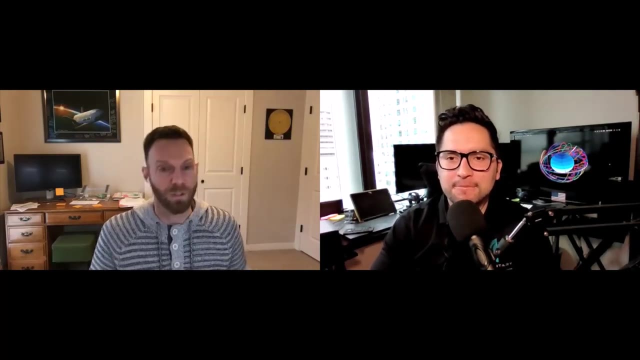 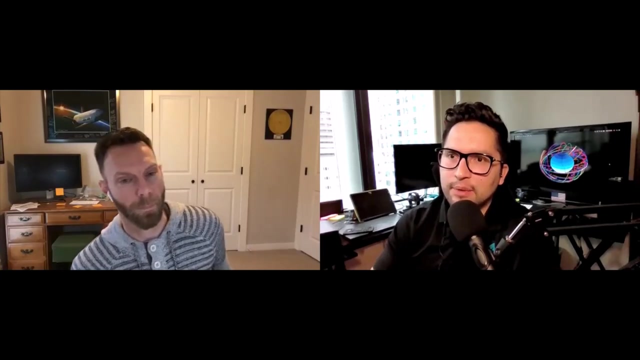 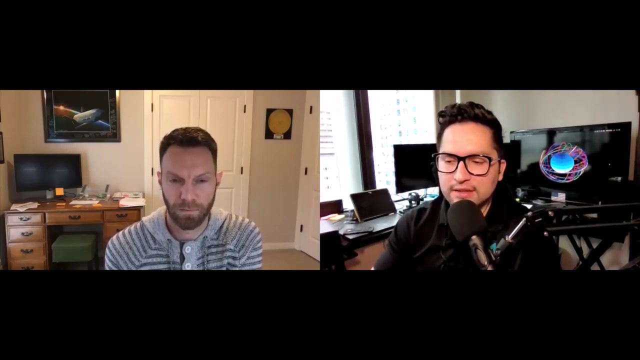 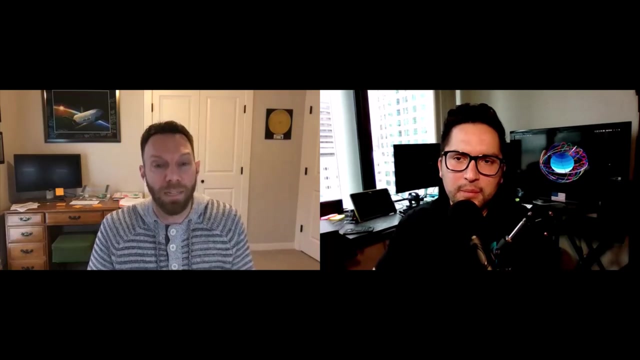 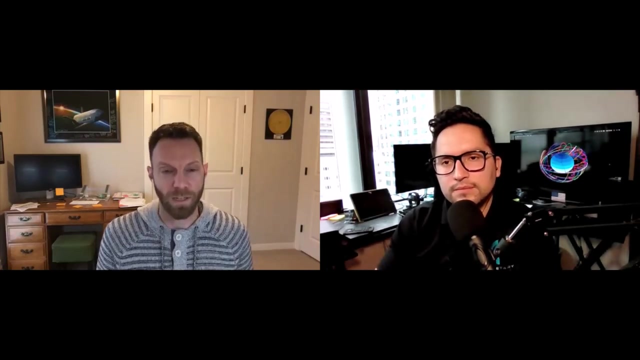 because the ADCS team then all of a sudden had a lot less pressure and uh and then it was like oh it must be nice to be the d scoped people uh but but uh you know we were still proceeding in the background you know building up our architecture and our algorithms and testing and our simulations and all of that stuff so that we could be ready for the next for the next launch but the idea was that a3 didn't need to function as a spacecraft fully it needed to be able to charge collect power store that energy it needed to be able to communicate with the ground it needed to be able to have all of its hardware architecture communicate with each other and we need to get data down from that and it turned out we could do a lot of that stuff with with a tumbling uh spacecraft for the most part so so that did end up working that you can kind of rely on is there being launched into space with some random tumble that you're able to do the things like communications and um you know if there was any scientific objectives like being able to image the earth or something so that was possible with that random tumble well the first part of what you said for sure I mean you can set up a spacecraft to to tumble I mean they're spinning spacecraft out there that that are stabilized because they're spinning and they're able you know their antenna patterns are set up in such a way that they can 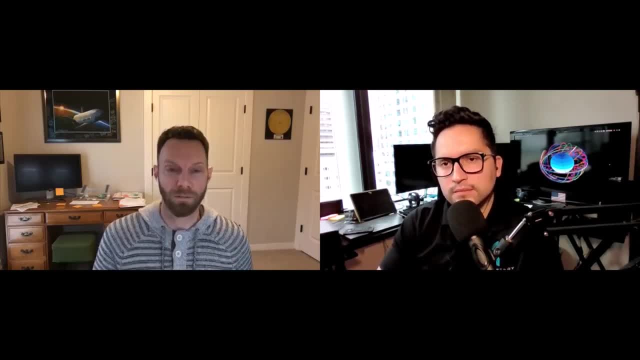 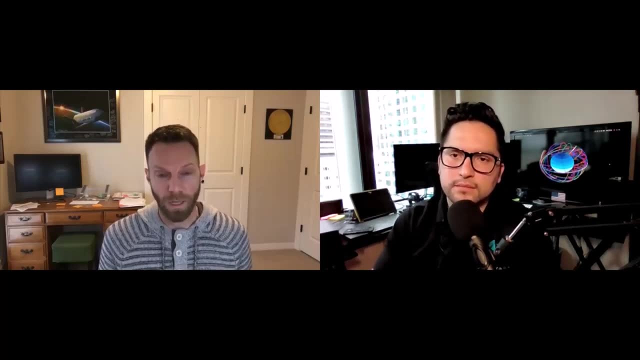 communicate with the ground and they can charge their solar panels are set up or you know maybe they're battery powered but um but yeah you can absolutely set up a spacecraft to to handle tumbling imaging the earth is a little bit trickier um I mean if you don't care what you're 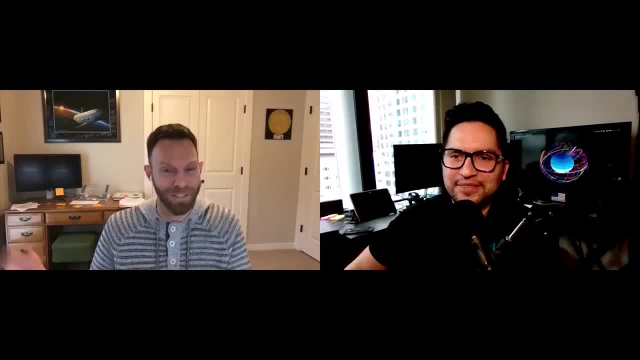 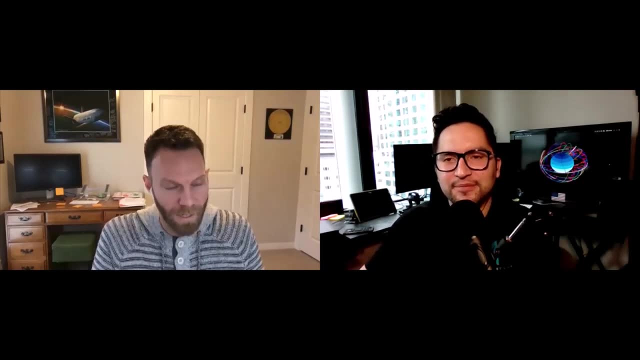 imaging and and you don't care if there's like smear in your image because you're rotating around sure you can you can you know take a picture um but that's not what a3 was doing um and a3 didn't 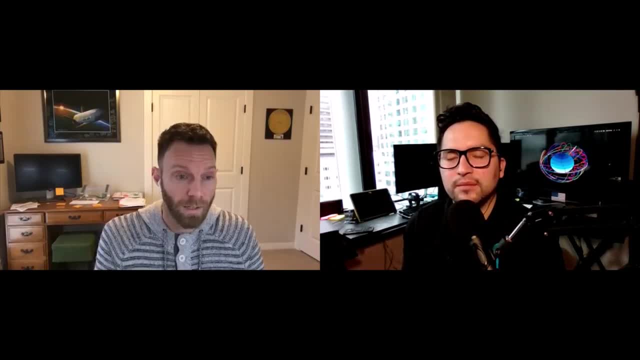 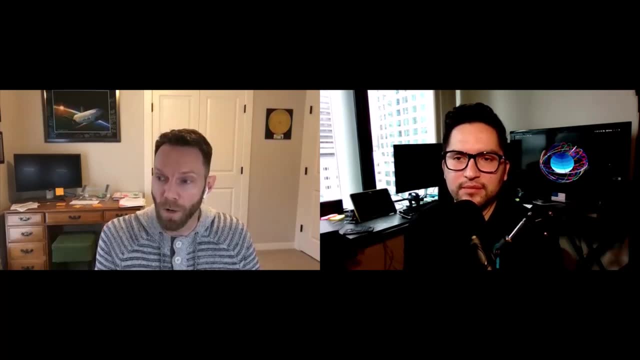 have science objectives at all I mean the objective was build a spacecraft as a team and and launch it um no matter what the outcome was you know the majority of our objectives were met when it launched because that was the whole purpose of it okay yeah so can we get into that how basically 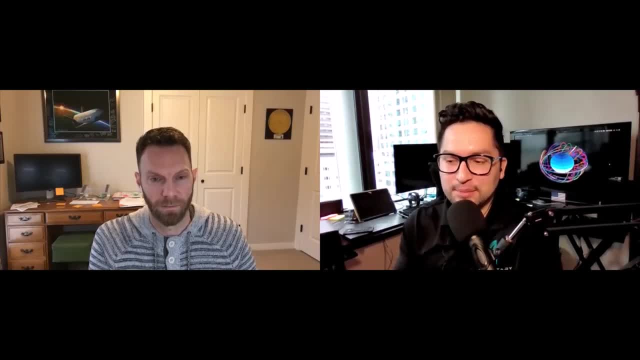 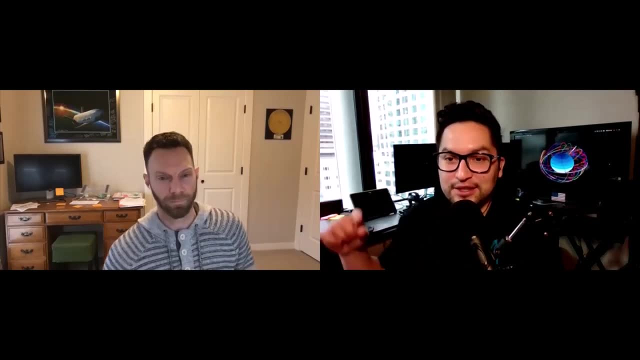 as you said the majority of the objectives were already met just by go ahead and building the um go into that experience of what it was like to watch it on the first launch the first a3 when it 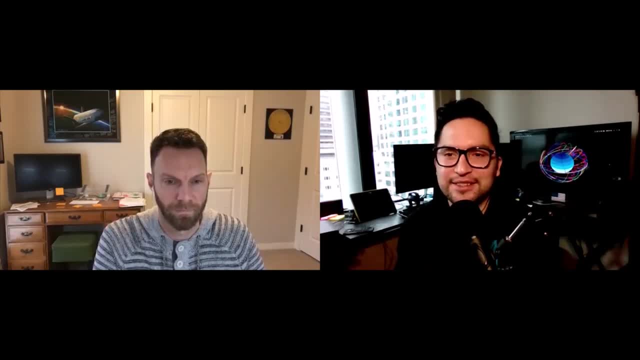 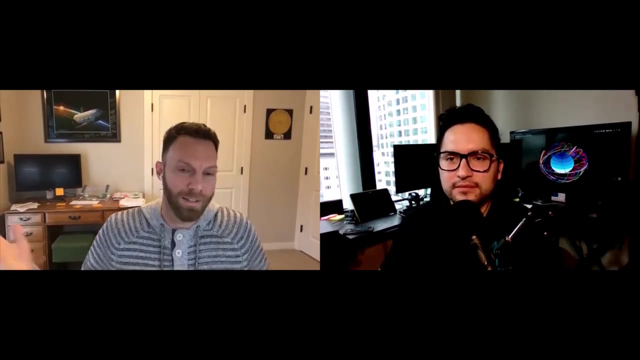 blew up and then the the the mindset of the team after that all happened and also during the time because that must have been a pretty crazy kind of experience yeah so our our first arctic three spacecraft uh blew up after I don't know 20 feet or so off the launch pad um which was surreal um that's the first time that's ever happened to me that's the first project I suppose that that I was part of launch that wasn't some giant National 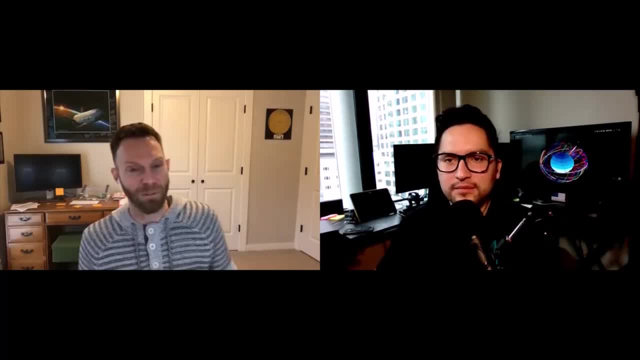 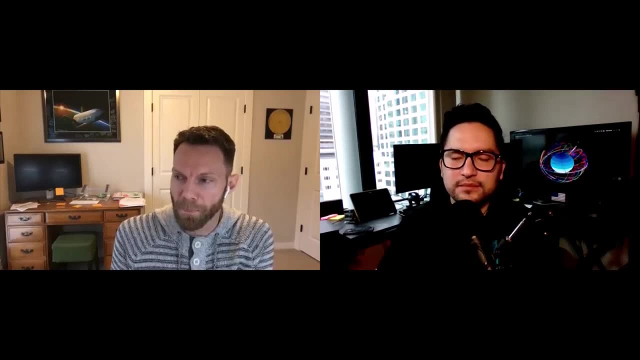 asset you know like that if it exploded it would be you know devastating um it was yeah it was definitely surreal um to watch that and and obviously disappointing uh the the thing with 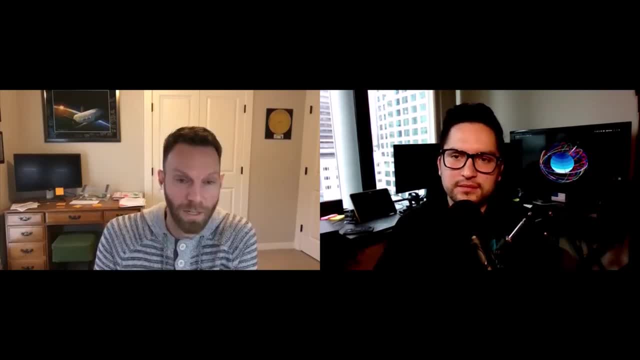 arca3 though it was going up as luggage to the International Space Station it was going to get fired off of the ISS sometime later 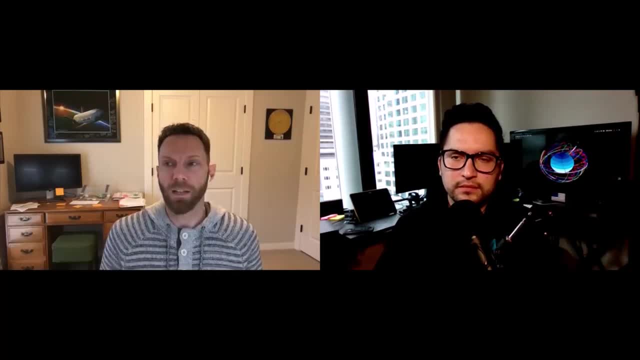 um it's not like we were all in our command center ground center you know ready to communicate with our satellite and turn it on and start doing operations because we were still months away 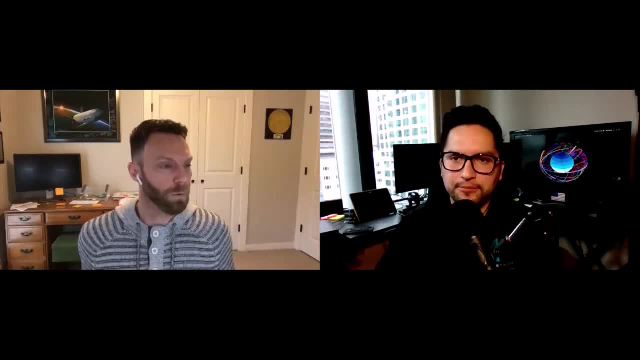 from that because it was just packed away so if I I feel like it was a little bit less heartbreaking because of that because we were there essentially having a party because our our spacecraft went together it launched 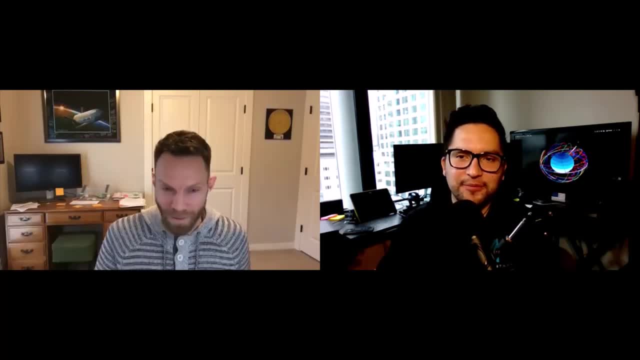 and you know we've got a few more months still before we really have to buckle down and start operating this thing um once it blew up though it was kind of a strange pivot for the company I don't 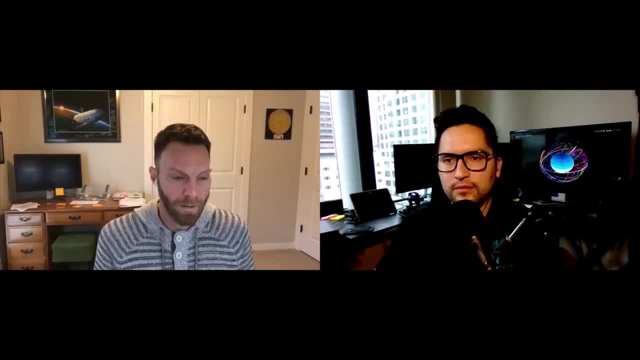 say pivot more of a split because we had enough spare parts we were already building up sort of a flight spare for arca3 and so um we were able to go off and and do that and get that ready for a second launch but 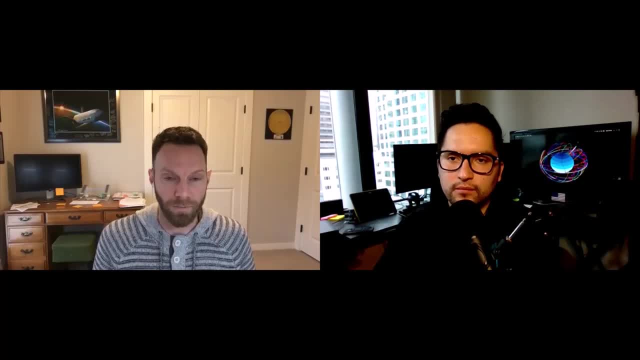 again arca3 wasn't the end goal of of Planetary Resources and since we had already met the 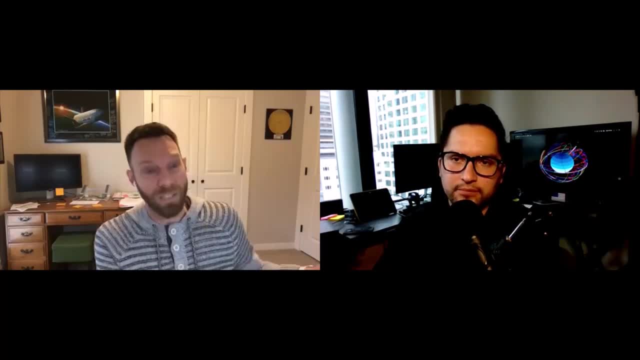 majority of our objectives already the most of the team had to go off and start working arca6 the six U spacecraft the next iteration the one with more sensors and more actuators and more hardware and more technology built into that so it was really only um a handful of Engineers I wasn't actually even on the team 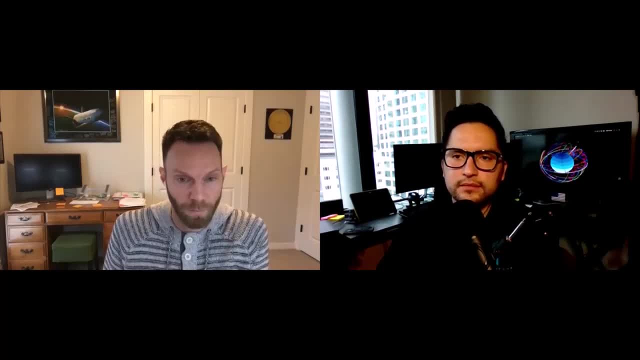 um building the second a3 I think it was just Hannah Goldberg um and and one or two others that were charged with put the flight spare together get it ready to to launch and go and the rest of the team is going off and working on the next project um already so it it was I I don't know I guess it was a surreal experience but at the same time we had so much work to do that it was like okay on to the next thing now 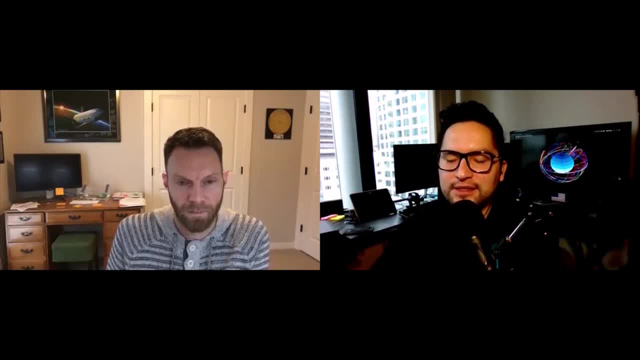 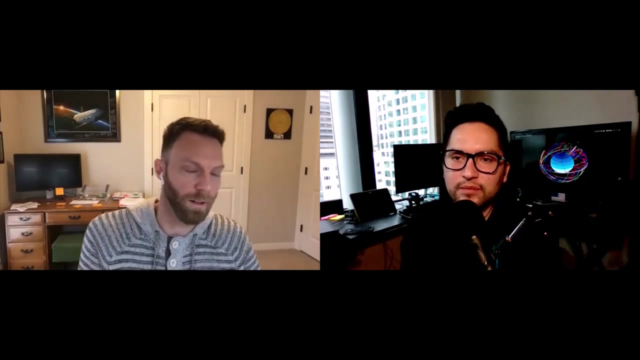 what was I guess so what were the lessons learned from the a3 after after the next time it launched and that you took into a6 specifically to the ADCS side so we can start getting into there well um again there wasn't much ADCS on a3 ours was sort of a continuous evolution of our system we took that opportunity 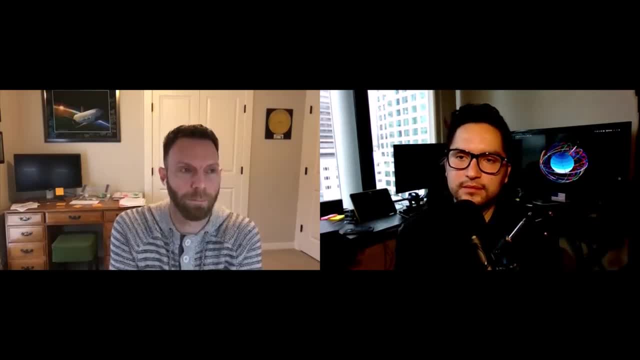 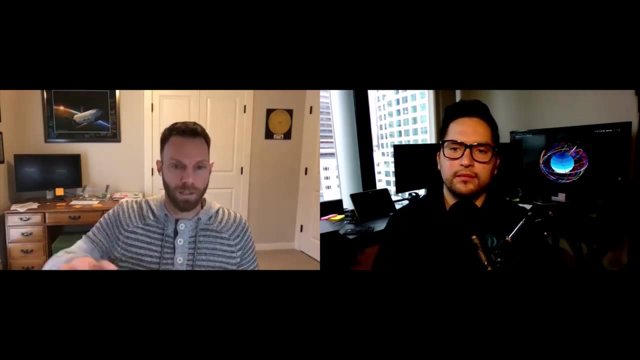 time that we had to really plan out our development um schedule and what supporting equipment and supporting software did we need to generate in order to ensure that the system was going to be 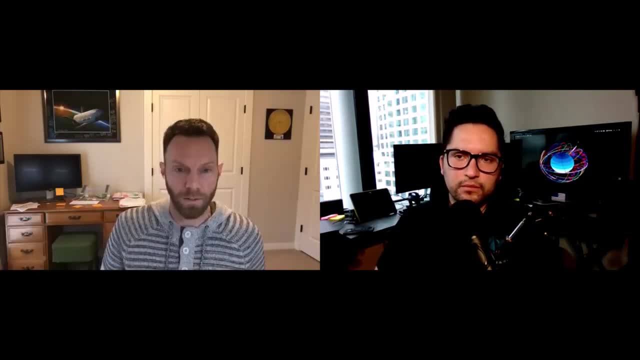 verified and validated throughout its life cycle so then it was ready to go for a6 um and and so we spent that time 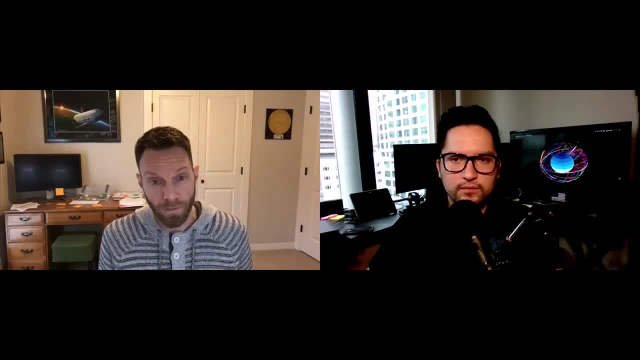 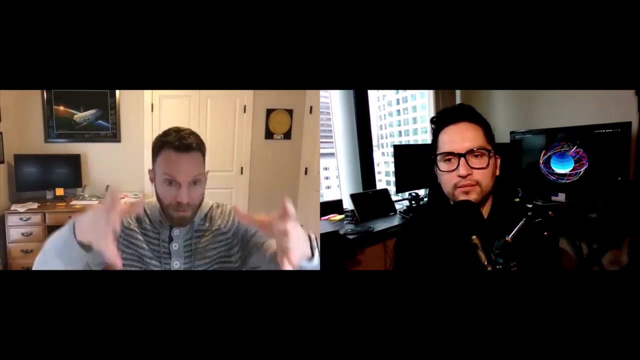 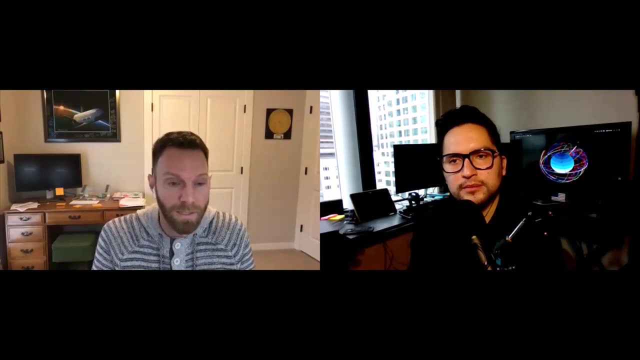 um building up a a higher Fidelity simulation and uh getting like spherical air bearing tables which is uh it's kind of like a a really sad air hockey table because it's just a it's just a post with a concave uh you know uh a groove in it that Air comes out of and then a semi sphere sits on top of it and allows this basically frictionless connection um in in three axes or so, um, that we can place our spacecraft on top of and test at least some of, some of the degrees of freedom in a frictionless environment. Um, so we didn't, I, I don't want to say we didn't have any lessons learned from A3 because, you know, you're always learning stuff, but we didn't have those sort of big takeaways that we said, next time we're going to do this completely differently because we didn't have an opportunity to test anything out on A3. Um, we, I mean, there were some takeaways from the larger spacecraft, which was that, uh, power generation and communication while possible to be done while, while it's possible that you can do that with a tumbling spacecraft, it is not guaranteed. There are some, there are some, pathological cases in the, you know, the spin axis of the spacecraft where you can get into 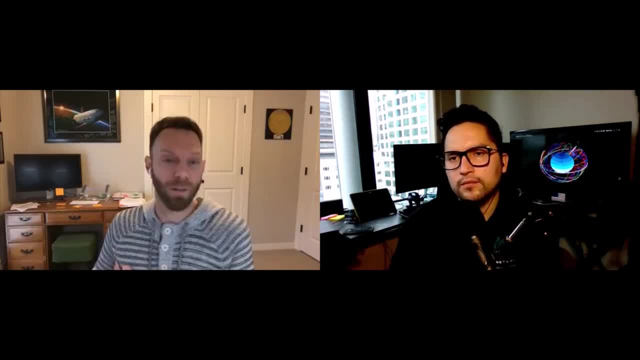 these situations where you're not charging at all for long periods of time. And, and you can't get out of that, or you can't communicate for long periods of time and you can't get out of that. 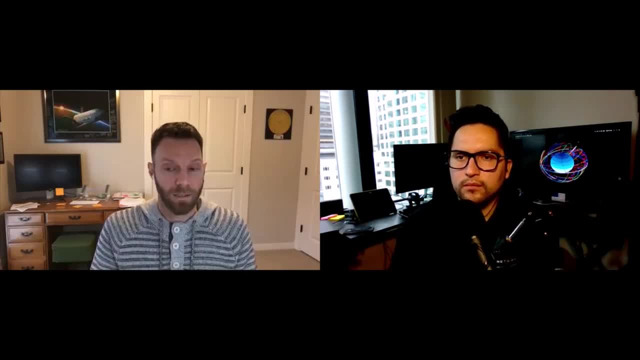 And so, um, we knew that we needed some form of rudimentary control, even if the main spacecraft computer never turned on or didn't work whatsoever, that, um, that we wanted to be able to control the attitude of this spacecraft, even with just some of the smallest, you know, edge compute elements that, that exist, these, these distributed compute elements that exist throughout the spacecraft. So can we go deeper into that, to the distributed, um, compute elements? So, 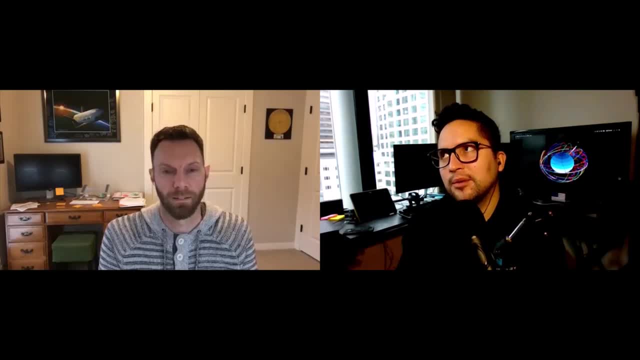 sure. So in general, I would imagine that when you design a control system, that you're going to have the main computer actually doing all the calculations and then sending the commands to say your reaction wheels. But you say that you guys built kind of a fail-safe system sort 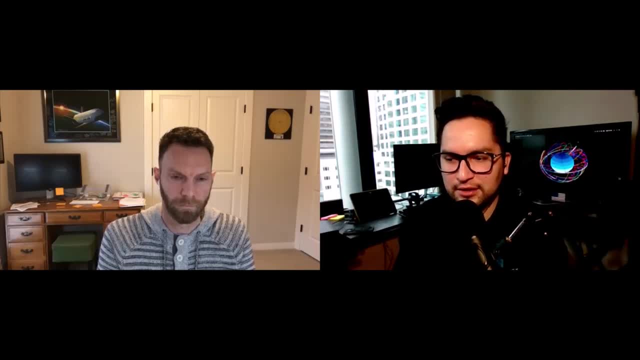 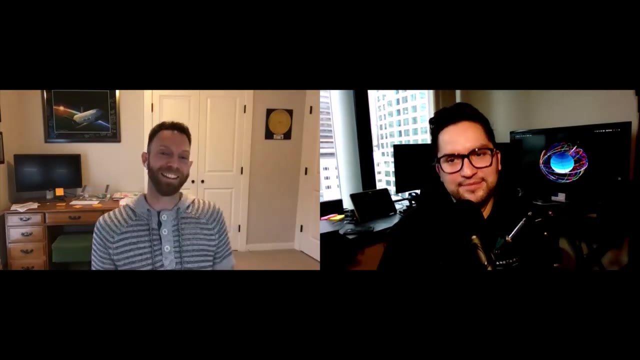 of, um, where if the main spacecraft computer went down, just these other compute elements could also just do some sort of rudimentary. So maybe just point at earth and point at sun. So how did that, how did all that work out? Well, well, I mean, it worked out great in, in, in the end, it was really difficult to get all of these compute elements. 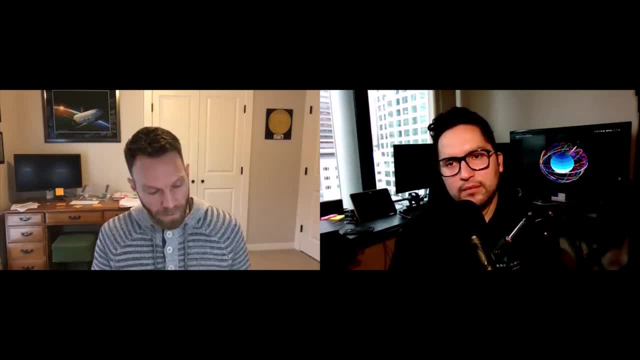 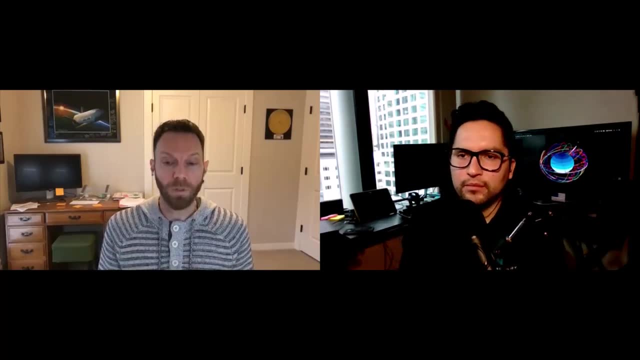 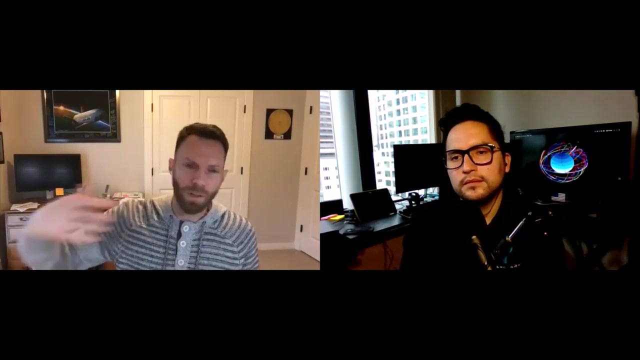 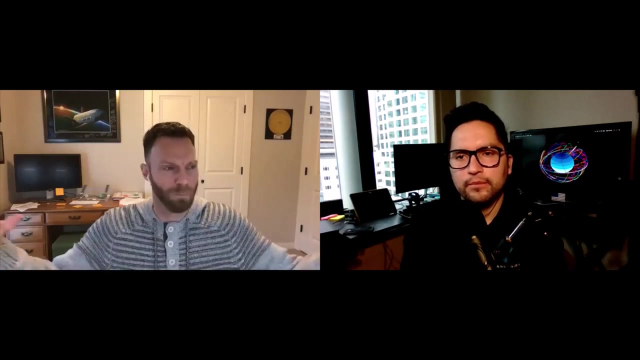 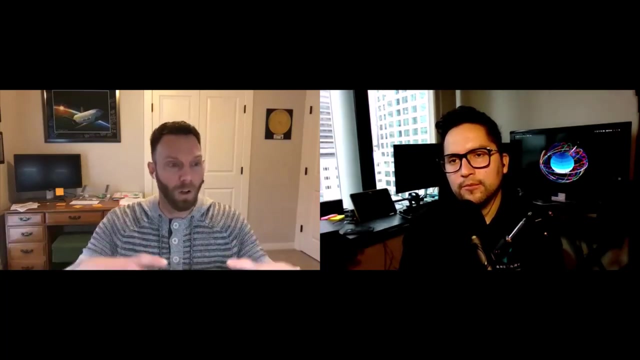 Working together in the way that we've architected it, but that's a different story. From a controls perspective, um, when the main spacecraft computer was operating, it was doing the bulk of the ADCS calculations. It was doing the path planning. It was doing the state estimations. It was doing, um, the, the actual controller itself. It was doing all of the mode logic and everything, you know, it's, it's, it's what you would kind of expect, which is, uh, go out there and do all the calculations, do all the calculations, do all the calculations, go out there, collect all of the sensor information, give me the sun sensors, give me the star trackers, give me the accelerometers and the magnetometers. Let me get all of that information. I'm going to filter it, um, uh, rotate it all into, you know, the control coordinate system. 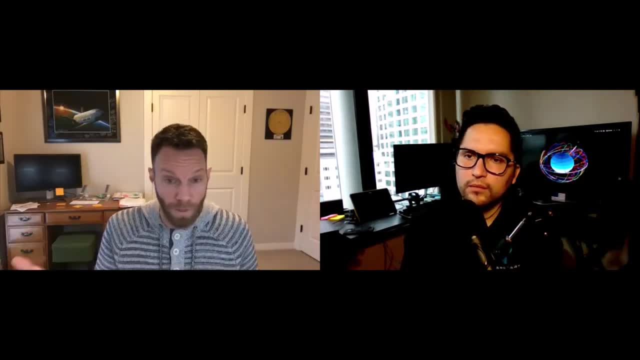 I'm going to throw out any data that I don't trust for whatever reason. I'm going to estimate the 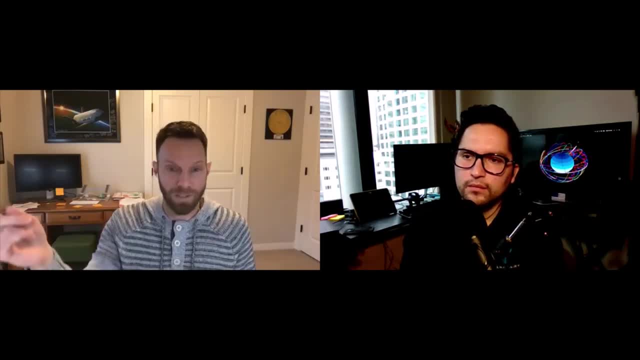 state of the vehicle. I'm going to determine where I want to be compared to that data. 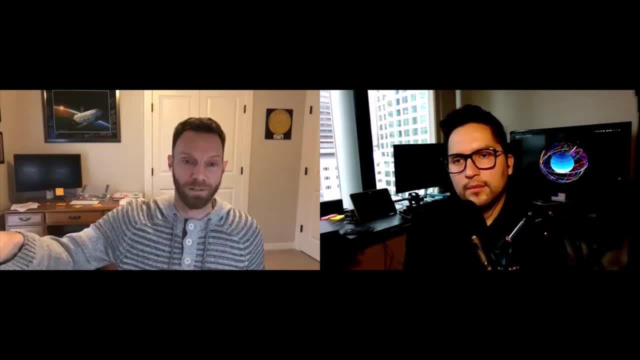 And then I'm going to drive the actuators to, to close that error. Um, and then the actuators are 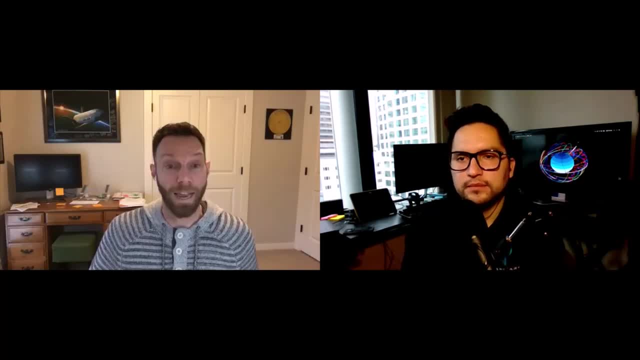 torque rods in our case or, uh, reaction wheels. So that's all what you would expect. The difference 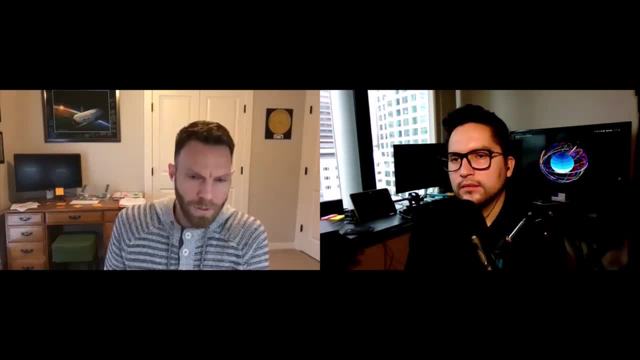 is that our, what we call device managers, the, the software element that would manage the actuators and manage the sensors, they did all of that on their own distributed, like, 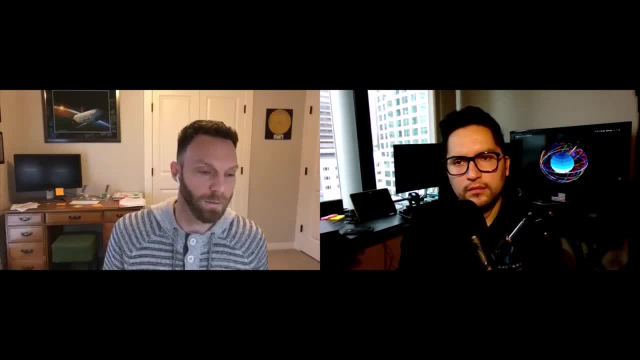 compute element. And, and these compute elements are, are really weak. I mean, they're the, they're the types of, of, of microprocessor that you might have in your watch, for example. I mean, just real, 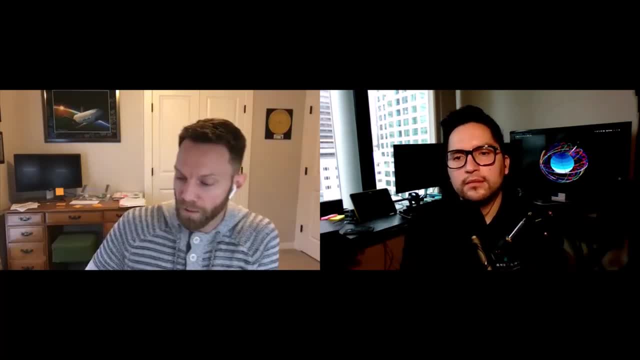 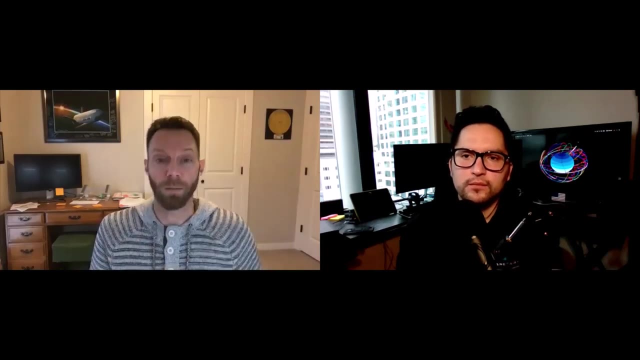 real tiny things. And all their job was, was to, uh, generate telemetry from these nodes, like the reaction wheels, run the reaction wheel motor controller. So the main spacecraft computer would say reaction wheel spin up to a thousand RPM. And then the smaller compute element would take that, 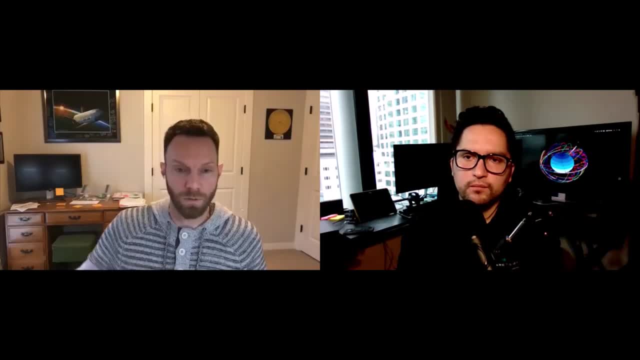 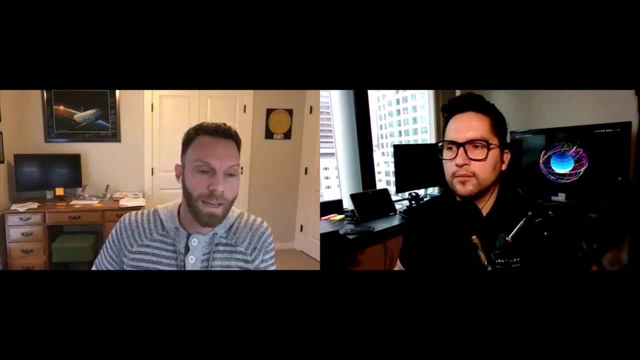 and adjust the, the, the current and voltages to, to the, um, the wheel to control it to a thousand RPM. So the motor controller was down there. And, um, you, you, you know, so it, so it distributed 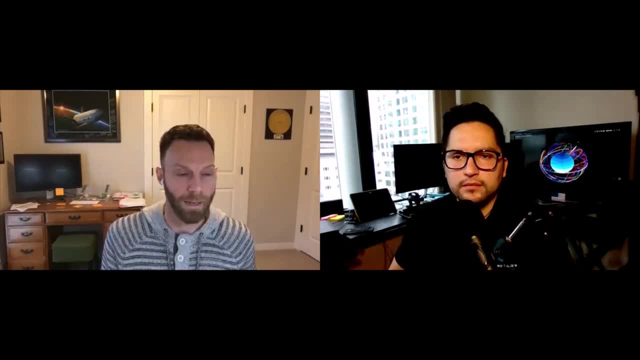 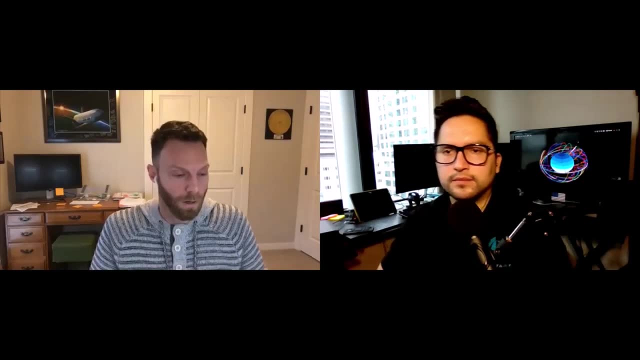 some of the low level, some of the low level commanding and, um, messaging and things like that to these, to these distributed elements. Um, and that was, that was our architecture. 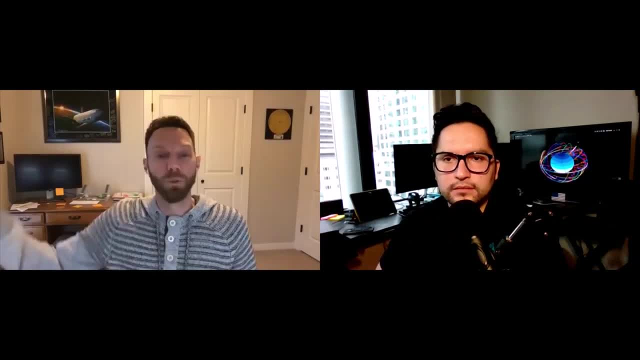 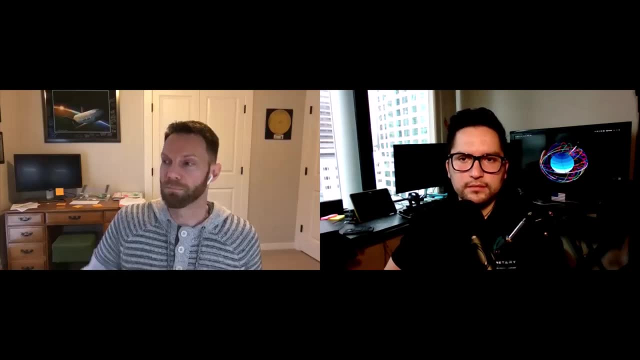 The nice thing about that was that it was modular, so we can remove, uh, reaction, wheel and we didn't have to change the flight software very much because the flight software would understand that there wasn't a node there and therefore it's not in the design 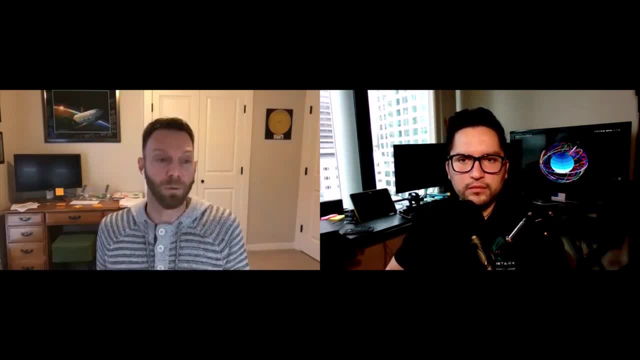 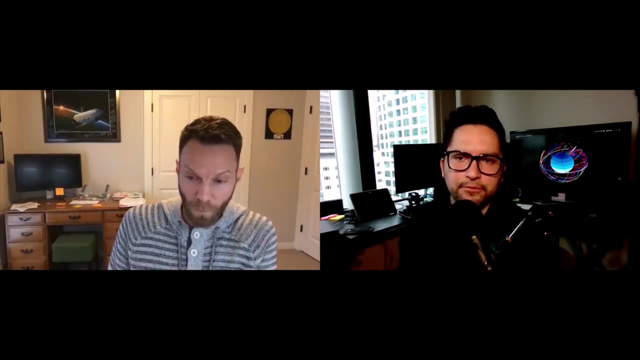 what we what that ended up allowing us to do is if the main spacecraft computer died we were thinking well we still have a computer that can talk to the reaction wheels and control its rpm we still have a computer that can read the sun sensors we still have a computer that can read the imu and and all of these things we just don't have the big brain to process all of that information all that data and and come up with the calculations for the actuators so we added another low power small computer whose sole job was to communicate with all of these other 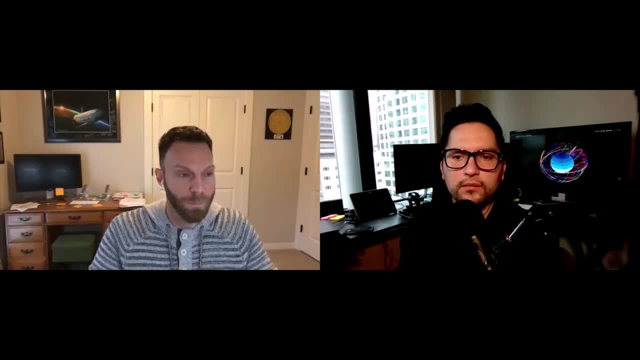 distributed nodes and and do the most basic control which was figure out where the brightest object was was that it can see like look at all of the photodiodes and the sun sensors and say where do 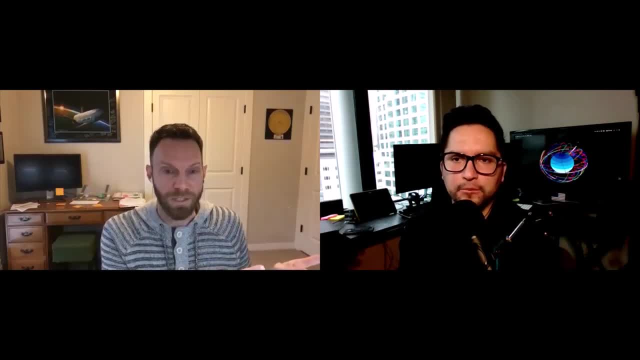 i think the sun is and then move the reaction wheels in such a way that points the solar panels towards the sun like it doesn't know where it is in orbit it doesn't know hardly anything um it's 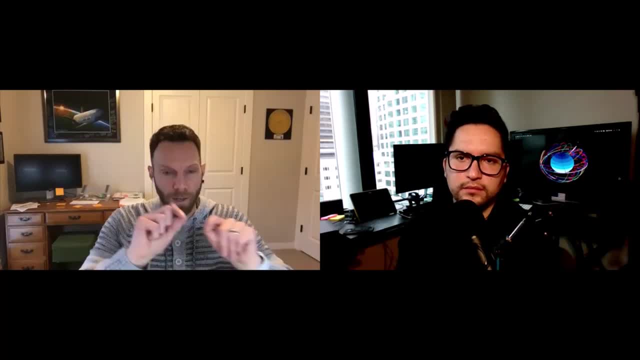 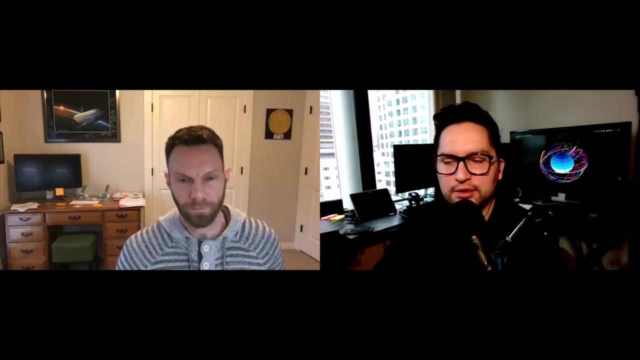 just a bare bones controller that can operate on a bunch of these little low power compute elements distributed throughout the vehicle so off of so going off of that i want to learn a little bit about the the actuators that you use as far as in the trade so was it as far as a 3u cubesat was it a bit obvious or how much trade was there going into choosing i want to use reaction wheels and in order to desaturate i want to use torque rods magnetic torque rods yeah well i mean i 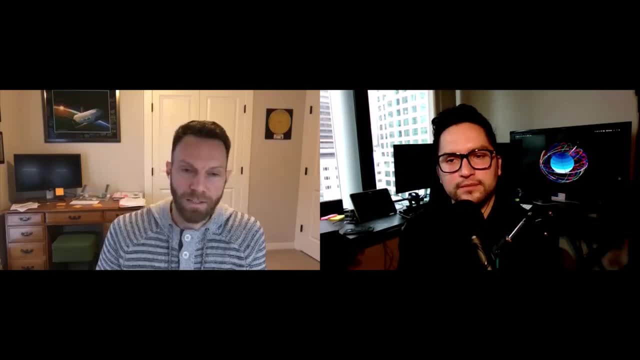 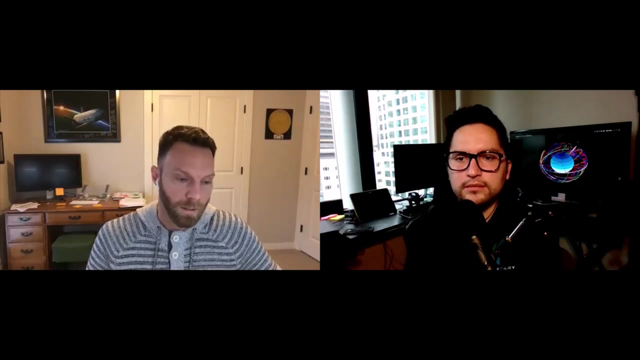 At some level, every decision you make is a trade and sometimes it's a no brainer and you do that trade really quickly in your head. You're like, do I want thrusters? No, you know, and then you move on. Uh, so, so for, for some of that, that's what we ended up doing, right? We didn't do a lot of formal trades at the beginning to determine reaction wheels. We knew that we didn't want thrusters because thrusters on CubeSats and adhering to the CubeSat spec with them and everything was, it's just more complicated than we wanted. And we were going to be developing our propulsion system for later, larger spacecraft. So we didn't want to mess with that. Um, so reaction 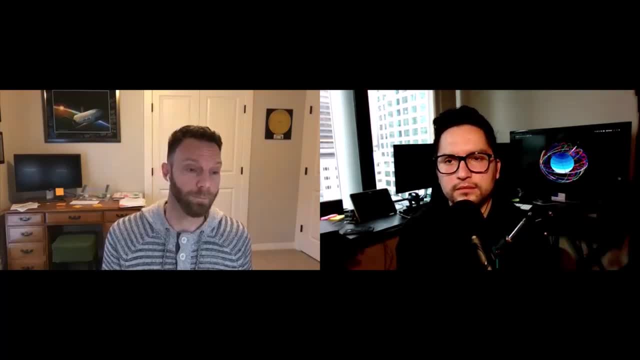 wheels were the natural choice for, for, um, managing our momentum. You know, there's CMGs, 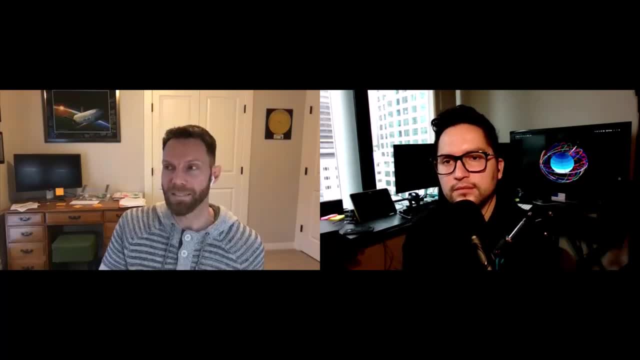 the control momentum gyros. Uh, but typically those are for these high torque applications. Um, they're a lot more complicated mechanics. 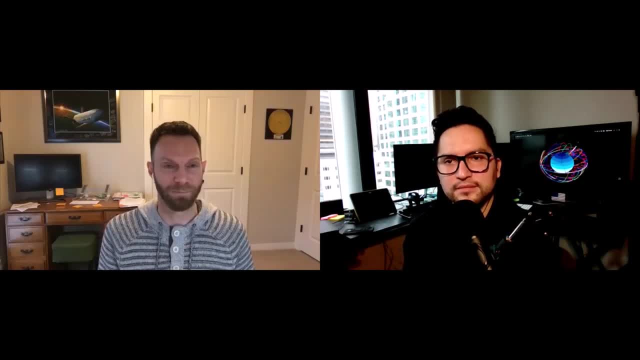 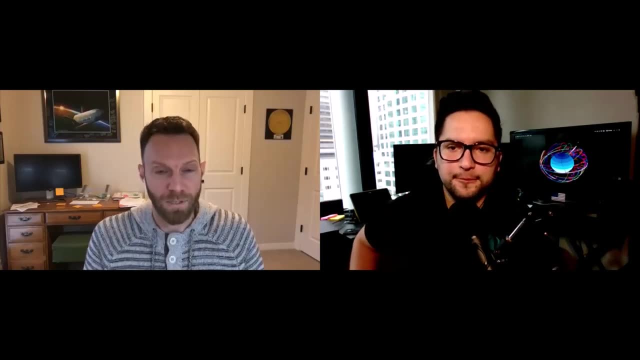 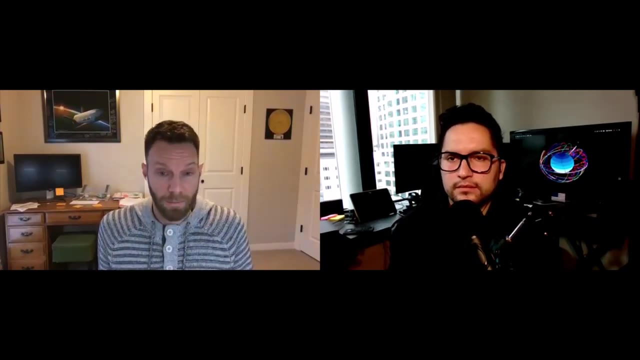 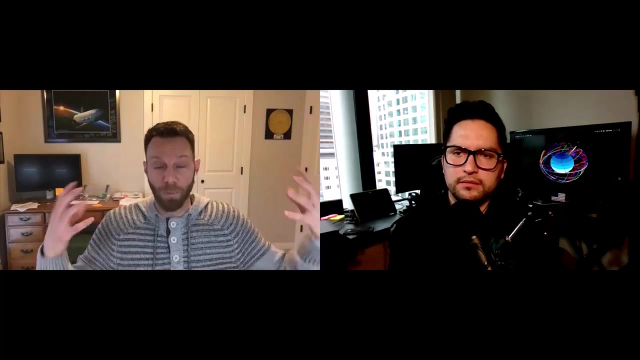 Mechanically and electrically. And it's just not something I'm not actually sure if anybody's built them with CubeSats that maybe they have, but I'm not aware of any CMGs on CubeSats. So reaction wheels were the obvious choice. And, um, uh, the trade came in. What do those reaction wheels look like? Right. Do you want three wheels? Do you want four wheels? Do you want five? How, how much momentum do they need to store? How much torque do they need? 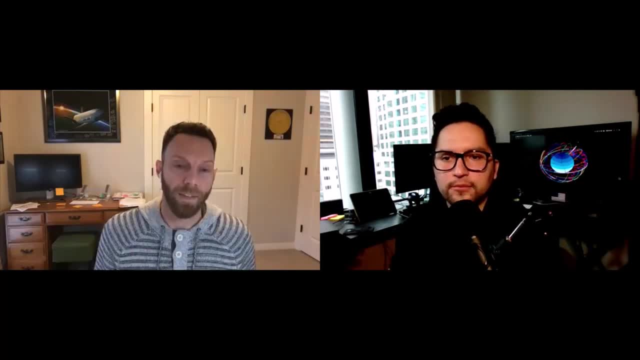 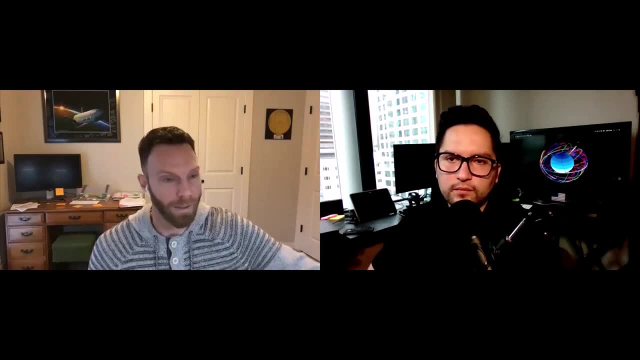 Um, what does the physical volume that they have to fit within? And that's where our trades really took off is once we've decided on reaction wheels, um, we, we started going down the path of what orientation do all of these wheels need to be in? How much momentum do they need to store? How agile does this spacecraft need to be? And so on. Now reaction wheels are a, a momentum, like they transfer momentum between the wheel. 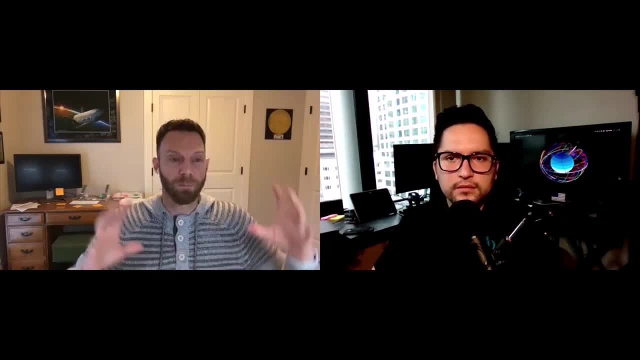 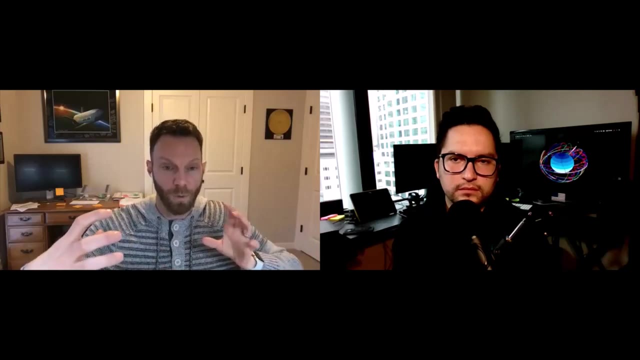 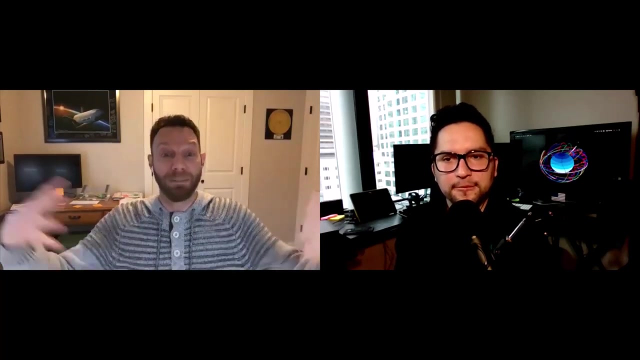 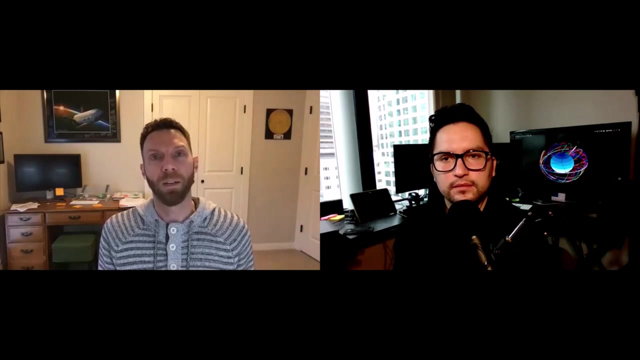 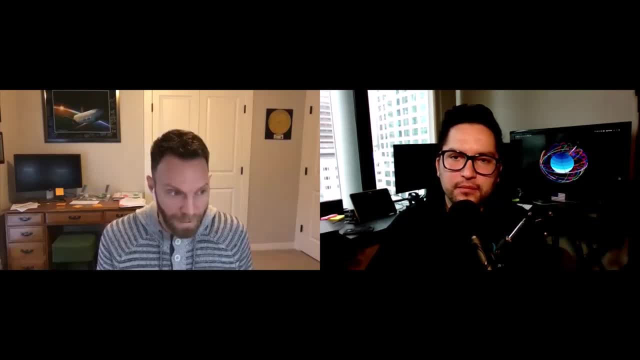 And since we knew we weren't going to have thrusters, we needed torque, magnetic torquing capabilities. And torque rods are a much more efficient way of generating a magnetic field than a torque coil. Um, they, they tend to take up more space and they're heavier. Uh, but if you care about power over mass and volume, um, they're, they're basically the way to go. So that was sort of our, our decision making process for why we 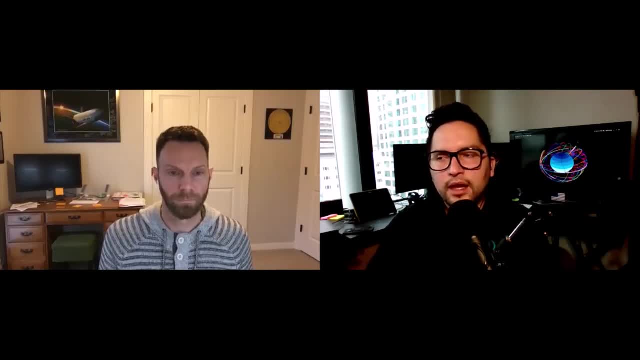 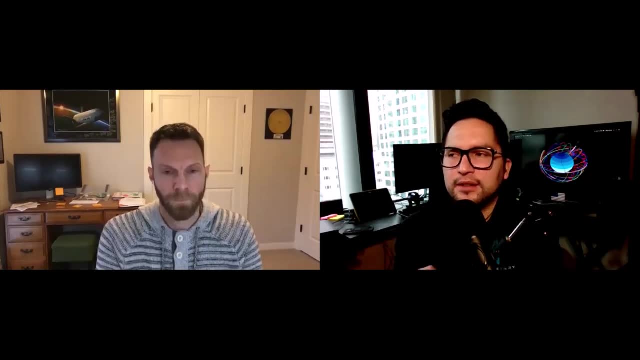 ended up with torque rods and why we ended up with reaction wheels. And then, so going from the attitude control to add to determination. So what were the decisions there? Because from what I remember, star trackers are like really accurate and seem to be a pretty good solution to do attitude determination along with other things. Like I believe if I remember correctly, I think there were magnetometers on A6. So what were the, what was that decision process as well of doing the trades of how are we going to do attitude determination? 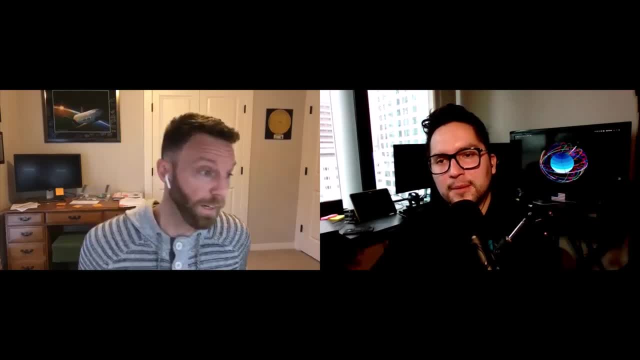 Yeah, well, I mean, usually it starts with some requirement. How well do I need to point? Um, and then you, you decompose that into, you know, into subsystems, all of that stuff. And you come up with the font with some value that you said, I need to know my attitude to this degree, what sensors are available that allow me to do that. 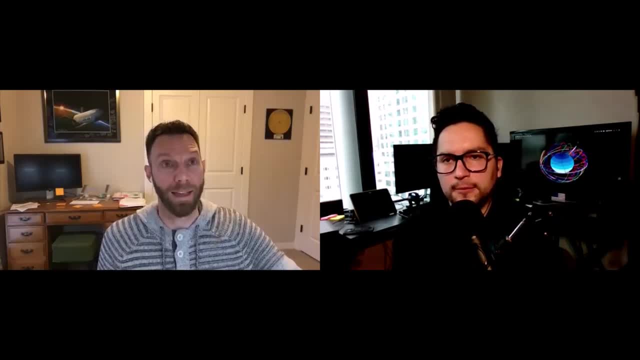 And not only do I need to know my attitude, but I have to be able to determine my attitude when I'm in eclipse and, you know, any, any number of things. And so that's usually where you end up with your sense. Speaker 3 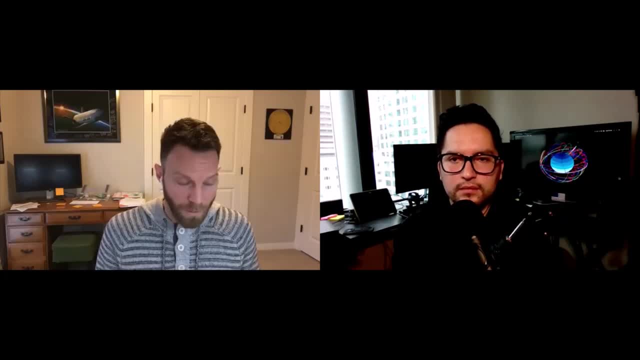 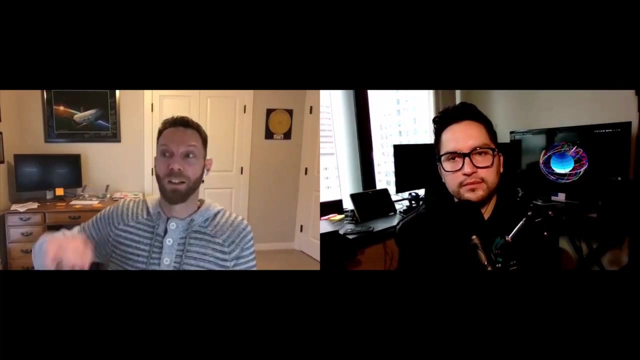 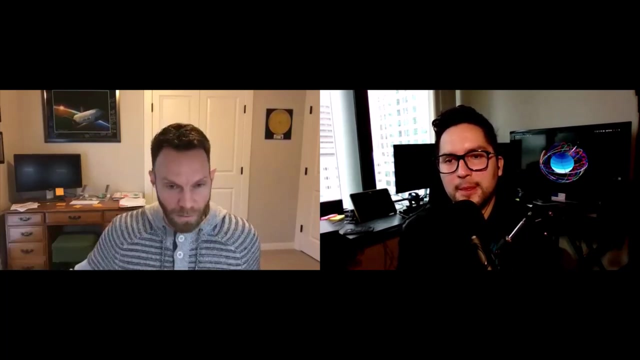 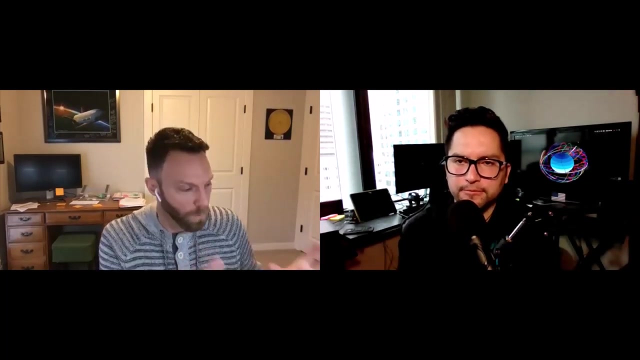 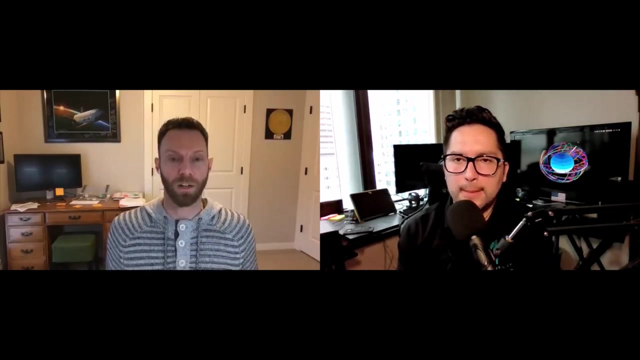 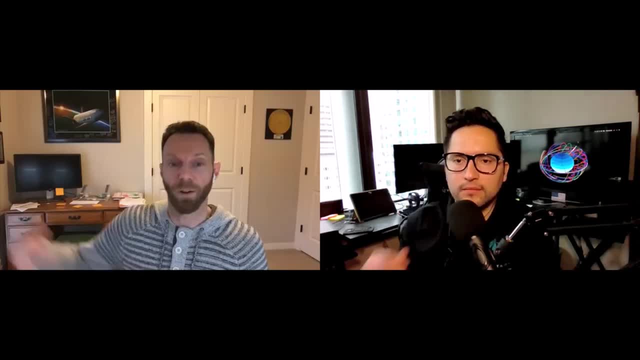 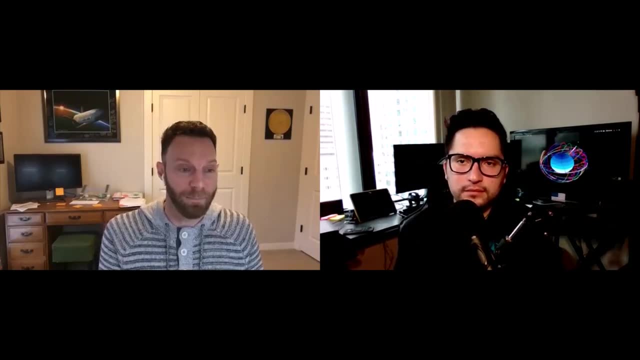 and test it on this platform as part of our future goals of going into deep space. Um, so, so we sort of, uh, you know, we had a bottoms up kind of approach to engineering there. We didn't say we 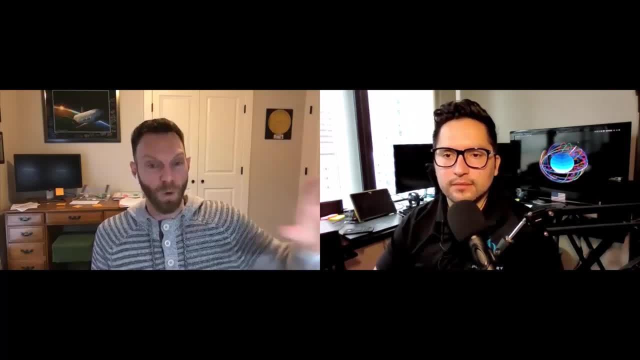 needed a star tracker because we had to meet pointing budgets. We needed a star tracker 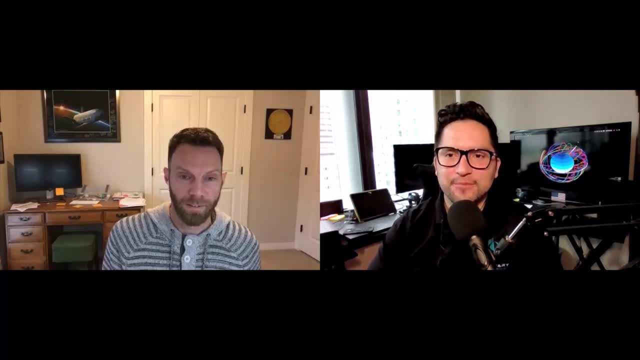 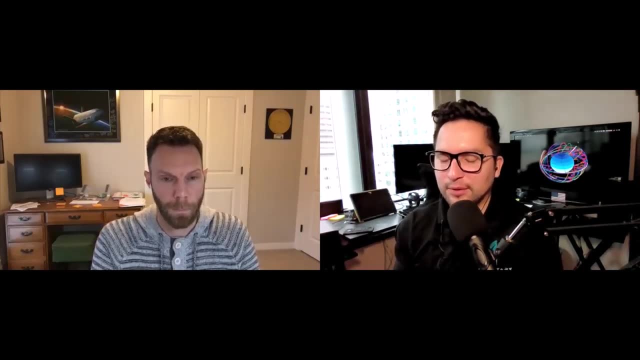 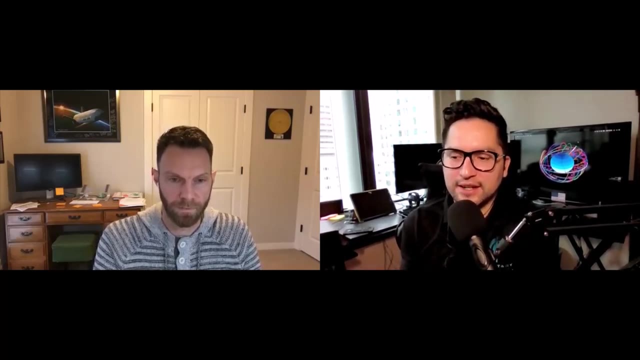 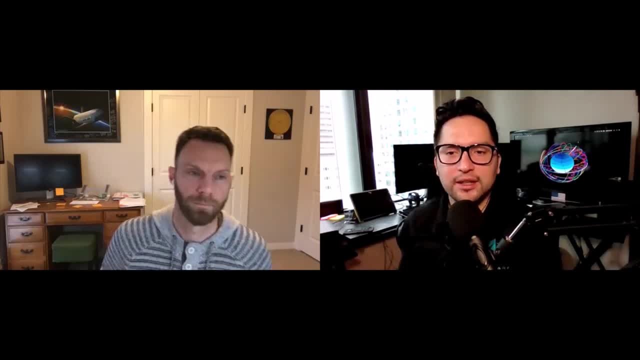 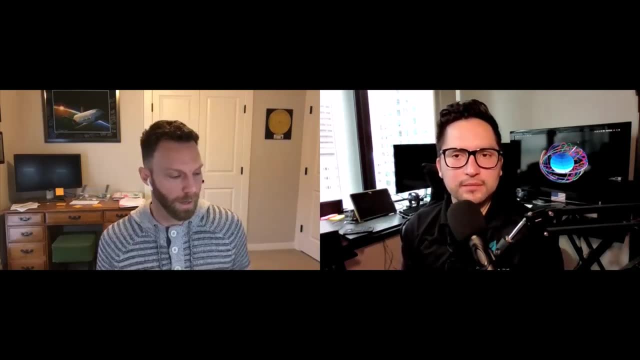 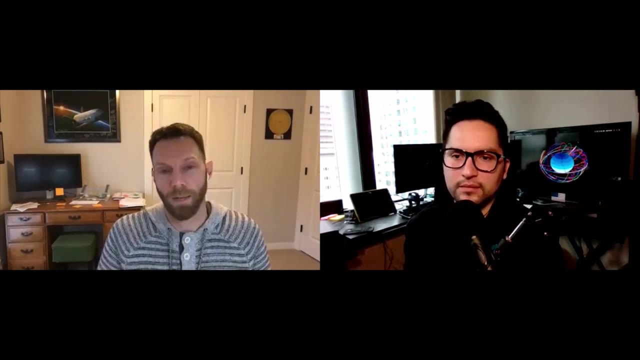 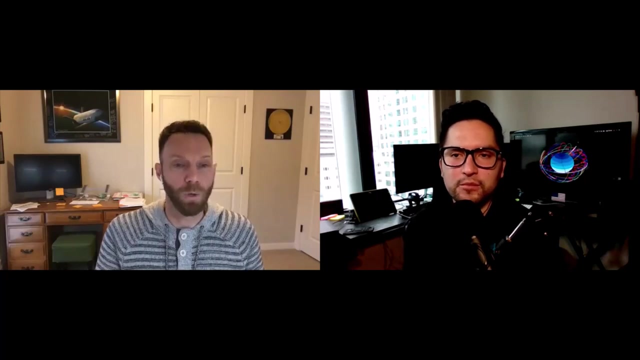 So can you go a little bit deeper into kind of how they actually work? Yeah, I mean, you've got the basics down. The details are all a little bit different by algorithms. But basically, they take a picture of something, you know, sometimes the moon's in there, the sun, the earth, hopefully not, you know, hopefully you're pointing somewhere into deep space. And you get back a mostly black picture with some, you know, bright dots throughout it. And, and let's assume all of those for now, let's assume all of those dots are stars, you would then have some kind of algorithm that would go through and scan through that whole image and determine what it thought were bright enough points to be labeled stars. And then it would label all of those stars and say, I think I've got these six points here are stars. Then the then there's another algorithm that's essentially doing a pattern matching between those six stars and what it already has in its star catalog of 1000 or 2000 or 10,000 stars or whatever it is that you need in order to to be able to determine your attitude in four pi steradian space to the degree that you want. So you want your smallest star catalog possible. 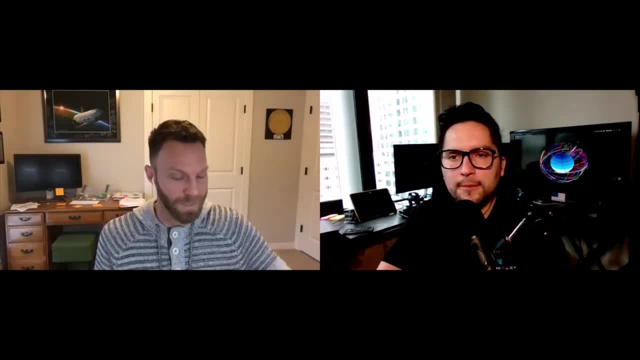 Because it, it, it costs a lot of CPU time to do that pattern matching. So you don't want a pattern match through 100,000 different stars. For example, if you don't need it, that's, that's just 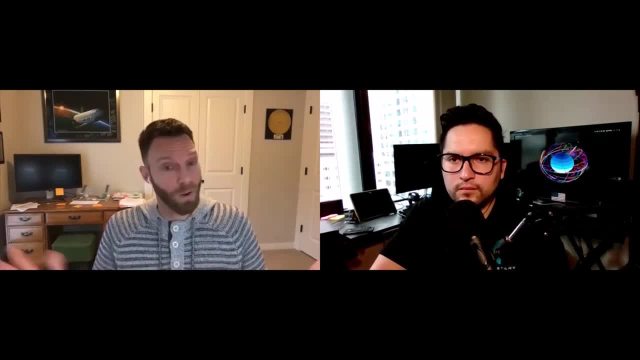 sort of wasteful. Now how they do that pattern matching there, they all do them differently. 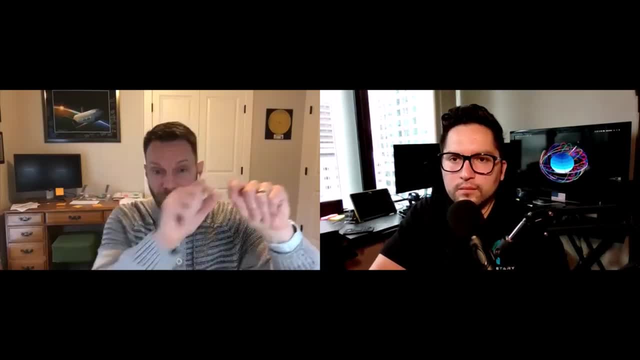 You can you can build like triangles between sets of three stars and you can you know characterize that triangle 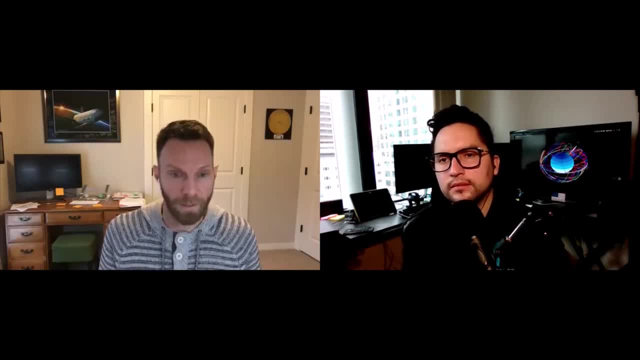 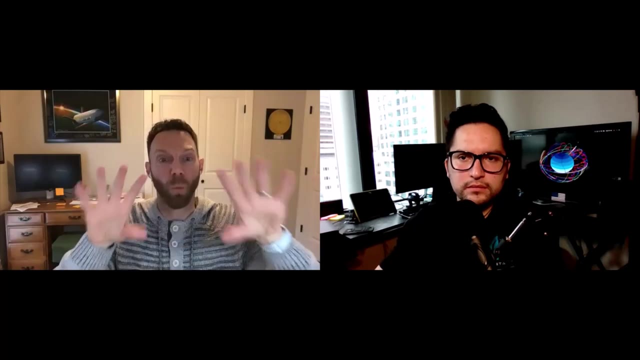 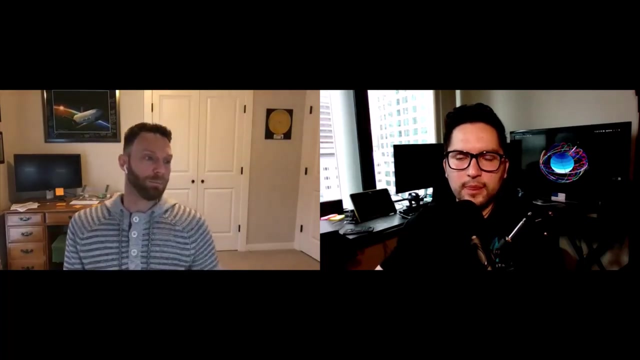 in some way either by the three lengths or an area or something like that and then you can quickly look through the triangles in your catalog and see which ones have the same ratio of those three lengths and and then how many of those can i match in one scene so that i can get more and more confidence that i'm actually matched the right pattern um now it seems easy but it's really 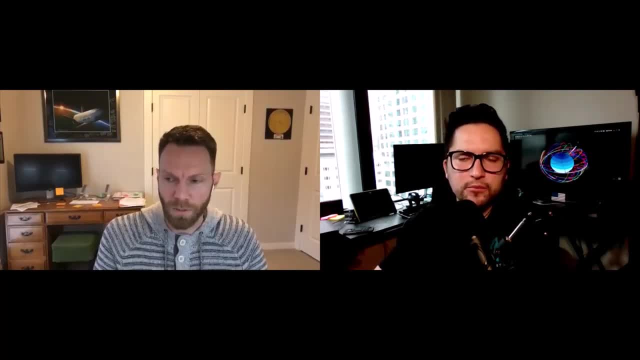 really it can be really difficult in certain situations because um cameras are are you know are sent are sensitive detectors and they're sensitive to like deep space radiation and all sorts of other hazards of space and so over time you start to get hot spots you know in dead pixels and so what you know you know 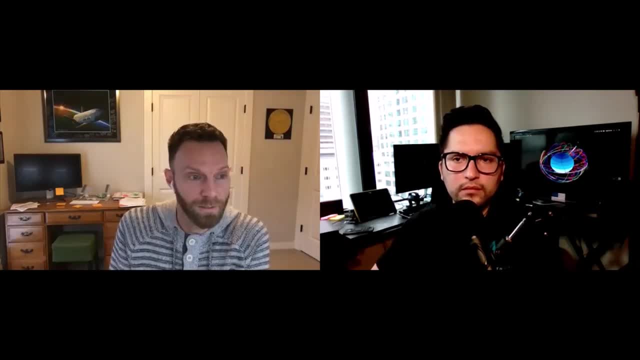 was a nice clean image at the beginning of your mission now has a bunch of what look like fake stars peppered throughout them um and you can then start mapping those dead pixels with like a 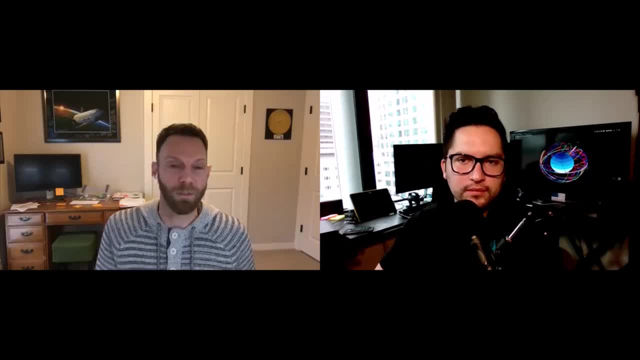 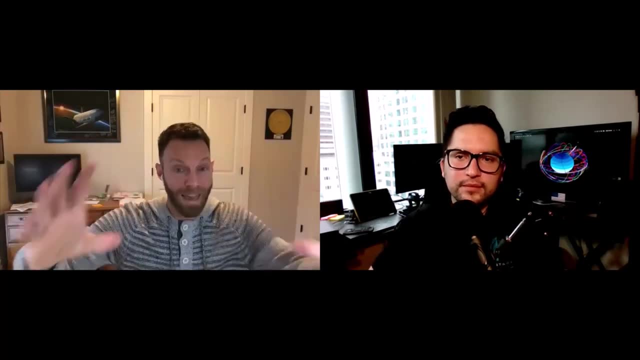 pixel map and subtract those or take them out over time and you're building up that map um there's a lot of sun glare you know the sun coming in at some side angle if your baffle isn't designed 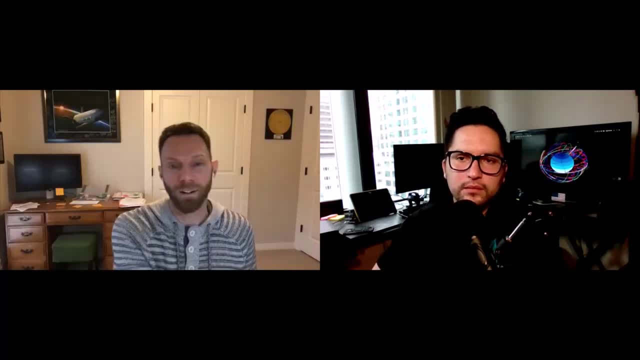 properly or isn't you know large enough you get a lot of glare and glint across your screen 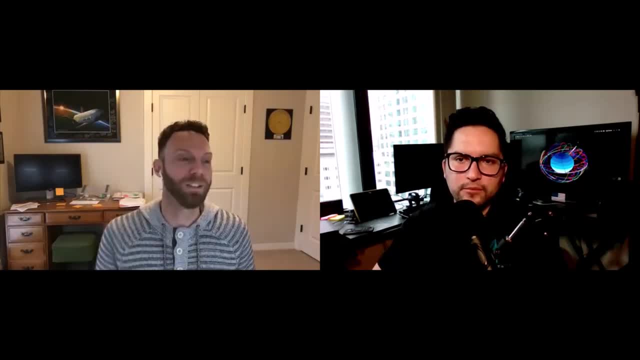 um the earth is in the way the moon is in the way and um and it's and it's easy to get confused as to what is a star and what is not a star so you know building a camera that can take a picture of 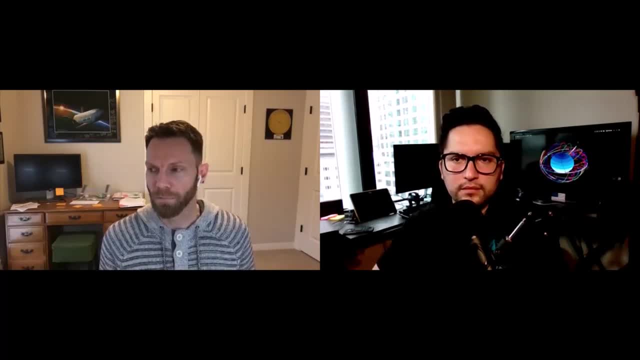 the stars is a relatively trivial thing building one that can operate in space and to the degree necessary so that you can your algorithms can actually pick out stars in the image is is tricky 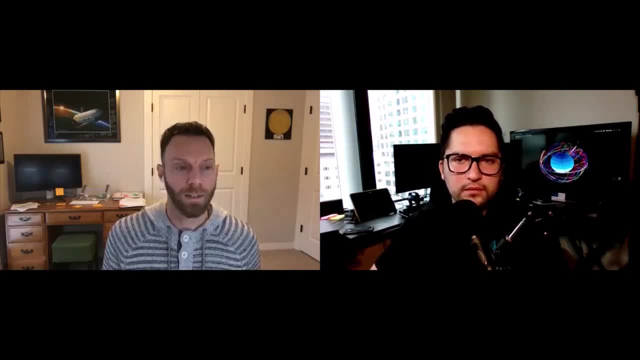 and it takes a lot of people a lot of time to get that right um so more often than not if you're only using one or two or three star trackers in your project it makes a lot more sense to buy one that somebody else has already gone through all of this effort of verifying and validating and 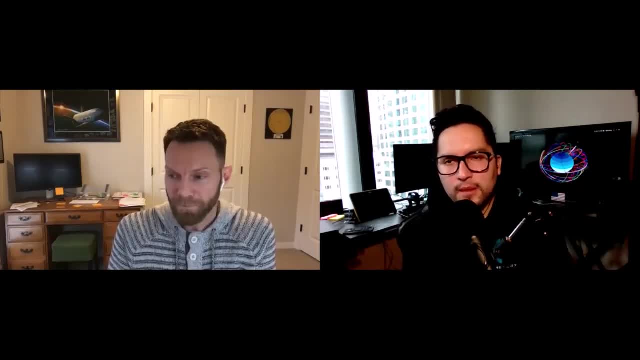 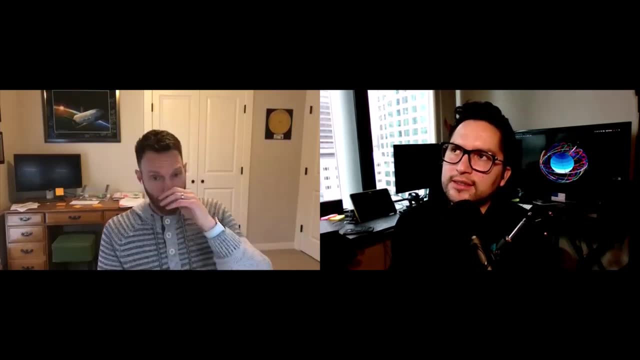 just running with it than designing your own it's not like a photodiode or something that can be done relatively simply so and what is 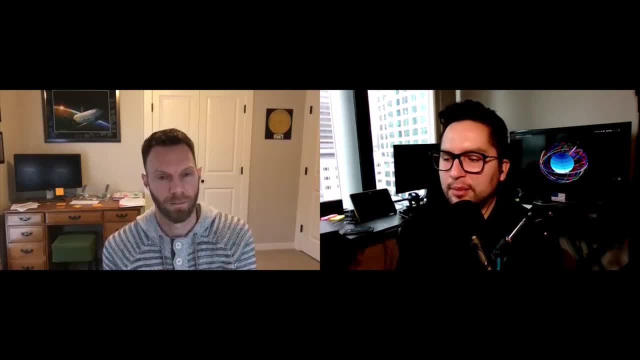 i don't think this is a trade but how much do you rely this is the question that that i want to go 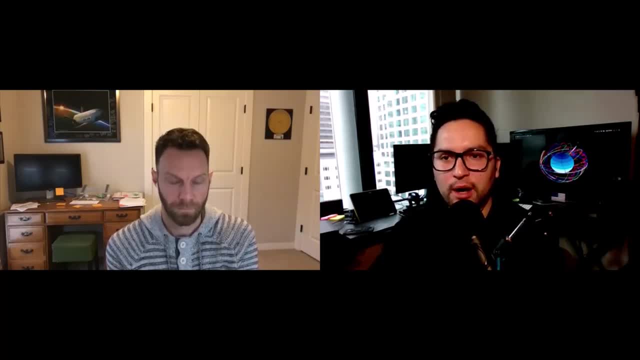 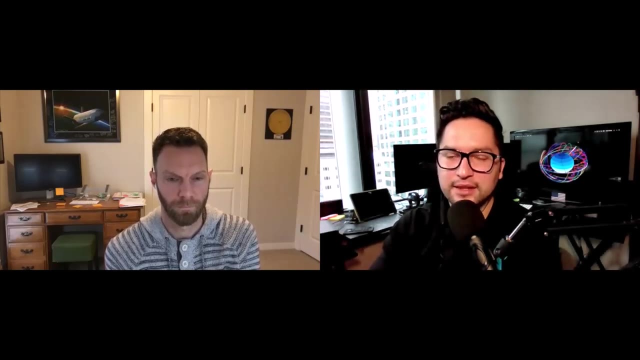 to is more is towards common filters so how much do you rely on say a star tracker versus a magnetometer as far as being able to determine your attitude and also does does it matter at what point in the mission you are because as you said um things can happen to the camera where it can make it less reliable so yeah so does that change over time and how does that change over time 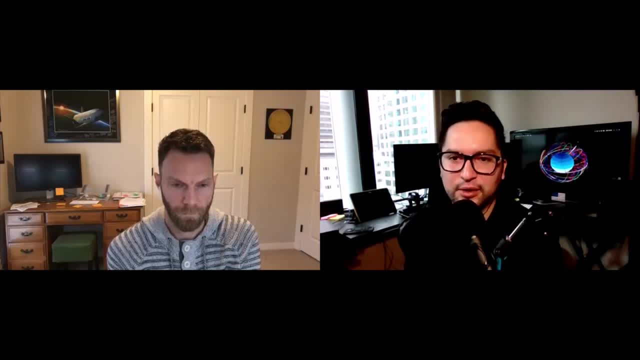 and how does that whole process go of determining how much i trust one sensor over another yeah so i mean there's the general idea of 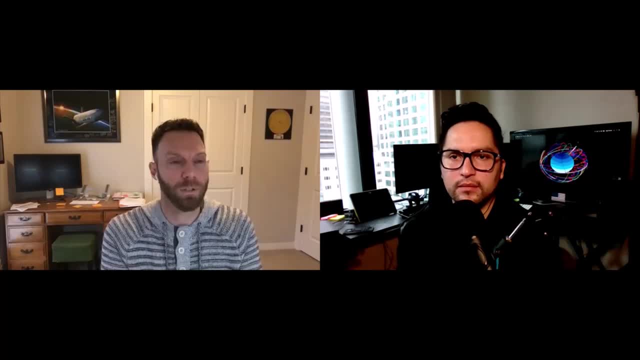 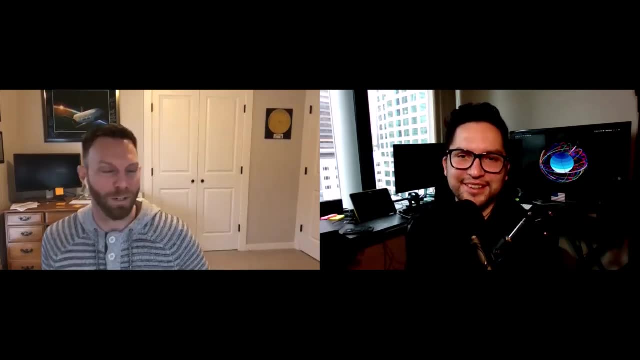 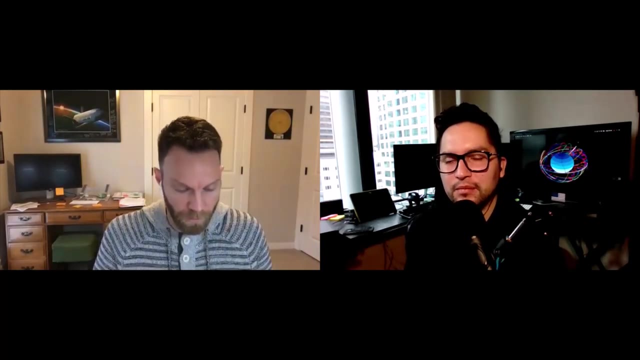 kalman filtering or like statistical estimation that um i don't know i could talk on this forever i don't want to take too much time so i'm gonna i'm gonna relate it back to what we did on a6 for example so in in a kalman filter 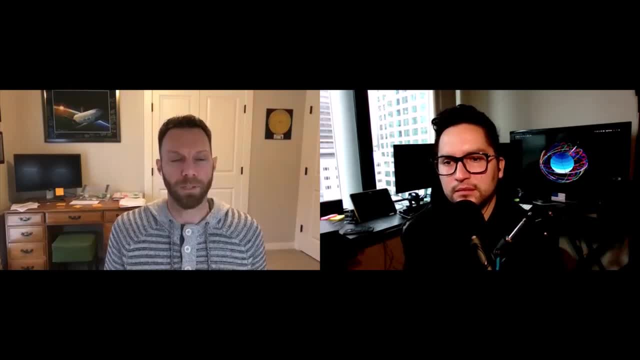 you are you have a mathematical representation of your system a mathematical model in the form of you know state-based equations or something and using that model you are predicting future state you're estimating what the system is doing over time without without looking and it would be like similar to being in your bedroom closing your eyes and walking to your kitchen you have a pretty good understanding of the map of your house 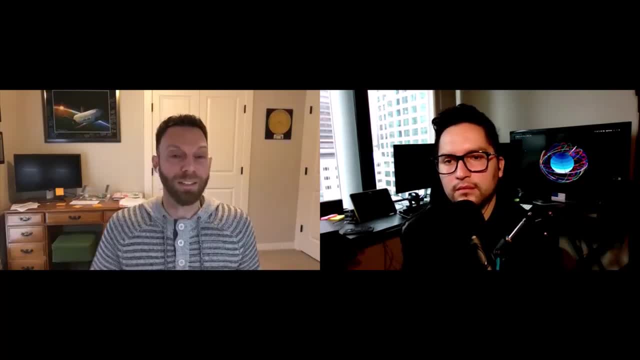 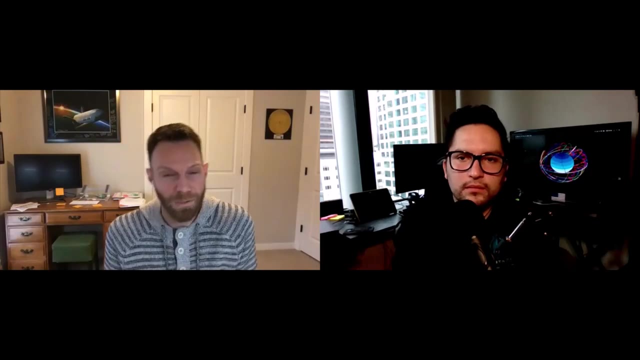 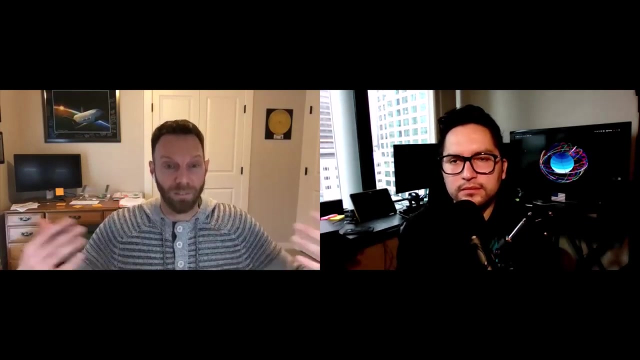 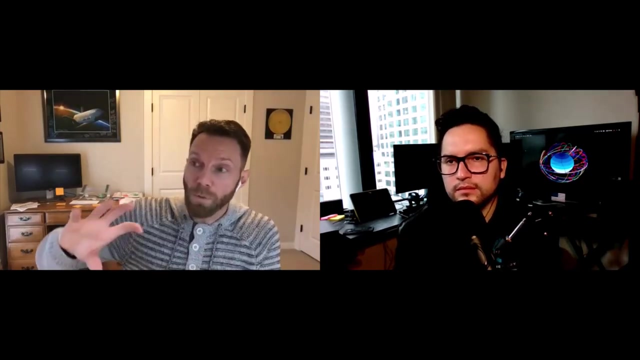 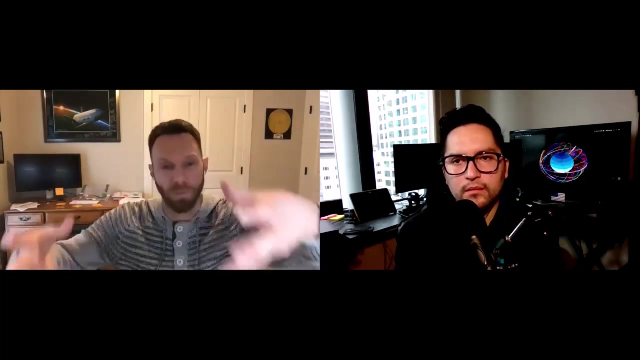 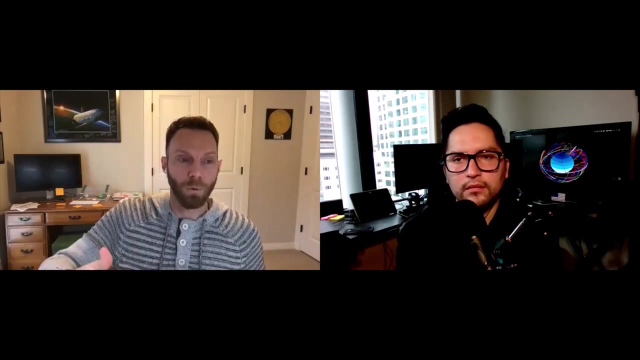 and because you can feel how you're walking and moving you can estimate where you are but the longer that you're estimating where you are the less certain you become in your accuracy i think you can easily walk straight out of your bedroom door without running into anything and being fairly confident but now if you turn did you turn 90 degrees or a little bit less i don't know and you walk a little bit further and a little bit further and eventually this estimate you trust less and less and less right and that's what this mathematical model is doing for us is it is essentially saying well i was rotating at this rate and in this direction before so in one second i should be whatever you know a little bit further and i've estimated that and one second later i should be a little bit further and the longer you go predicting and estimating your future state the less confidence you have in it so then occasionally let's go back to walking across the house you get halfway there and you're like i i feel like i'm going to hit a wall i'm just not confident that i know exactly what i'm going to do and i'm going to hit a wall and i'm going to hit a wall let me just open my eyes real quick you reorient yourself you're like ah here's where i am and then you can close your eyes and keep walking and that's essentially what we're doing with a star tracker is we're opening our eyes occasionally and saying where are we actually and then the 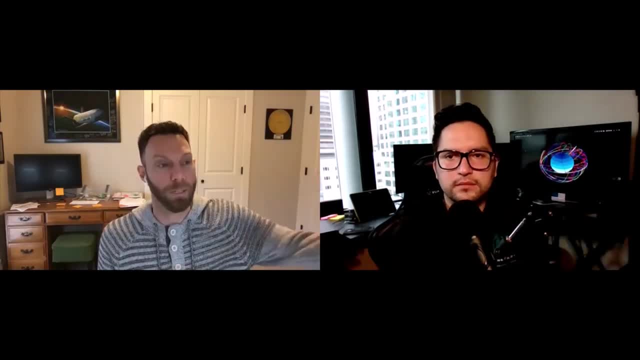 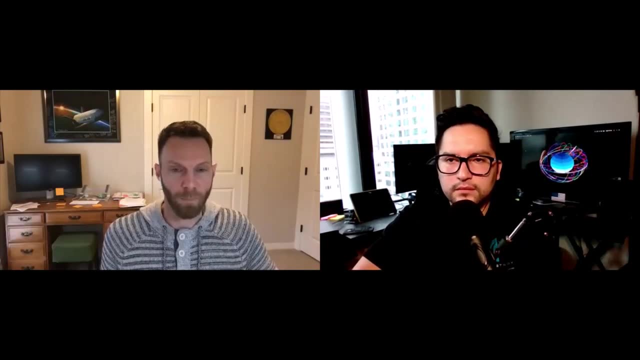 kalman filter combines those two estimates the one that we predicted with a model and the one that we sensed using a sensor um with the case of your eyes your eyes are probably pretty accurate so you would trust them 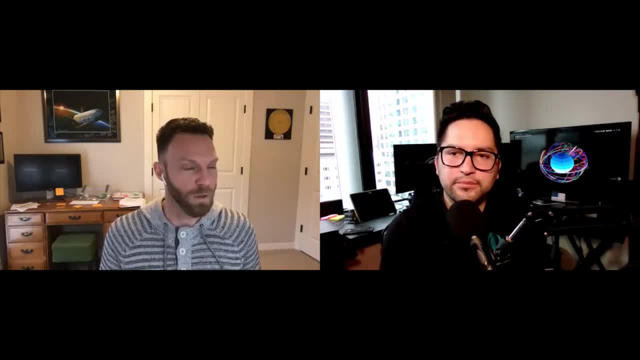 a whole bunch when you reorient yourself unless maybe you know you you wear glasses you don't have your glasses on it's like a fuzzy world right you may not you may have some error in your 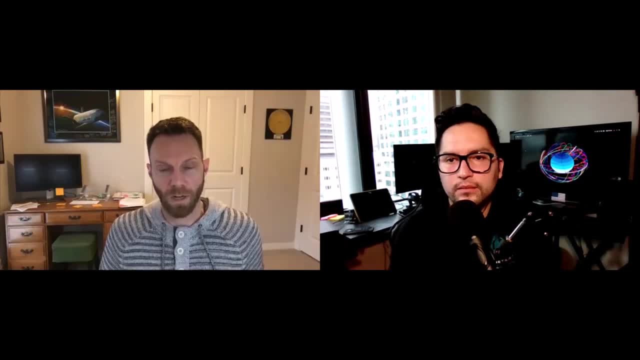 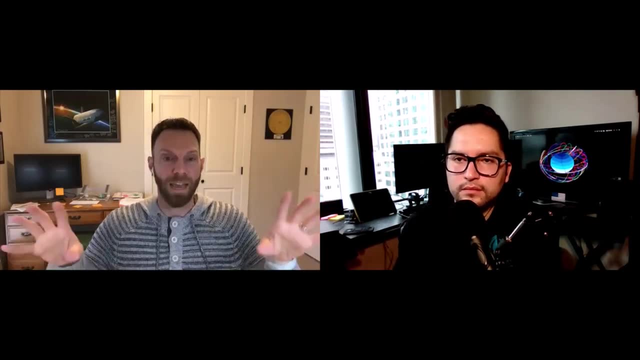 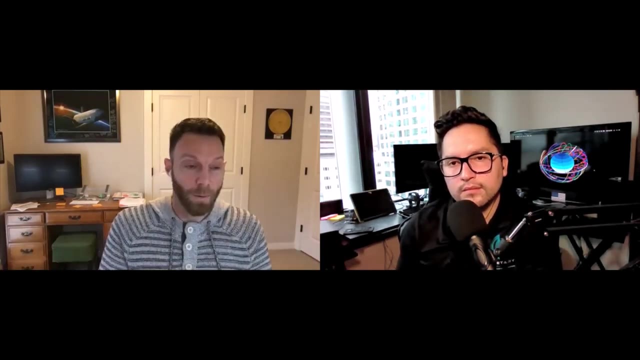 sensors well on our spacecraft we do have errors the star tracker isn't perfect our estimate's not perfect and the kalman filter is a way to blend these two imperfect estimations one estimated from a sensor one estimated from a model blend it together to get a good state estimate now 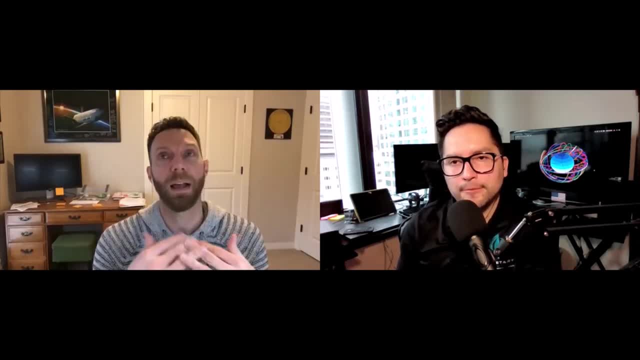 how that estimation well not how it's done but how much do you trust your prediction and how much do you trust your 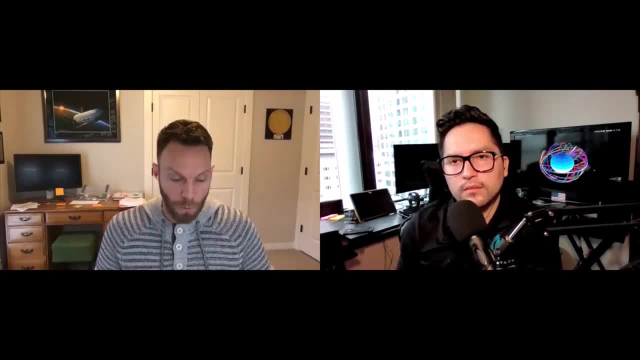 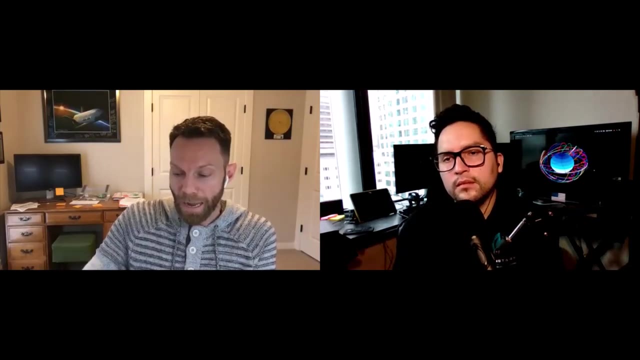 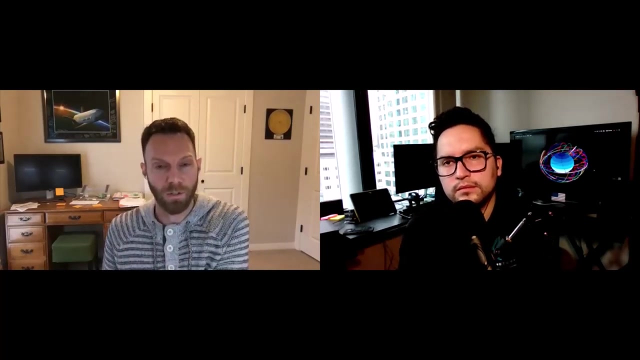 sensor um you you can bake into the kalman filter ahead of time by knowing how good you built your model and by knowing how good your sensors are but in the case of star trackers and other sensors that degrade over time you can change how your your your sensor um noise like how how much noise there is in the sensor and you can change how much noise there is in the sensor and you can change how much noise there is at that at that point in real time so with a star tracker i said like if you 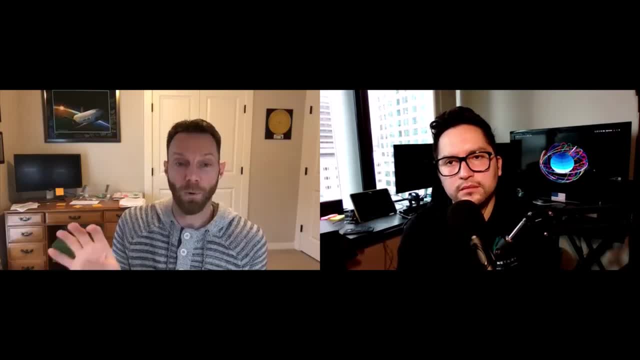 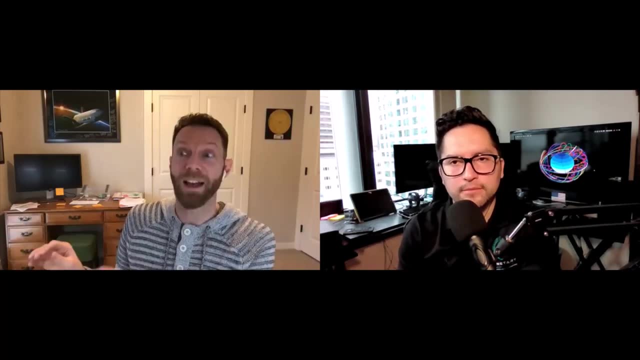 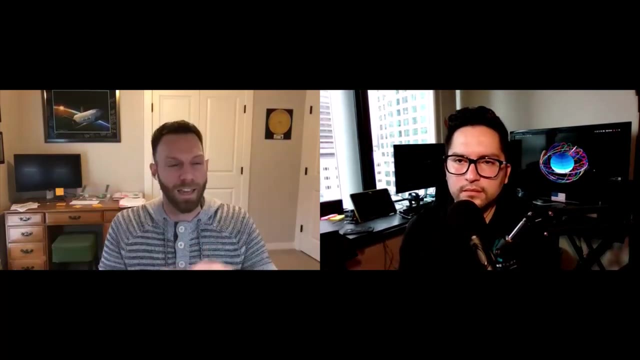 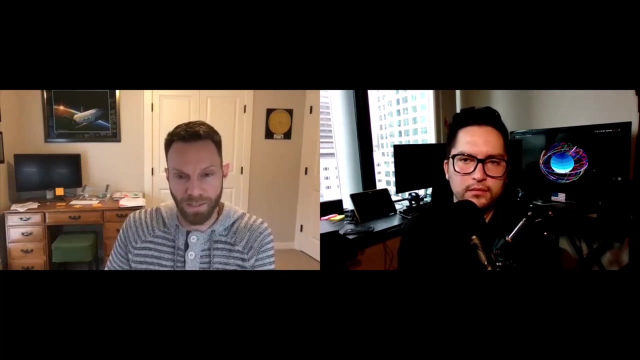 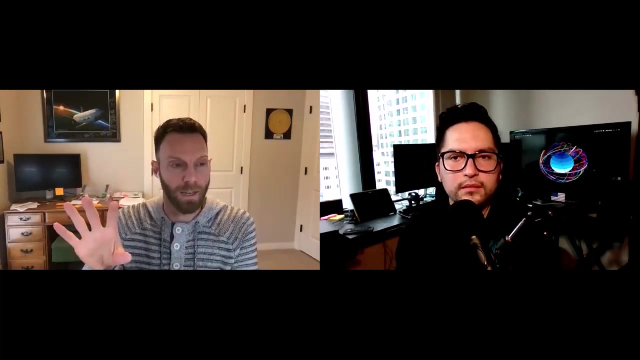 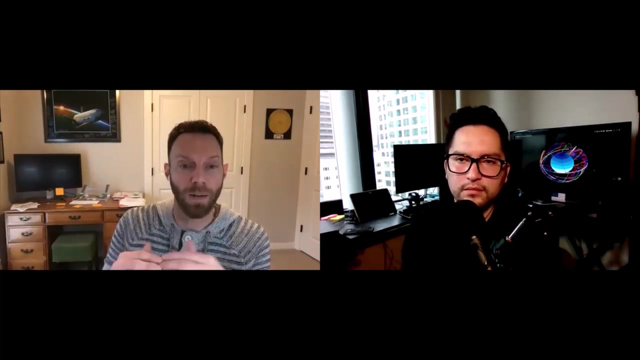 can see four stars that estimate is not going to be as good as one if you can see 16 stars imagine 16 stars and you can match that pattern into your star catalog you're going to have a lot of confidence that you're looking at the right thing and each one of those errors of each of those stars is going to kind of blend together and and rss root root some square out of there and you're going to have a better estimate of where you're pointing versus four so the star tracker comes back you're going to have a better estimate of where you're pointing versus four so with its own guess as to how good it's doing based on how many stars it sees and how fast the spacecraft is rotating. Because you can also imagine that when the shutter is open on this camera, if the stars are sort of streaking across because you're rotating, you don't have these nice point stars. You don't have these streaks. And you think, okay, well, I can still send TROID on that streak and say it was in the middle of that streak. But were you rotating at a fixed rate? If not, then it's not the center. So rotating a spacecraft while doing star tracking decreases its error. So you can take all of that information and then how long you've been operating, like one month later, three months later, four months later, you might start to degrade your sensor just because, like I said, with these hot pixels and dead pixels and stuff. 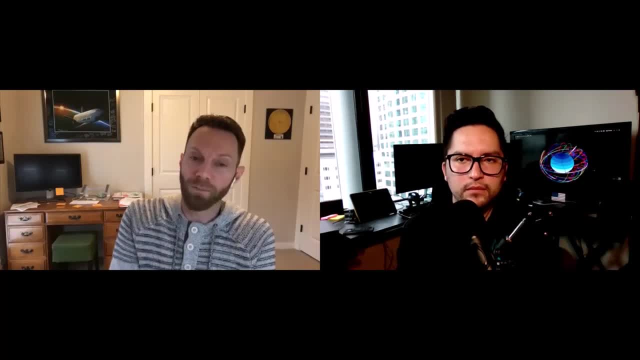 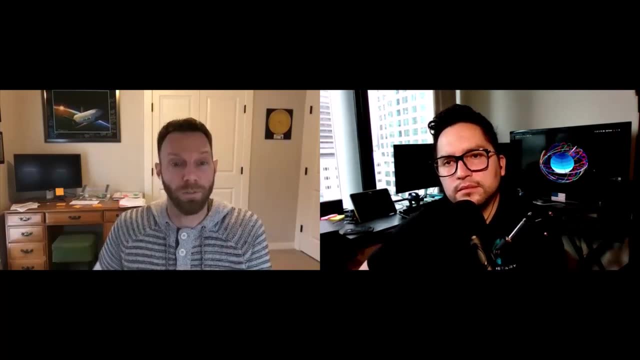 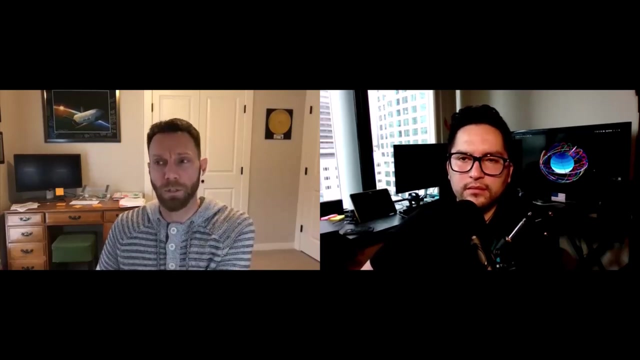 So you can take all of that information and you can put that into your Kalman filter and say, this is how much I trust my star tracker. And this is how much I trust my model. And this is how much I trust whatever other sensors are going into it, my magnetometers or whatever. And the beauty of a Kalman filter is that it takes into account all of those statistical distributions and comes back with an optimal estimate given all of that information. So as long as your information going into it is accurate, what's going to come out is the optimal estimate. 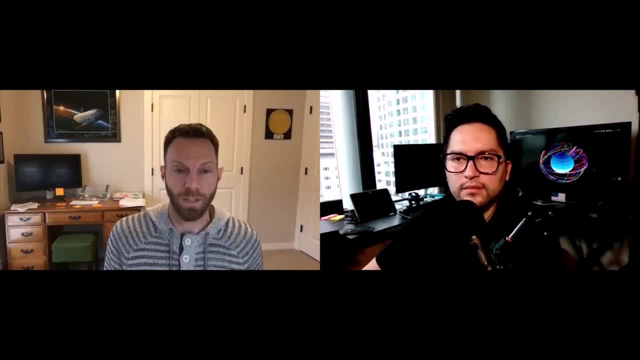 That blends all of those statistical uncertainties and everything. 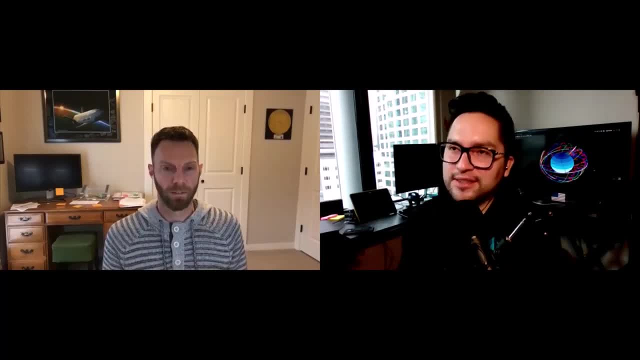 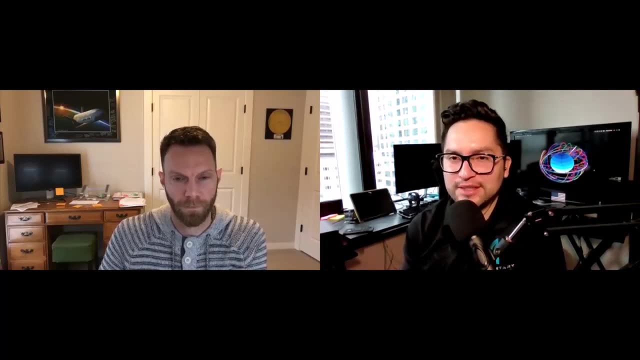 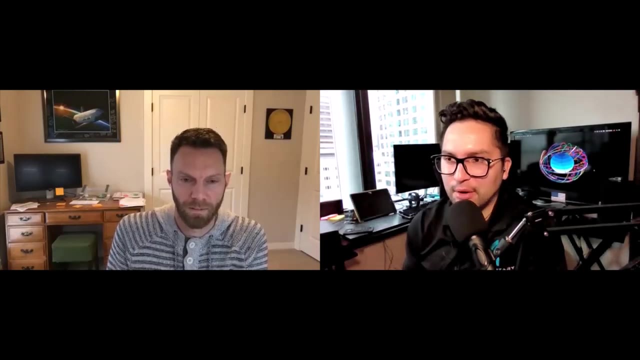 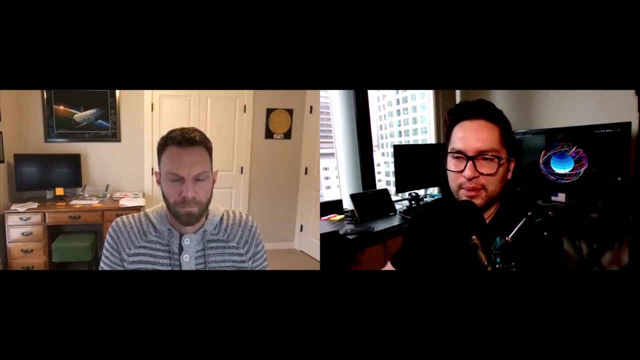 So that sounds, that was the, the process sounds more involved than what I originally thought for star trackers. So how does that, so I want to get into flight computers and I know you said you don't know too much, but I still think you know more than most people. So how does the process of picking a flight computer, so how much compute power do I need? What kind of clock speed do I need in order to be able to do that? How do I need to be able to make all these calculations in real time on board the spacecraft? So I kind of, yeah. How does that process go of picking a flight computer? 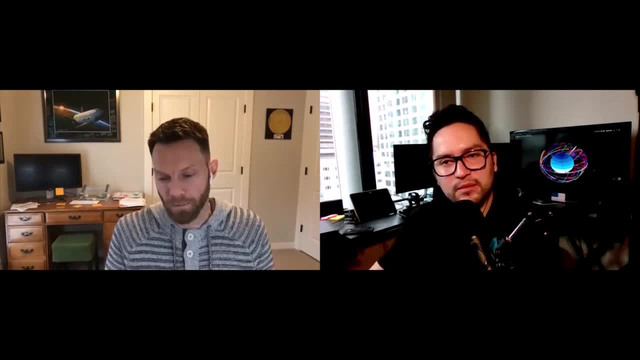 Yeah, well, I'm, let's stick with star tracking for now. And it's, it's not straightforward. It's not like you can sit down and say, this is, this is how much processing I need to be able to do because there's trades in everything. 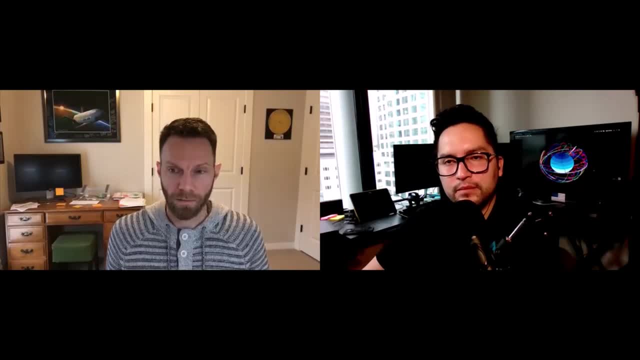 The algorithm that you choose to do pattern matching can vary in how many operations it takes wildly, right? And, and the result could be that it is, you can have a slower processor with less memory and, and have a less accurate result because you need to, you know, you need to do your star tracking in a 10th of a second. So just get, get me whatever you can in a 10th of a second. That's all I have, like for example. 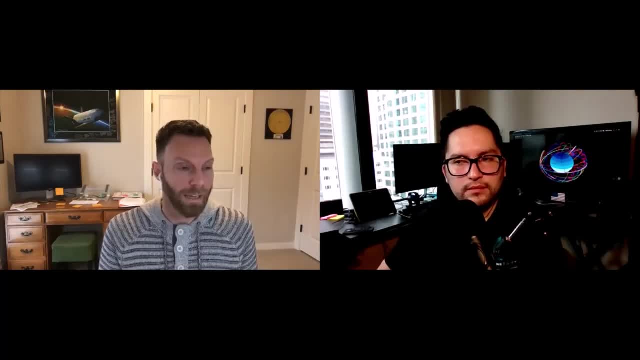 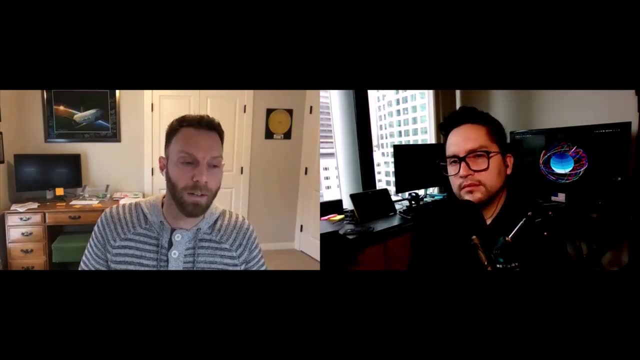 So, so there's the algorithm side of things. There's the flight software side of things, and there's the requirements on pointing. Like maybe you need a star tracker to update a hundred times a second because it is your only attitude sensor and everything else runs at 100 Hertz. So I better be getting measurements back from my star tracker at a hundred Hertz. Otherwise I don't know where I am. You know, let's say. Versus. 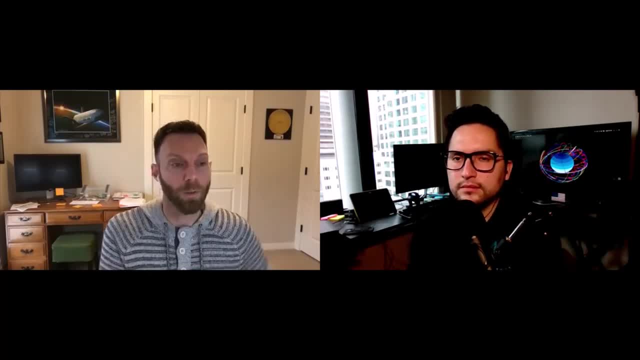 My IMU, my inertial measurement unit and the rate gyro built into it is really accurate and I can dead reckon using just the IMU for an hour before I start to break my pointing budget. 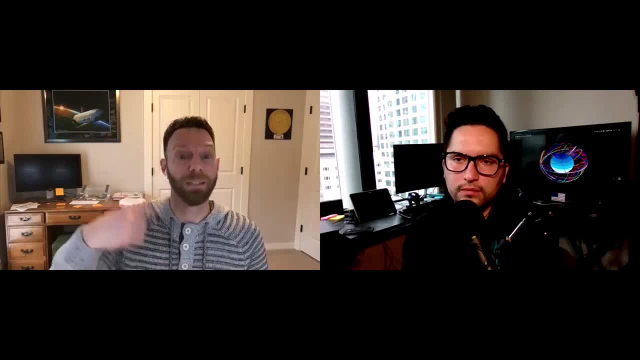 In which case the star tracker can be turned off because I'm just going to predict where I am over time. I'm going to use that mathematical model and I'm going to predict where I am over time using, you know, my IMU. And then once an hour, I'm going to wake the star tracker up, take a picture and it can turn on that picture for 10 seconds because I don't really care. My IMU is amazing. And then you're just going to turn slowly for 10 seconds, return a quaternion or, you know, an attitude estimate. And then I'm going to fold that into, you know, my Coleman filter and I'm going to, you know, estimate new state and then turn the star tracker off and then just keep going. And all of these things are interrelated with each other. 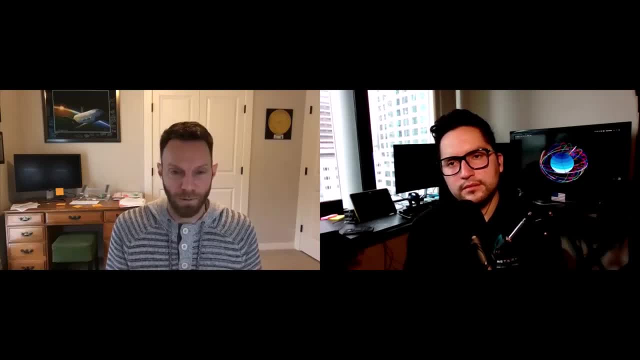 So it's this big swirl. It's really just a big swirl of how good is my algorithm? How much, how, what are my requirements and what compute processors exist? 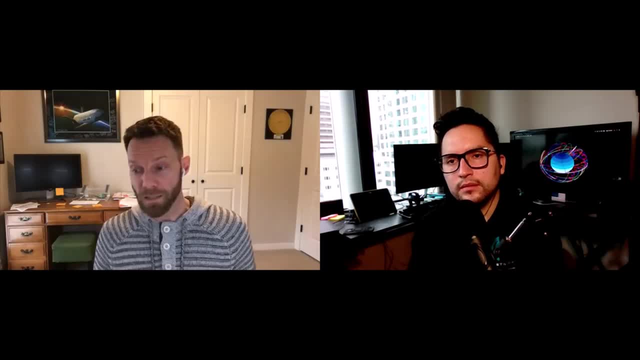 And what can we get away with now for A6. 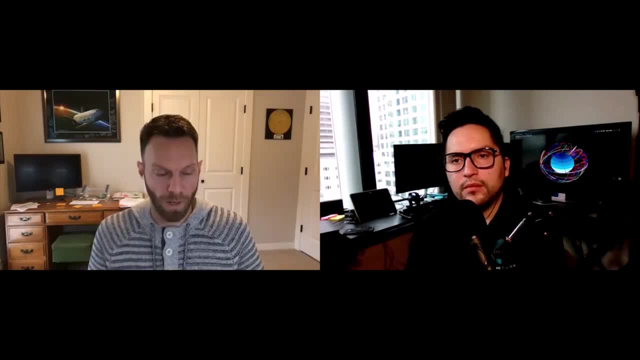 We weren't, this is why I say I'm, I'm, I don't know a whole lot with it in this side of things is because we ADCS. When I say we, I mean ADCS didn't drive the selection of the processors. 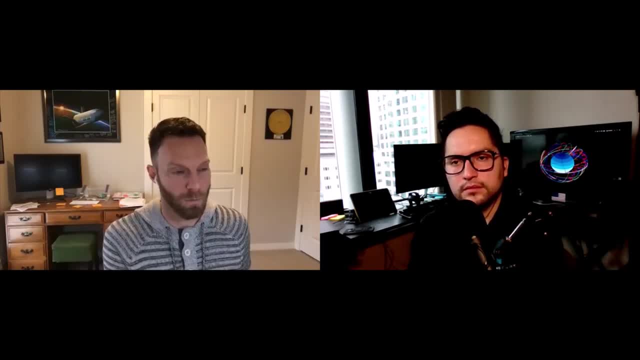 We those, those processors because they existed you know some of them existed as a carryover from a3 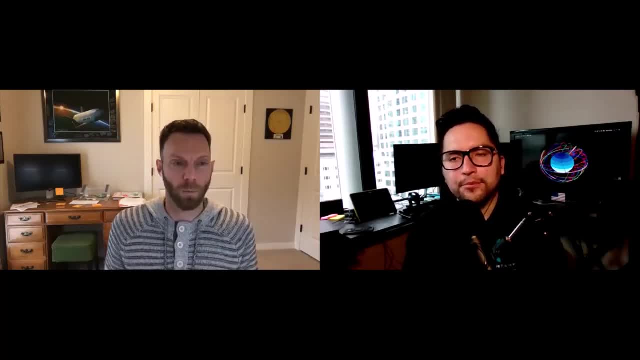 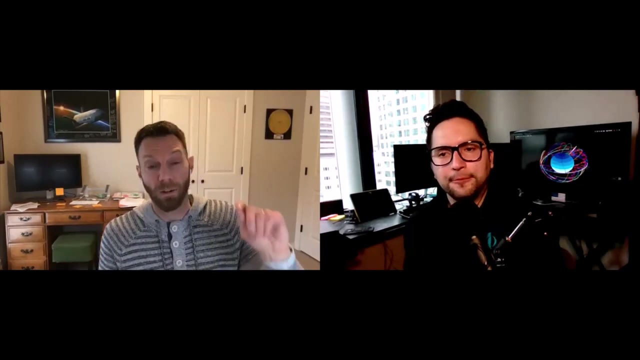 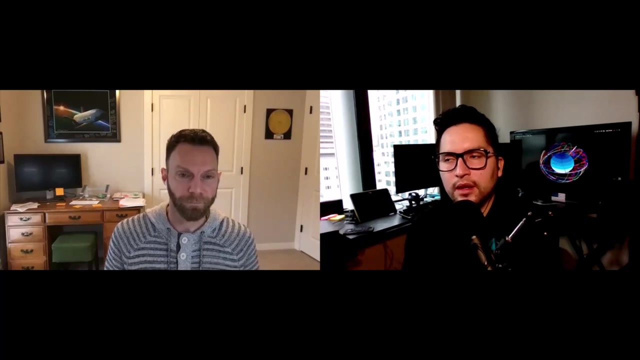 and the architecture already existed we had to find a way for the most part to fit into the box that was already created for us and so we had to um we had to use the resources that already existed and we had to adjust our uh requirements in some cases but we had to adjust that trade between how good does our algorithm need to be how good does our imu need to be because our flight computer can only do so much for the most part so you you mentioned quaternions and i want to get 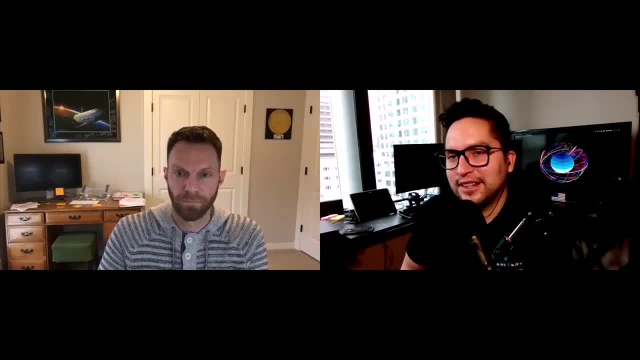 into that because first of all i think quaternions are super interesting and then you can get you 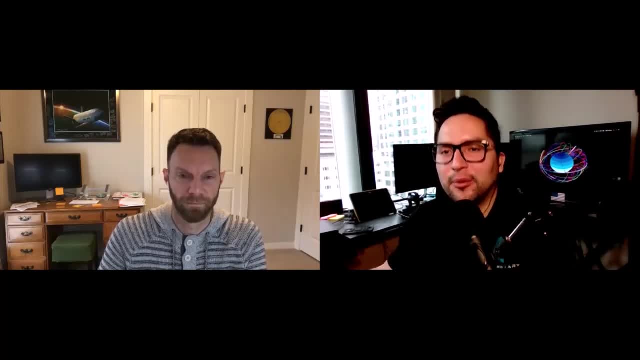 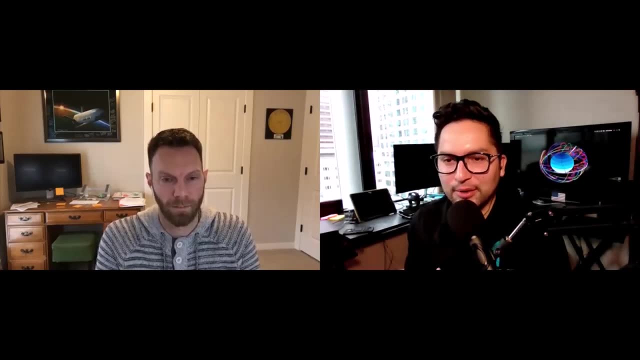 know deep into the math where it's kind of just really crazy um but one thing that i'm struggling with and i kind of want to get your guidance on is that i'm currently working on making a video about euler angles and i'm a little bit struggling 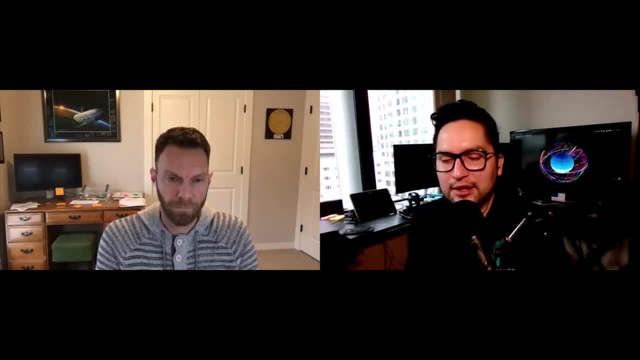 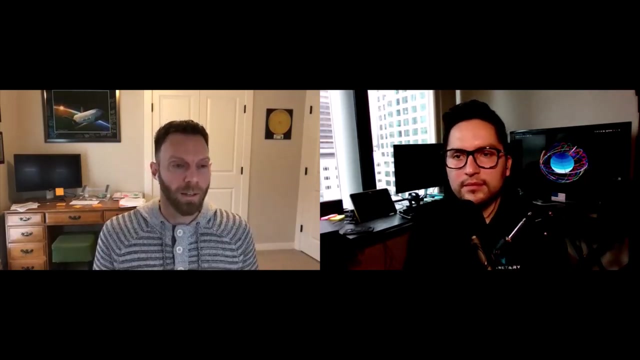 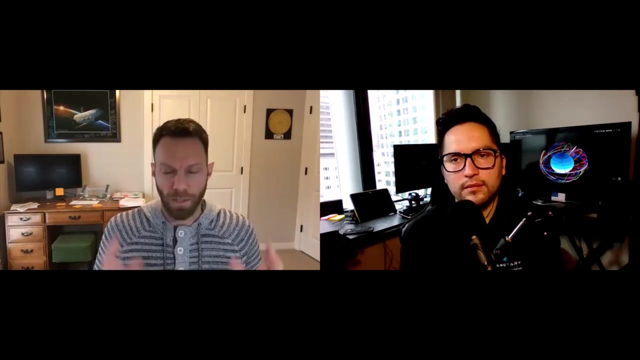 to find out because i know mathematically this is how you use them this is how you describe one reference frame with respect to another using euler angles but how did you use and in general how do you use euler angles or if you do for spacecraft attitude control for doing analysis on a control system and and also that versus quaternions and then when do you do one versus the other yeah so quaternions which is which is using four elements to um to represent a rotation between two coordinate frames so that's what we're talking about here we're talking about a rotation um is is a very i mean there's a lot of benefits to using it within flight software you know you don't have the gimbal lock problem you don't have nine elements that you have with a direction cosine matrix you only have the four so it's very compact and you don't have a you can set up a a multiplicative callman filter to to do all of your attitude estimation in 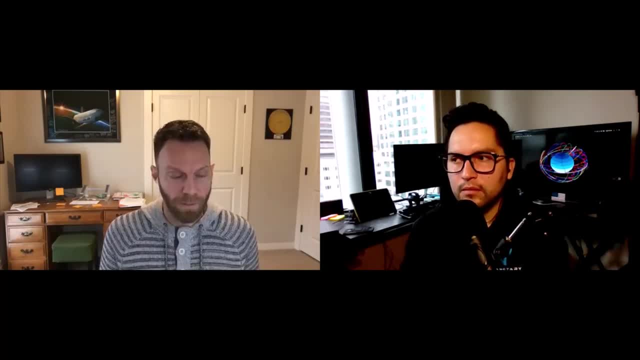 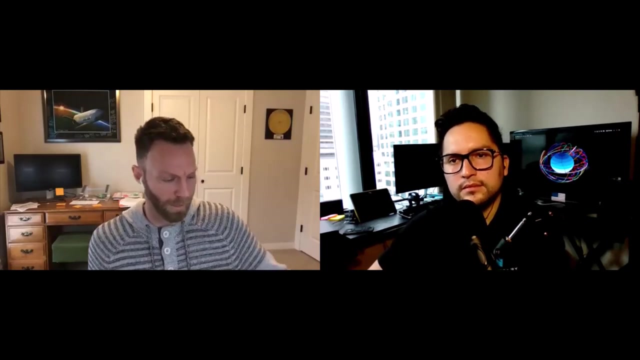 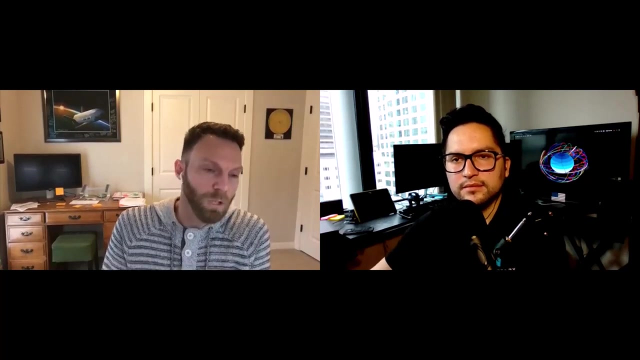 in you know with quaternions and all that stuff but they tend to be a lot harder to visualize and understand and so we did all of our processing in with quaternions on the flight software but then we did all of our visualization in well not all of it but the majority of our visualization in euler angles so when we determine how um you know just we're we're we're looking at at a time history of pointing for example more often than not we would convert that into something that we can look at and make some sense of even if it was um you know we didn't have to do this but even if it was like a small angle approximation which is oh it's a small angle approximation which is a small angle approximation so as long as uh you know like a like a zero like a no rotation of a quaternion is like one zero zero assuming the scalar is first um then then as long as the rotation off of that is really small all of those three numbers after the one is all really really small you can just take those and i can't remember it off the top of my head here but like double it and those are the gradients um in euler angles approximately uh something like that uh well you know you can take those and you can take those and you can you can get a sense of how how things are are are progressing in your control system very quickly just by by looking at it that way um so i agree like euler angles degrees 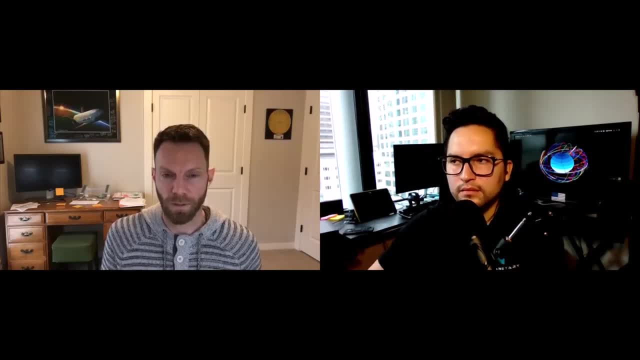 those types of things are much easier often for humans to interpret but we we wanted to keep everything consistent within flight software so there's no reason to use degrees within flight software for us there was no reason to use 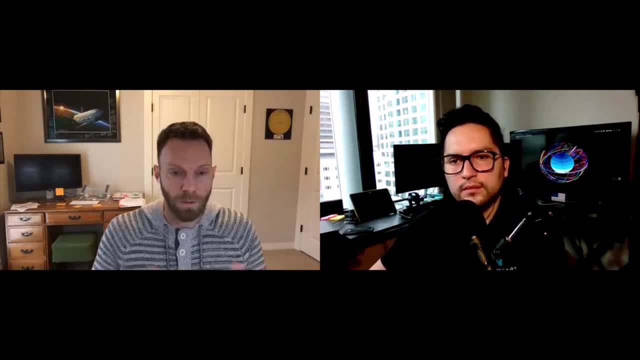 anything other than quaternions because the computer is interacting with itself there the software is interacting with itself only only as an outsider when i command something we may want to command it in degrees possibly we may want to view it in euler angles possibly all of that stuff 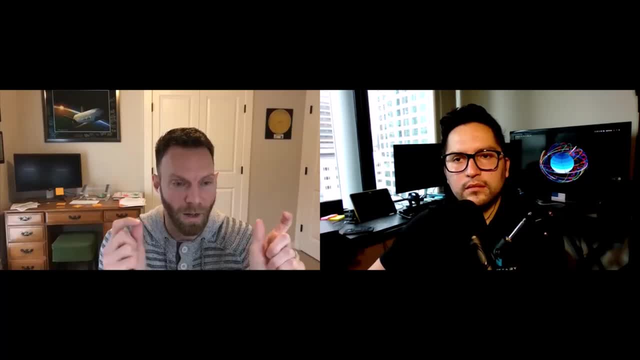 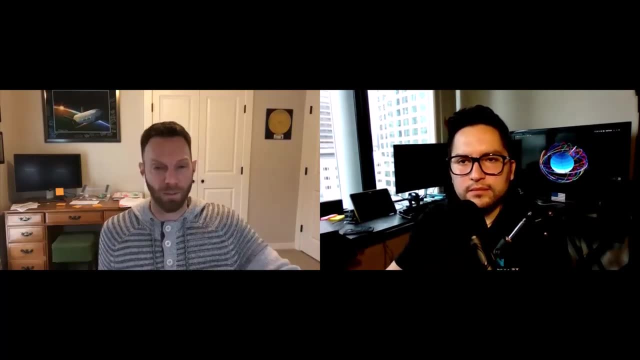 are sort of wrappers that we would put uh or you know or post-processing algorithms that we would put outside of flight software everything 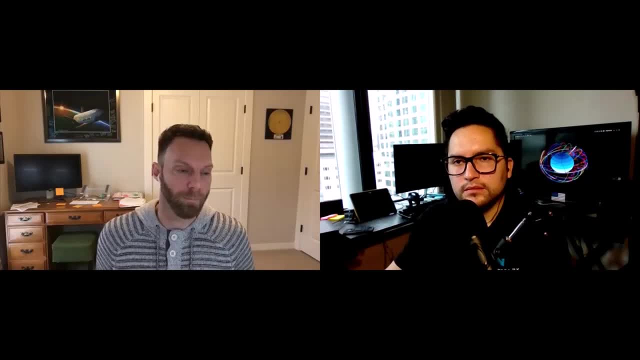 within flight software is consistent with with units um that that are set up for the algorithms themselves and not for people to interact with them so putting you on the spot a little bit is 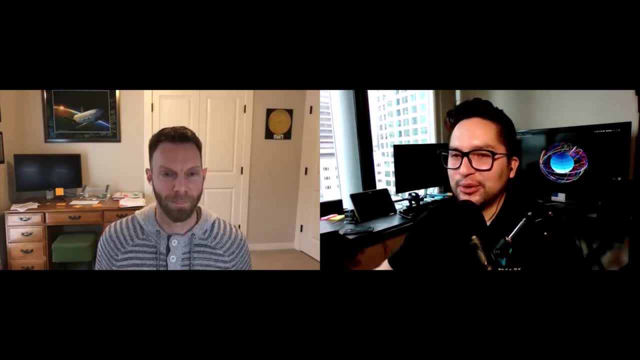 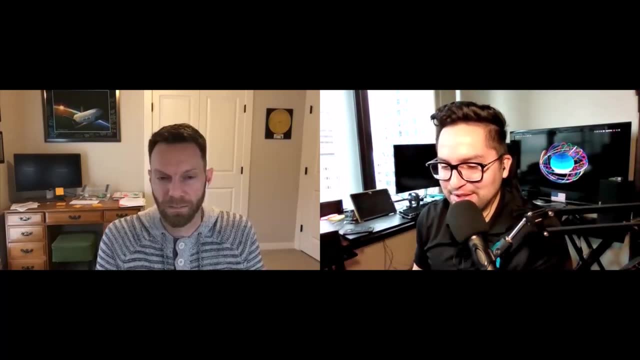 there any way do you think that you could intuitively explain quaternions because i think they're super interesting and just you know the fact that they're four dimensional imaginary numbers is kind of crazy um so yeah do you have anything that you use in your head that you kind of for yourself just intuitively explain quaternions because i think they're super interesting and just 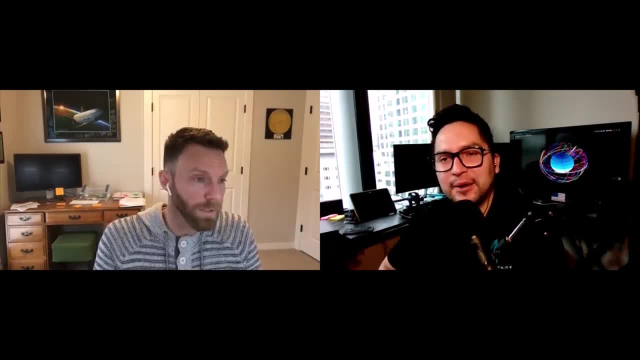 intuitively what a quaternion is well like a quaternion you know the specifics of how those 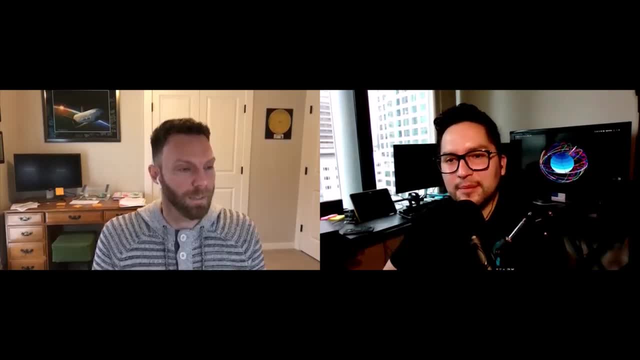 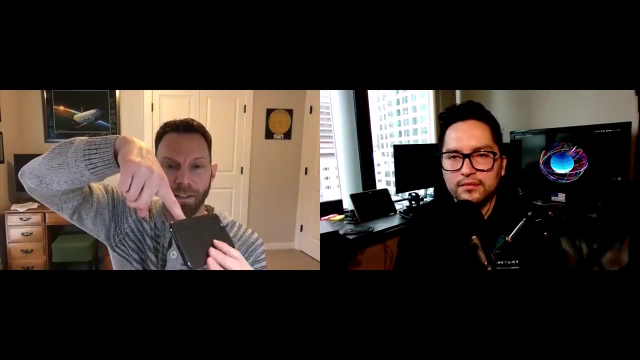 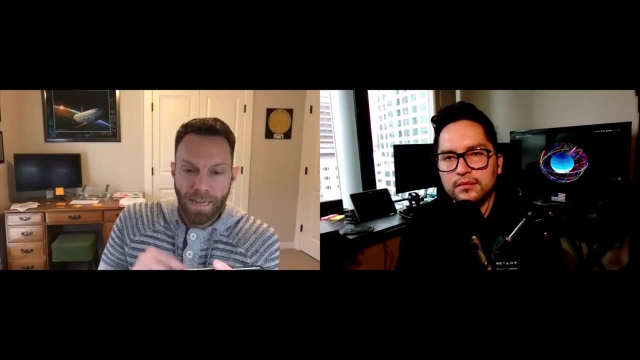 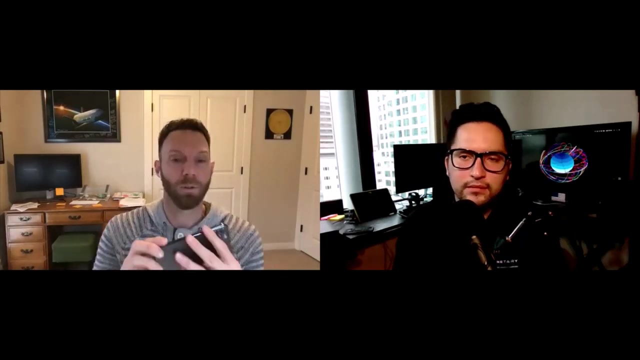 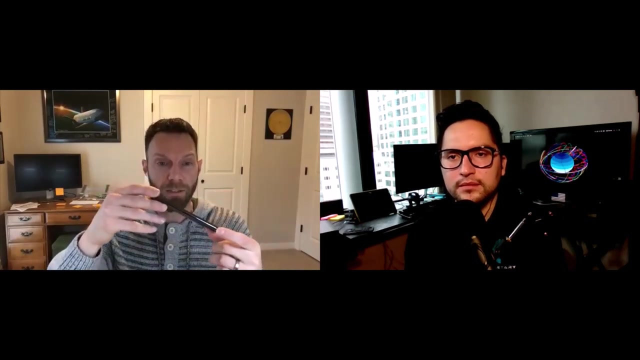 numbers come about can be a little bit mind-bending but i think in terms of angle axis um like representation makes a lot more sense so uh the the craziest thing about angle axis in my mind is that you can you can describe any rotation like if i have my phone here i can get from this orientation to any other orientation by rotating along a single well defined axis so i can go from here with this vertical axis here and rotate around it this way i mean that makes a lot of sense and i can rotate it around it this way but if i rotate it around some crazy angle off to the side it's going to do some kind of weird flip and it's going to end up somewhere so the key the key to angle axis is that some axis in in in any direction and you know if you define that axis and you rotate around that axis some amount of radiance you can get to any other rotation so that's sort of the key behind it and the intuition behind that is is lost on me right now i wouldn't know how to explain like why that's the case uh but if we go in with that assumption that that's the case things start to make a lot more sense so now instead of euler where you're saying rotate first in this axis then in this axis and then that axis instead of doing three rotations 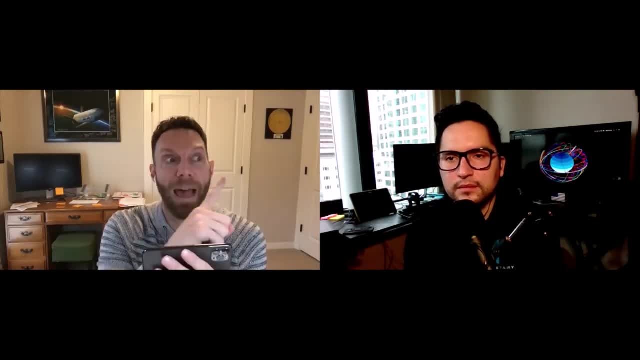 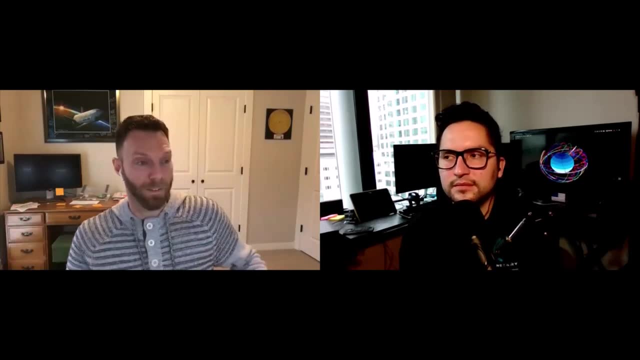 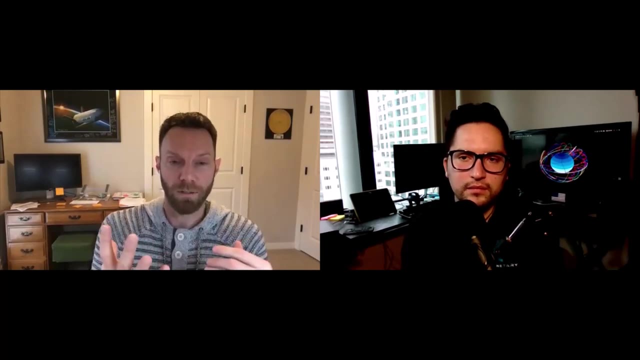 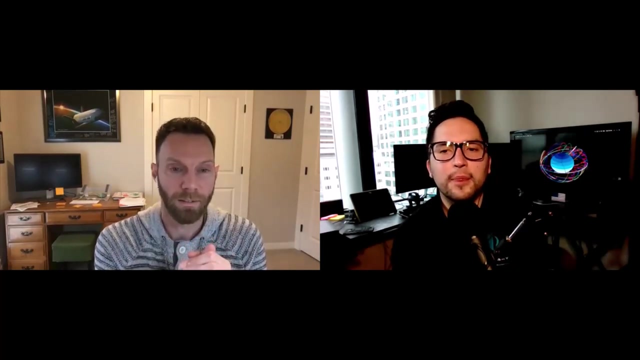 you're only doing one and you're doing one rotation around some axis that's really strange like some weird direction and that's it so now you can find that axis determine how far to rotate along that axis and you got your four numbers the axis is defined by three of those numbers and then the the angle around that is defined by fourth number but now you now you have to say like well that's not quite what a quaternion is 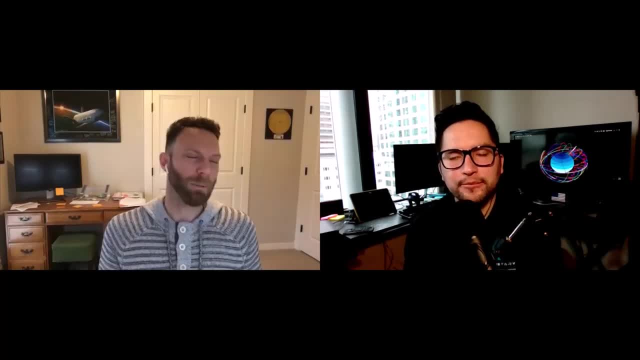 because a quaternion is like normalized to one and they have all of these weird mathematical rules but essentially the underlying concept of a quaternion as it relates to rotations is that it's an angle and an axis and then some math is done to package it into the quaternion form 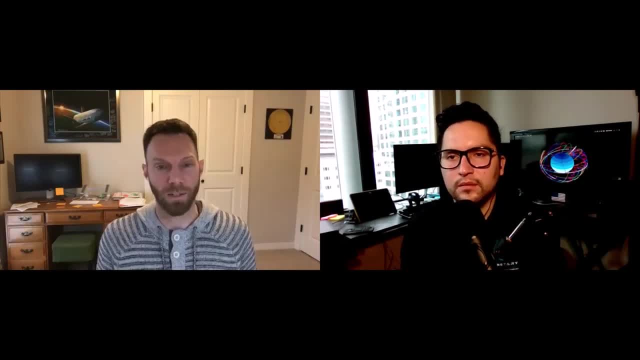 so that whatever it is like i squared equals j squared equals k squared equals i times j times k equals negative one or 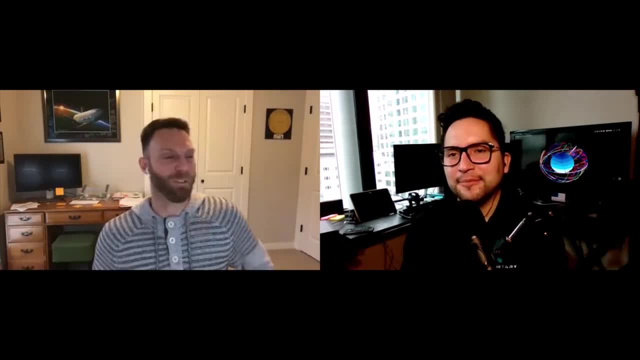 whatever whatever uh you know that that is that i can't remember off the top of my head but there's some sort of logic um to it but the other thing that that helps is that just like a an imaginary number is a two-dimensional number a quaternion is just a four-dimensional number it's just you know four dimensions and each dimension represents 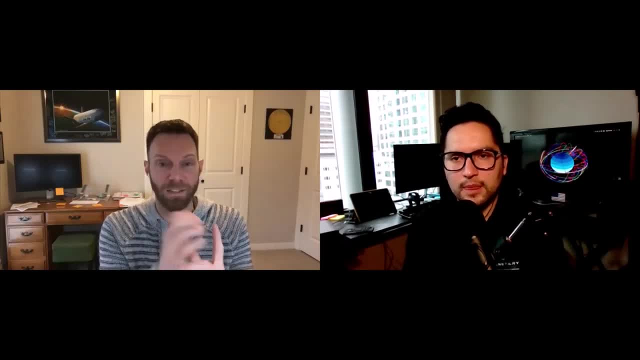 something akin to an x-axis a y-axis and a z-axis 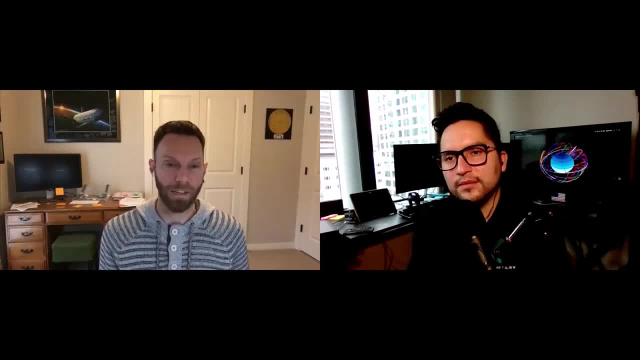 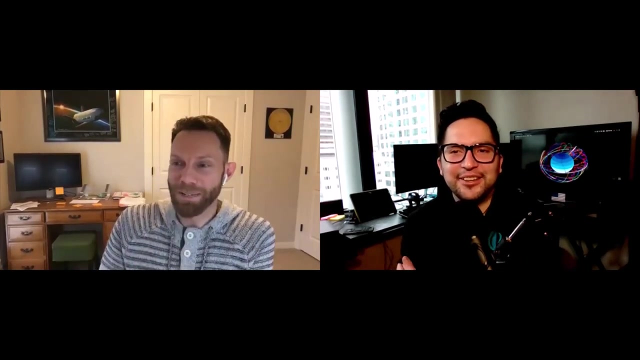 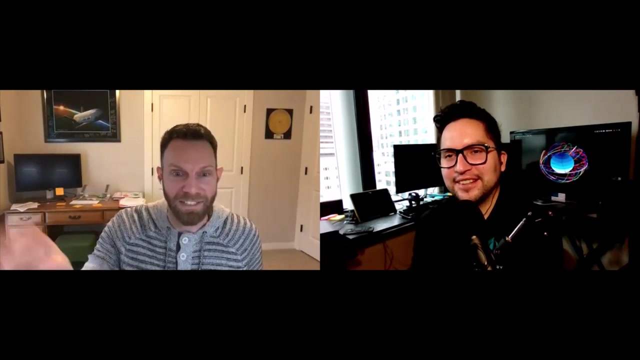 component and an angle a scalar value around that axis okay yeah yeah that makes more sense because when you do a principal axis and rotation those are four values like you just said so it's kind of similar in a way to the quaternions um and and if you do a principal axis rotation it makes sense in quaternion world too so this is um let's say this is one zero zero zero and i don't know if this is the y-axis so if i rotate whatever 90 degrees then it becomes zero zero one zero like that one is in the y-axis point i did i did a max rotation in one direction in the y-axis um that that didn't help at all i'm realizing but um if you start using them enough you can kind of i i'm not there yet i mean some people can look at quaternions and i feel like you know they just they just see it 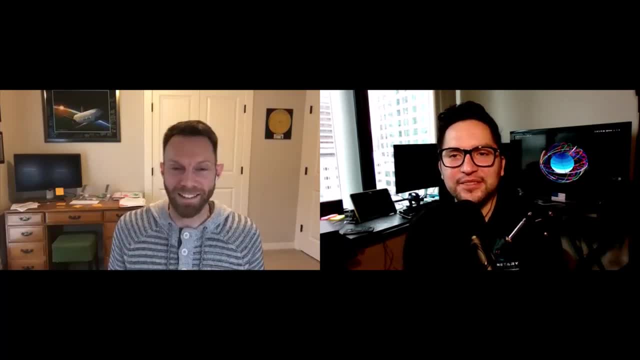 um you know certain rotations i can look at and be like oh okay i kind of get it uh but but they are useful and i guess that's why we use them 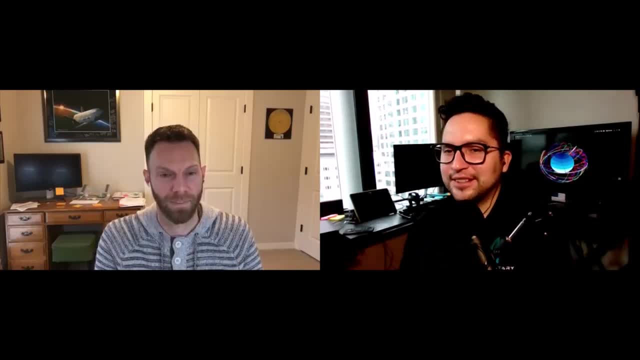 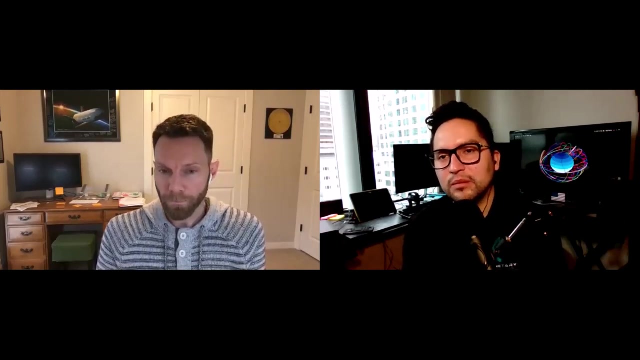 so then i also want to get into simulation and specifically soft sim so i guess can you give a first of all can you give a brief explanation of what soft sim was at planetary resources yeah so spacecraft are are difficult actually most engineering projects are difficult in the sense that if you want to test them in the physical 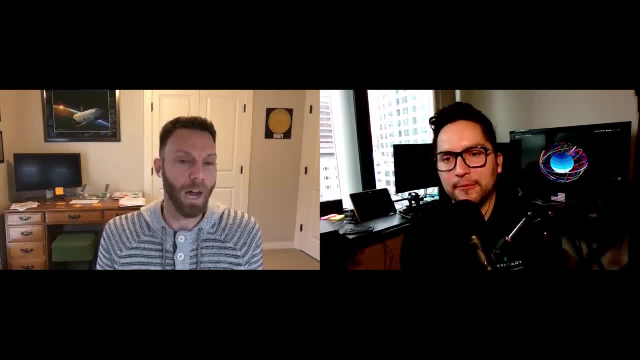 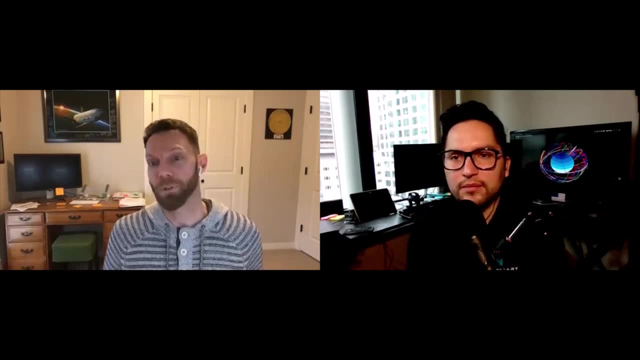 world it is expensive and possibly impossible right if you want to test a car in the snow you're going to have to go somewhere where there's snow and hope there's the right snow and all of 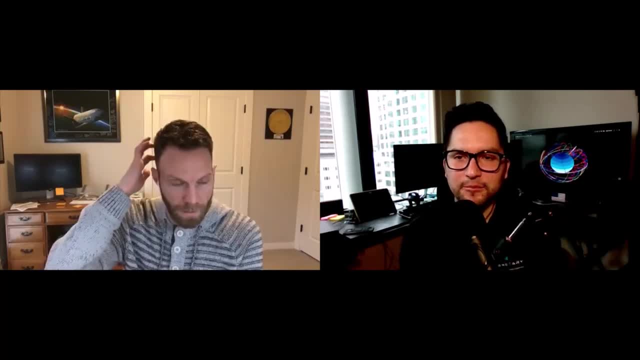 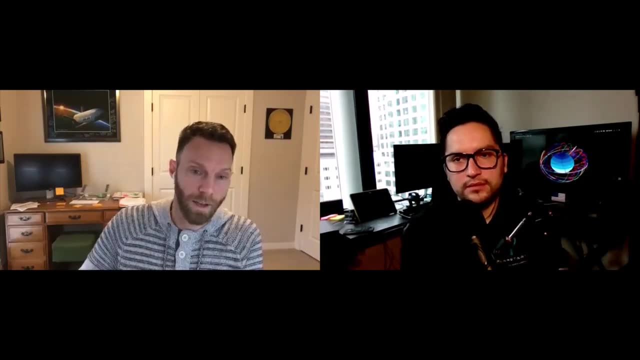 that kind of stuff uh and and physical testing is is absolutely critical and necessary but a lot of testing is done in a simulated environment and especially when that physical environment is 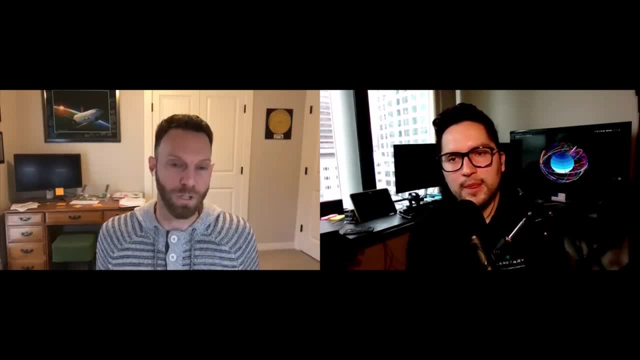 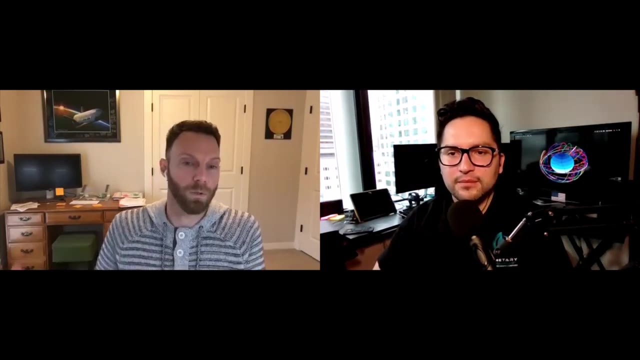 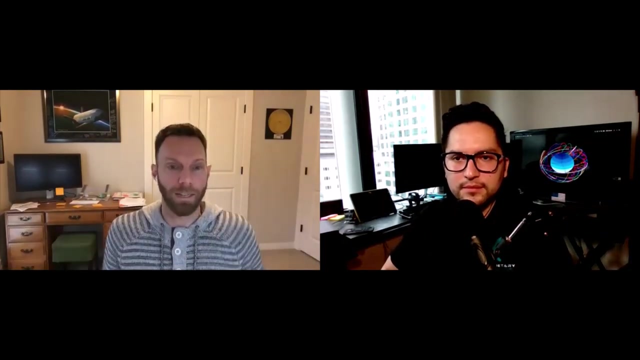 is impossible to get to like zero g or microgravity of space you know low low friction and all of that stuff so we built simulators like every you know everybody does um that that simulate the physical world that we can test our adcs system within soft sim was a larger simulating simulation 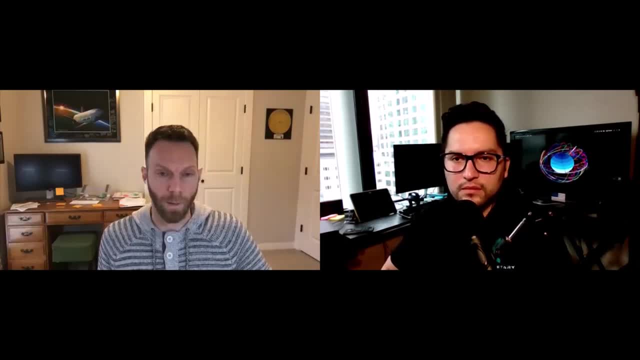 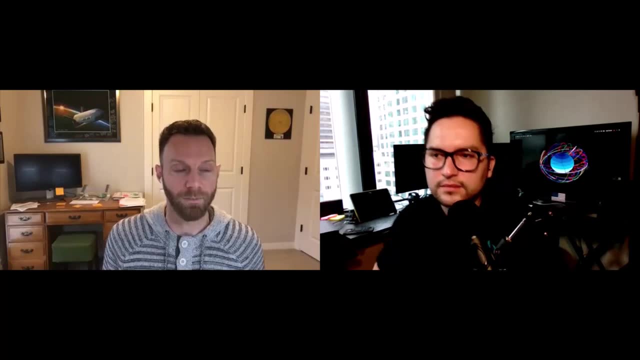 environment that allowed not just the adcs system to operate but also the rest of flight software like the actual flight software to to operate in this simulated environment um and it had things like uh antenna pattern models and solar generation 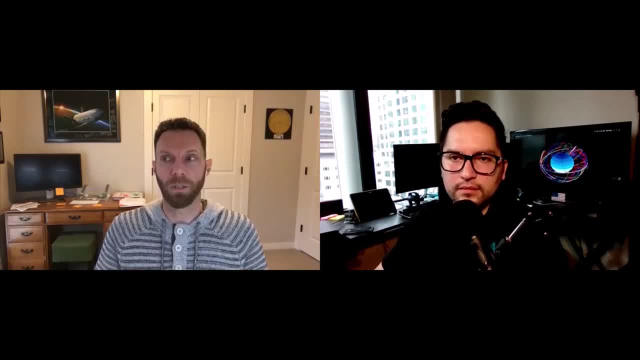 models and all sorts of things so we can we could build up these simulations running the actual flight software and determine how well the flight software does and how much power it's going to generate and we can switch between spacecraft modes and do all of that stuff like a day in the 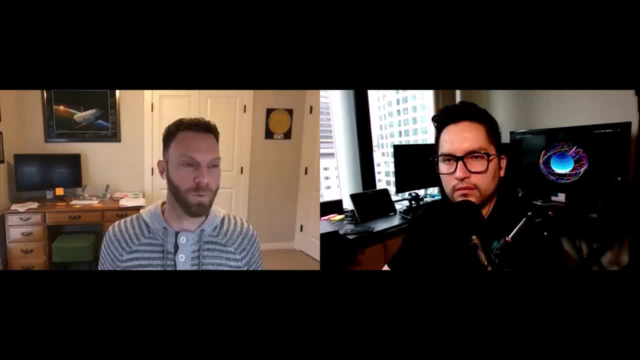 style testing so kind of in a nutshell that's what soft sim was soft sim was this way to to uh programmatically determine which elements we want in our simulation and then run a simulation 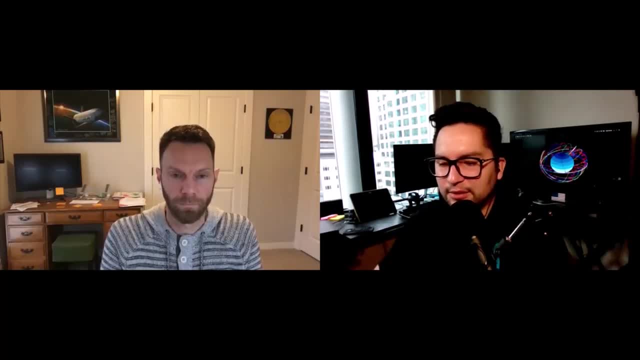 with flight software in the loop so then with the software in the loop part of it can we go into kind of the hardware in a loop as well because we talked about this last time but if you could 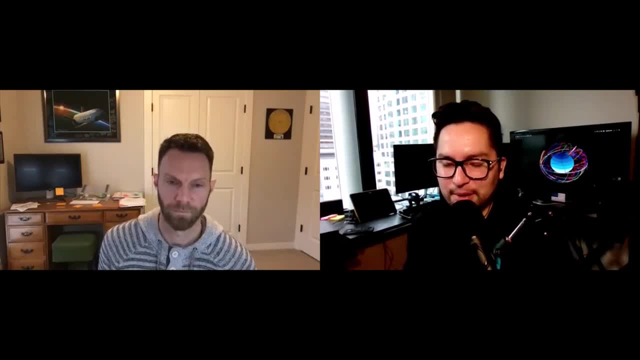 go over this again kind of the spectrum of what hardware in the loop simulation 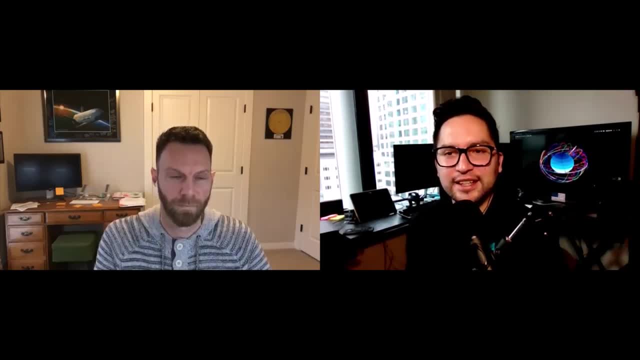 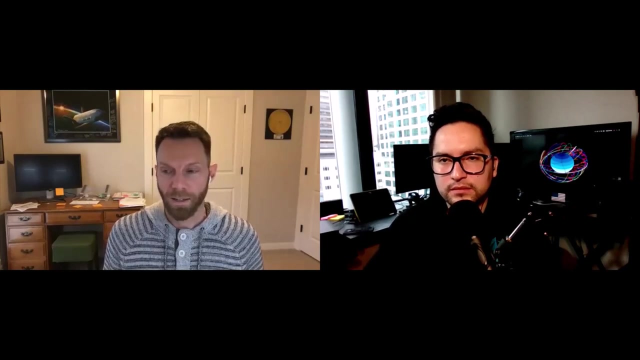 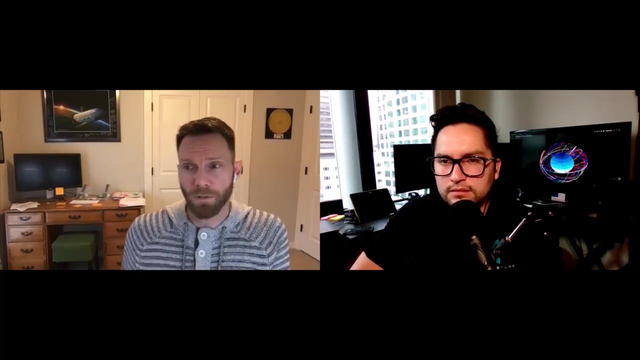 is and then how it is useful sure so i think i said this last time also but there's a quote that i like and i don't i don't remember who said it but but the best simulator in the universe is the universe itself uh so you you know and there's also this other saying that that people like to throw around which is like all models are wrong but some are useful and a model is just a representation of reality which is all you know a simulation is is that you've got a bunch of models of reality and they're just imperfect representations and so you can easily convince yourself that your system is working if all you're doing is is running it in a simulated environment and this environment is uh you know is um is not quite matching reality and so you say oh everything is working perfect in my simulation but then you go and put it on 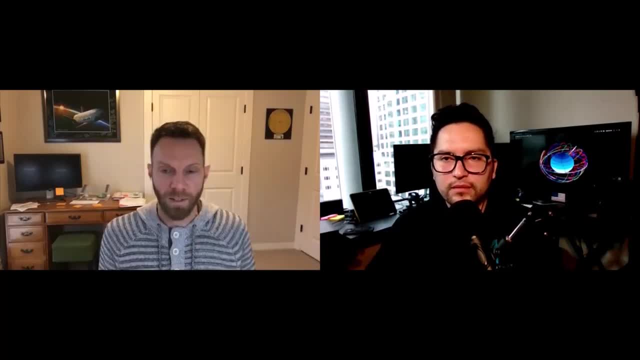 the target hardware and you go fly it in the actual environment nothing works um so so because of that hardware testing 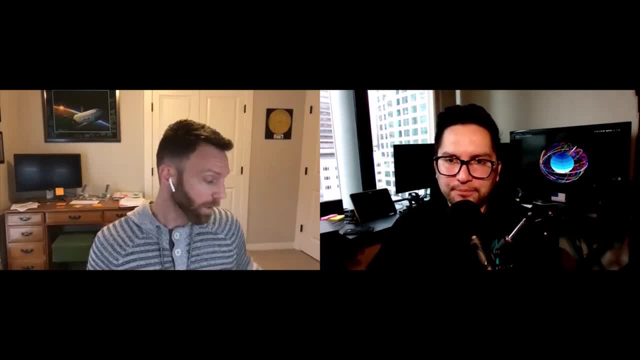 is critical right and we do a lot of hardware testing like thermal vacuum testing where we test 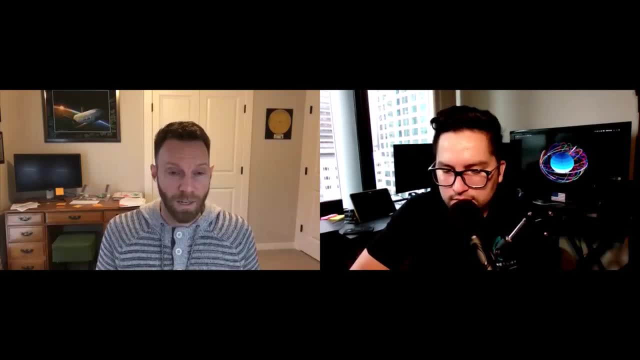 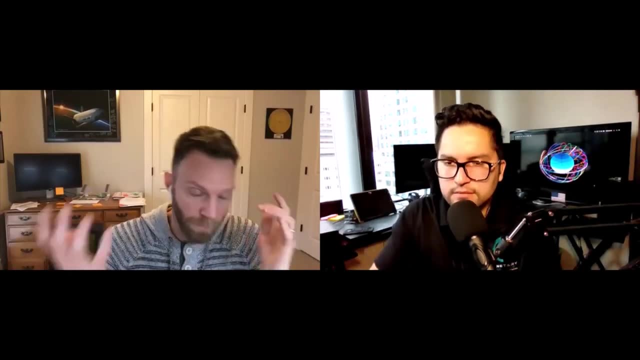 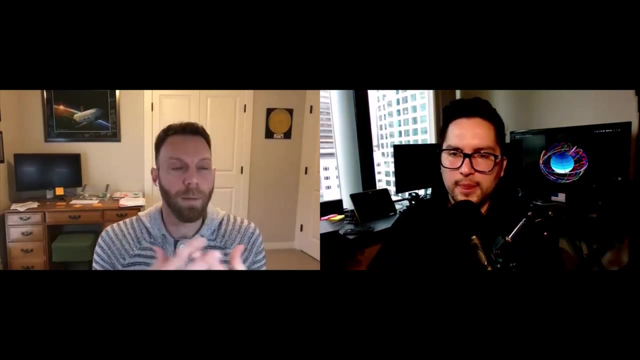 the entire spacecraft in a in a thermal environment and in a vacuum to make sure that you know heat transfer all that stuff is working properly but there's things in between those two of like a purely simulated environment and a purely physical environment is that you'd like to combine those 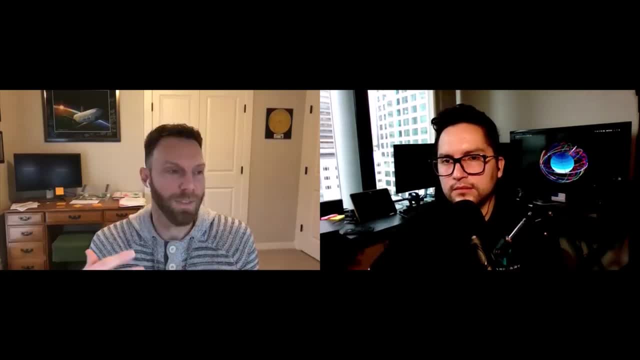 two in some way and there's like a spectrum of what that looks like you could have the full-up spacecraft 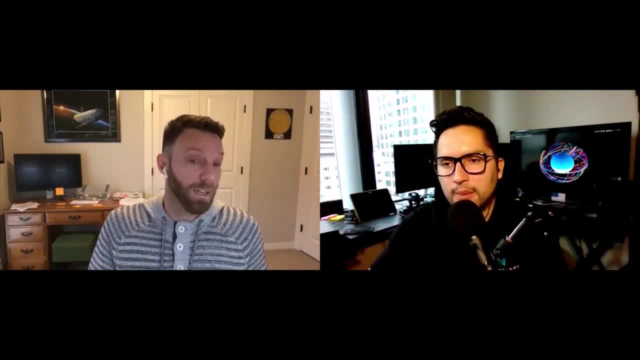 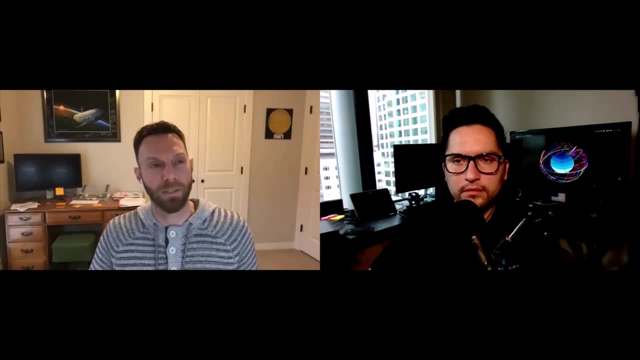 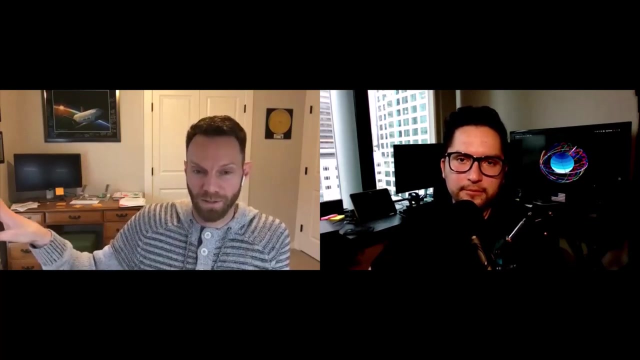 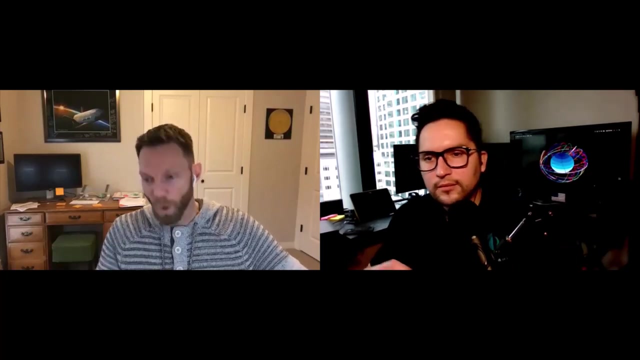 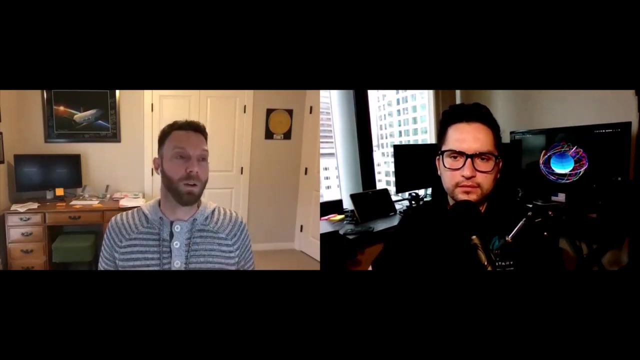 you know sitting on a table thinking it's in space but interacting with a simulation of the environment so what happens then is is you know the imu is measuring earth rate because it's just sitting on a table but you you you uh cancel out that message and you say no no no don't trust the real imu i have a simulation of an imu here and my imu says that you're flying around the earth and so you're rotating at a distance and you're not flying around the earth and so you're rotating at a different rate so let me insert that different message into that uh into into that that pack you know override the imu and now the spacecraft sitting on the table thinks it's rotating and so because it thinks it's rotating it says oh i need to move my reaction wheels so then the reaction wheels on the table start spinning up and uh your simulation uh you know intercepts those reaction wheel commands and says oh they're spinning up the reaction wheels start adding torque and 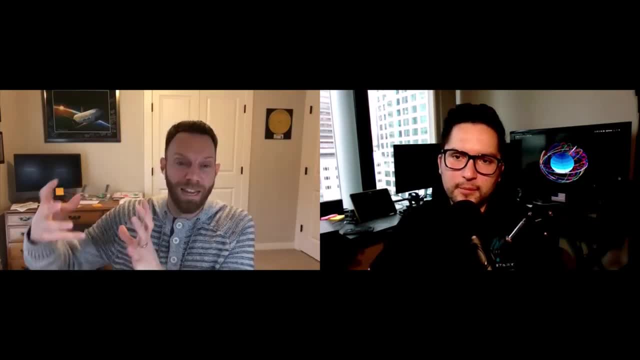 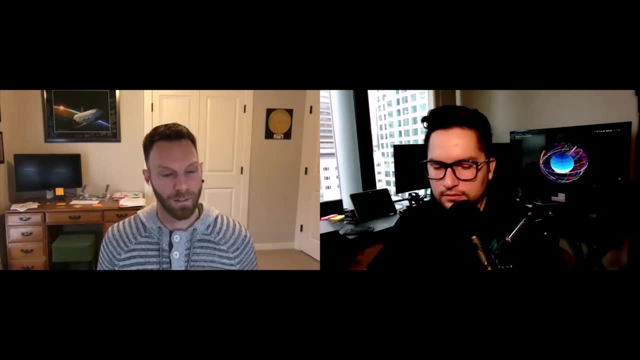 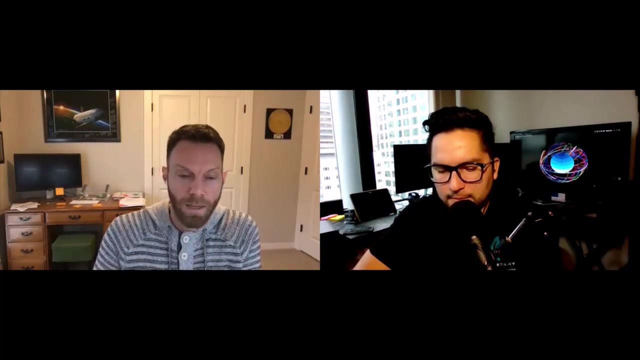 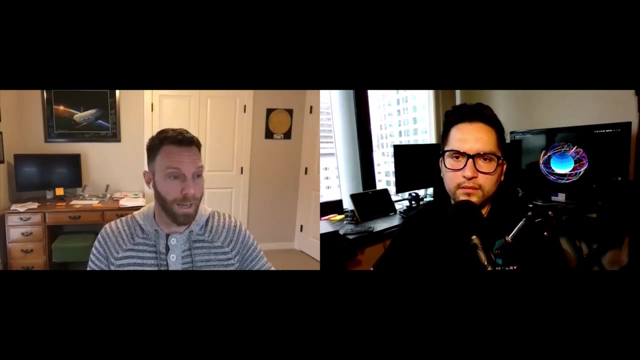 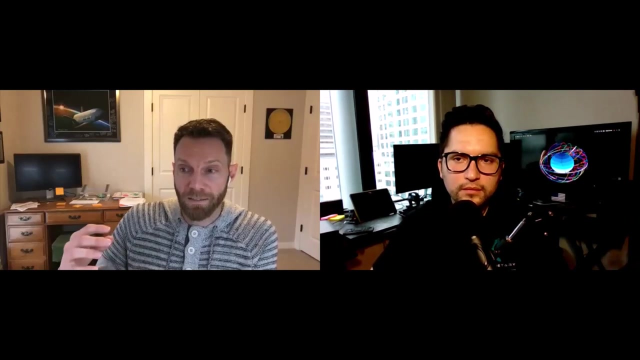 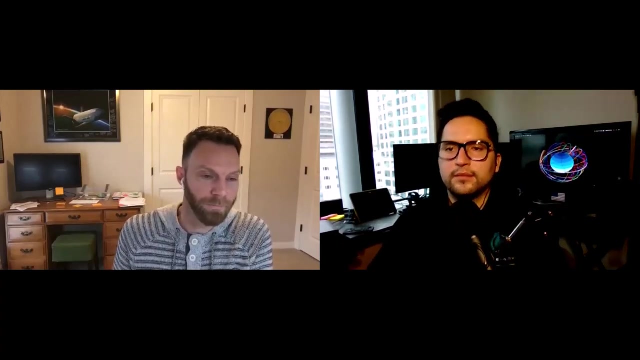 my system in the model and start rotating the spacecraft as though the reaction wheels are really affecting it which then affect the sensors which then go back into the uh you know the satellite sitting on the table so in that way you get sort of the the best of both worlds in that you have control over the environment and you can inject faults and you can put it in situations that are difficult to test but you have the actual flight software running on the actual hardware interacting with the actual battery potentially um sending commands to the reaction wheel and the other devices and you can see all of that you can see the reaction wheel spin up and you know all of that kind of stuff um it's it's a good it's a good not compromise it's just it's a it's a good set of tools that you have at your disposal to do engineering which is allow the real hardware to interact with simulation and simulated models and you can take that like i said in a spectrum you can do what i said right there which is have the full spacecraft with a simulated environment you can just simulate you know the rest of the spacecraft and flight software and everything and have it hooked up to the real reaction wheels because you want to see how the reaction wheels are going to react for example or something so so it's it's a way to combine models and simulation with the real physical hardware so that you don't have to 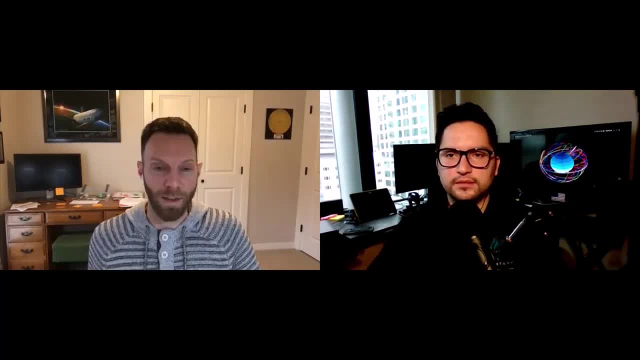 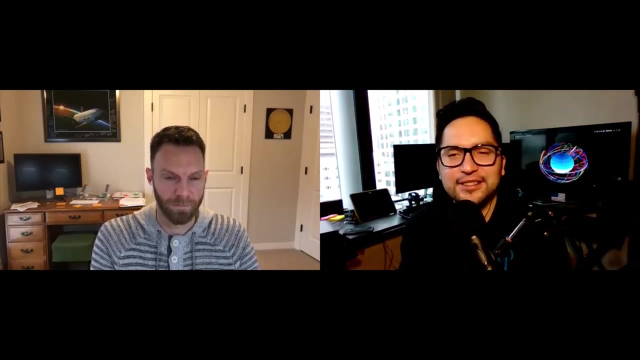 rely on a imperfect representation of that hardware you can get the actual hardware operating in in the real physical environment can you talk about because you mentioned this last time the that one big mistake that um brandon found where you had the polarity oh yeah with the control system yeah so can you talk about that kind of first of all how he found it and then yeah yeah 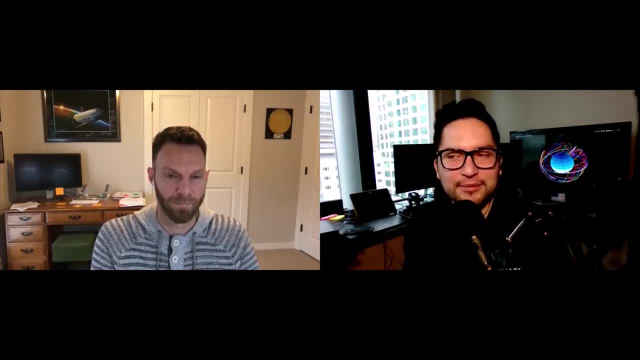 just how he found it and kind of i guess if you had maybe a lesson learned i don't know what lesson he you would have learned besides like put a negative sign maybe yeah yeah yeah that whole process 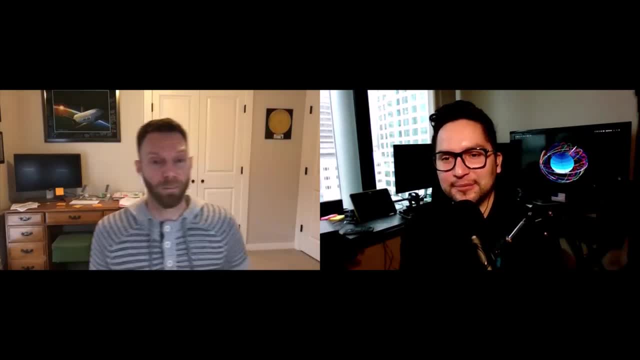 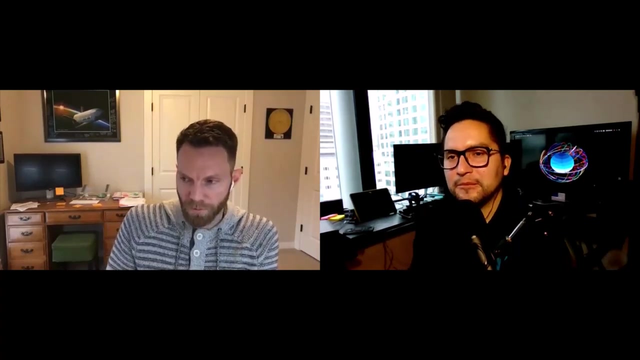 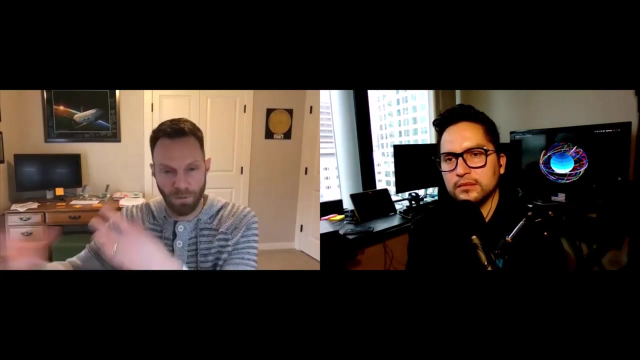 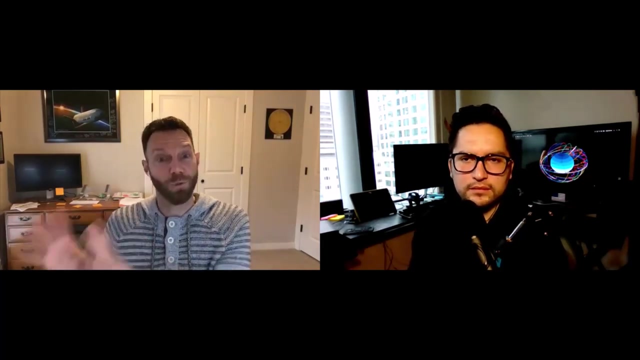 for sure so first off we're talking about brandon block um who was a member of the adcs team gnc team um at planetary resources and um all around superstar engineer by the way i'll just throw that out there now um one of the troubles with designing your flight software against a model and what i mean by that is like model-based engineering where in instead of designing your control system on the actual physical hardware and you know you're you're getting feedback right there you you build a model of your hardware you build a model of your environment you trust that 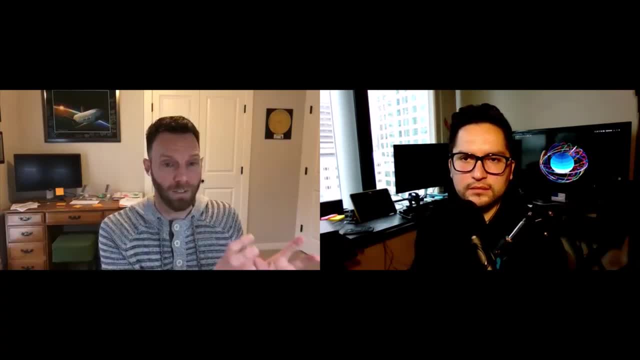 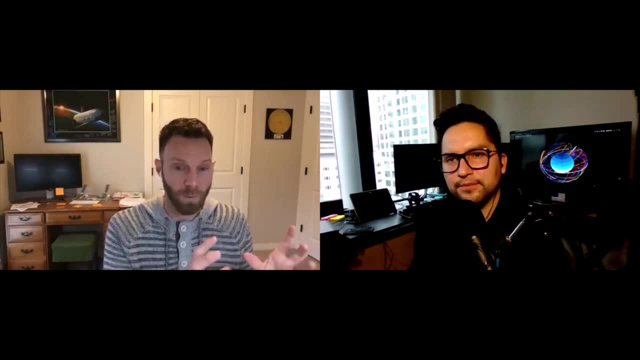 model enough to go off and design your flight software against it in our case our attitude determination and control system so we're going to design our flight software using this model of everything 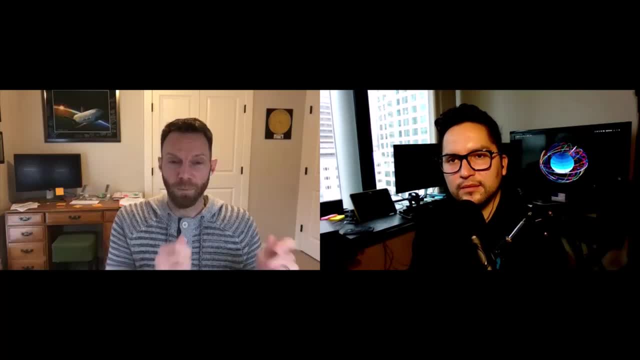 and the hope is that that model is good enough that when we take our hardware our software and we put it on the real physical hardware it's going to work 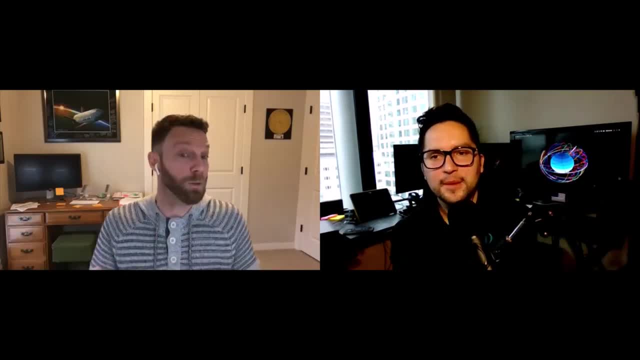 well enough and maybe we'll have to tune it a little bit but for the most part it's going to 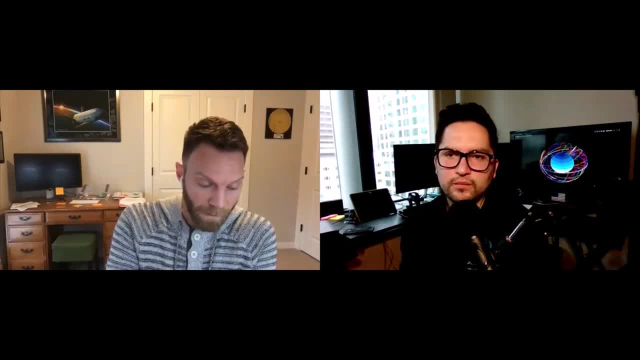 work well enough um well the the the issue came where i i uh built a magnetic model of the earth and i built a 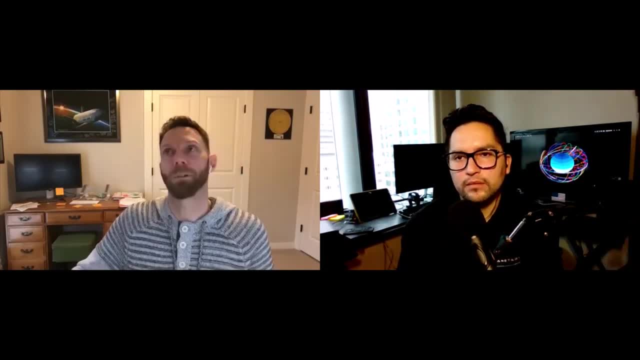 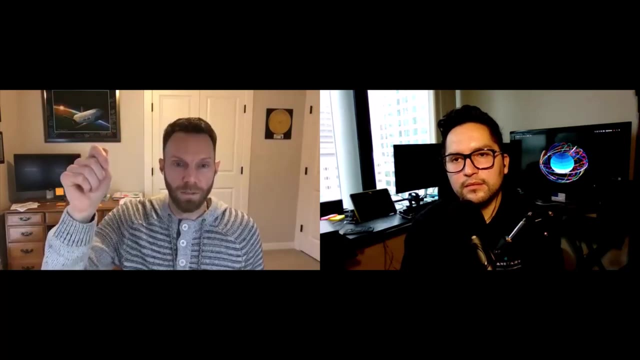 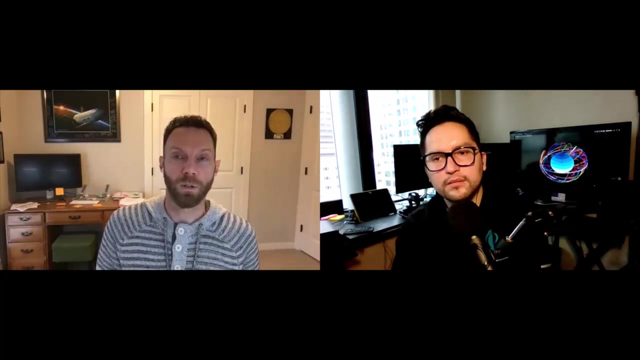 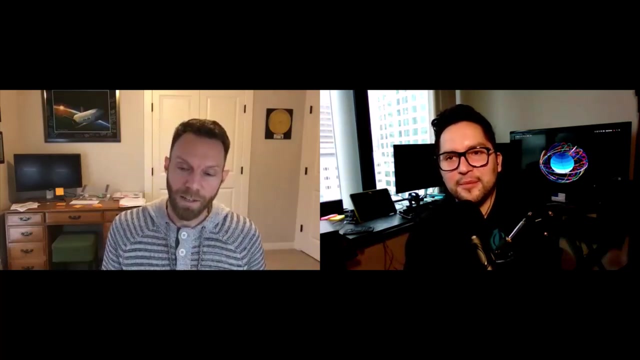 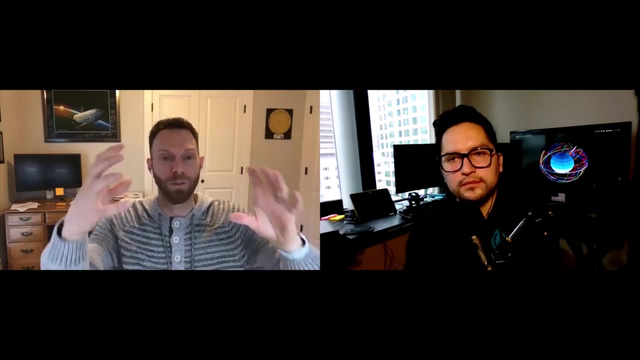 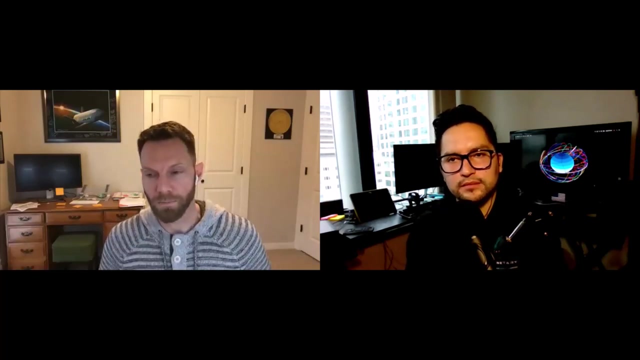 a flight soft and a magnetic uh magnetometer or i'm sorry a a torque rod model in our simulation on the flight software side i wrote a control law that would detumble the spacecraft and basically what that is is when the spacecraft is rotating you can measure the earth's magnetic field and see that the earth's magnetic field is rotating because it's relatively fixed over you know 10 seconds or so in orbit so if the earth's magnetic field is moving relative to the spacecraft you know you're the one doing the moving because the magnetic field is not moving and so because of that you can fire these torque rods at the exact right time to push against earth's magnetic field and slowly slow the spacecraft down and detumble it and basically get it fixed relative to earth's magnetic field and and it worked great it was it was quite amazing all of our simulation runs 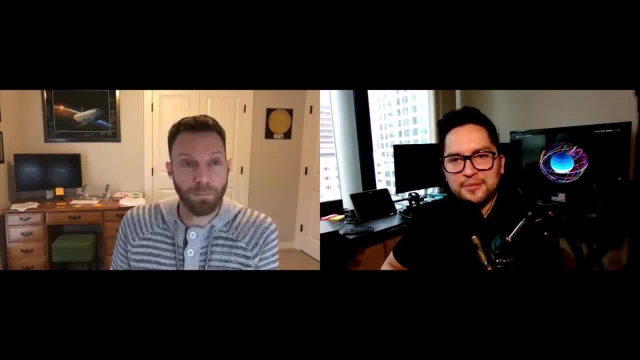 everything looked good and and the problem with this particular set of actuators is that it's extremely weak 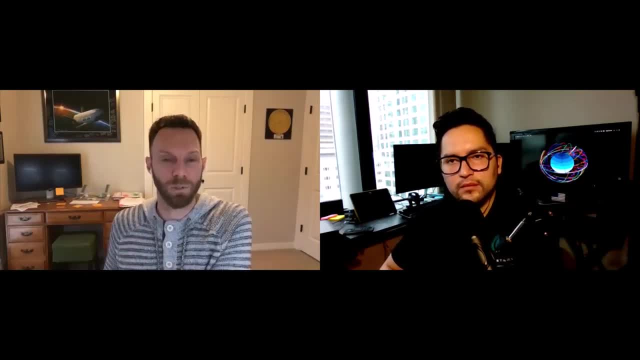 um these these torque rods produce very very very little torque not a noticeable amount of torque that we could put this thing on an air bearing table and see it move there's just no way 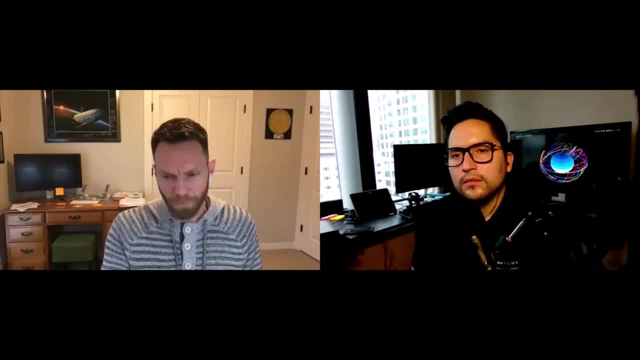 so the only way to really test it is to you know put an external magnetometer against it and say yeah it's firing in the right direction and all of that kind of stuff and i had convinced myself 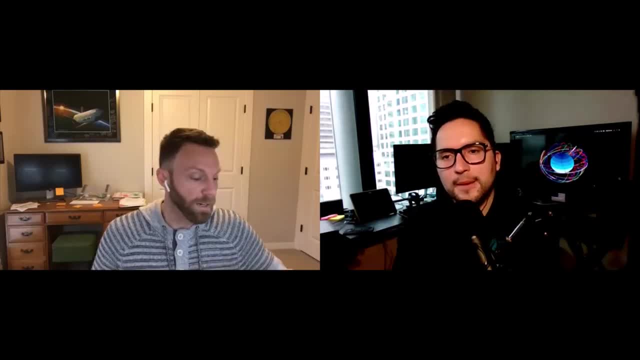 that it was all set up correctly um and in an audit and i don't remember the specifics of why i think brandon was just going through and 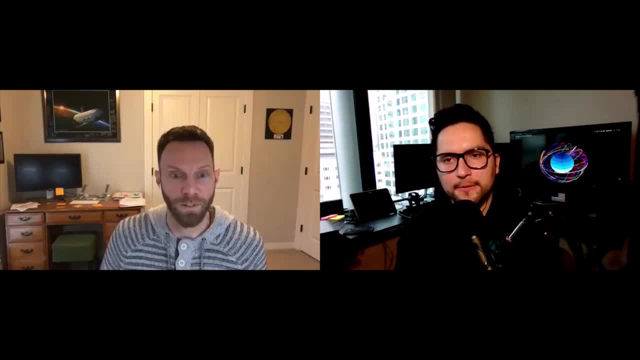 and double checking things because we were you know a couple months away from delivery uh found that there was a polarity issue or a negative sign flip on both the flight software 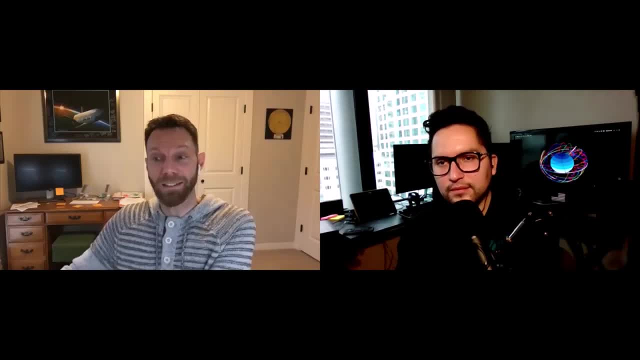 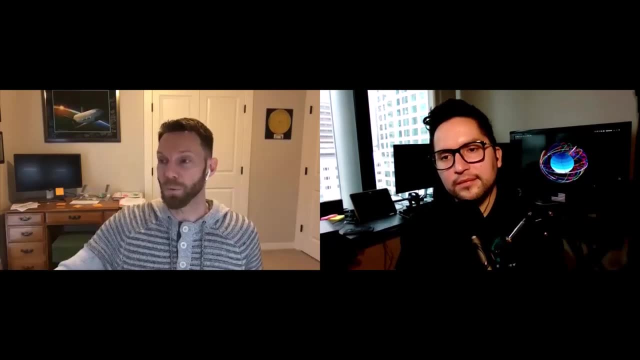 algorithm the thing the controller doing the detumble and on the simulation side and so those two negatives canceled each other out and so in the simulated world everything worked perfect and in the physical world it was still firing the torque rods but since they weren't producing enough torque to to see we couldn't take it and we couldn't take it and we couldn't take it and we 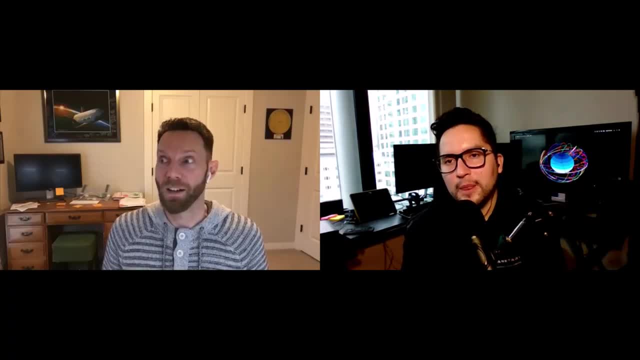 couldn't tell that they were in the wrong direction and i had uh done the calculations 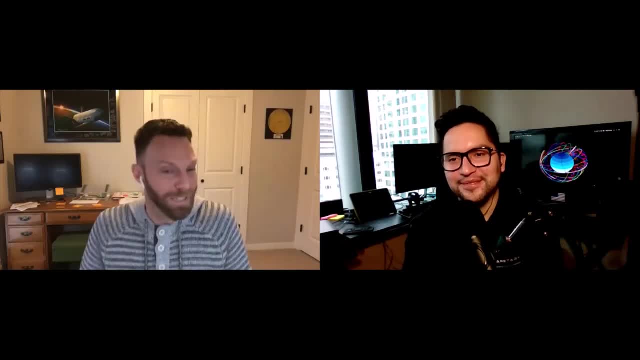 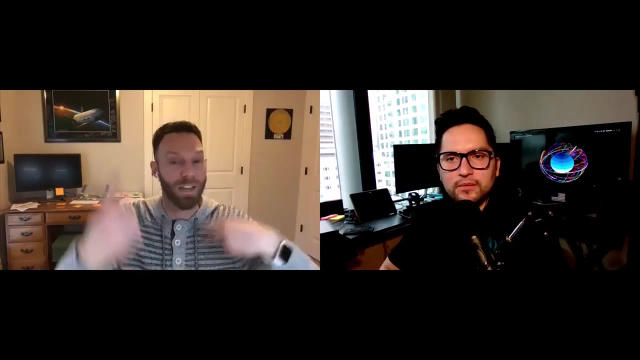 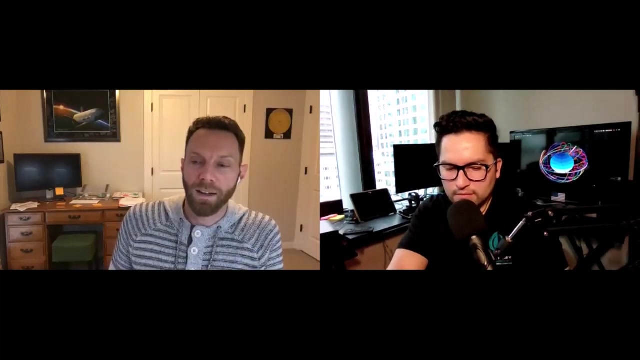 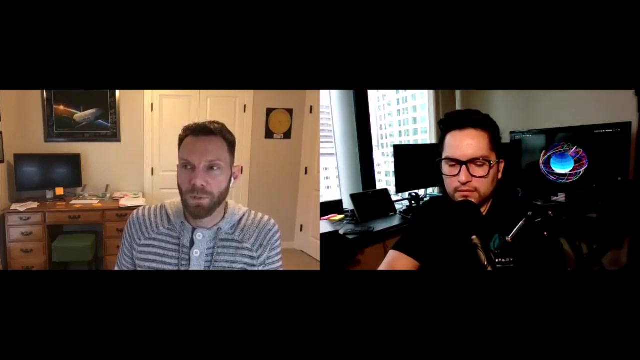 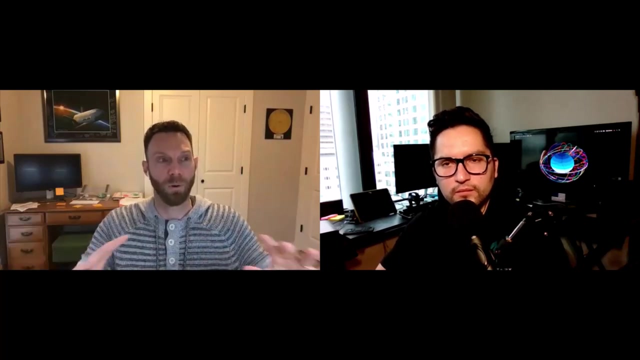 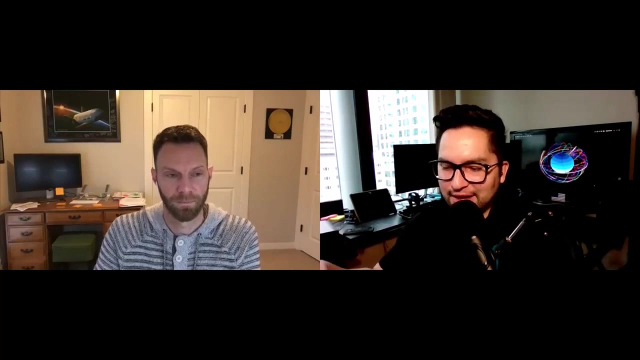 and they said it was the right direction brandon redid the calculations and said that they're not in the right direction and we had this you sit down and and you know he was right and it would have been essentially mission ending because instead of detumbling and slowing down the spacecraft it would have just been getting faster and faster and faster because it would have been pushing the wrong way against earth's magnetic field so that was a mission saving um uh find that that he found and and it you know i'll forever be grateful that he that he found that when when he did um but that's that's sort of kind of the moral that story is like it is easy to design bad flight software that looks good if you're designing it against a bad model because the two things you're going to design one to that model and so the whatever errors you have in the model you are going to incorporate and cancel out perfectly and you're going to your flight software and so it's really critical that some amount of validation and verification of the model is done against reality before you spend a lot of time building up your you know your your system using that model so one thing i remember that goes along the lines of you can't really or it's hard to model in simulation is that the as far as the avionics go there's sometimes where the magnetic field that is caused by a current can actually be used to simulate a 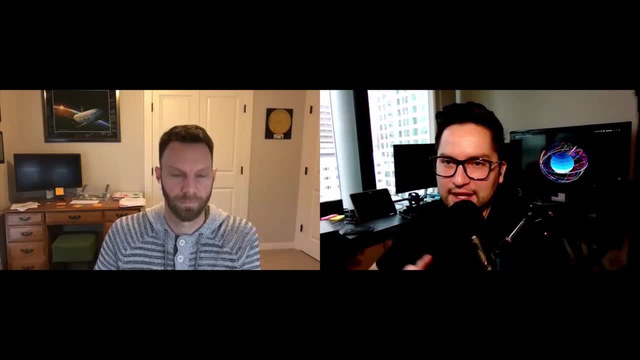 magnetic field that is caused by a current that is caused by a magnetic field that is caused by a mess with the magnetometers and what they're seeing and i think if i remember correctly 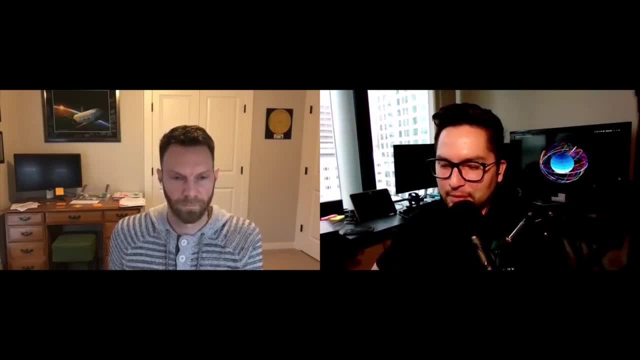 when i was there i think third summer we were taking a look at or krish was having me take a look at kind of how when the spacecraft heaters were on um so that current because there's a lot of current that they was messing with the magnetometers and then was then messing with 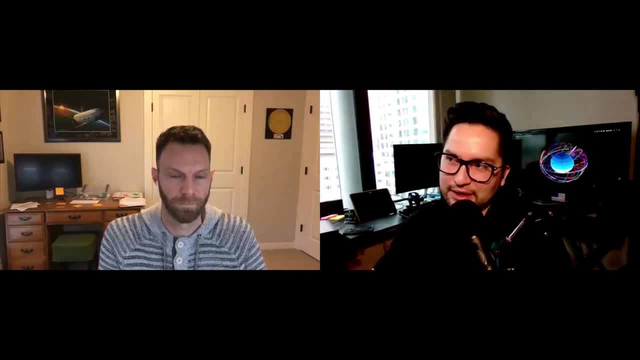 the attitude determination system i don't know if i remember that correctly but i think this goes into flat three so i'm going to go back to that and i'm going to go back to the first one 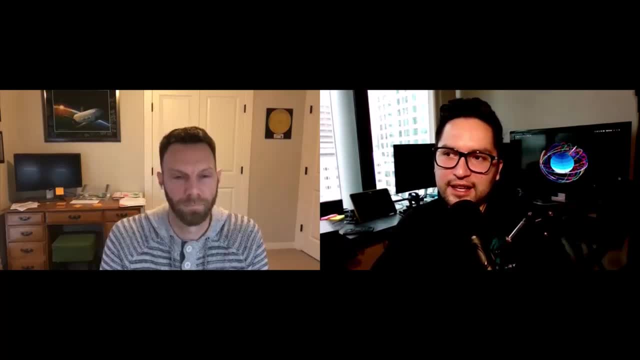 and kind of what a flat set could do is that the kind of mistakes that you would want to catch or you could catch from a flat sap simulation or i'm not sure what the question is there but i 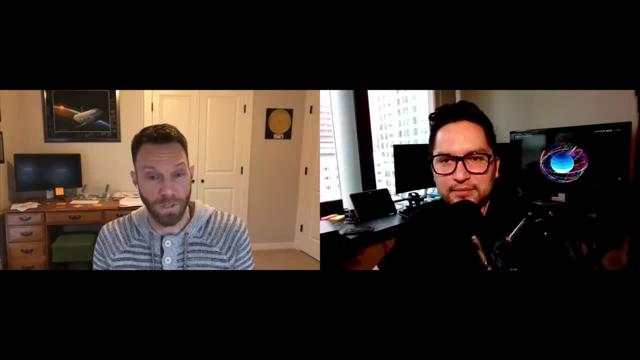 okay well first off you you mentioned krish this is krish casey also a member of the adcs team also superstar engineer um one of the things i lucked into at pri was that uh the team was amazing um and and uh 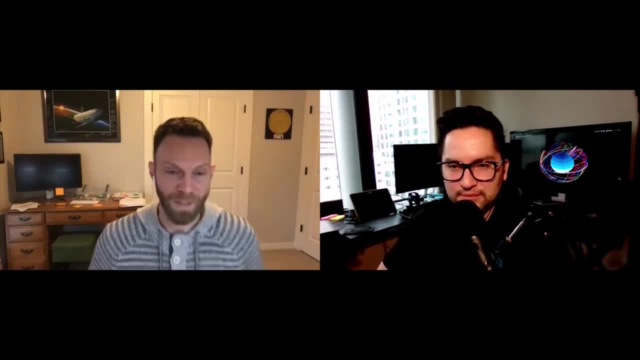 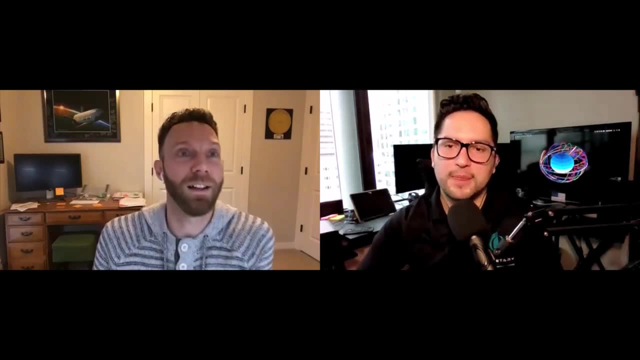 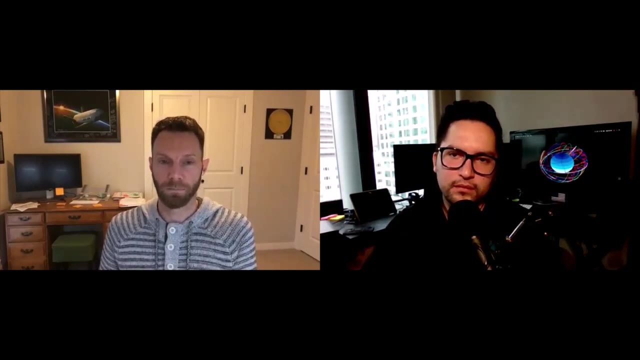 that was mostly done before i even got there so that's why i said lucked into it but yeah so um well let's imagine this um a magnet a magnetometer is not measuring earth's magnetic field it is measuring a magnetic field and coils of wire generate magnetic fields 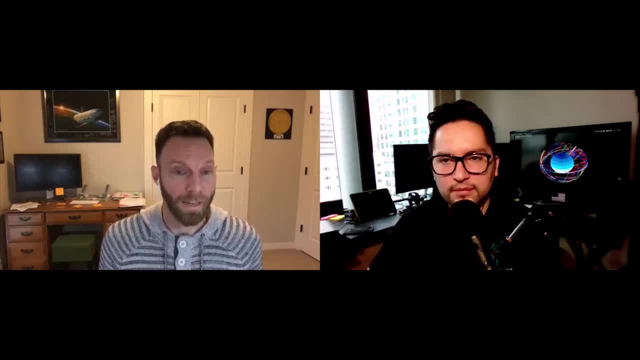 when current runs through them and some 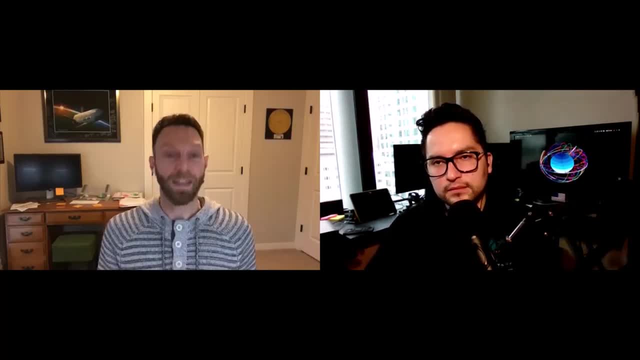 metallic structures bend magnetic fields when they trans when they when they pass through them 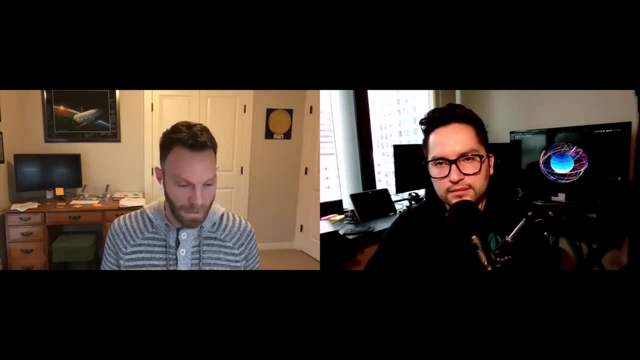 they change the direction of them um in in some way and permanent magnets like those in motors like those in reaction wheels have their own magnetic field and so now you've got 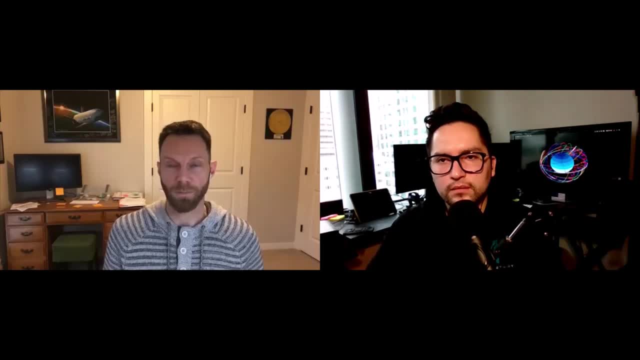 moving magnets on a spacecraft in terms of reaction wheels you've got coils 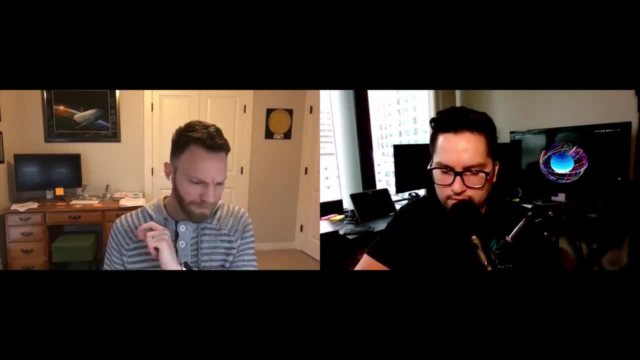 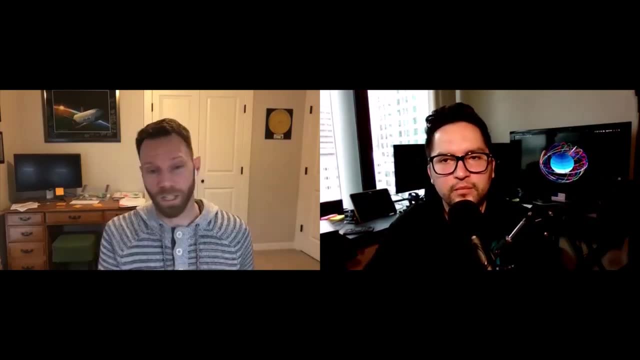 that are that are driving high currents through them and those are dynamic so like when the solar panels are charging a lot of current's going to be going through that sort of power bus 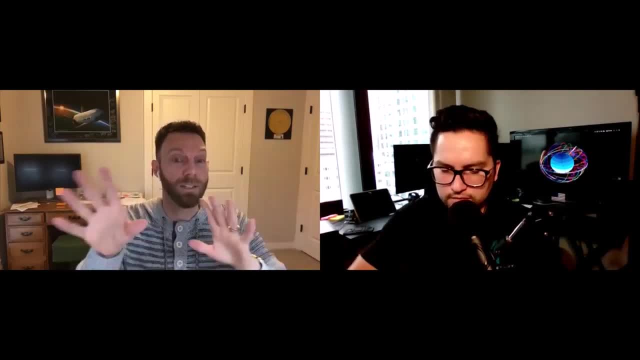 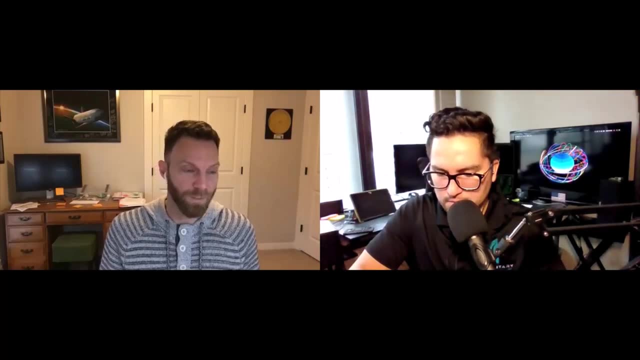 to to the battery and that's going to generate some kind of magnetic field and then when that stops it's going to go away um and then you've got metallic uh um ferrous 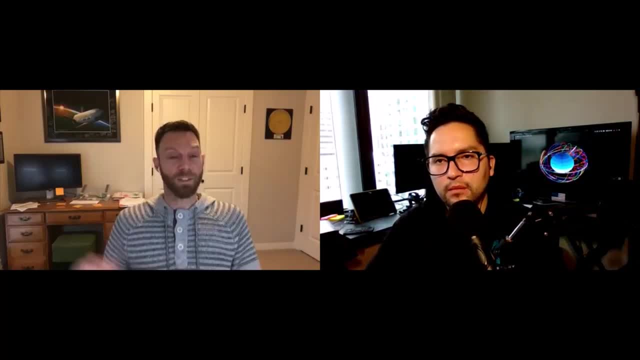 structure on the spacecraft that's going to bend the direction of earth's magnetic field so all of that is working against you because that's what you're actually measuring when you're 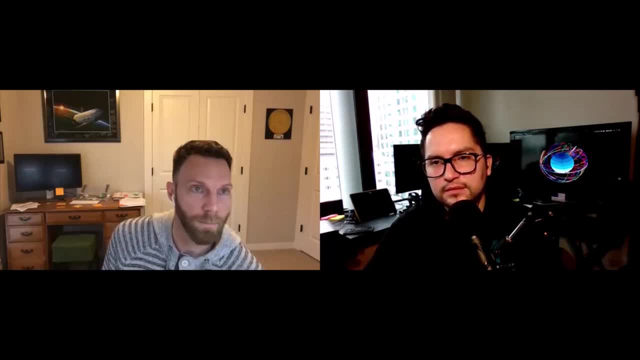 measuring something with a magnetometer uh and and that is something that is very difficult to predict ahead of time like maybe if you had a really amazing model of your spacecraft and all of the electromagnetic fields and forces and everything like that you could predict it ahead 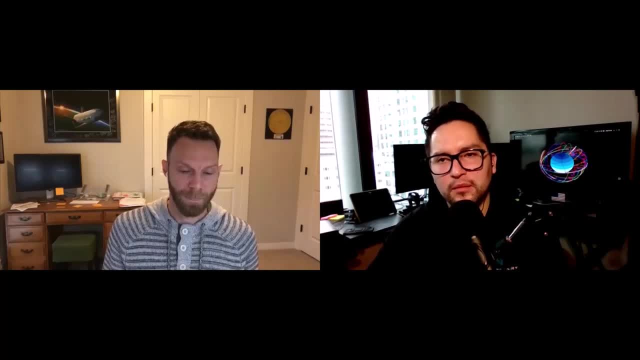 of time but but for the most part um i'm not sure of anybody that does it that way what we did is we 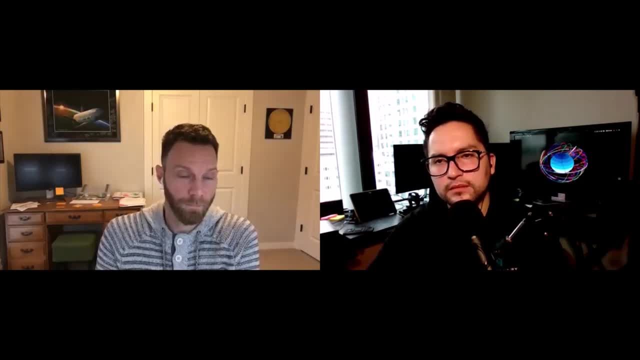 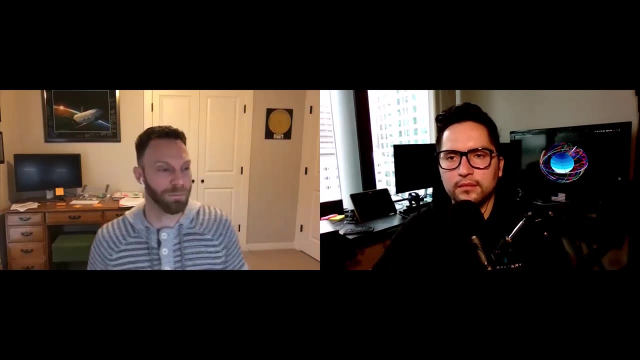 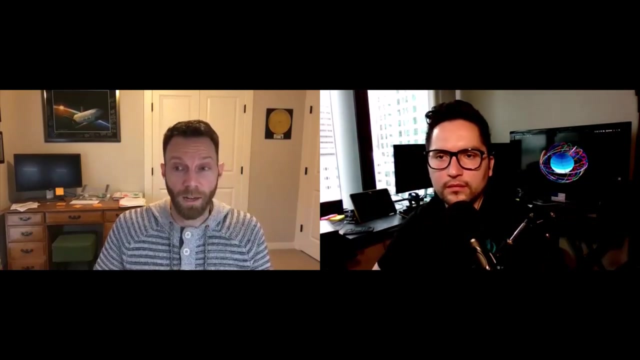 characterized the vehicle after the fact and we uh we set ourselves up with some requirements and said we need to know the magnetic field of earth to within some value plus or minus you know some statistical you know deviation so some sigma value and um and and then that set a requirement on how well we had to calibrate our system so it became a calibration issue after the fact 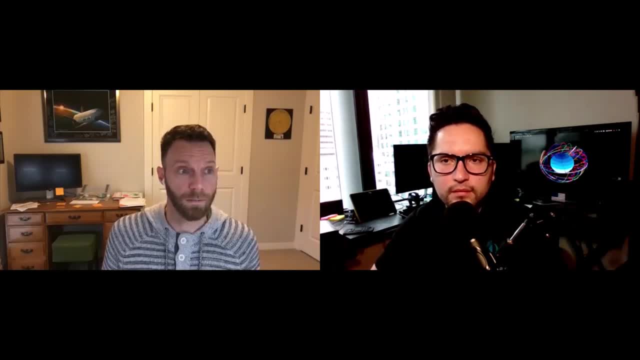 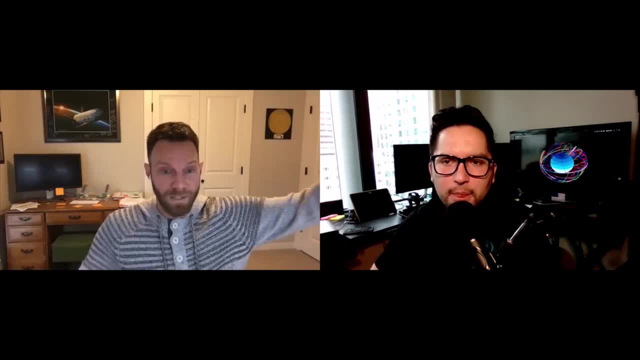 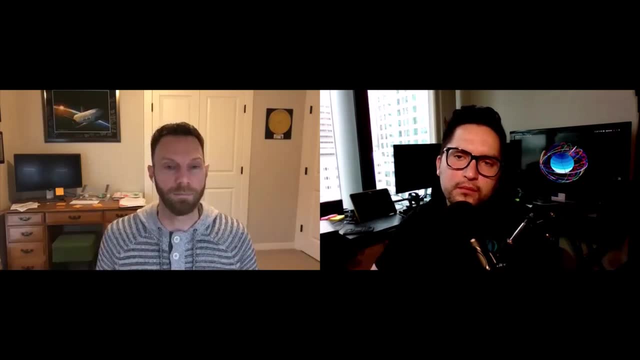 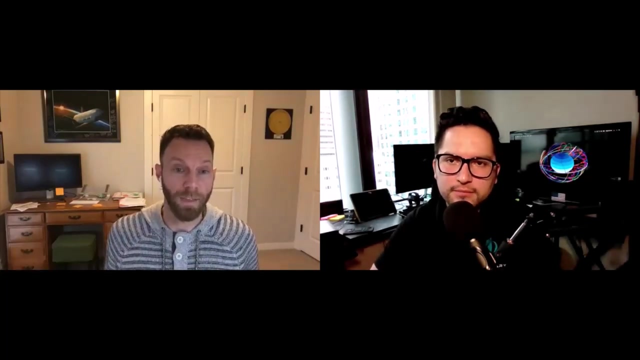 just take your space your spacecraft in a fixed uh magnetic field so either the earth's magnetic field if you trust that the building you're in is not affecting that or in some sort of like hemmholtz coil where you have control over the magnetic field you take it and then you rotate it in all four pi steradian directions and um you can build this calibration matrix from that that takes care of all of that stuff so we did that for sure the problem is some of those sort of things that we did that we did that for sure the problem is some of those sort of 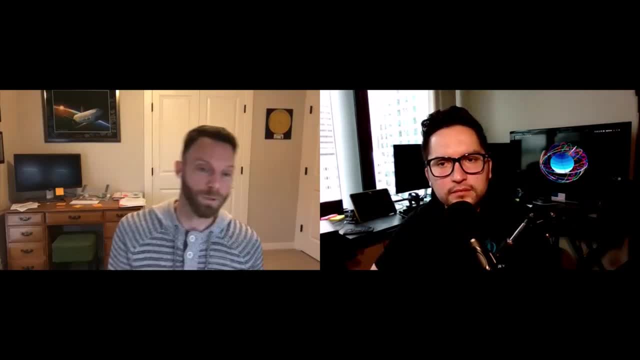 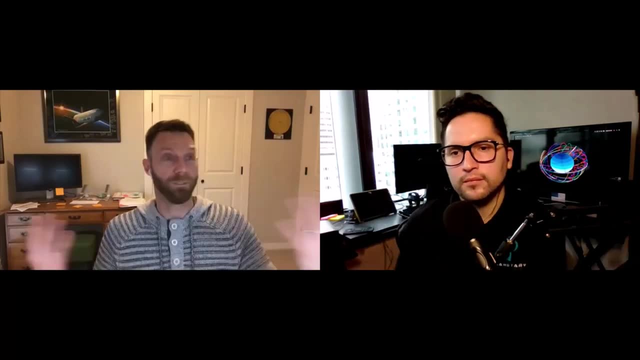 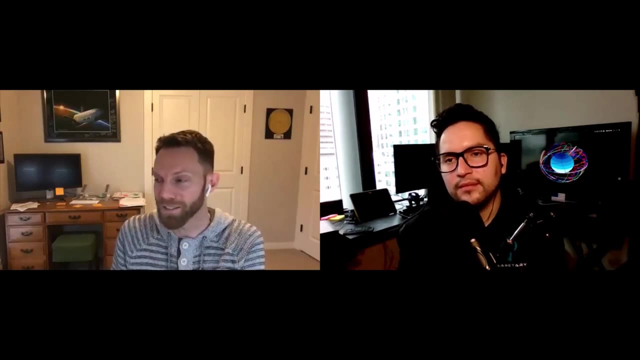 sources are dynamic right they're not static sometimes you're charging sometimes you're not charging sometimes you've got some high power compute element on that pulling a lot of current and for whatever reason the path that that current takes does some kind of a loop you know it's not like a straight shot somehow um so the other way to do that is to schedule different calibration coefficients based on the mode of the spacecraft so we would do that four pi steradian thing with the spacecraft completely off and then we did that again when it was on and then we did that again when it was charging and if if they varied greatly between any of those modes we had 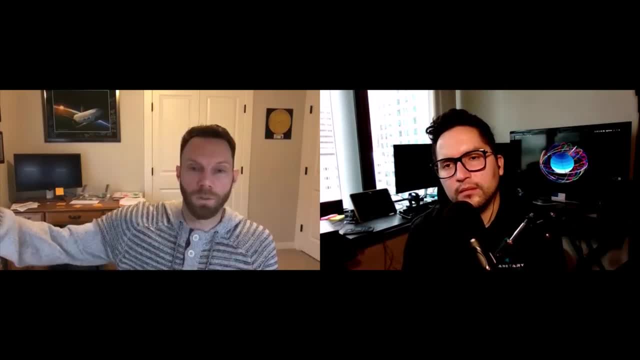 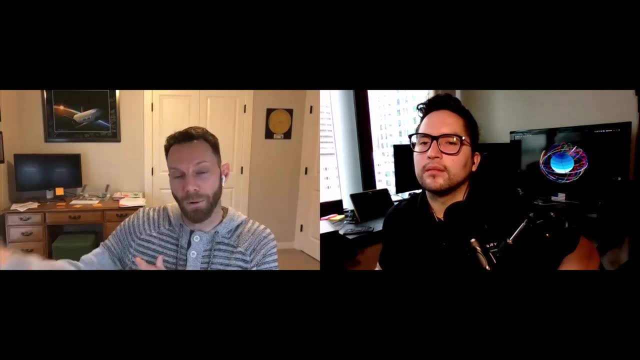 to schedule a switch so whenever the spacecraft would go into a different state like a charging state we could switch to a different calibration set for the magnetometers so that we could take out that particular interference magnetic interference could you real quick explain 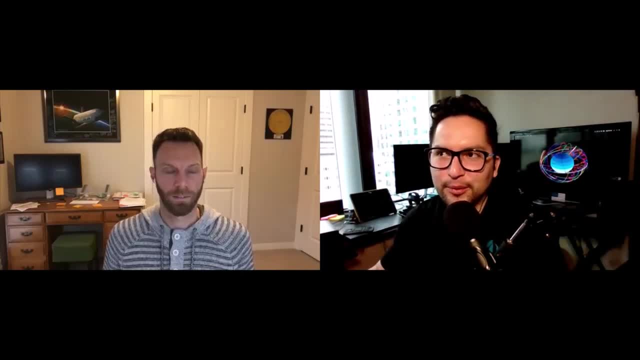 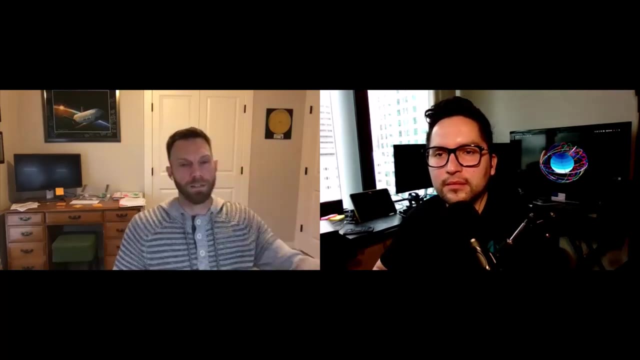 the steradian because i think that was a term that i never heard before before planetary that it's kind of like an angle in 3d if i remember correctly yeah it's a two-dimensional angle so like a radian is a one-dimensional thing it's like an angle and and and a steradian is uh i'm gonna get this wrong because i just used the term i haven't really defined it but it's it's 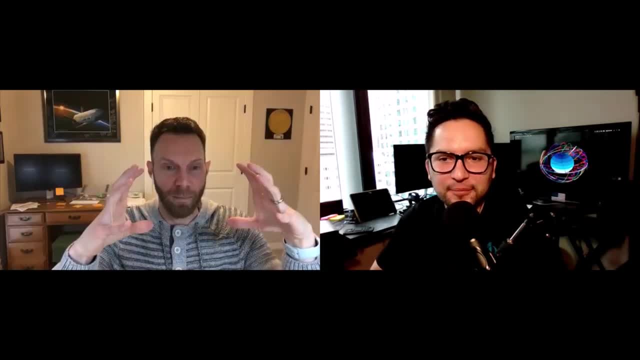 essentially like an area of a sphere um so instead of a circumference of a sphere it's the area of 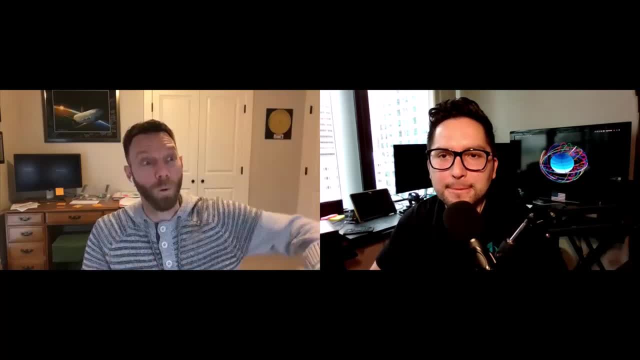 a spherical shell and so you want to say like four four pi steradian is the entire spherical shell like all in all directions 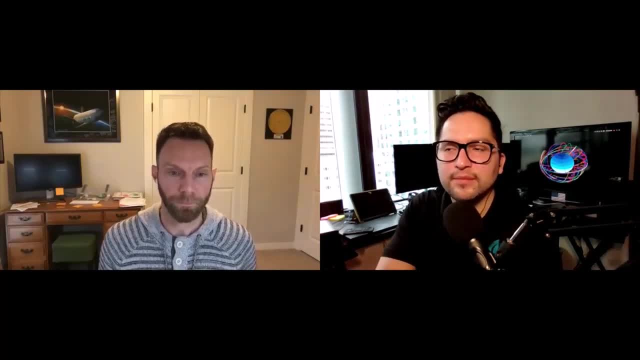 that's the area of of a of a sphere yeah that's kind of what i remember and um so one thing going 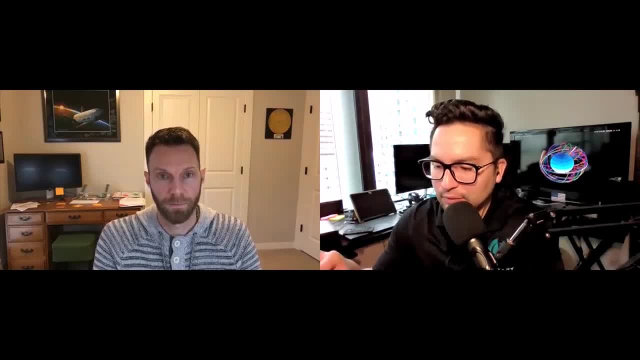 back to controls i was wondering if because you can implement and design a really complex and a 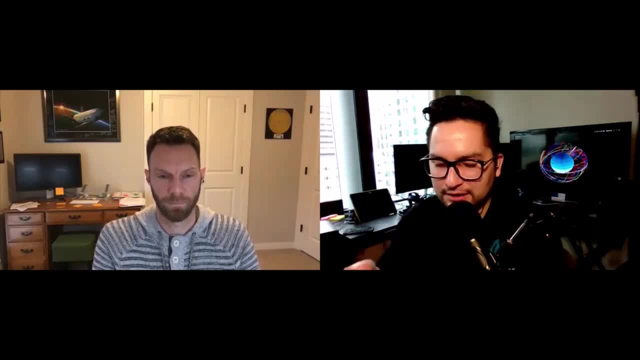 really good control law on the ground but going back to the flight computers is that sometimes you're limited on compute power so if you're limited on compute power you're limited on compute power 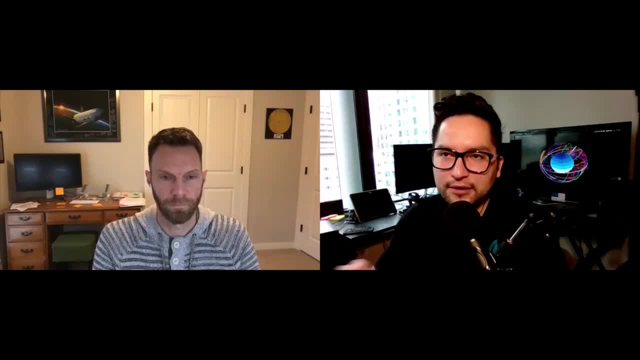 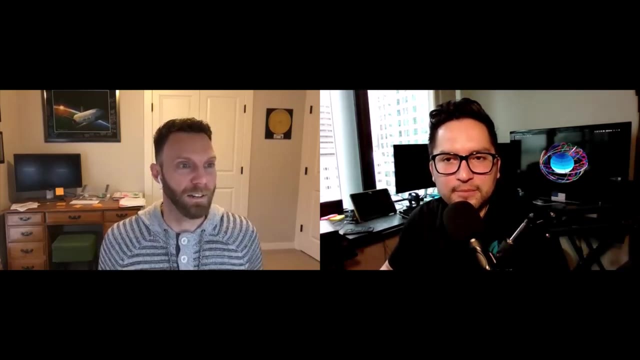 so are there cases and or trades where you kind of have to use a simpler control law say for the adcs than you would like to say on the ground because you have more compute power oh i mean sure i mean it it's it's the uh it's like the statement how much how much data do you 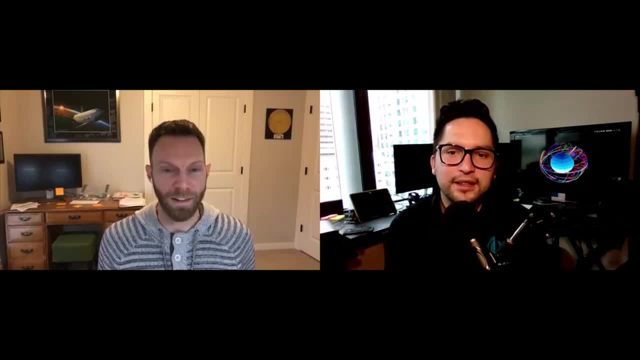 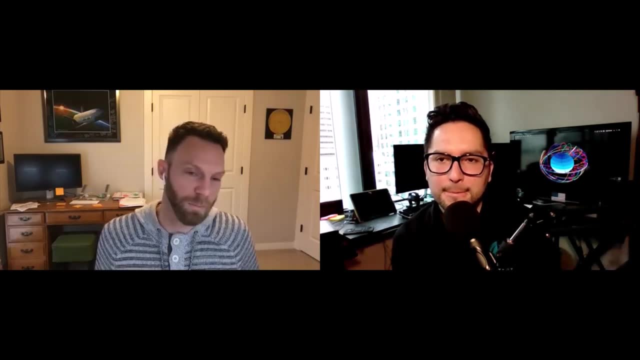 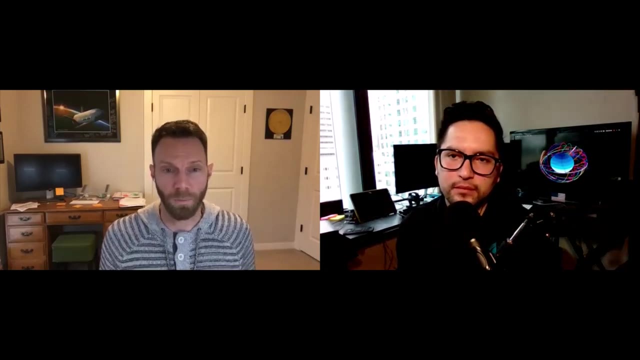 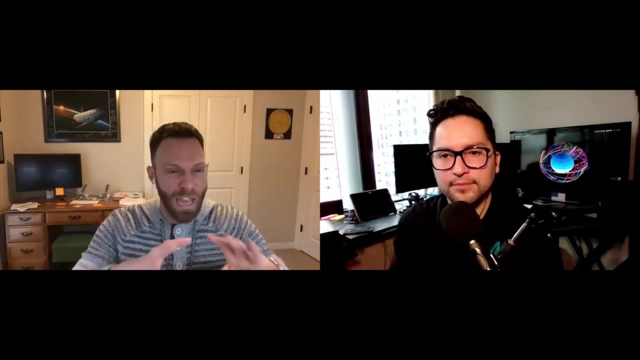 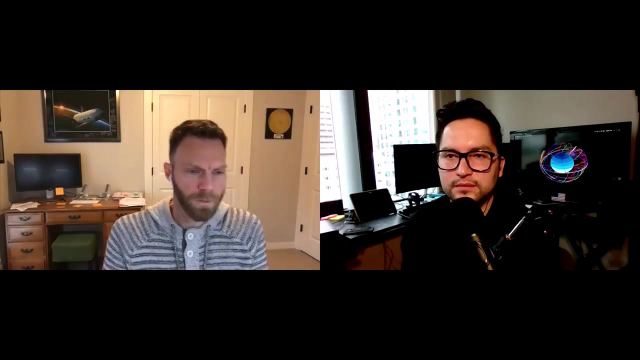 want well i want all the data and eventually you're gonna run out of bandwidth to send that down and then you have to start making trades right you want everything that's going to be as best as possible from an engineering perspective uh from a practical perspective you want to meet the requirements and just meet them like you don't want to exceed them because you're robbing from somewhere else that needs that right you're almost always on the like the edge of infeasibility across the system for the most part they can give and take um so what 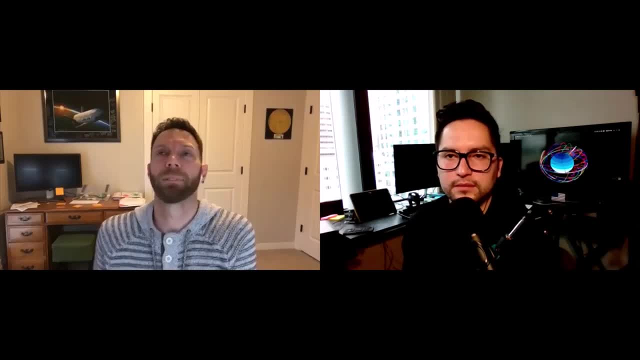 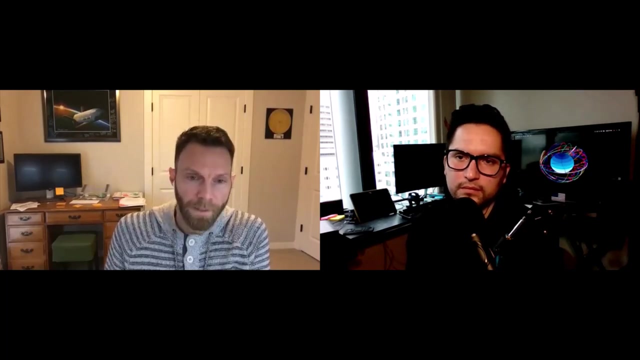 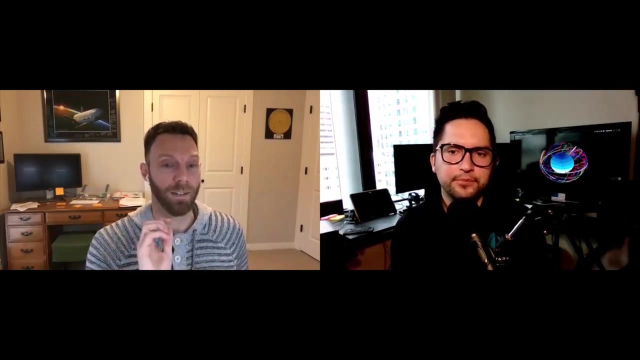 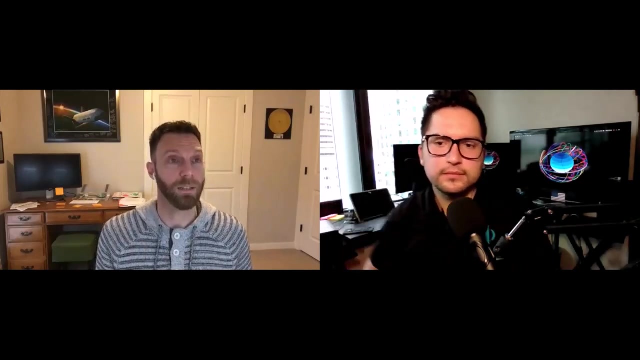 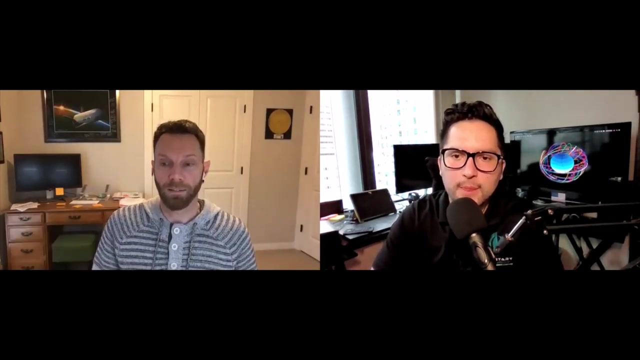 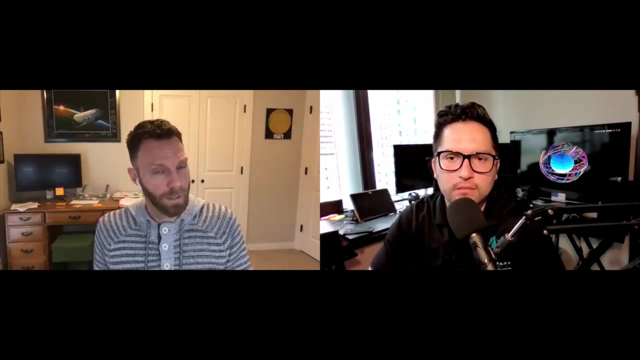 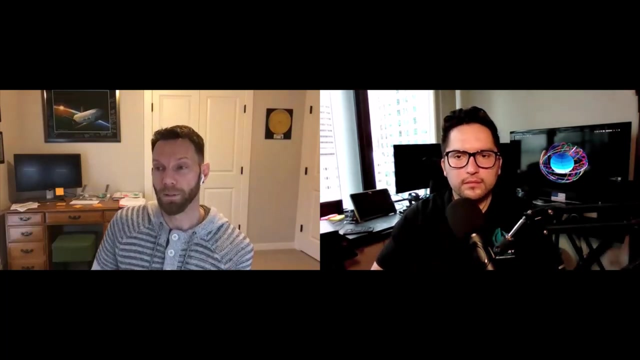 well let me let me answer a slightly different question if that's okay which is more often than not my decision on the controller that i'm using doesn't come down to the compute power but this is just the projects that i've worked on um not in general this isn't a general statement but they don't come down to the compute power they come down to how am i going to convince myself and my colleagues that this is going to work and if i do a pid controller and i say look i'm modeling my system as a linear model and here is why i can do that it's very straightforward look at how close this linear model matches the real system now now that i have this linear model that we all agree is okay here is my pid controller that i designed using that linear model and look how good it works and there's a whole bunch of metrics and and and things that we could look at to show that it works well and people understand that it works well and and people understand pid and they understand like oh what all of those games are doing and it's a very simplified thing and so it's it is easier to convince yourself across the entire state space sometimes uh that that controller is going to work and it's easier to convince other people and whenever you make a change to your system it's relatively straightforward to retune the controller this pid controller and if you have to um uh go on to into the 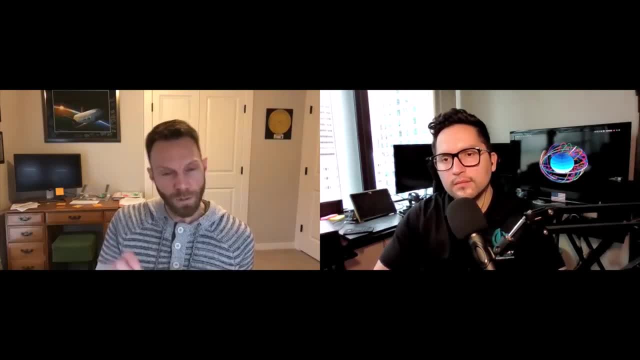 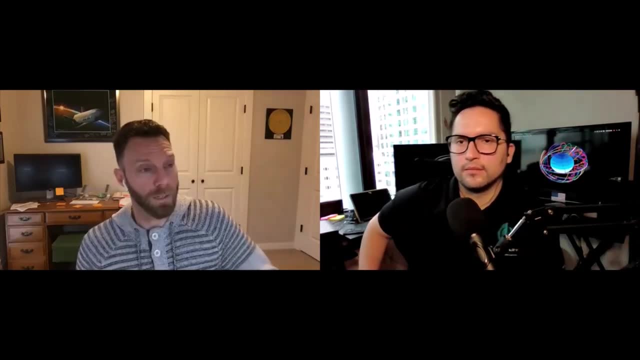 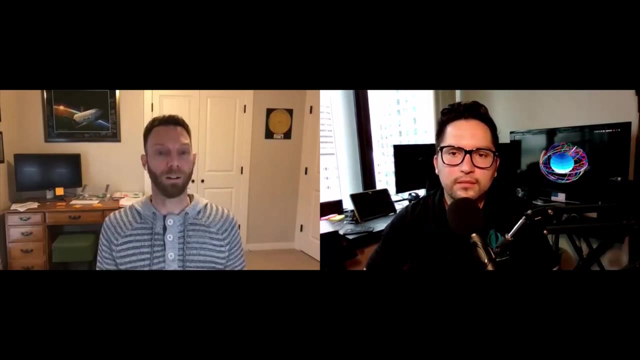 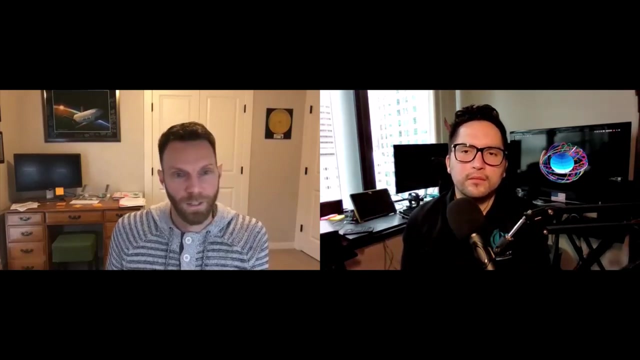 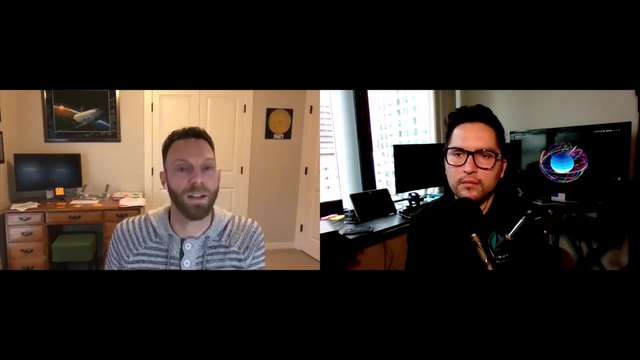 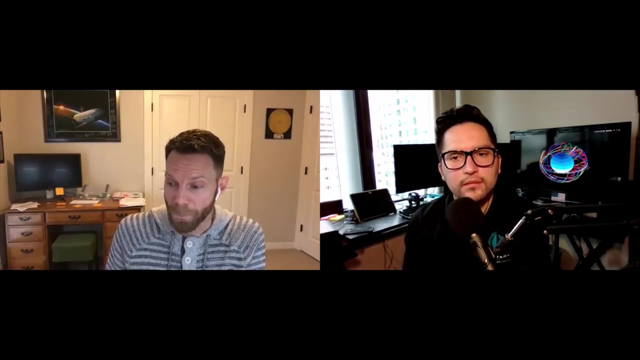 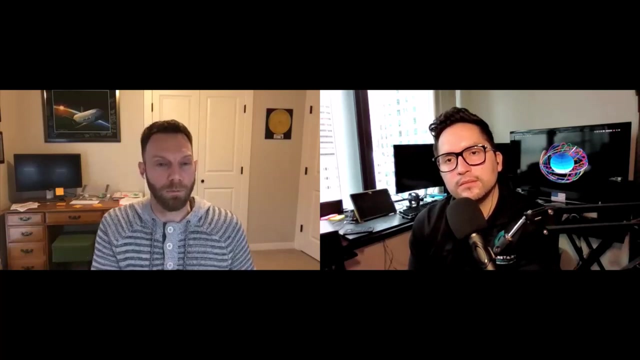 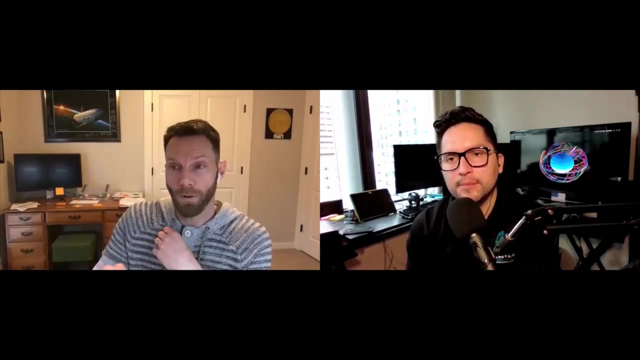 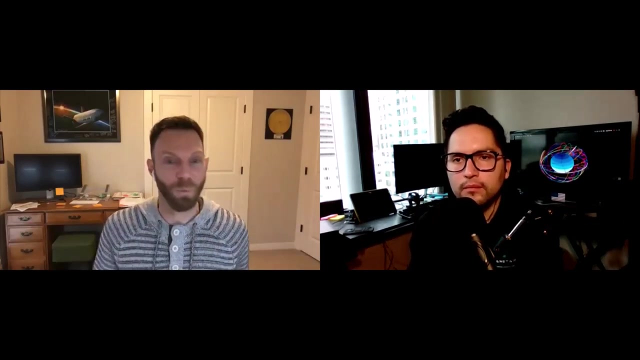 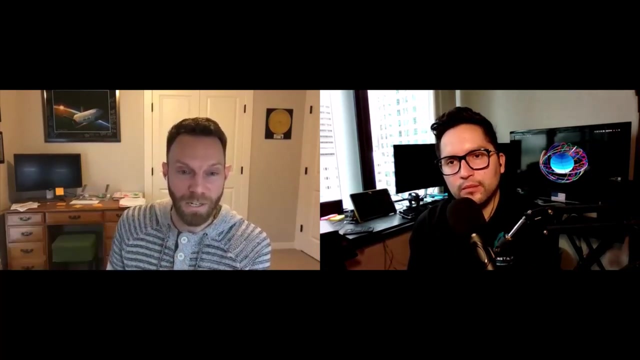 field and tune your pid controller in the field each of those three gains make some amount of intuitive sense so that's nice but i could get better performance if i do h infinity or you know maybe some form of lqr or something like that um but let's do let's stick with h infinity i can you know i can come back with this like 12th order control law with a whole pile of numbers that each individual number doesn't make any sense on itself but it works really well you know and it works i have all of this data to show look how good it works but it's really susceptible to the model more so than you know more so than than like pid is for you like you can you can design robustness pretty easily in pid and so with h infinity you say well i want it to be robust so now i want to make sure that i've designed into my model a bunch of uncertainty like which parts of my model don't i trust and how much don't i trust it so now i have this uncertain model and now i can design like a new synthesis controller for it and it's going to come back and it's going to be like 20th order and it's going to be crazy and i'm going to show like look as long as all of these error bounds you know the error stays within these bounds it's going to be good um it's just it would be harder for me to to convince myself 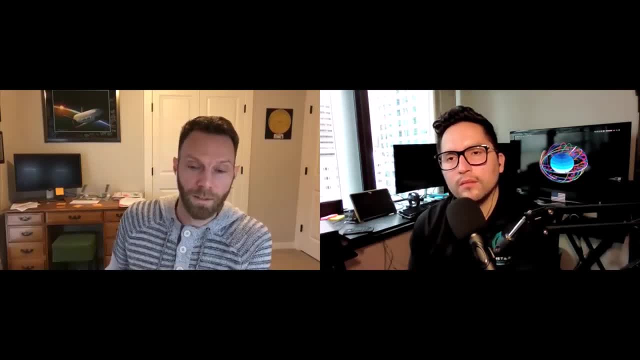 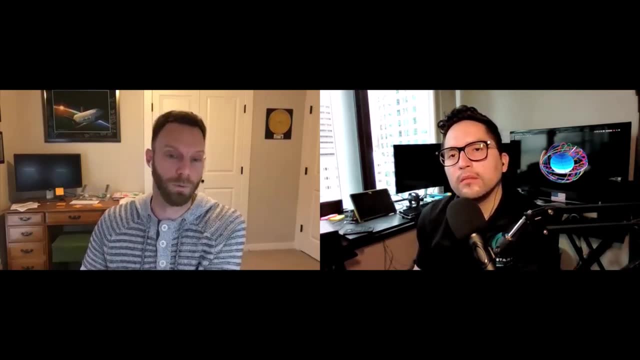 because it has so much reliance on the model then at that point to convince myself it would take more effort to convince myself that it's actually going to work on the real hardware and it's going to take a little bit more effort to convince the rest of the team and management and all that kind of stuff um and then the other downside is that the controller now doesn't have 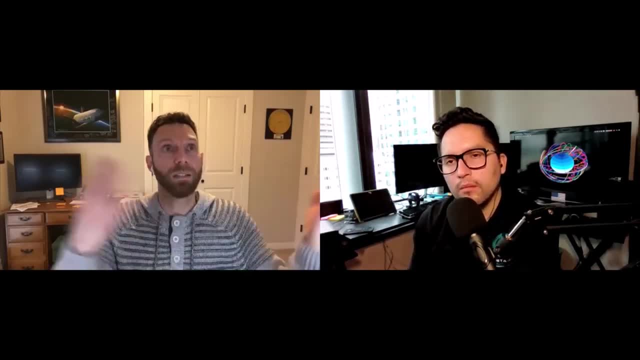 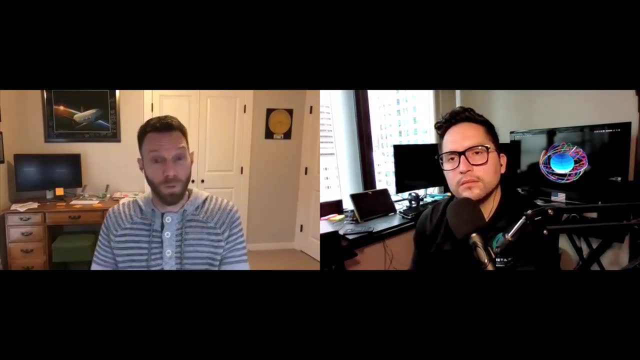 three nice neat intuitive numbers it's got dozens of numbers that don't really make any sense and so tuning it in the field becomes more of a challenge and so um and then to take that one step further why don't we just 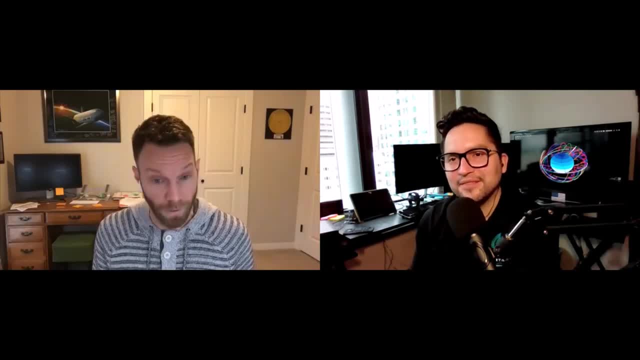 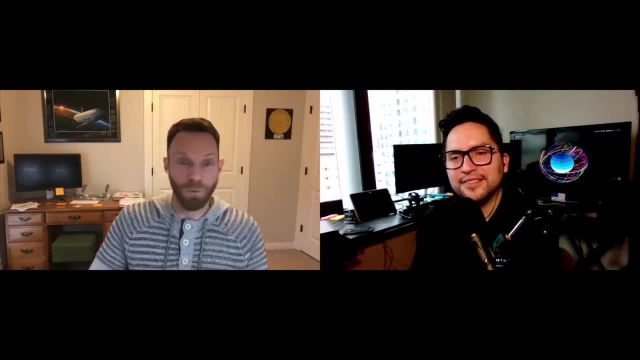 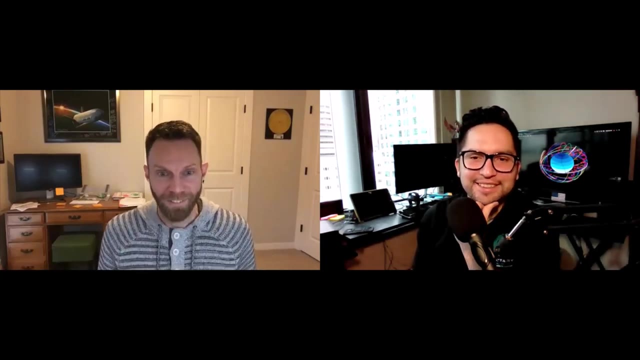 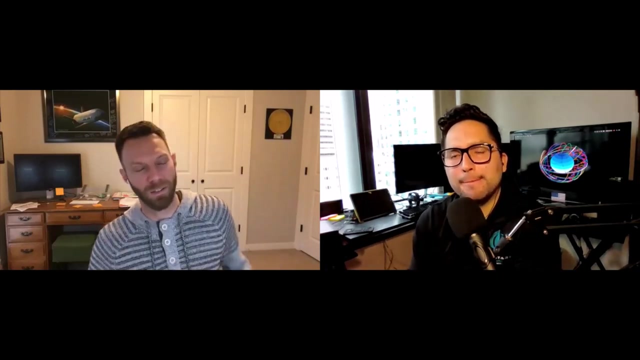 put a neural network in there for the controller and just do some machine learning to to figure out what the control system should be right and that's even more like like removed from reality it's super abstract and at that point you're like oh here's this table of a million numbers um it works in my model let me just throw it on my spacecraft and and it just comes down to the point of like convincing yourself and other people 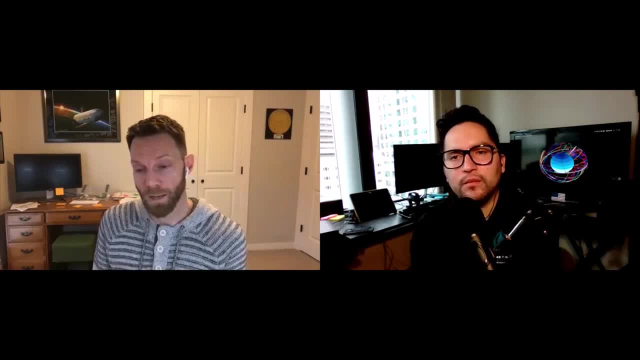 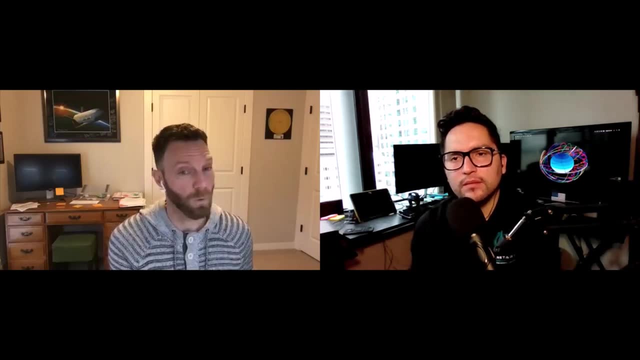 becomes time consuming and is that where you want to spend your time? so for me it has always been build the simplest controller you can get away with that meets the 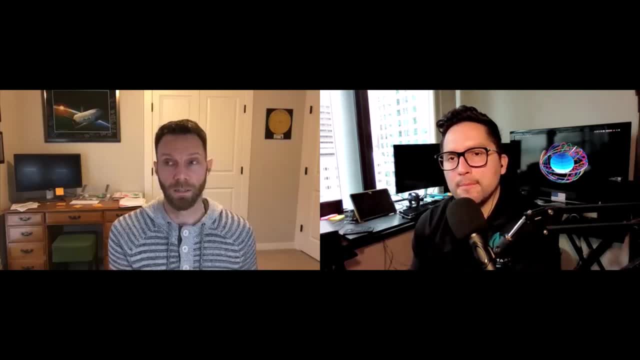 requirements barely because you're gonna save so much effort keeping it simple and there's a million 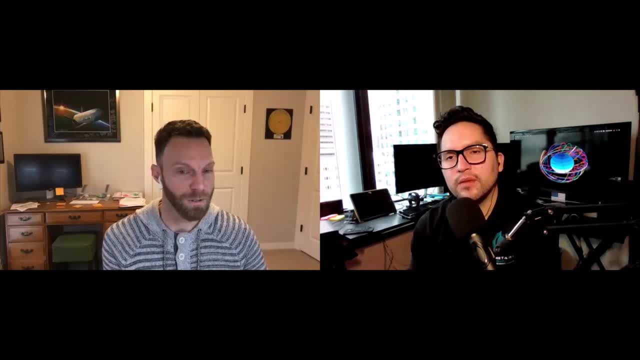 problems you have to solve on an engineering project so why are you you know you why are you saddling yourself with this really complex control law when you don't need it because you have to go off and figure out fault management and fault logic and you have to figure out how to do it right and so 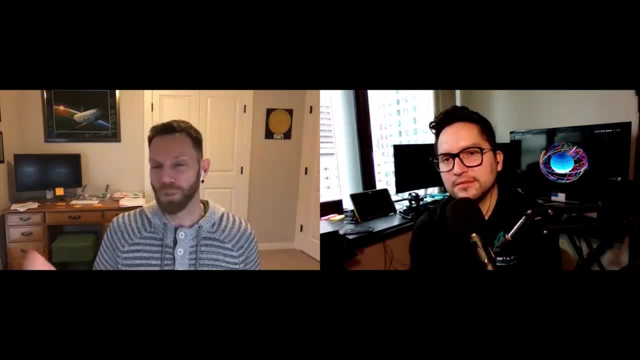 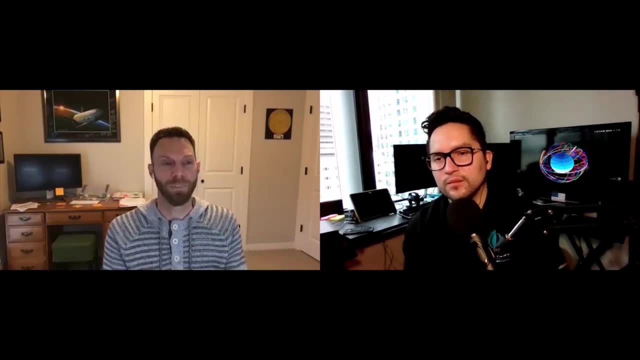 you have to go out and figure out modes and state machines you have to go figure out why your sensors aren't working right and you have to go characterize your sense it's just like a long list of stuff that you just have to do and so anywhere where you can simplify the system the 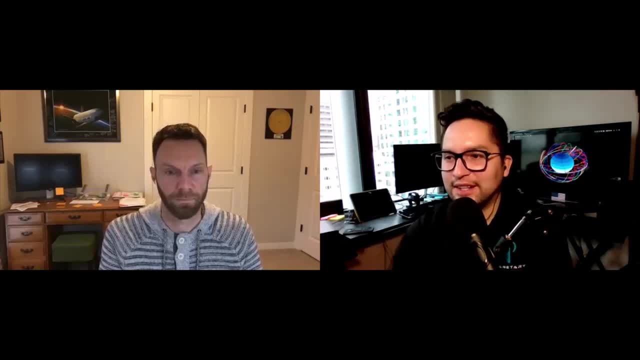 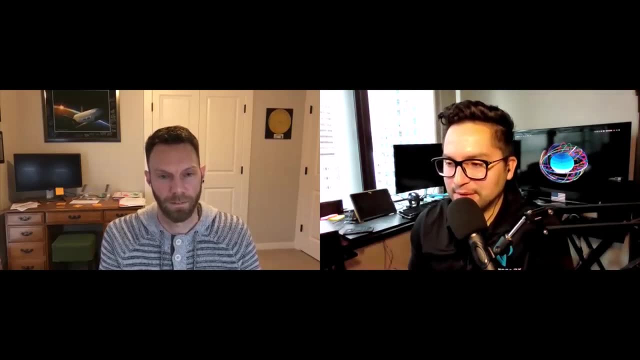 better. So you mentioned modes and I that's something that I'm kind of interested in and learning more about so basically there's different types of I mean I forget what the word is to say 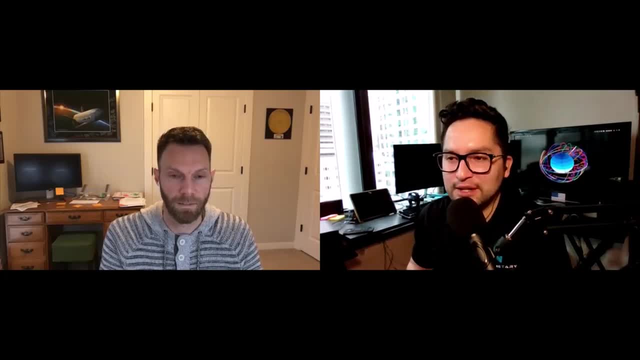 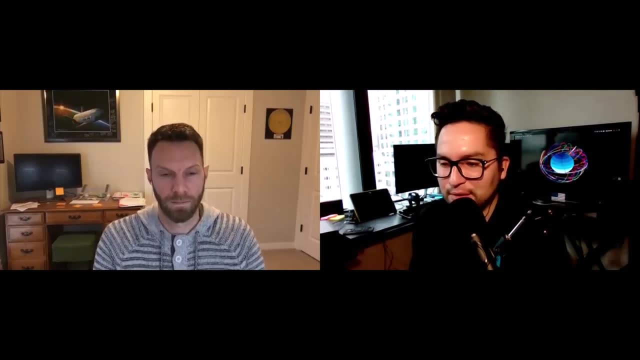 when you have like stages and lifecycle of a spacecraft to say when you have your initial activation you want to get initial communication like phase yes yes so can you talk about different modes so say like the activation mode and maybe also a safe mode so I don't know if this was the case in this kind of an extreme case but say you know a solar flares coming or there's some other reason why you want to go into a safe mode and what what systems would you choose to keep on versus off in a safe mode and is there a way to require 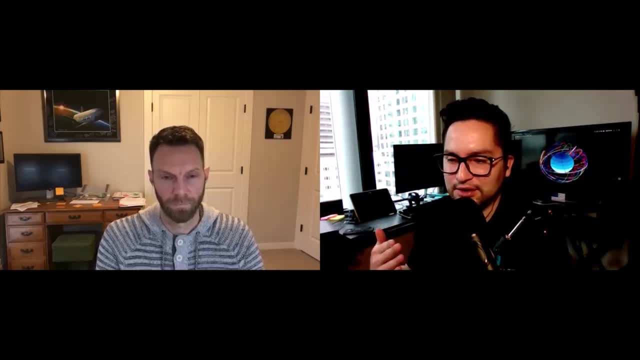 other modes like uh sun pointing so i just want to charge completely all the way or like earth 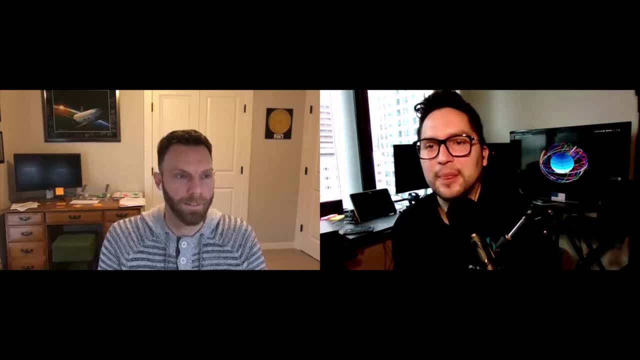 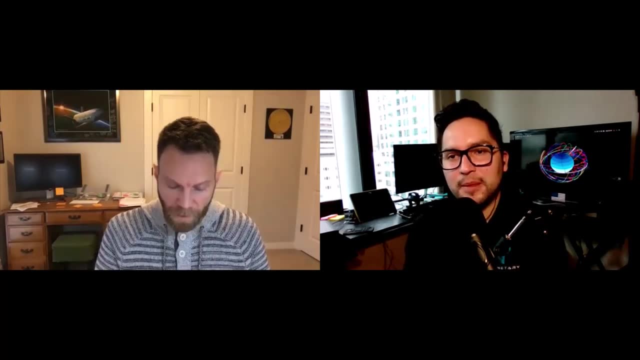 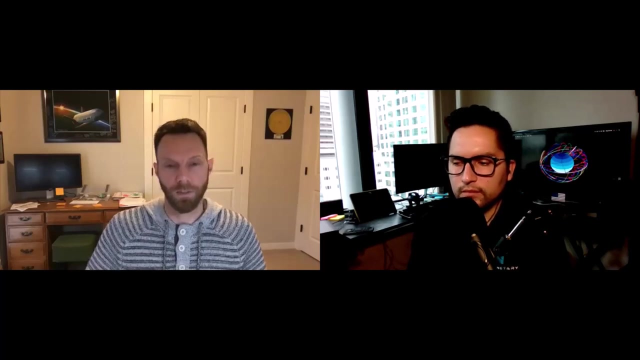 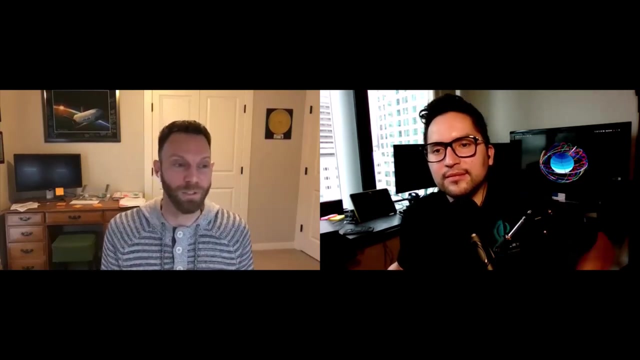 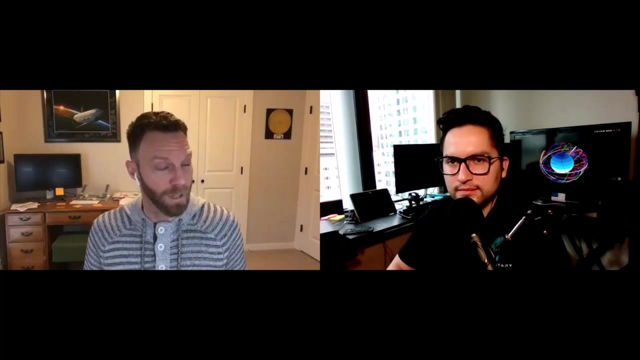 pointing and that kind of stuff yeah yeah there's a bit to unpack here um i mean in some sense you can interchange the word phase and mode and state it is like a condition that the vehicle is in and it's helpful to label a condition with something like activation because it focuses you on what is important at this particular time and what can i ignore and shed and what telemetry do i want to look at and what things need to be on and off and what are the requirements and all that stuff it's it's easy to sort of it's easier to to categorize various portions of of the mission in that way so they can you can focus and think about requirements all that stuff so within adcs right you look at the phases of the mission let's say with activation who knows what you're doing in activation you're turning everything on probably not everything right you may want to turn things on slowly because this is going to be the first time you've actually powered everything on and and they're communicating with each other in a space environment so you know you don't want to flip the switch and just go crazy you don't want to flip the switch and just go crazy you don't want to flip the switch and just go crazy and be like all right go um maybe you know maybe you do if you've got a lot of confidence in your 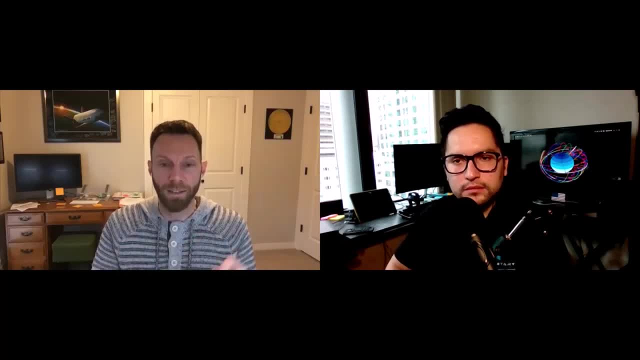 system but if you don't have a lot of confidence maybe you want to baby step your way in um there may be uh uh restrictions on activation like if you're cubesat maybe you can't turn on until you've left the the cubesat deployer maybe you can't start transmitting until a certain timer has as you know elapsed or something so so there's external requirements has as you know elapsed or something so so there's external requirements has as you know elapsed or something so so there's external requirements and internal requirements that you got to think and internal requirements that you got to think and internal requirements that you got to think about with each of these phases about with each of these phases about with each of these phases now we may say a mode or a state um now we may say a mode or a state um now we may say a mode or a state um also and that that might be like within also and that that might be like within also and that that might be like within like the activation phase of the mission like the activation phase of the mission 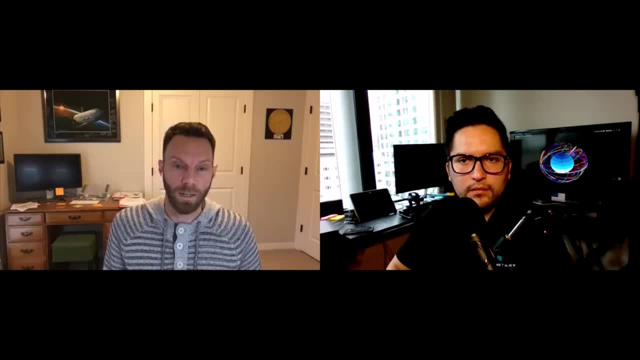 like the activation phase of the mission the spacecraft might go through several the spacecraft might go through several the spacecraft might go through several different modes different modes different modes um or may fault into a specific mode um or may fault into a specific mode 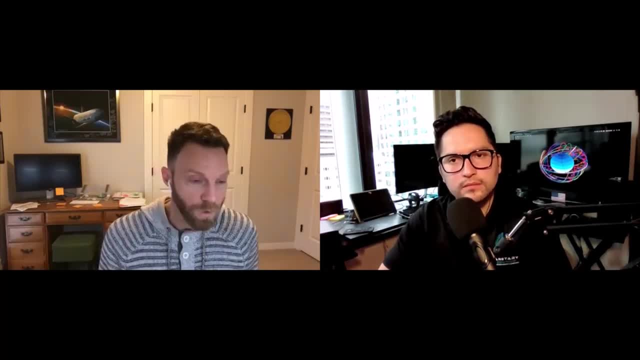 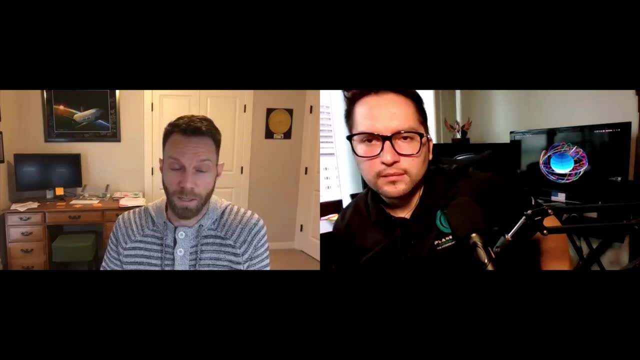 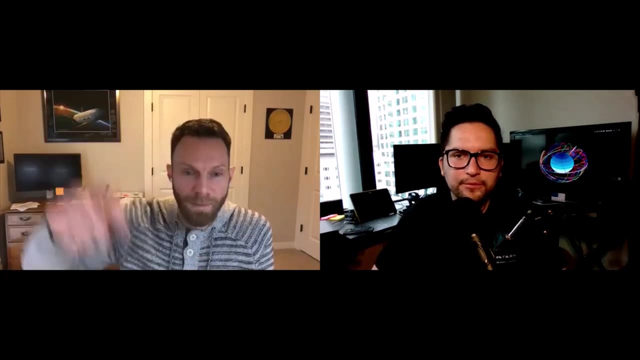 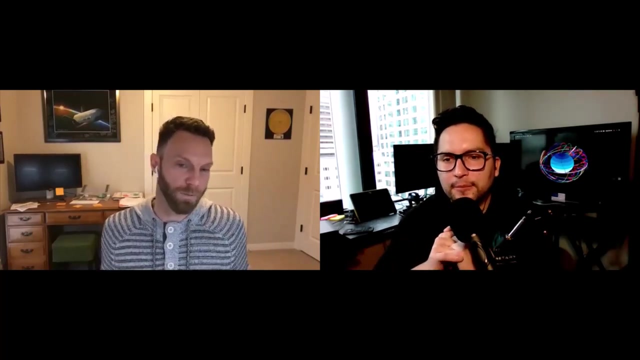 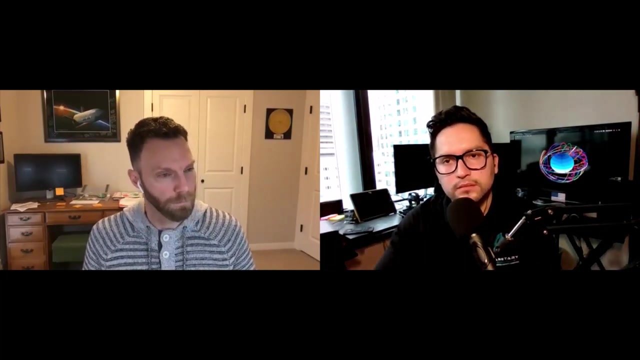 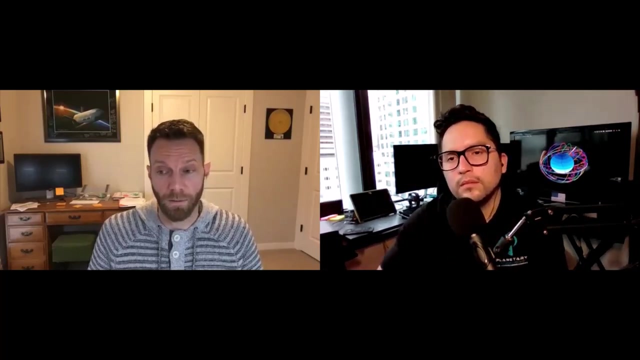 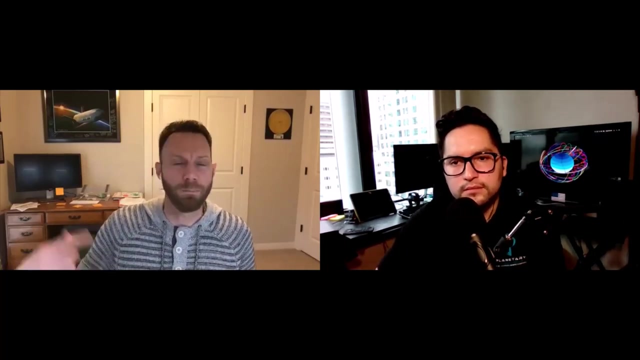 for example. And, and again, it's the exact same question is what, well, let's take fault, for example, what is the fault? You know, is it the check engine light come on? Is it low tire pressure? Is it, uh, you know, the smoke is coming out of my engine compartment on my car and it just stopped running, right? Each of those things are going to have a slightly different response and spacecraft are no different, right? Is the current to my reaction wheel slightly high? And troublesome, right? Do I need to shut down the reaction wheels because I'm worried that they are about to fail? Or does that high current just mean maybe I should desat because, uh, friction has increased more than I was expecting in like the lubricants. And so now I don't really want to spend these, these motors as high as I originally thought. So I need to desat a little 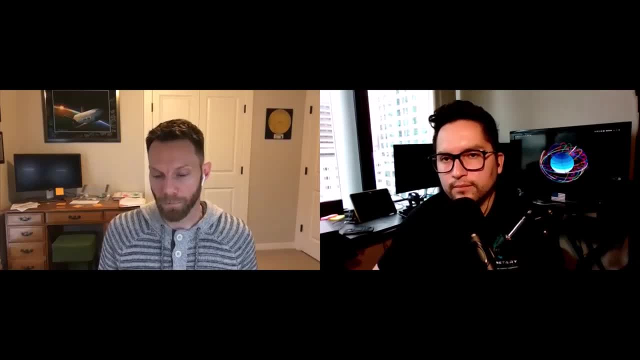 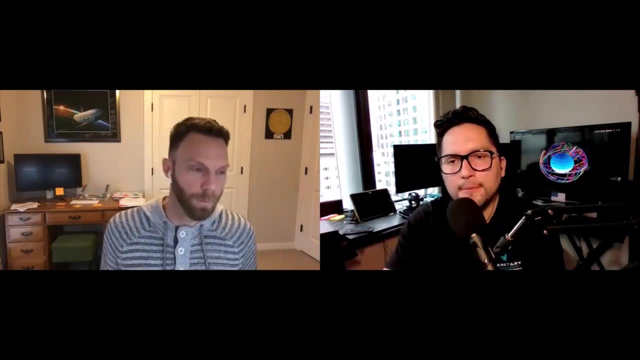 bit earlier. Now I can't store as much momentum. Um, or, or is, is there a messaging failure or something, whatever it is, right? You, you write all of these fault tests and you try to come up with all of these different ways that the vehicle can fail. 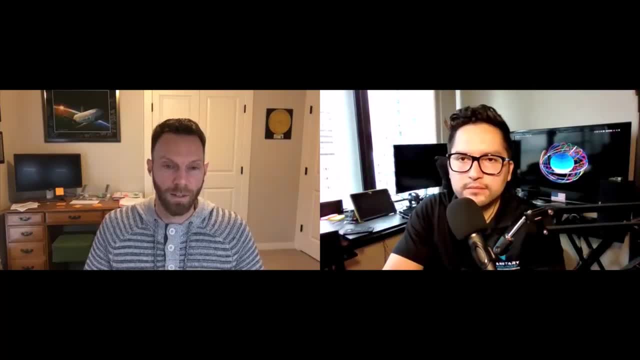 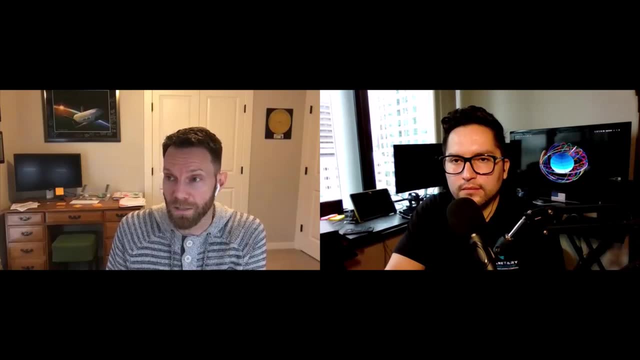 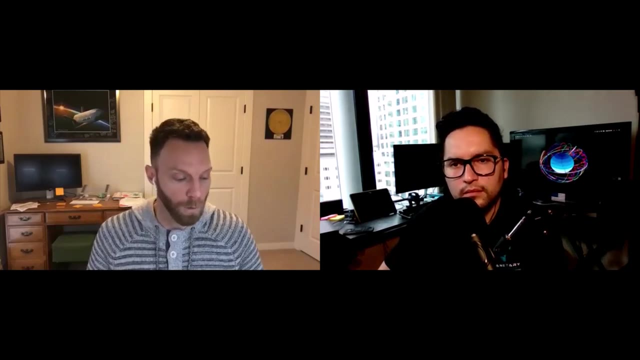 And how do you want to sense those failures? And then you can say, okay, what if that happens? What should we do? Um, should we safe the vehicle? And that means something bad happened, but I'm not quite sure what. So let's go into a mode that uses the least amount of power. Okay. That uses the least amount of hardware and software so that we can keep this vehicle alive while we figure it out. And so with a reaction, with a ADCS system, that might be shut down the reaction wheels, shed all the momentum in the system with the torque rods, point the solar arrays towards the sun, stop using your star trackers because they take too much power, 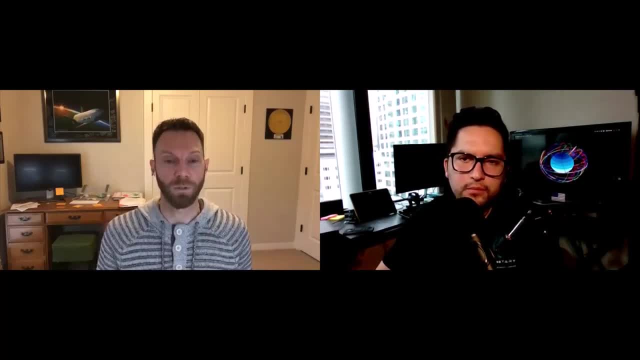 use the sun sensors, use the magnetometer and use the torque rods or something, you know, who knows it? 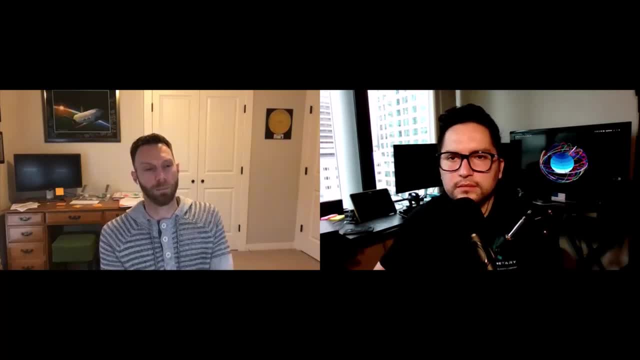 Depends on whatever anybody comes up with their, for their particular system. Um, but you know, safe mode versus pointing versus whatever. These are all just ways that you want to operate your 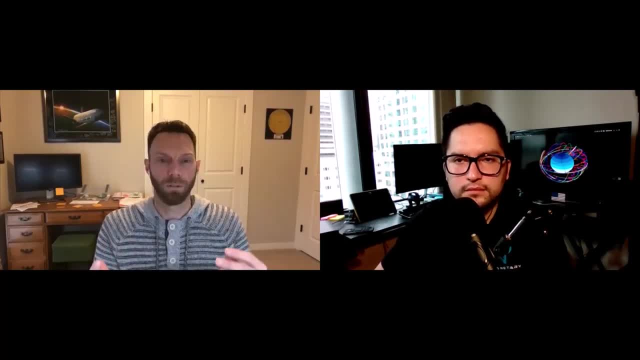 system. And it gives you a label to focus your thinking and determine what needs to work. What information do I want to have access to? And what do I want to protect against in this particular situation? 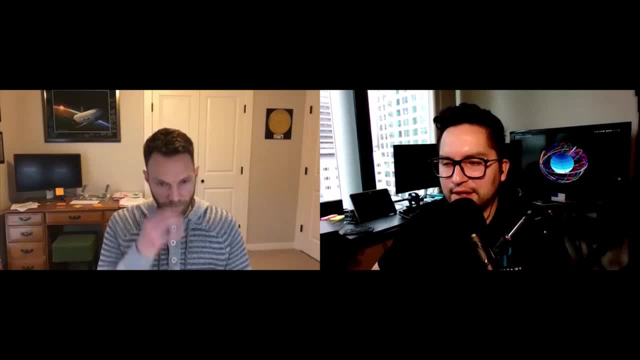 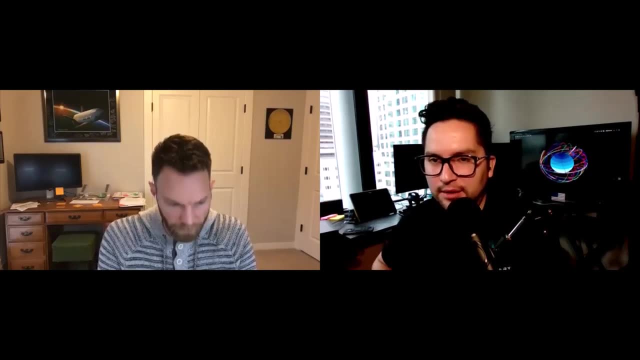 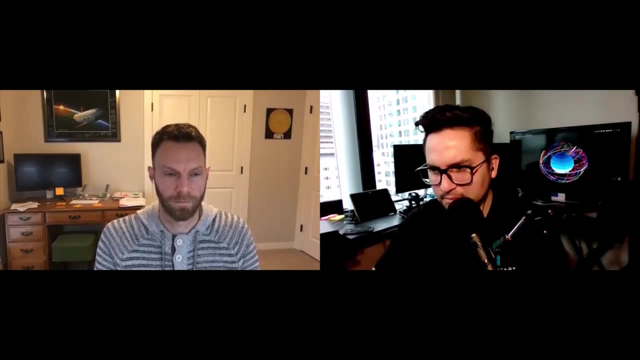 Going a bit of a different direction, I want to ask you a bit about orbit determination because I know there's a, there's a lot of ways to do that, just like attitude determination. Um, so in what ways did A3 and A6 go about that? Was it from the ground, just using the ground measurements in order to, in order to send the spacecraft, this is where you are, or was it more of an onboard calculating where am I? Yeah. Okay. So just like with any state of the earth, you know, you're going to have to have a lot of information. Yeah. You're going to have to have a lot of information. Yeah. 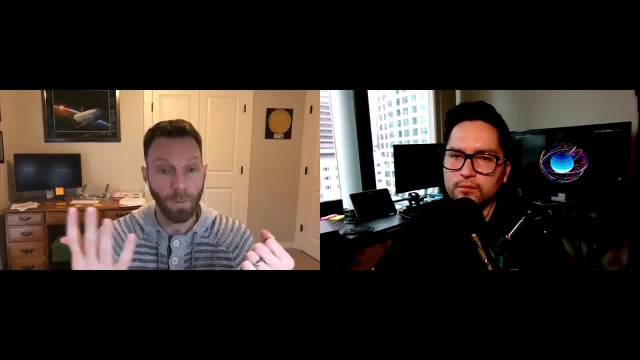 So the other way that you can do that is you can use the orbit estimation. Like we talked about with the Coleman filter is you can, you can estimate your state with a model and you can estimate your state with a sensor and you can blend those two together. 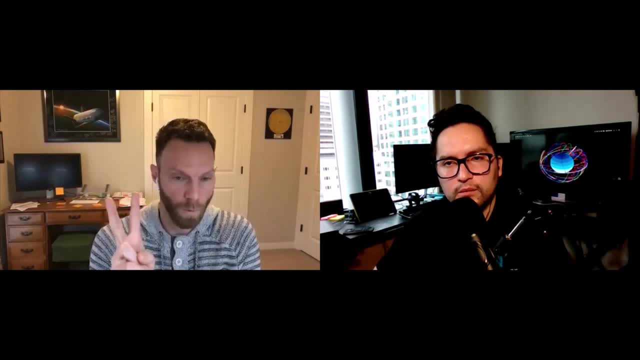 So with that understanding, we used two sensors for orbit determination. The majority or the main sensor was GPS because we were at a low enough altitude that we could still use the GPS constellation. The other one was a measuring instrument. 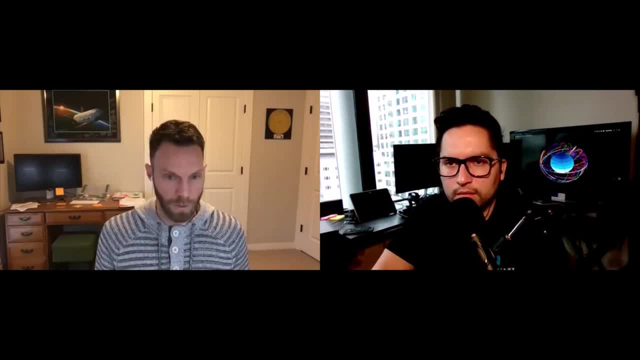 Okay. So it was a measuring instrument from the ground, from some tracking station on the 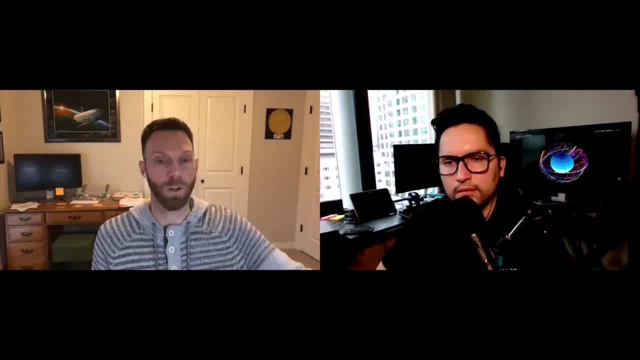 ground where they would say, this is your ephemeris. This is where you are at this time. You know, it's probably yesterday, but, but at this time, this is precisely where you were. And this is your, your state vector. Do you get that from a TLE or another? Yeah. 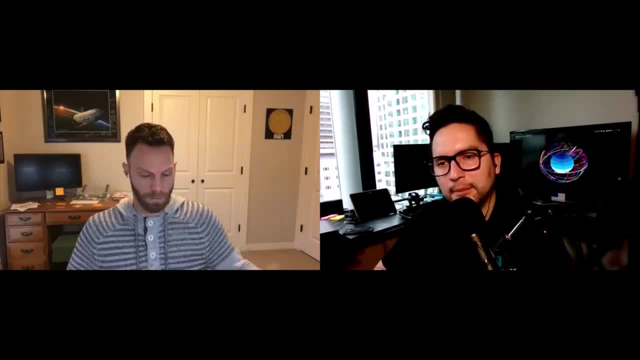 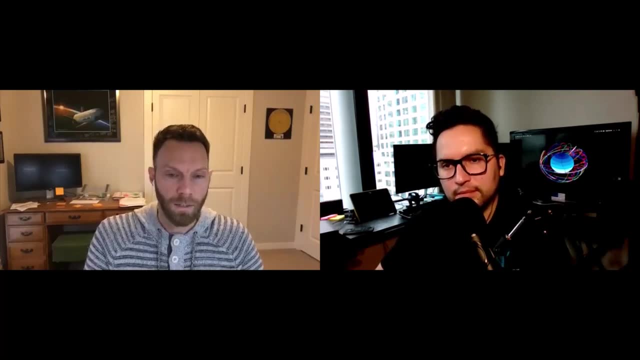 Well, yeah, you can get it from a TLE, you know, uh, through, through the government tracking programs and whatnot. You could also get it from, um, there's, there's companies that just operate. Uh, radar stations that'll ping your satellite and determine, and you can get that state vector in any form that you want, whether it's, you know, position, velocity and time or TLE or, or whatever. 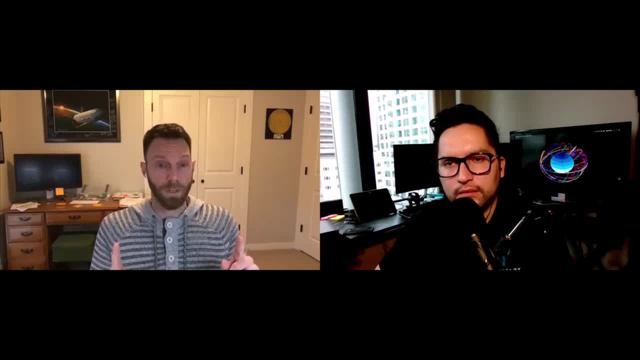 Um, so, so, so those are the two ways for us to get an update, to get a, a measurement, which is like the update of our orbit, which is at this time, here's where we were and how fast we were going from that point on. 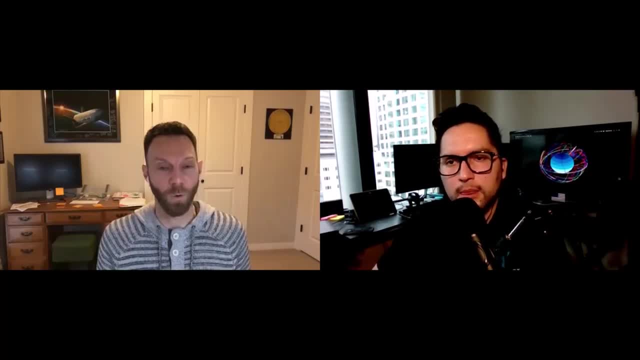 We would model where we were using an orbit model, like a, like a orbit dynamics model. For A6, we used what's called SGP4, simplified general perturbations for, this has been forever by the way. 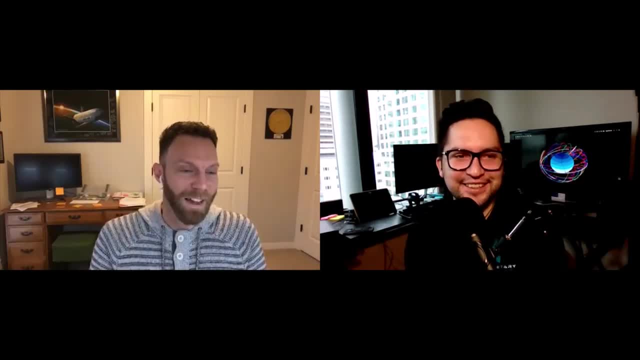 So, uh, double check everything I'm saying, um, uh, which, which, okay, good. Yeah. Uh, which was, uh, an orbit propagator. Yeah. 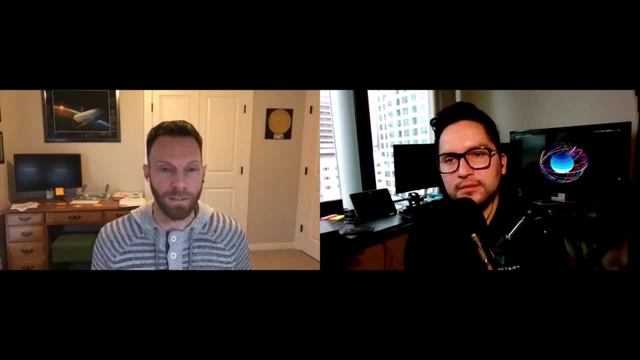 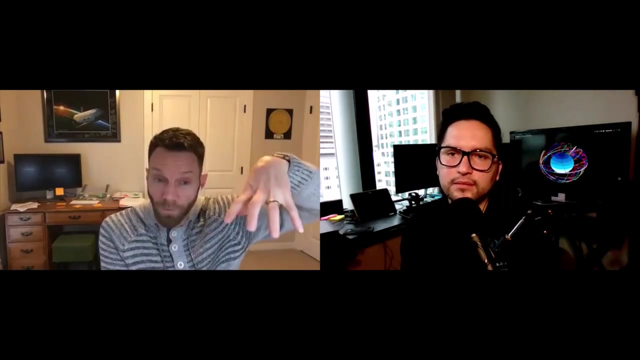 That, um, went hand in hand with like a, a TLE, um, and it, it is, uh, well, you could have, I mean, you're, you're better equipped to talk about this than me, but if you wanted to estimate an orbit, you could do so with like a simplified two body problem where you treat the earth as a point mass, you treat the spacecraft as a point mass. And then, you know, what comes out are like these ellipses, perfect ellipses, or you can give the earth some volume and you can say, oh, it's not a perfect sphere. It's kind of oblate. And so there's these like J2 perturbations. Yeah. That kind of mess with the orbit and I want to take that into account. And then there's, uh, like these long duration effects from tides and, you know, there's, there's drag and, you know, all sorts of things that can affect your orbit long-term. And so depending on the fidelity of your propagator, you may choose different models over another. And the simplified general perturbations model takes those, takes those perturbations, um, simplifies them, which is in the name and, and, you know, comes up with what it's, what it is as a compromise between the speed in which you can do the calculations and the accuracy. 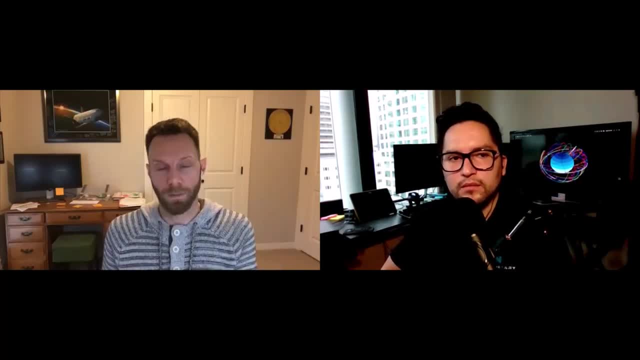 And the way that we seed that model with an initial state on the vehicle was from a TLE that we, uh, uh, that we would, you know, upload from the ground or from a position and velocity vector from GPS and then converted. I can't remember whether we converted the TLE into like position velocity or the position velocity into the TLE. Um. 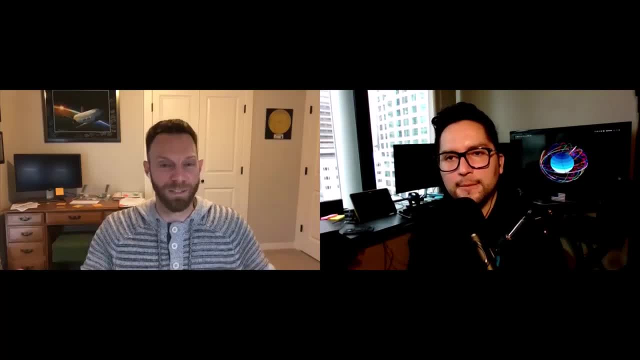 But either way, we had to put them into the same coordinate frame because the GPS and the tracking stations on earth produced state vectors in different, um, coordinate systems. 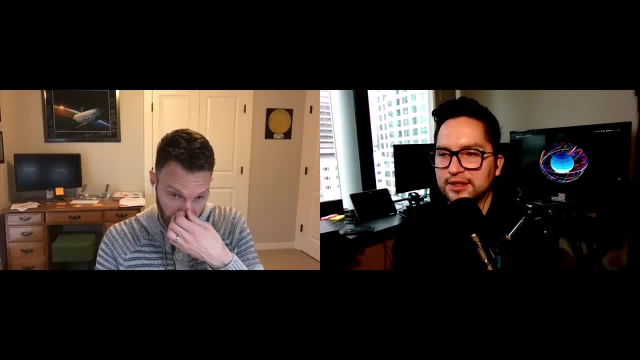 Can you talk a bit more about how GPS works because I don't know too much about it and I don't know how much you know about it, but I mean, it can get really accurate if you do it correctly from what I know. 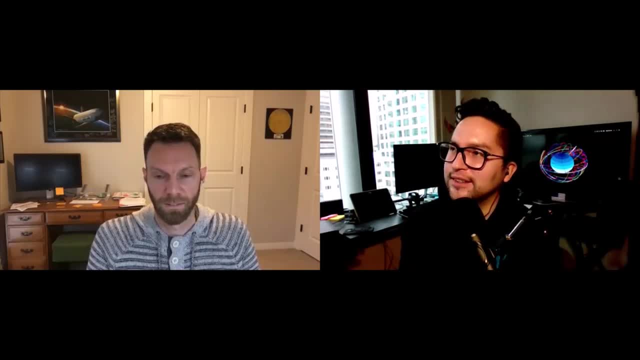 And then also, because I know at some point, if you want to say when you're on your phone and you're driving, you want to go somewhere, um, that those satellites have taken into account relativity in order to do that. 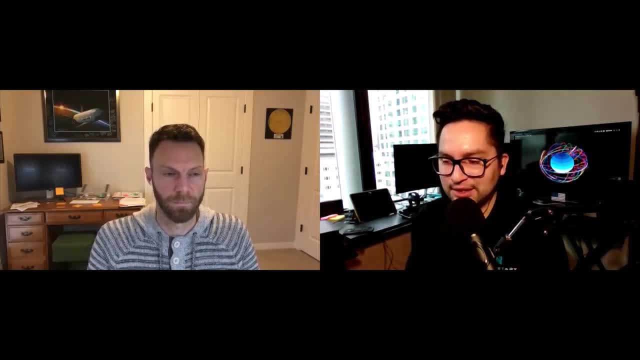 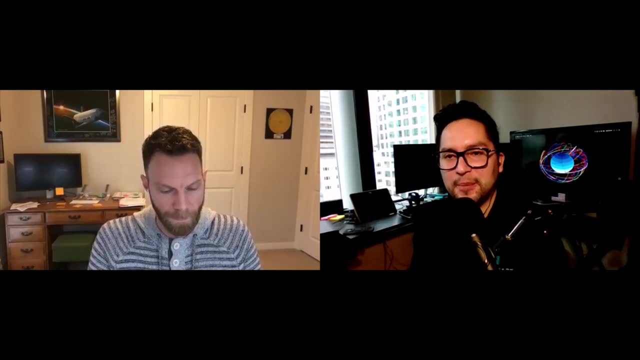 In order to get very, very precise, uh, information. So can you just talk a little bit more about that as much as you know, from GPS? Well, yeah, I don't, I don't know a whole lot, um, but I mean, they do take into account 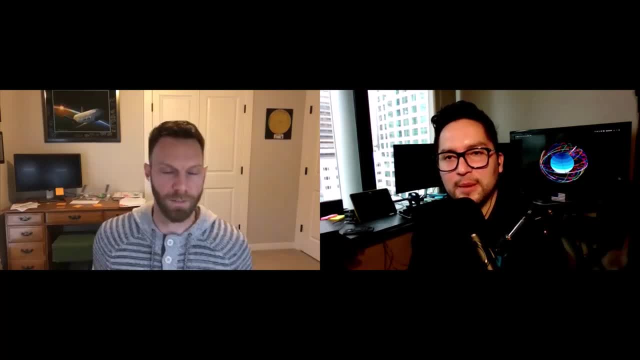 relativity. I mean, just from their clocks, right. They have to keep that, they have to, you know, the whole thing comes, it's like a big time system. 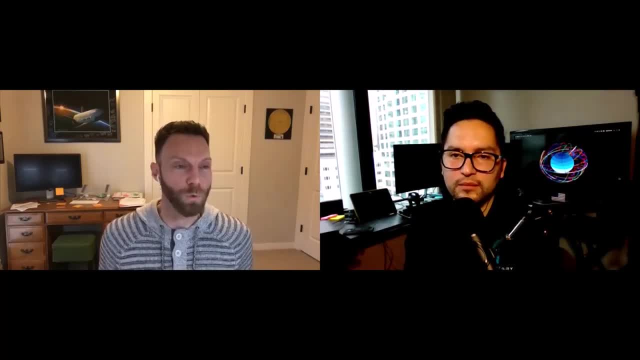 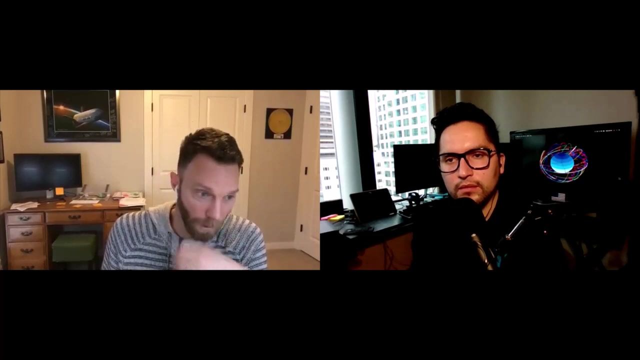 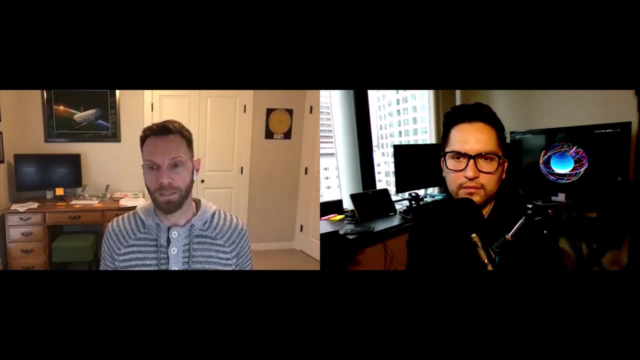 It's like a timekeeping system is essentially what it is. And if you know precisely where, uh, a bunch of every sat, every satellite is located, right. And each satellite knows precisely what time it is and it's all coordinated across all of the satellites, then it can send out, you know, these signals with a timestamp essentially. And you know, the idea of the satellite that it's coming from, and then your receiver can receive all of these signals and it can say, oh, satellite two, I just received its message and it sent to that time X and satellite three. I just received this message and it, you know, and at, at time Y, and I know where those two satellites are because they, it told me I can then triangulate, you know, you need four, but, um, I can then triangulate where I am based on these, you know, the, the, the time travel it takes for these messages to reach me. 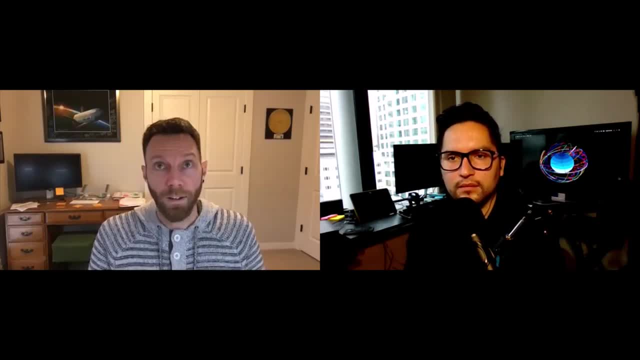 Um, and, and it's, you know, you can imagine that four satellites right next to each other versus four satellites. Right. Right. 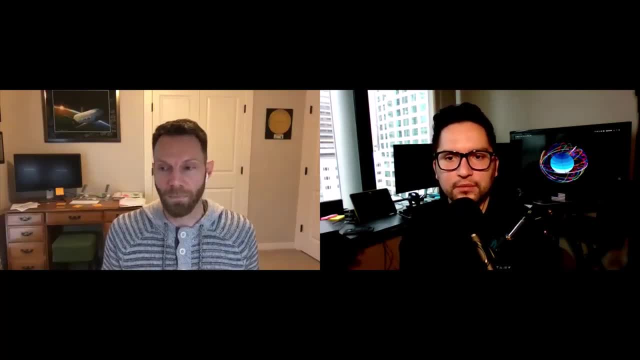 Out across the entire sky are going to produce different results because, um, you, you know, the, uh, the, the, the ones that are all clustered together are essentially going to be tarred to, to, you know, there's not enough separation between all of them to get a good measurement, right. 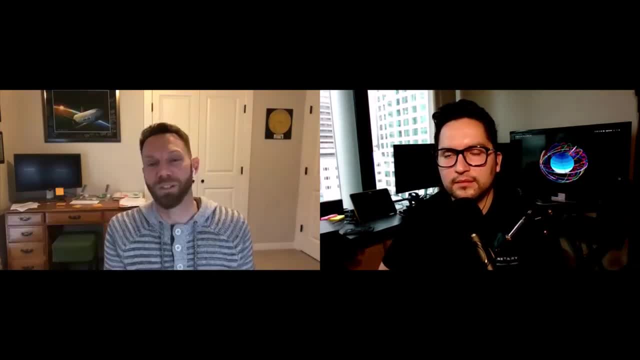 You'll know exactly how far away you are from all of them, but there's not enough in the other dimensions to get a good X and Y location. 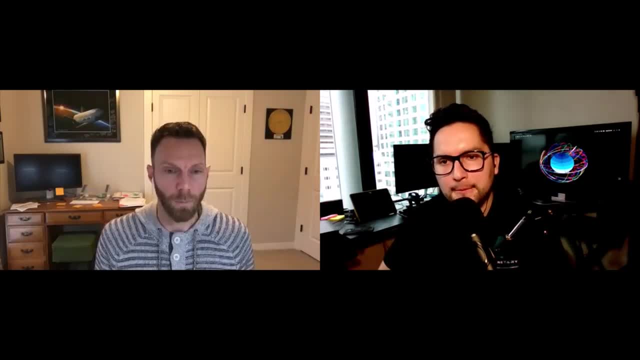 So there's this thing called dilution of precision, um, DOP, which come down, uh, or calculate. Remember the GPS receivers calculate that. And so you can use this DOP value to determine how much you should trust your GPS measurements because it is a, it is a value based on which satellites it's using and how spread out they are relative to you. 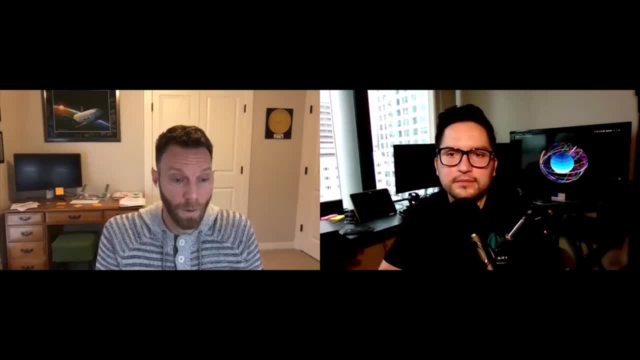 Um, so we use that in, in our state estimation, we use, you know, DOP to determine how well, how well the trust GPS. And then, uh, satellites are moving. Okay. They're moving really fast. Right. 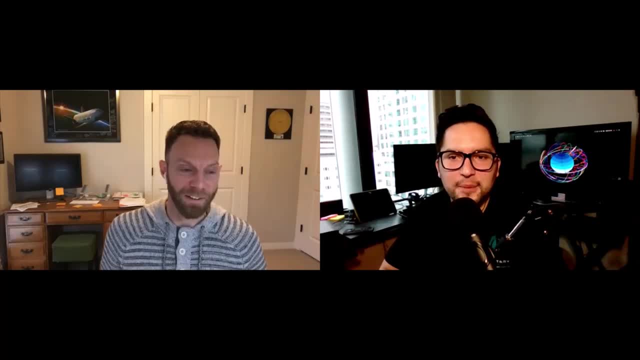 I mean, you know, kilometers per second. And so, uh, the cross track axes, the ones that are not in the direction of travel tend to be a lot more accurate than the end track direction because you're moving so fast and 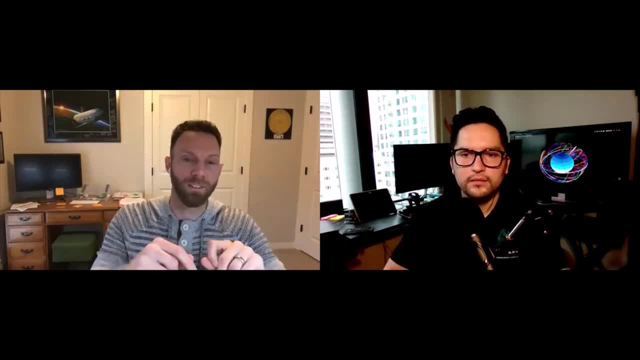 velocity needs to subsequent measurements to determine. And then you're like, well, I'll just average them and say that my velocity was at this time. 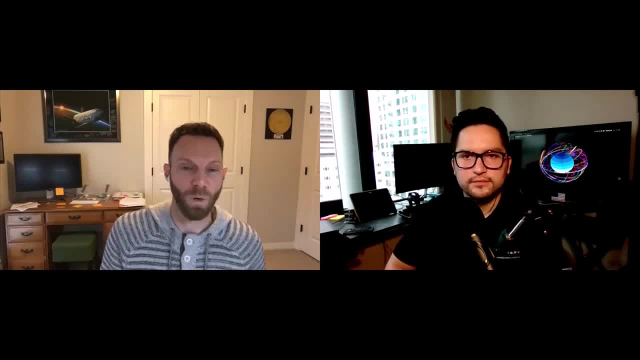 And I don't know, it just gets a little bit tricky with timestamps and, and what to trust. 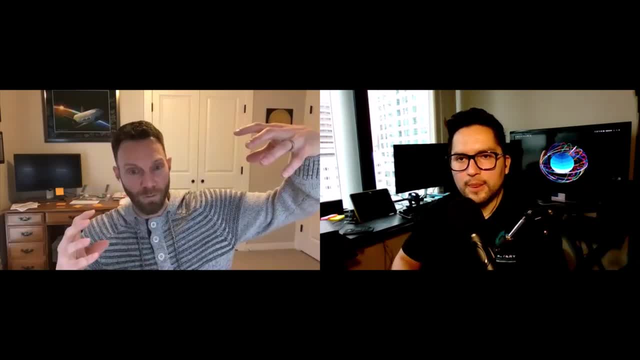 So the, the error ellipse tends to get. It's stretched out in the direction of travel, um, and you, you tend to not have as much accuracy in that direction. 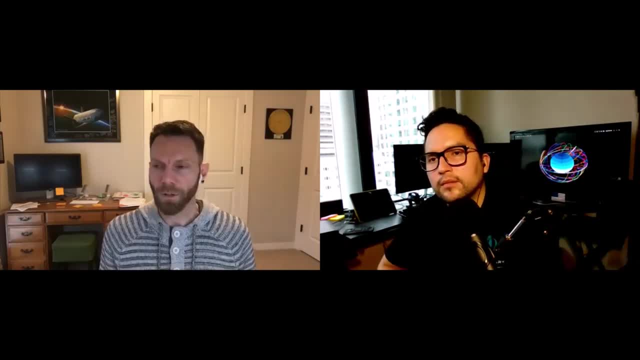 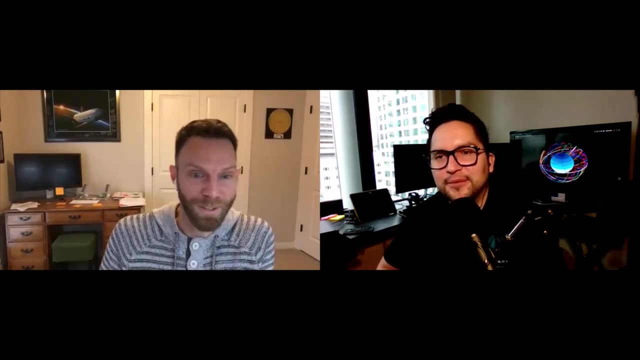 So, um, yeah, I don't know, I don't know if I answered any of your questions there, but those are the extent of my, you know, how we use GPS and the things that I was concerned with anyway. No. Yeah, definitely. You did. 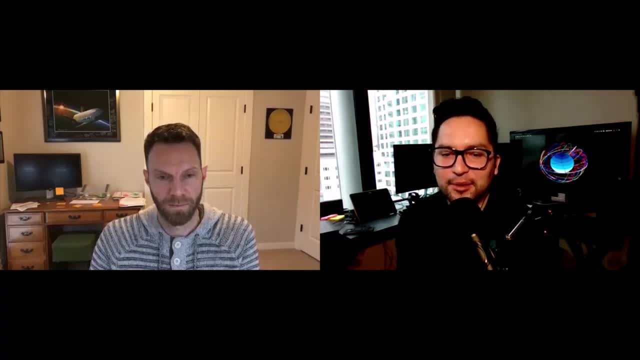 Um, so I want to bounce back a bit to soft SIM and Monte Carlo simulations, because I think that's pretty interesting. And then, you know, you can go a lot of different directions. Yeah. 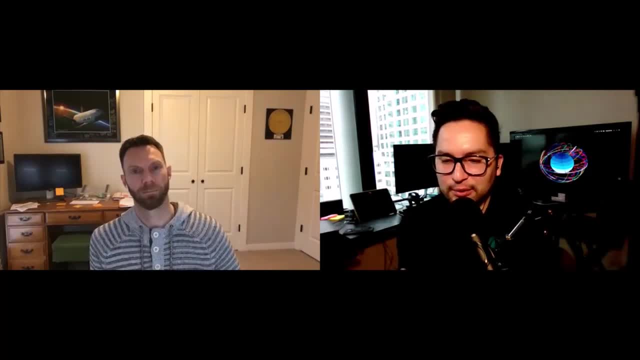 You can go a lot of different ways as far as the software goes. So from your experience at planetary, how were Monte Carlo simulations use and then what were they useful for? 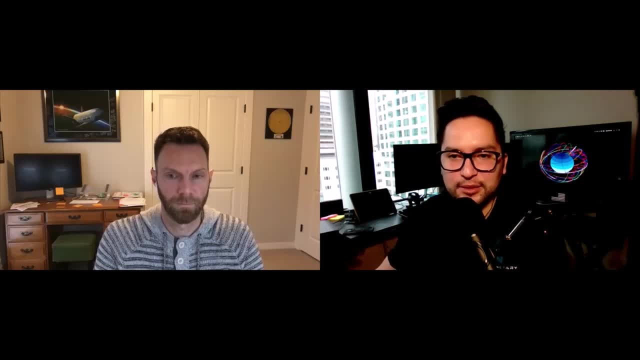 Like what kind of stuff were you looking for in doing these simulations? Yeah. 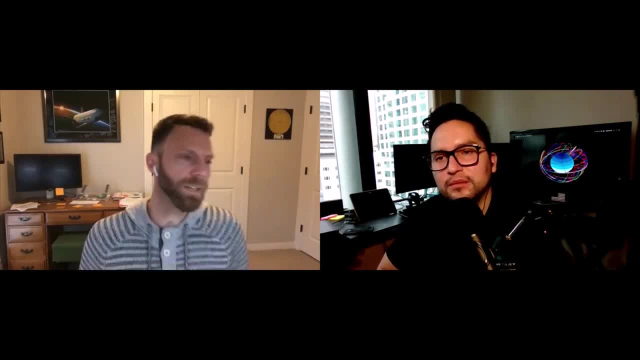 So a Monte Carlo simulation, well, let's say, um, anything that has statistical variation. Yeah. 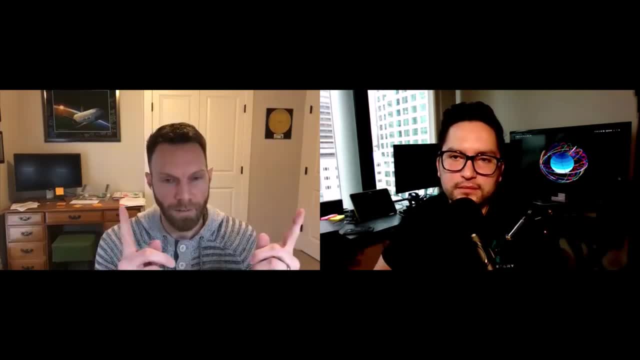 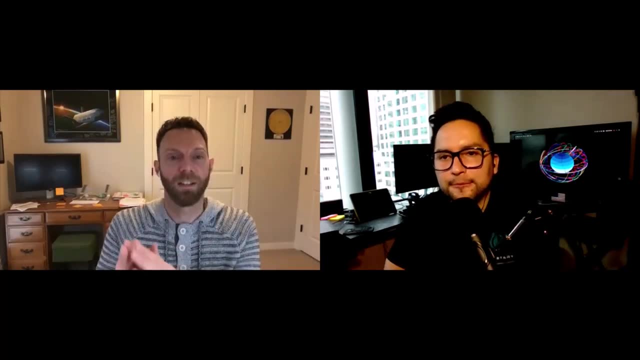 So it's going to be, if you're building something, the length of a rod, every time you build that rod, it's going to have some tolerance there that, that is, you know, based on some statistics that, you know, maybe it's normally distributed or something in some way. Um, same, same with everything else, like sensors, sensors are going to have some amount of error. There's going to have some amount of bias. And that bias is not going to be the exact same. 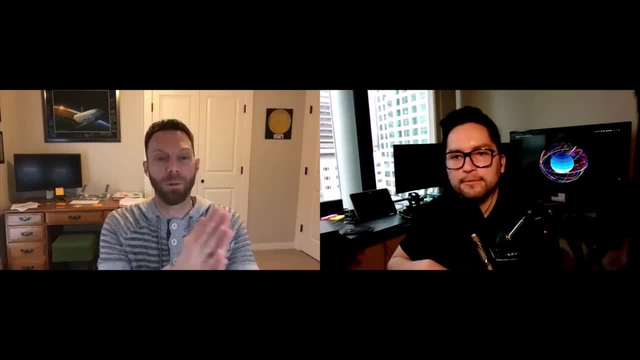 Every time you turn off and turn on the sensor, that bias is going to move and how it moves is going to have some distribution. 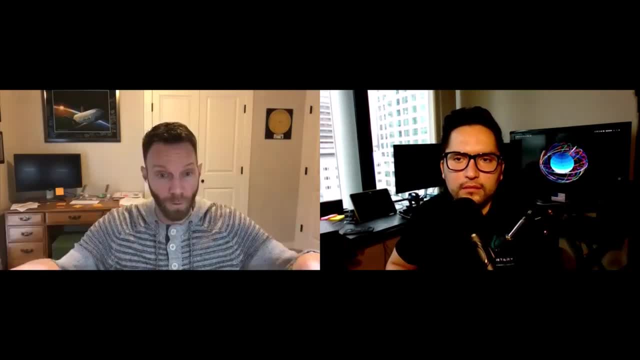 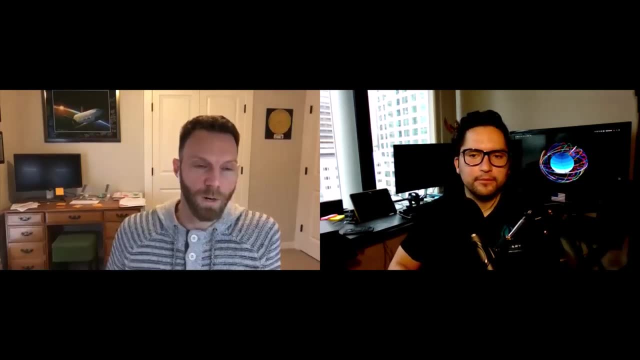 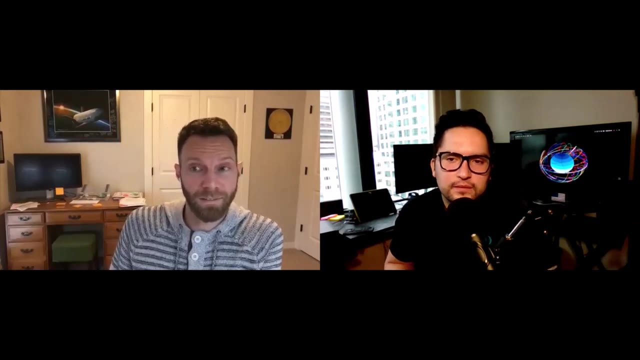 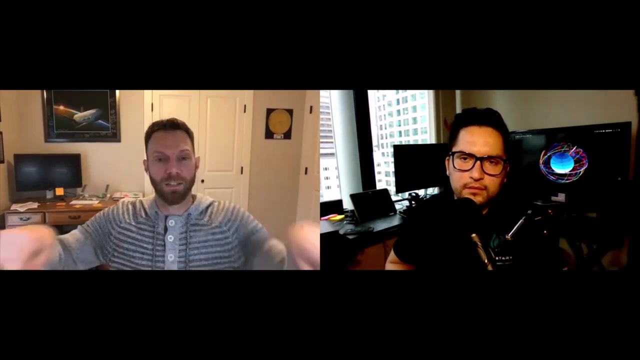 And it might be a little bit different. It might be distribution and it might be Gaussian. It might be uniform. It might be some crazy distribution, whatever it is, you know, um, and, and, and so you want to ask yourself this question, can my, I know my system, well, maybe you don't, but let's say I know my system works if everything that I'm predicting about it is right on, but everything has these statistical variations in it. 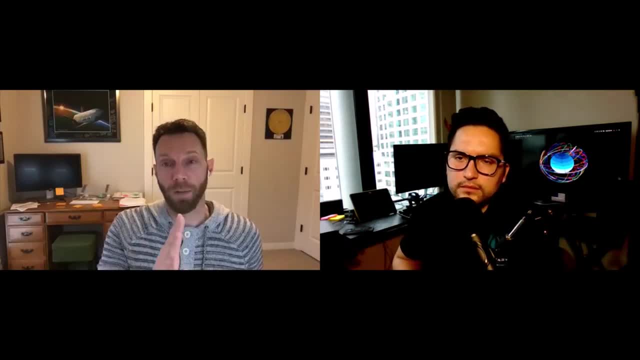 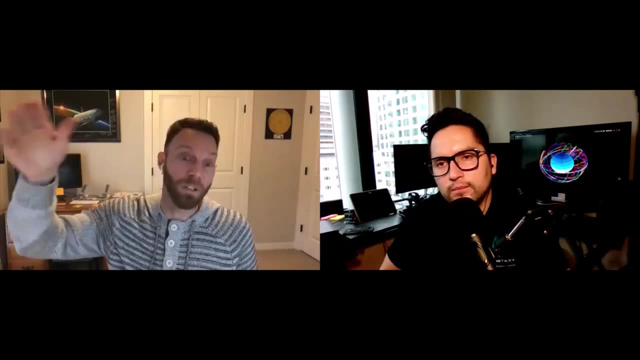 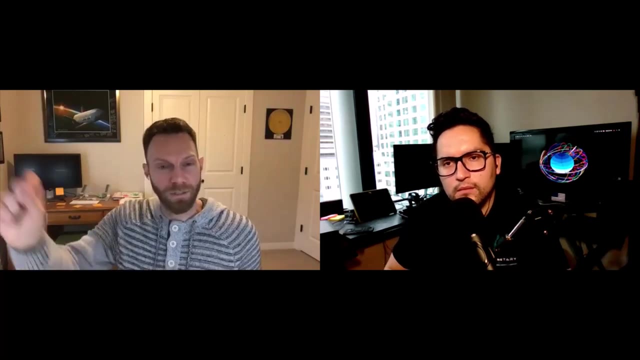 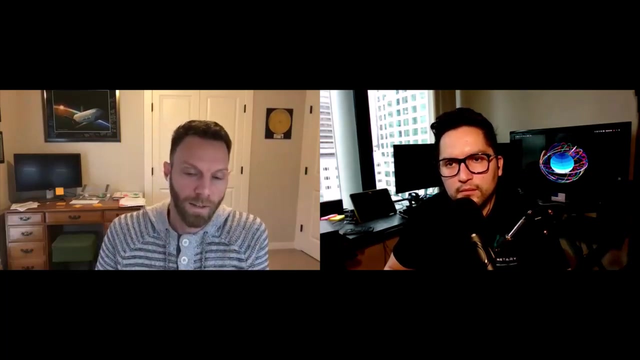 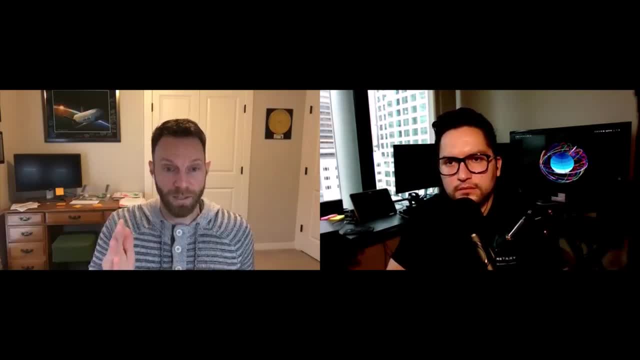 What you end up doing is just sampling your system hundreds of times or thousands of times at every sample. 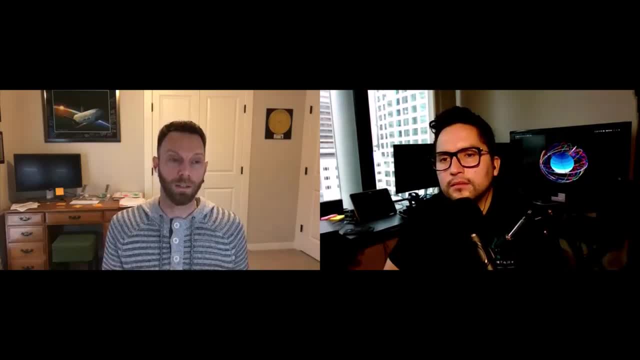 Every time you, you create a new instance of your simulation, all of those variations are tweaked according to their own probability distributions. 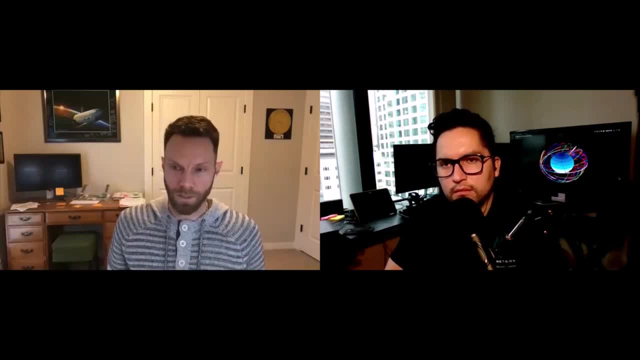 And so that as the number of samples goes to infinity, you will have simulated your system in every possible feasible configuration. 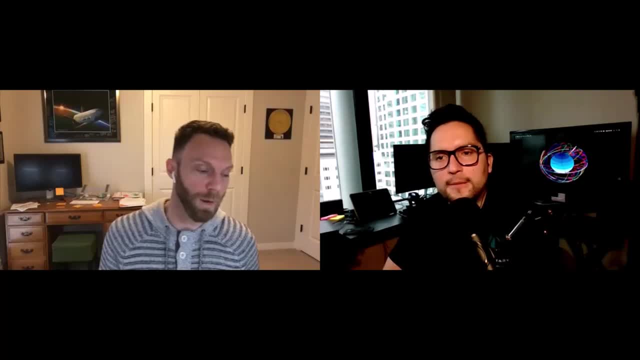 And that, that, that, that exists, obviously that's impossible. So what you aim for is enough runs to get a, you know, statistically significant swath of the entire state space. 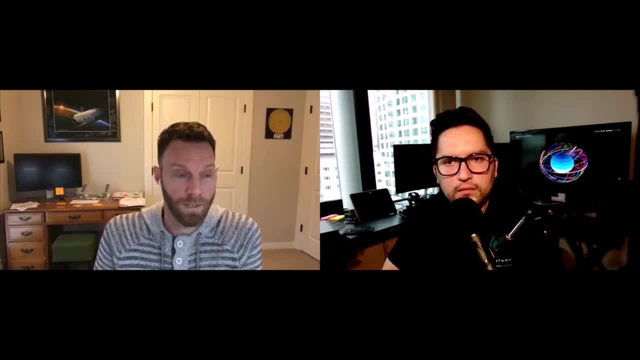 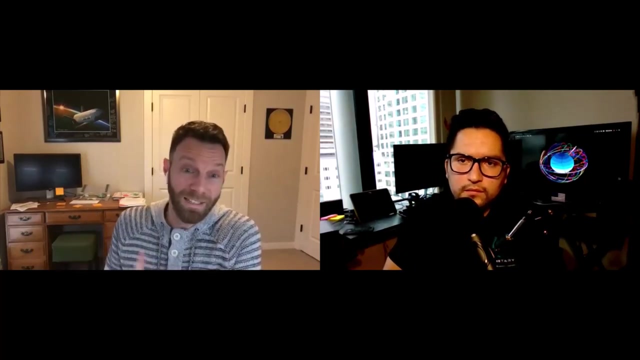 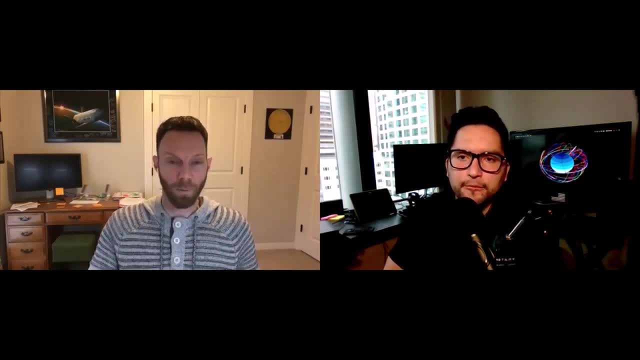 There's three configurations out of a thousand where I miss my pointing budget. Well, that's where the statistics come in on the requirements because the requirements 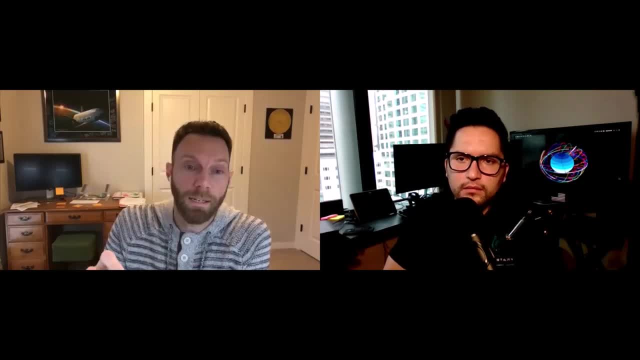 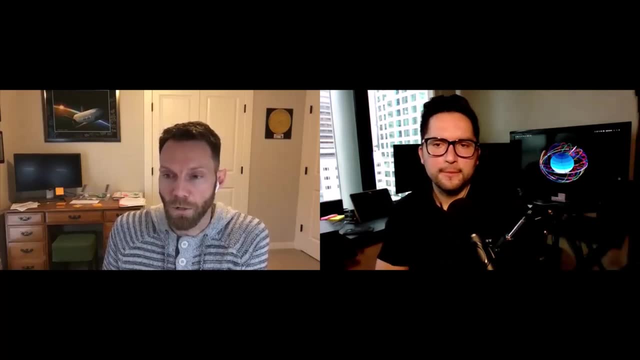 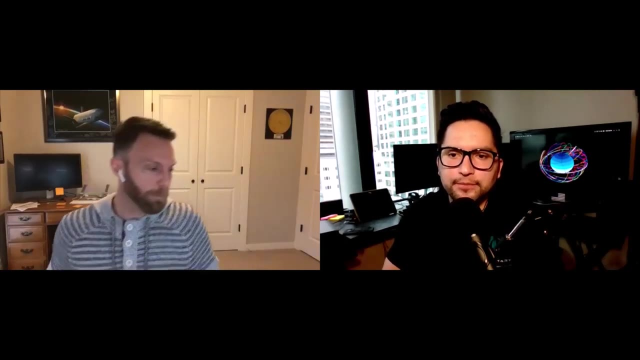 might say, I need to meet one degree plus or minus three Sigma. And what that's saying is like, you know, or, you know, three, yeah, one, one degree of three Sigma is basically it's saying like three out of a thousand times, it's okay that I missed that as long as the other times I'm within, you know, I'm within my, my requirement. 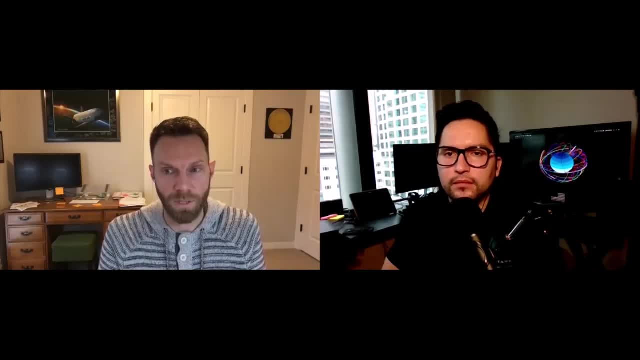 And so that's what Monte Carlo is good for. It's, it's allows. You to set up your simulation with all the probabilities of everything that you think, and then just brute force run through a whole bunch of different variations and, and get statistics on how well your system does. So as long as you have good enough models for all your systems, all these, um, kind of statistical variations of every single component of your system, you can create kind of, as you said, like a brute force state space where you say this many times out of this many times. And is that. Enough to be able to convince a whole team or to go forward with a design that says this system will work to this percentage of certainty. 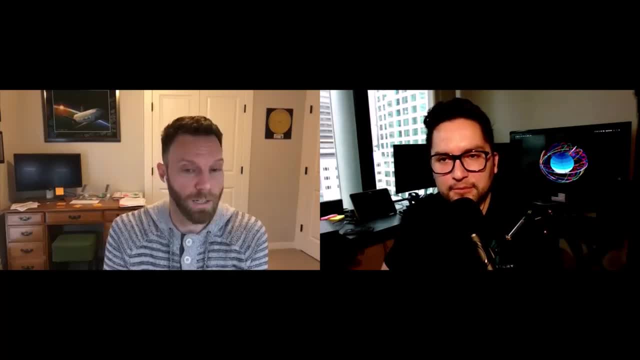 Well, you sure. I mean, it's the same as anything, right? It's model based design. 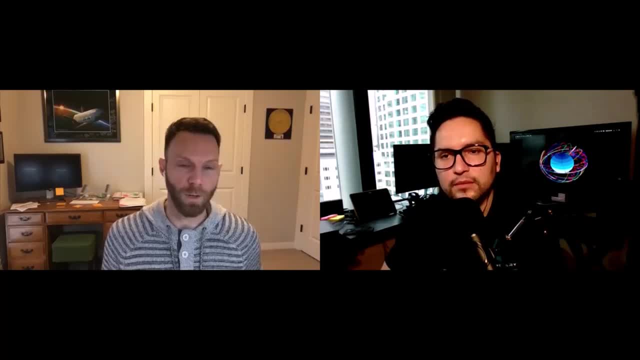 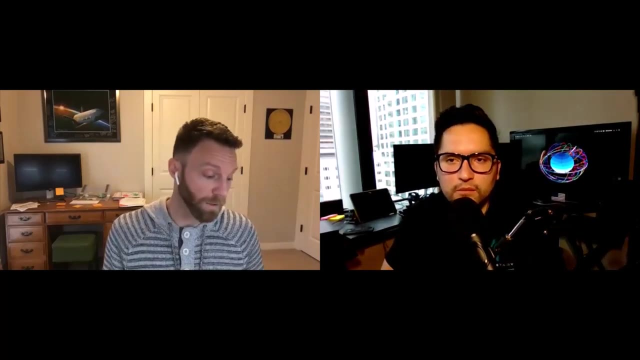 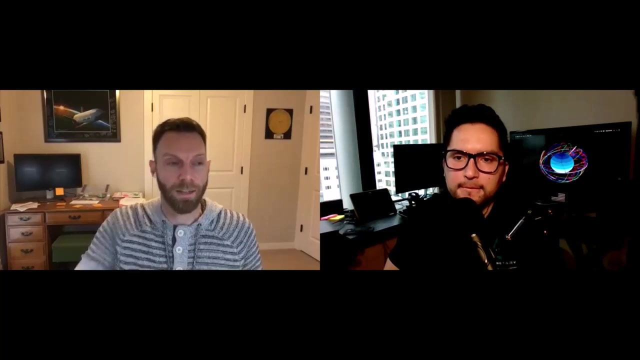 So it's only as good as your model. And so the majority of, if you have to go off and, and defend your design, if you do model-based design, a lot of your defense is going to be in defense of the model, and you're going to say, here is why I trust this model. I compared it to this physical hardware in this situation. I compared it to this peer reviewed paper in this other situation. I compared it to what project X did last year, you know, whatever it is. And you're like, I've, I've gained trust in this model. Um, here are the, here are the parameters I varied, and these are the statistical distributions that I chose and why. 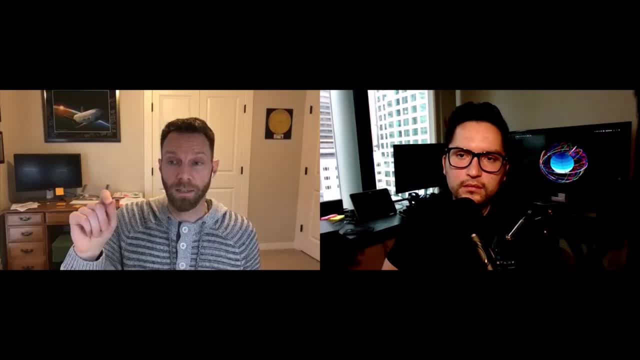 Okay. And these are the parameters I didn't vary because I, for whatever reason, I did a sensitivity 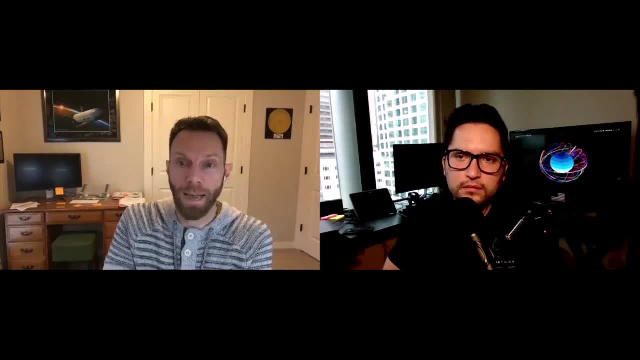 test on this one parameter and it didn't seem to impact the, the, the design at all. So I've ignored that. This one isn't on in this mode. So I've ignored that. Right. And you just like set up a defense. You just say, here's why I trust my model. 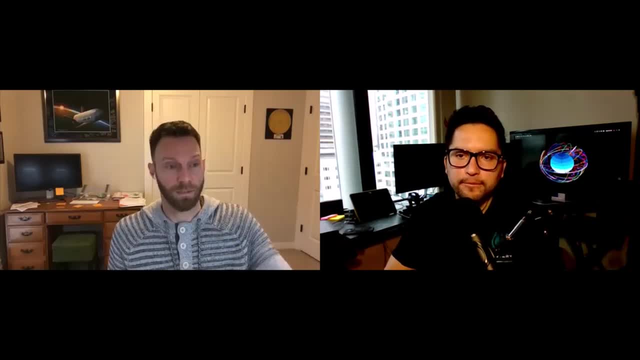 Here's what I did. And then here are the results and this, you know, and then, then you get peer reviewed in, right. You get external auditors or people that, that, um, you know, know what they're talking about and haven't been involved in it day in and day out to come in and say, oh, but did you think about this? And then you say, yes, I did, or no, I didn't into whatever. And, and eventually, you know, you've convinced yourself and some, you know, independent auditors or whatever it is that your company or has decided to do, um, you know, to gain trust, but Monte Carlo is no different. 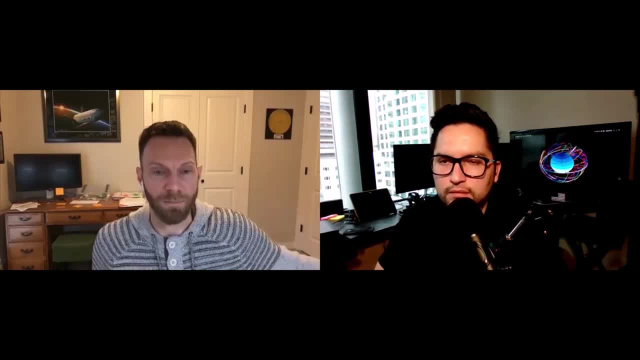 Then model-based designing your control system to begin with, right. It's it's, do you trust your model? 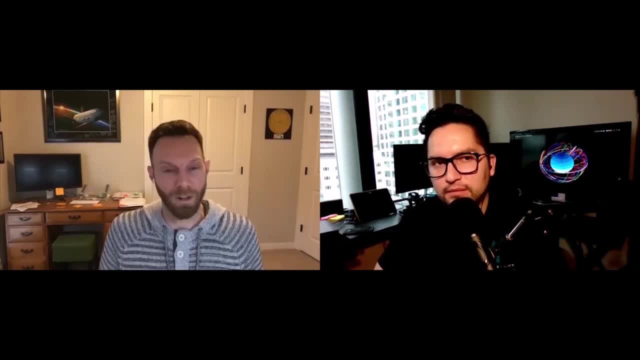 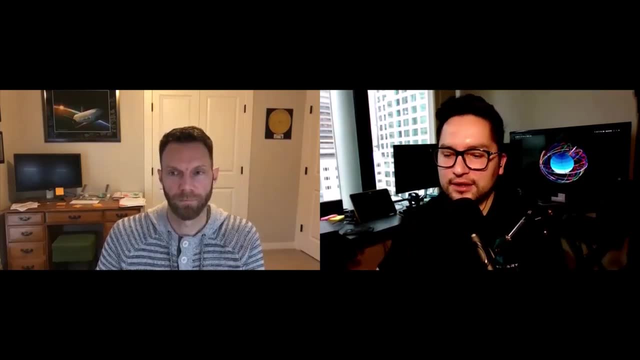 And if you do, then essentially all you've done is run your model a thousand times. It's kind of the balance of knowing. 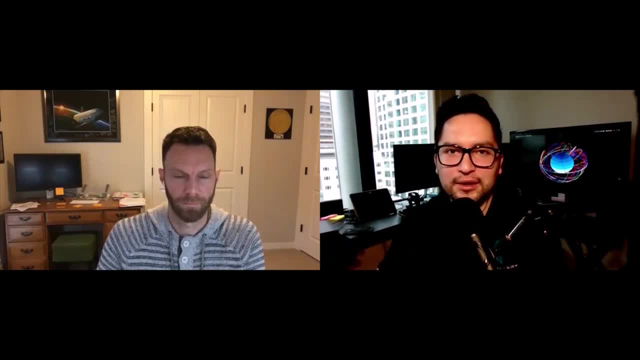 So say you do a lot of work in Simulink and MATLAB. So the balance of knowing all that Simulink and MATLAB versus actually knowing what's going on underneath the hood, because they're both very high level languages that you use. As a, and just like Python versus as opposed to say a C or C plus plus or Fortran, so kind of that relationship between being able to work very proficiently in Simulink and making these very complex models versus actually getting into the weeds of knowing what's going on as to actually how it's being implemented into embedded software. 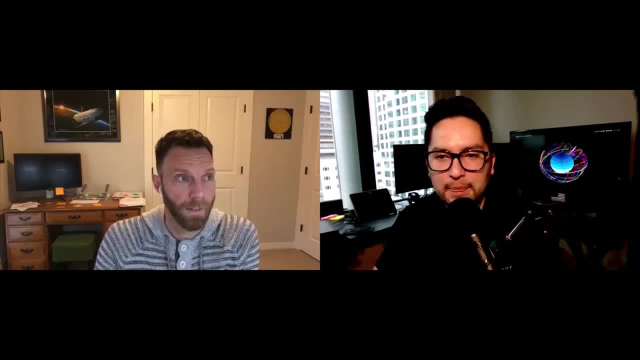 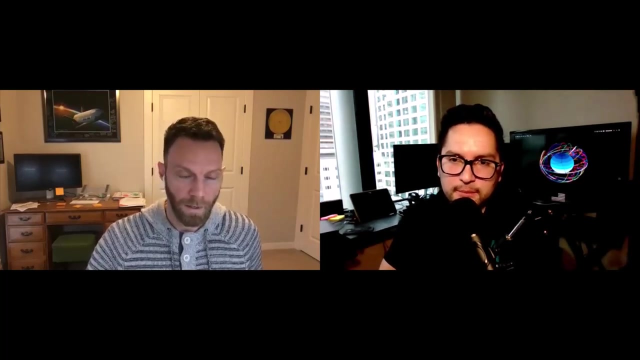 Well, um, I, I, I think it comes down to where you want to spin. And your time, um, I'm not a, a software engineer, but I would imagine that if you could include a library of functions that does what you want it to, that you want to accomplish, that's going to be preferred, especially if that library has already been vetted, um, and used and documented. That's going to be pre preferred over writing. Right. Right. That's going to be pre preferred over writing your own code from scratch. 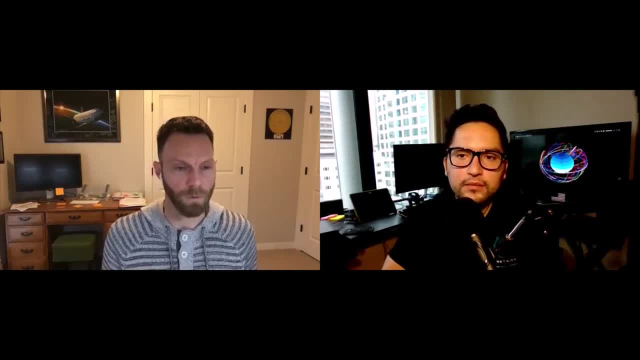 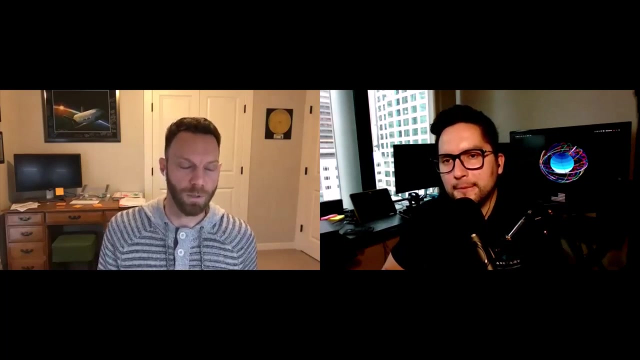 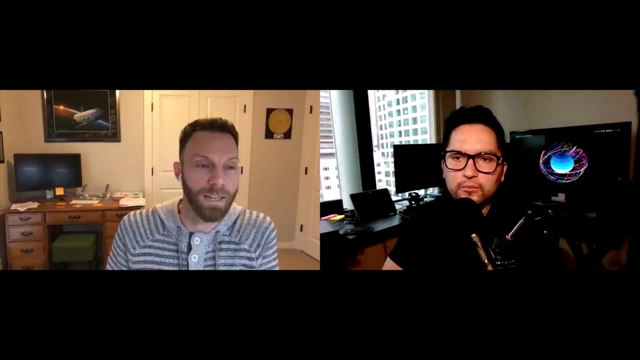 Um, in a lot of cases, I mean, sometimes libraries don't exist and you have to write from scratch or you're doing something highly specialized, or you don't want all the bloat that comes along with, you know, some kind of built-in function, but, but for the most part, um, you want to reuse things that have already been created and reusing something shouldn't preclude you from understanding it. keeps you from having to write it yourself and keeps you from making the same mistakes that everybody makes whenever they do anything right just you know they don't understand they forgot to include something they made a typo whatever and so it just saves on time there but i wouldn't advocate anybody include a library or something else that was already written without understanding what it's doing and so now when we get to matlab and simulink i think of them as as libraries of algorithms and an ecosystem that allows you to connect them and simulate them and visualize them and generate embedded code from them uh in a way that is simpler like you don't have to spend as much time doing it as you would if you did it you know yourself um you know you know from scratch in some way and it keeps you from making those kind of same mistakes but i wouldn't advocate for anybody you . 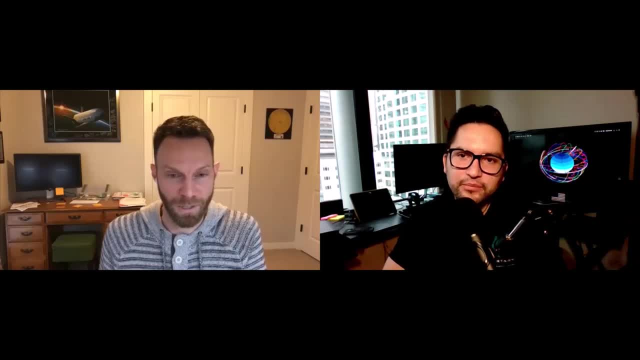 connecting blocks and simulink and writing in some matlab code and functions without understanding what's going on um underneath it you can absolutely do that right that's but you 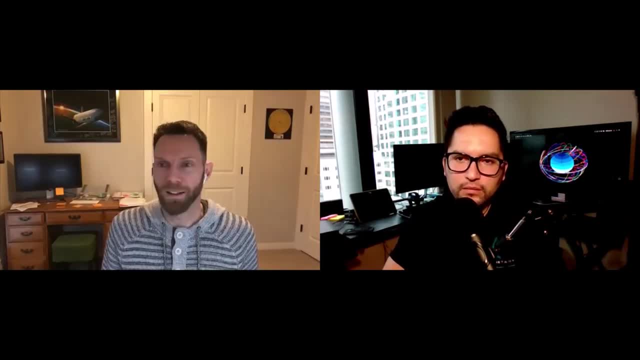 can do that with anything you could you know you could uh put a bunch of numbers in excel 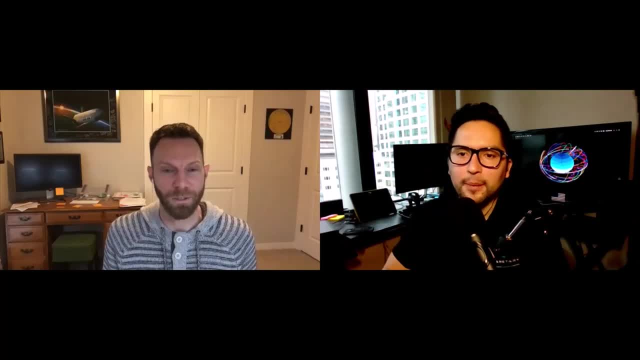 highlight it and say plot a linear line and give me a linear regression give me a best fit line and you can run off with it and you could be pretty successful with it but if your job depended on that answer 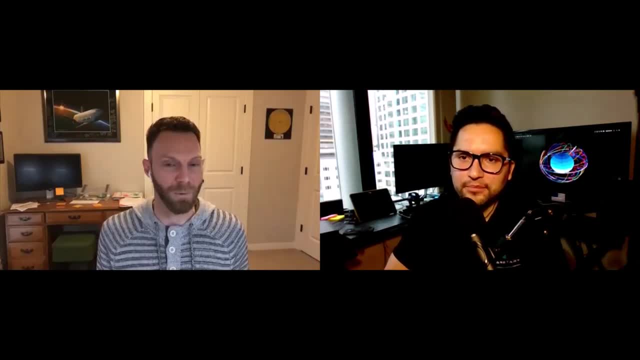 i would spend a little bit of time understanding what is this thing even doing you know what is the what is you know what is linear regression and understanding it and that's what i would advocate 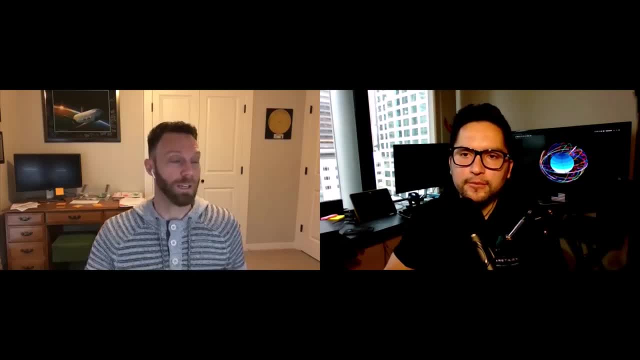 for using matlab and simulink um also it is a fantastic tool and it's a fantastic set of libraries but it shouldn't be used um like blindly because you can get yourself into trouble if you just say oh this is a three degree of freedom block let me just pull that in and move on because you don't quite know what it's doing all the information is there you can find out it's not like a black box 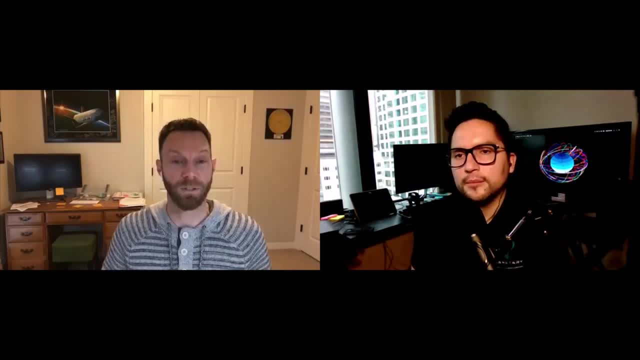 um but it just keeps you from having to write all of that stuff yourself and and and research 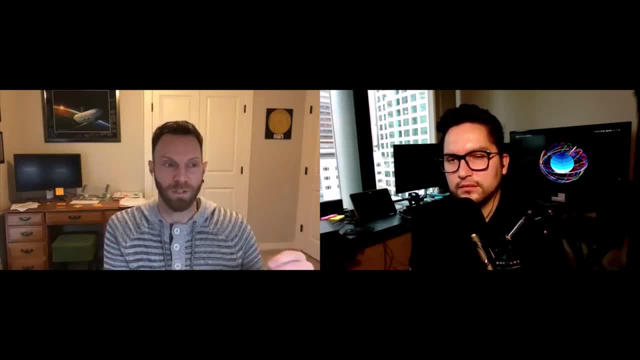 everything you can you can read all about it and know exactly what it's doing and figure out whether that is what you want to apply to your situation um but you're still going to understand what it's doing and then going off that 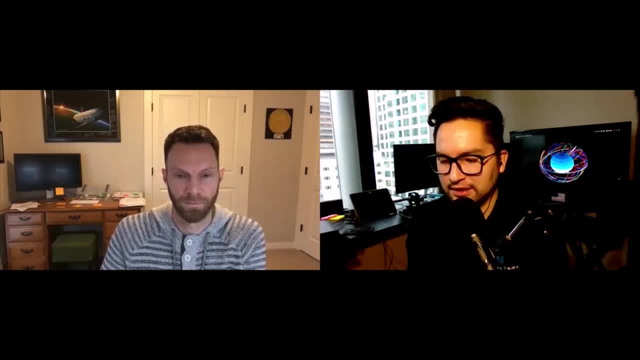 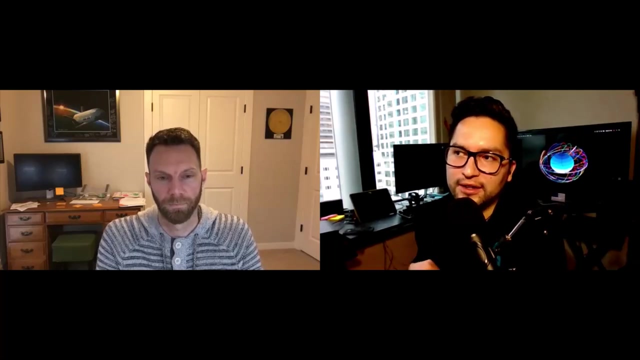 can you talk about a little bit of the trade between using the autocode feature of simulink and matlab versus say hiring a bunch of embedded software engineers who could also write that software and maybe interact with the controls engineers who are writing say control laws or general architecture of the flight software kind of where that trade goes and when you want to do when you want to rely more on say an autocode versus hiring a bunch of embedded software engineers 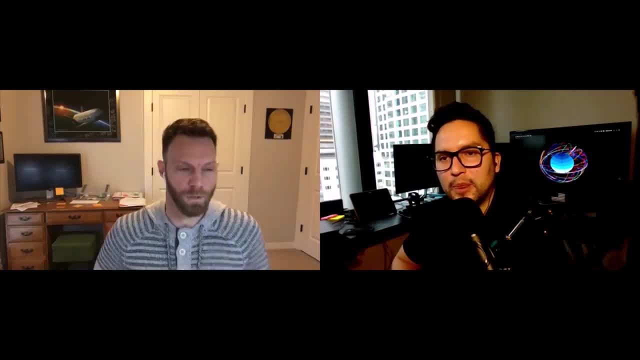 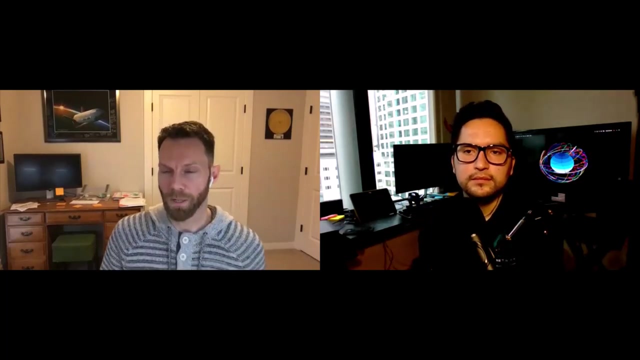 don't really i haven't given much thought into the trade outside of adc and s so this isn't a general statement um but from my experience um being you know control systems adcs gnc all of that stuff is a specialized field and you can get the basics pretty quickly but there is a lot of just of of 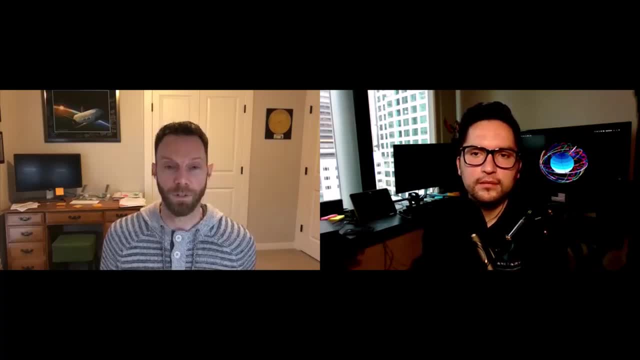 experience and breadth to this field that you have to know and understand in order to not sort of fall 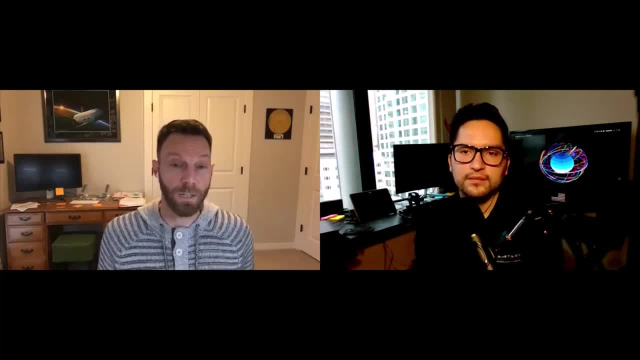 into the same pitfalls that people have been falling into for dozens of years you can learn from them and not do that and in order to learn from all of that it just takes you know some experience and study and and things like that same for embedded code right embedded code is a complex field like you could probably write some code pretty pretty simply that you know does hello 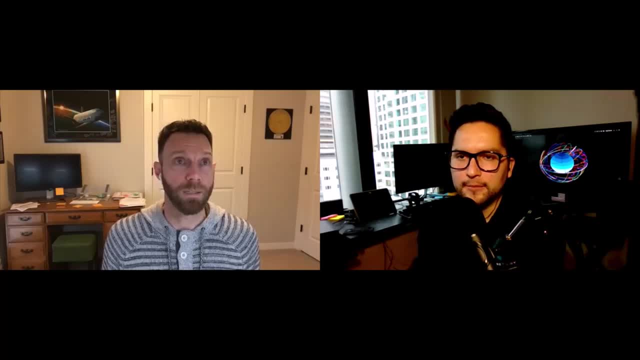 world or whatever runs on the embedded processor but you don't know if you're missing any any 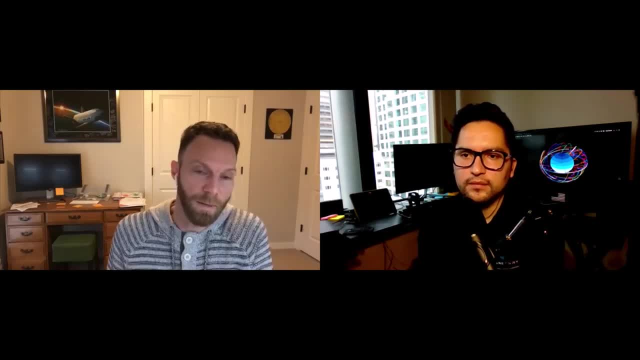 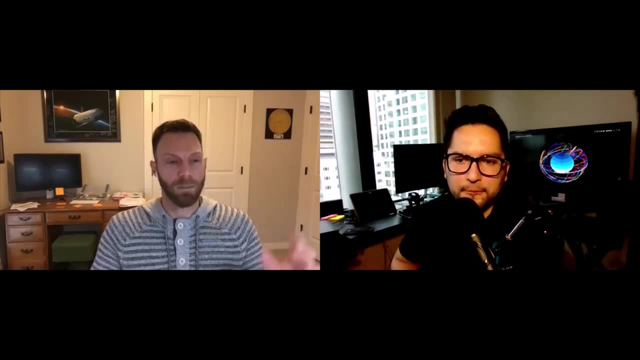 you know um best practices for example that that people have learned dozens of years ago and you're just falling into the same trap it requires a lot of expertise if you can find people that have both 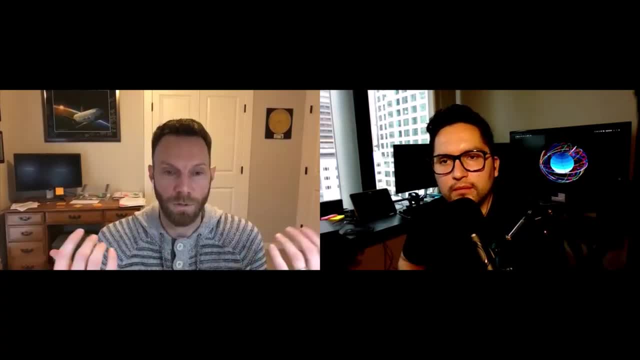 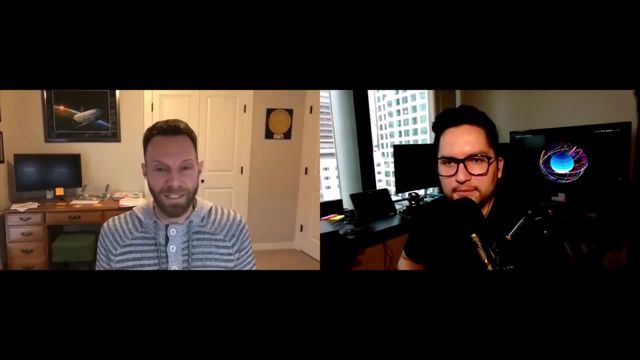 of those expertises that's amazing and you should do that and you can save you a lot of heartache probably to have the same person design these complex algorithms 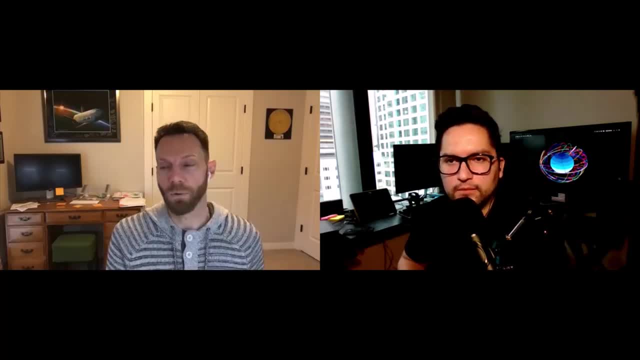 and then embed them into the flight software write it themselves do all of those testing but there's also some really fantastic adcs engineers out there that don't know code 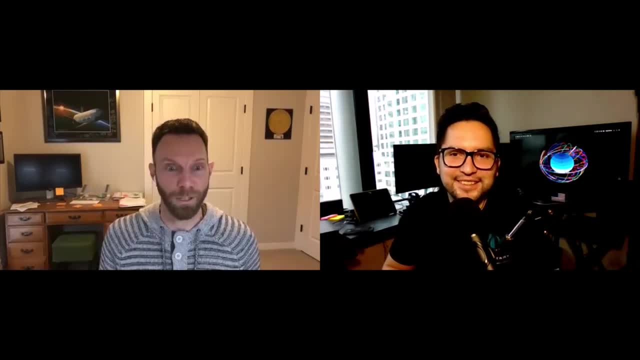 like me i consider myself i guess fantastic but terrible at code uh and then vice versa there's some great embedded code um software engineers out there that don't know enough about adcns 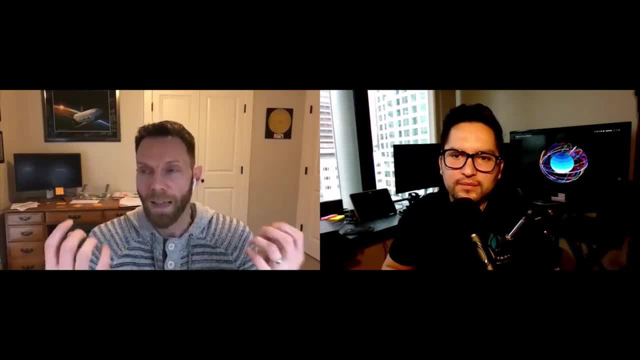 and so it's like okay well how do i bridge that world now how do i uh capture the knowledge that's on the web what's the best way to do it and then at the end of that process we get the 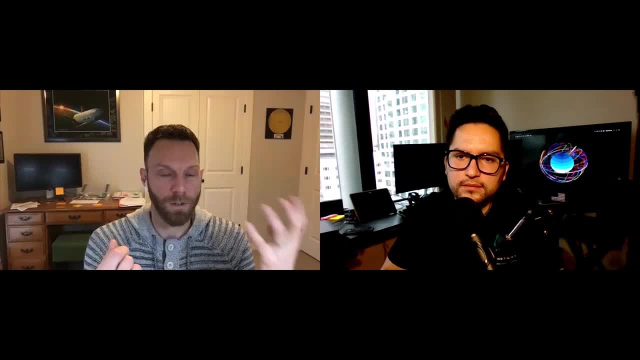 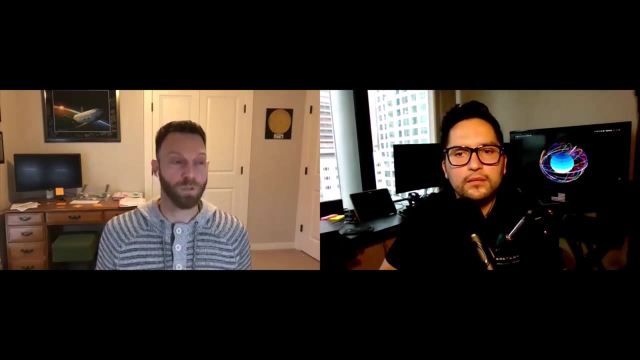 knowledge of algorithms and and adcs knowledge from one group and apply it to this other group that's actually doing the coding and at boeing at least one of the projects i was on we did that by writing what's called algorithm description documents which were just massive volumes of block diagrams and text that described what we wanted done in minute detail and we would take that avd that algorithm description document and hand it over to the software team who would then read through it and code it all up. 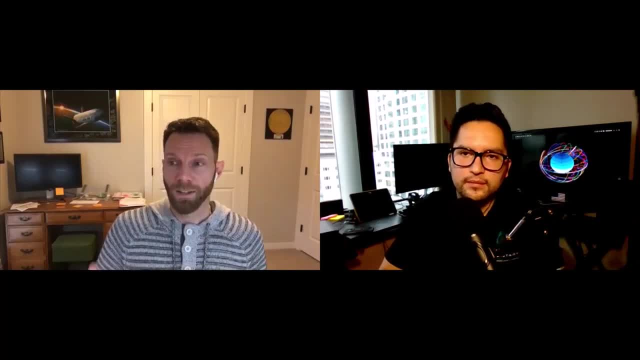 And it was terribly inefficient because we may have designed a perfect algorithm, but described it poorly. Or we may have described it well and they interpreted it poorly. 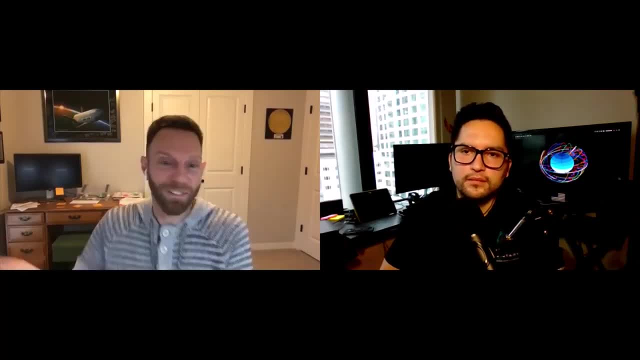 Or they interpreted it well and we tested it poorly. You know, all of a sudden you've added all of these places in there where error can creep in. 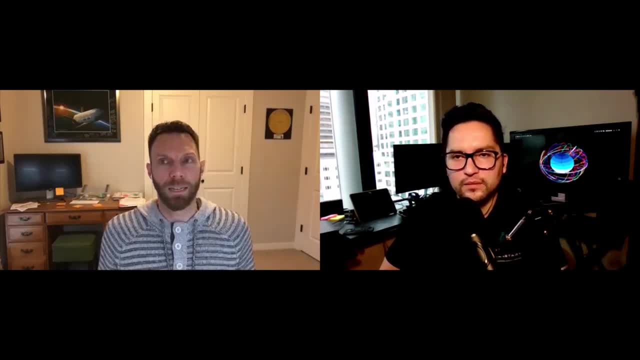 And so that's where autocode can be nice because it allows you to take the expertise of the person developing the algorithm, the capabilities of the software to develop to generate embedded code from that, and then the expertise of the embedded software team to wrap the rest of their flight software around it. 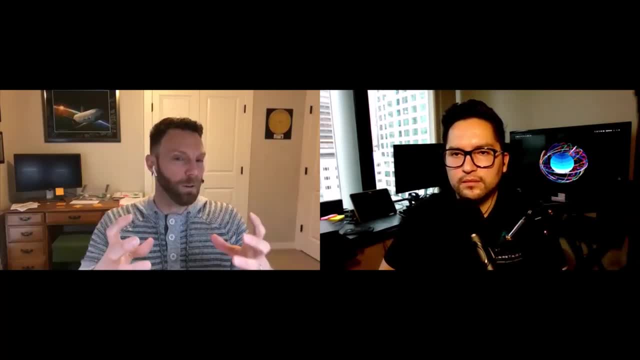 Now they don't have to be algorithm experts. They can take those algorithms, take it out. 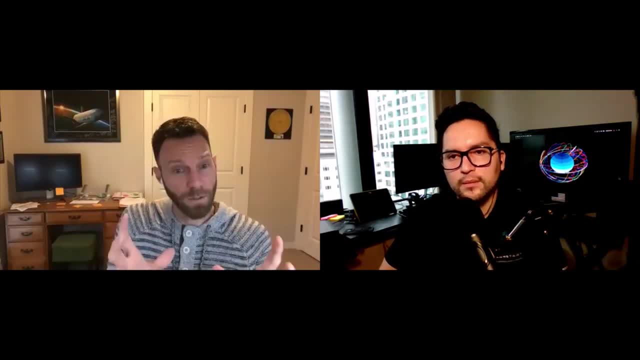 They don't even have to use the entire embedded code. They can take those functions and they can take those algorithms and they can take those functions that were generated and then just stick them into the embedded code that they're writing. 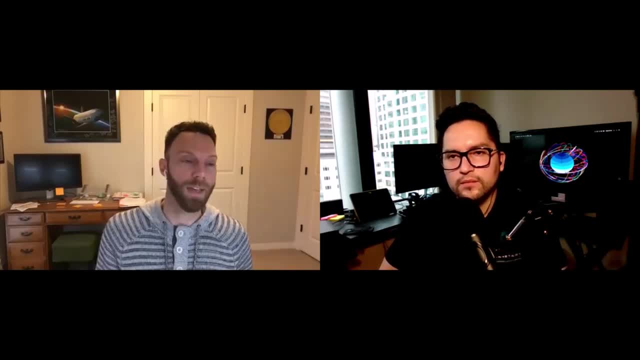 And they know all of the nuances and the details of hooking all of that up, but they don't have to be experts in the algorithm itself. 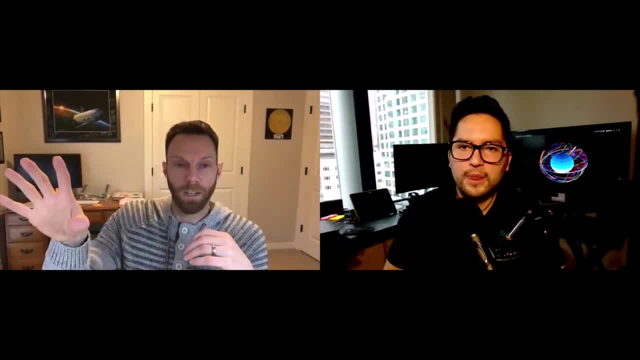 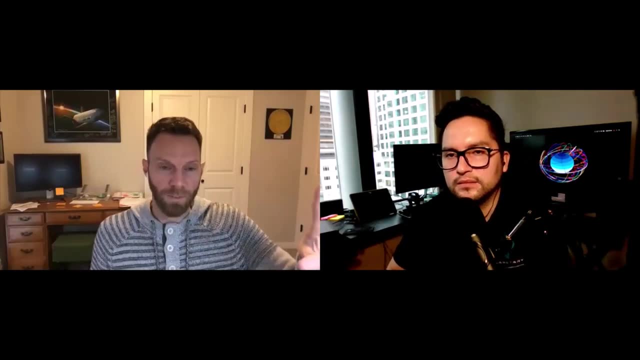 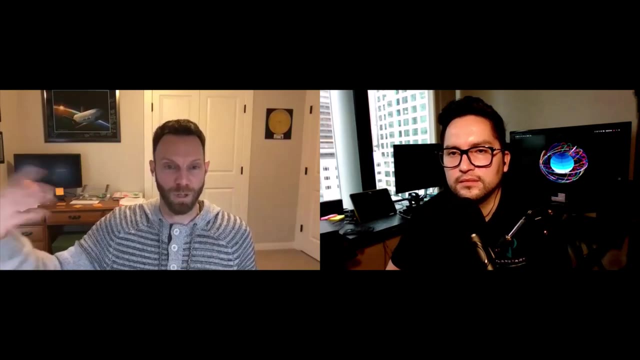 And now those two teams can work closely with each other with one developing essentially the source code in MATLAB and Simulink, if that's what you're using to do your autocode. The other one building flight software, and then you can get together to test it and say, hey, here's what my flight software is coming up with. Now, does that, does that match what MATLAB and Simulink was showing? And you can say yes or no and troubleshoot. 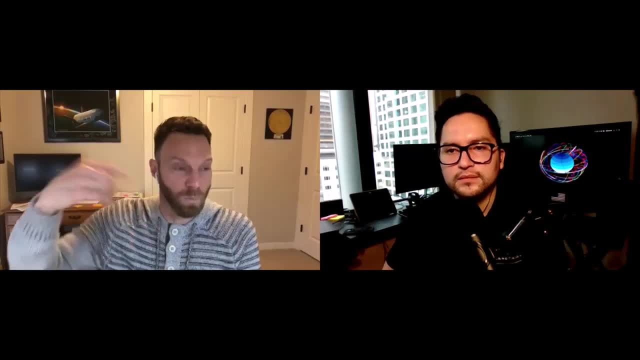 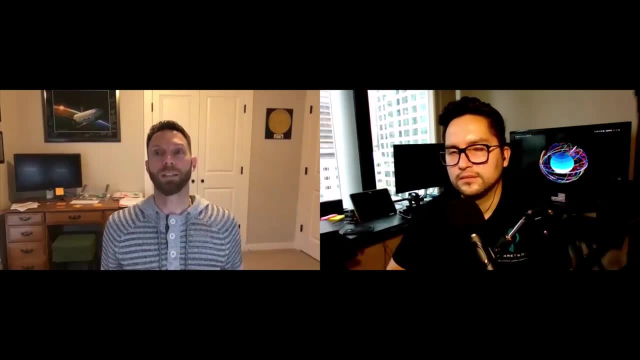 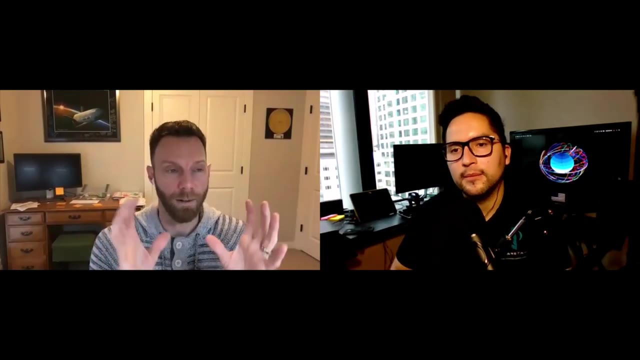 And then once you get that handoff done, then it's relatively easy to just make changes on the Simulink side, autocode, pull into the flight software and you're off and running. And it's a nice way to bridge the expertise of these two groups without requiring these highly specialized employees that are experts in both. Let's shift into your videos. 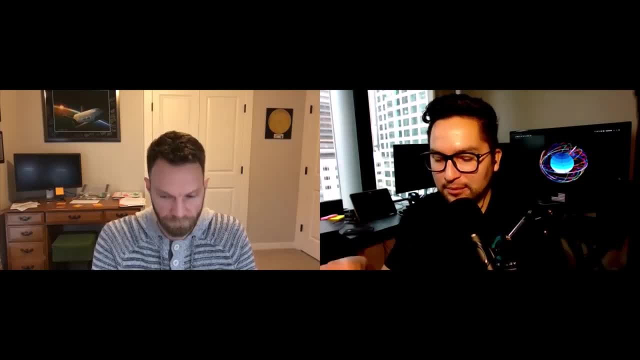 So in the early days, first of all, what prompted you to start making videos in the first place? Yeah, because I don't even, that was a really long time ago. So yeah, so I guess way, way back then, what was your name? It's making me seem old. What was that? Yeah, go ahead. 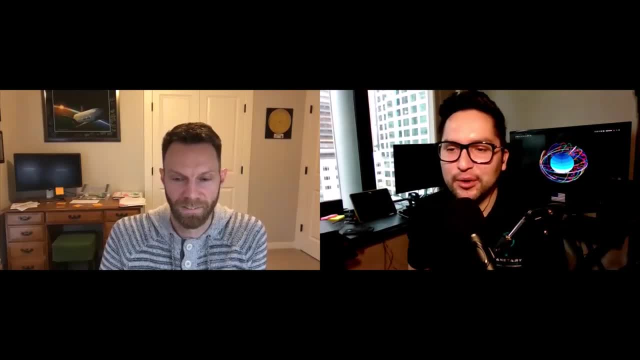 Go for it, sorry. Oh, just, yeah, just what was the kind of motivation that says, okay, I wanna teach people, I suppose, or? 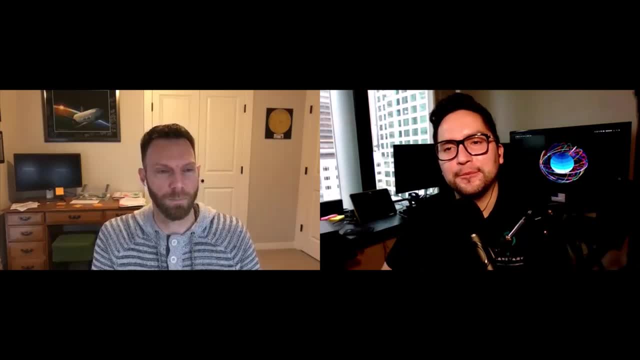 Yeah, well, I've always wanted to, I've always enjoyed teaching. So that's been around forever. 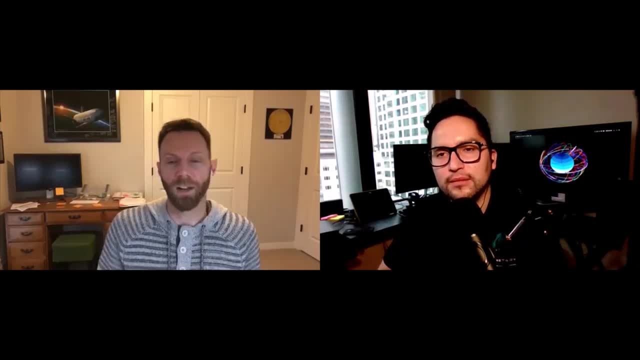 And I always thought I would go into industry for some amount of time, learn a bunch of stuff and then go off and teach. I didn't think it was gonna be like this. 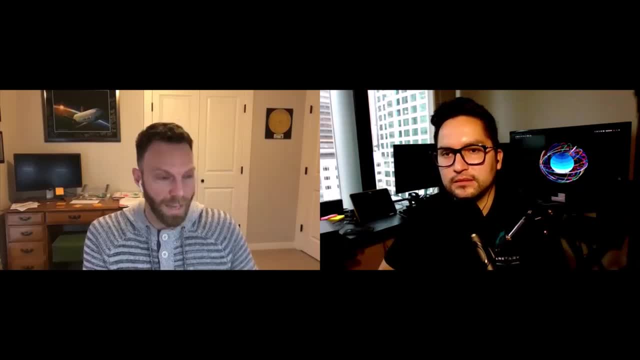 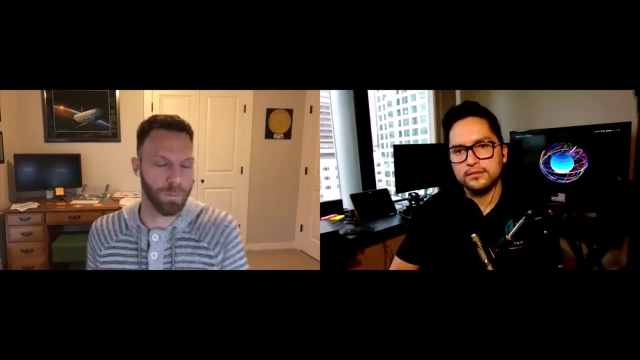 But the genesis for my videos actually came when I moved up to Seattle with Boeing. My cubicle, like next door cubicle mate was a man named Monty Evans who worked triple seven flight controls for a long time and was just, really smart in understanding control theory, specifically frequency domain classical controls, which I had very little experience with at the time. 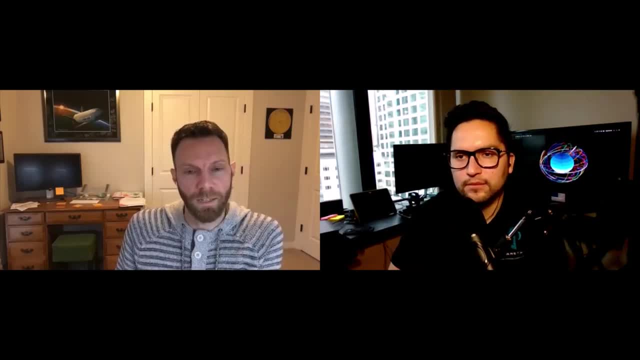 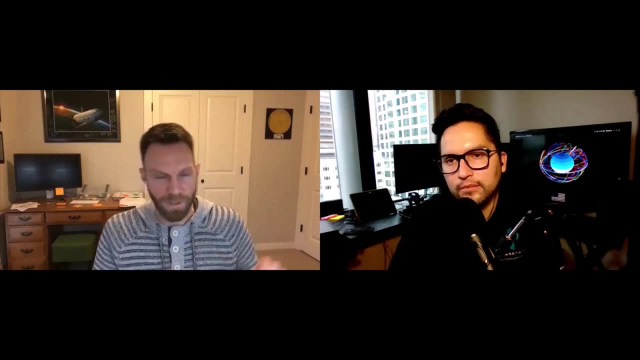 And I lucked out because I was right next to him. And not only was he really, really good, he had a good intuitive grasp on things and he liked to answer questions. And so I would have a question for him and then he would come over and he'd write it down. He'd say, oh, you gotta think about it. You gotta think about it like this. And it makes more sense if you do this. 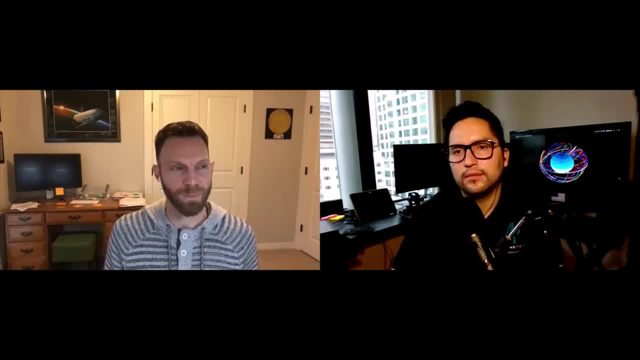 And I remember thinking, man, this was such a good explanation. 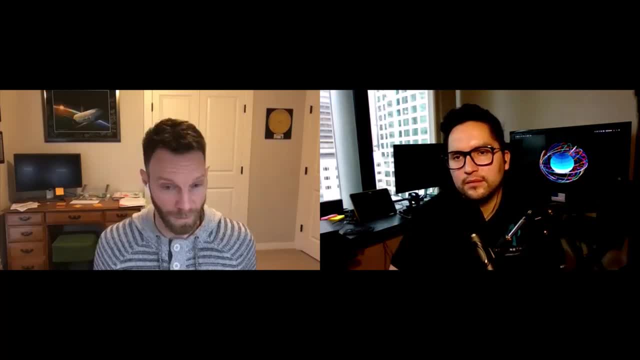 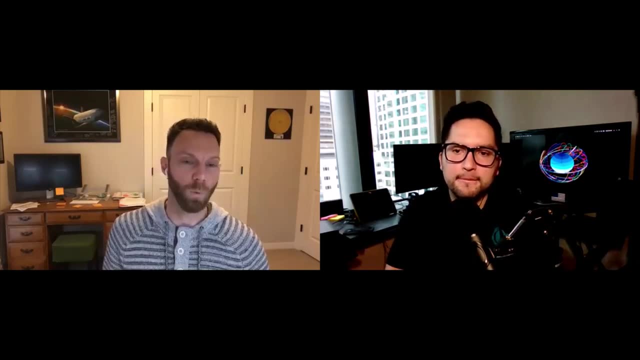 If I just had that, the math would make a lot more sense, right? Like I spend so much time trying to learn this math without having a good understanding of what it was before I got into it. 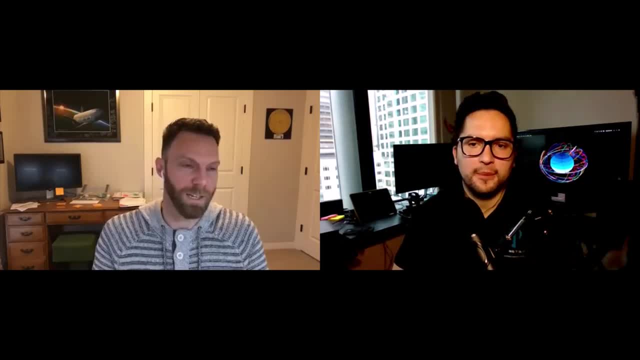 And so I thought just for my own sake, it wasn't intended to be this big thing on YouTube. 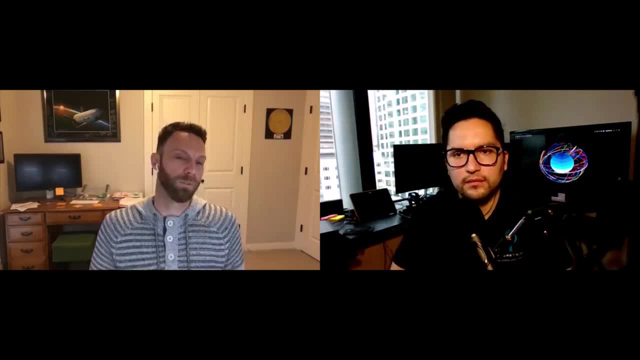 Just for my own sake, I wanted to kind of, walk through a few concepts in the style of Monty, of how he explained it to me, where I set up the problem, not from a mathematical perspective, but just from an intuition perspective and say, this is what we're doing and this is why it makes sense and what it all means. 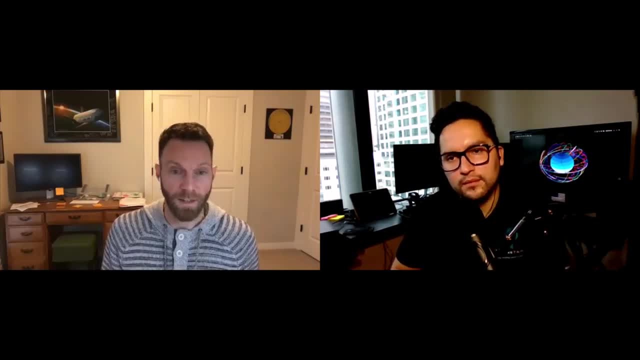 Now you can go off and read the textbook and hopefully it'll all make a little bit more sense, right? 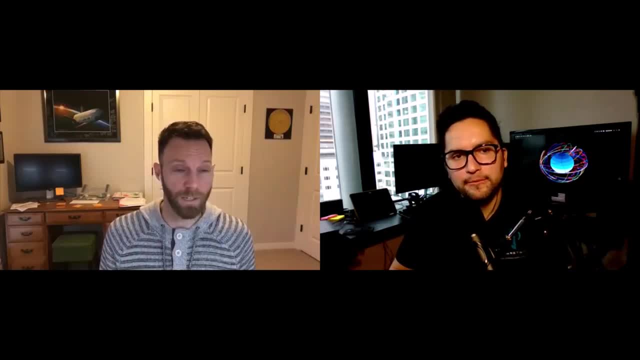 Not go into the math, just stay with the intuition. And I made a couple of videos. 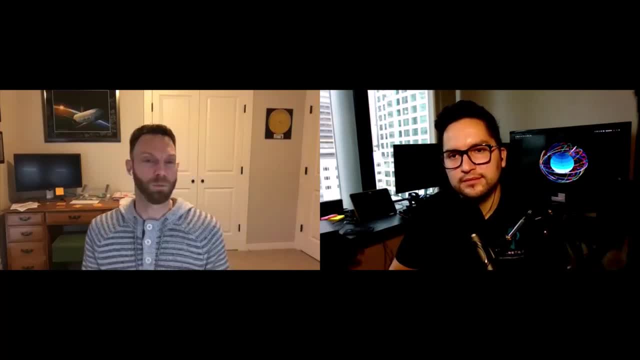 And then I got comments that were like, you know, I got like 11 views or something, which was amazing. And, you know, I got a few comments of like, hey, I'm looking forward to the next one. It was like, well, I hadn't considered it next one, but maybe I will. 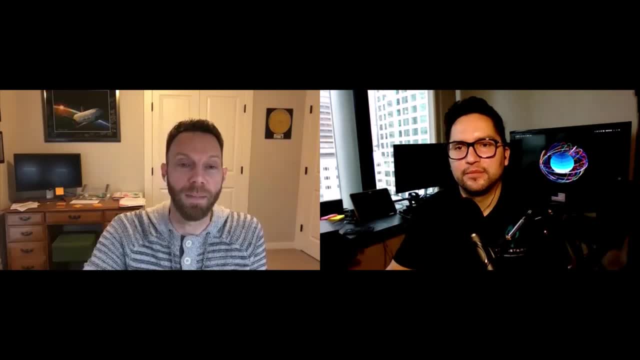 And so for the first year or so, comments really drove me to keep making more. I would talk with Monty and other people and I'd kind of craft a story. And then it just sort of took off from there. It was always a hobby. It was always something I would do on nights and weekends or something to come back and fiddle around with videos. Oh, this was great.